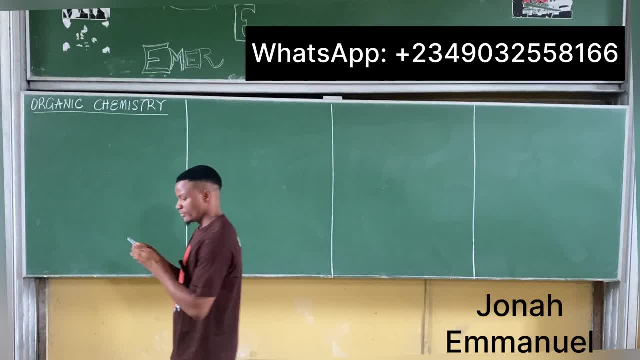 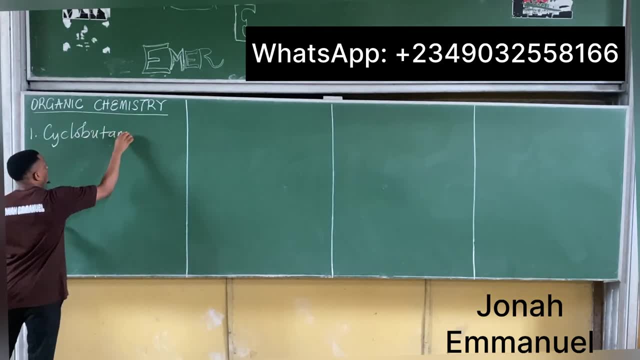 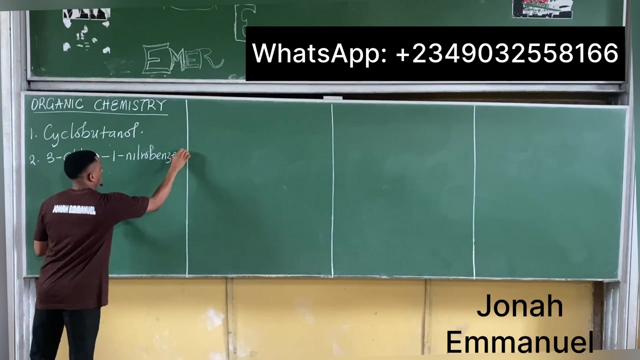 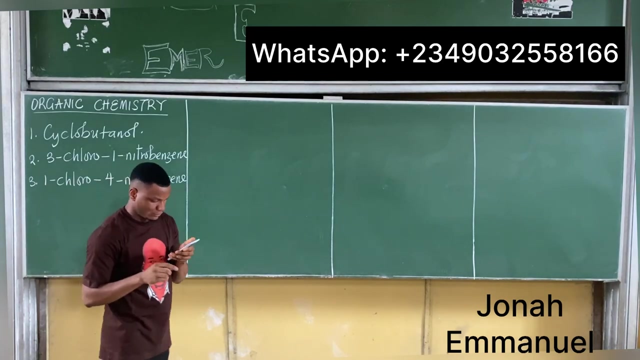 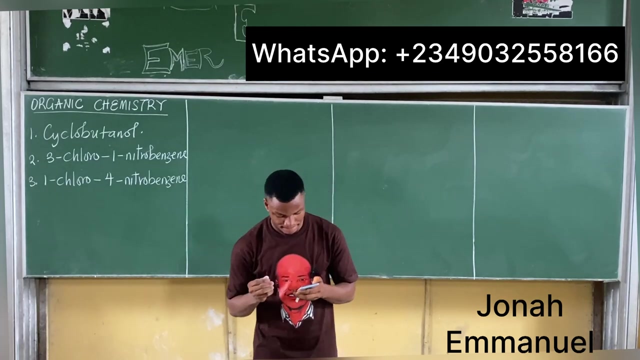 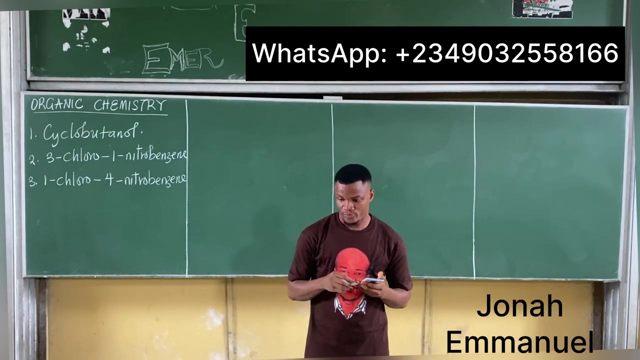 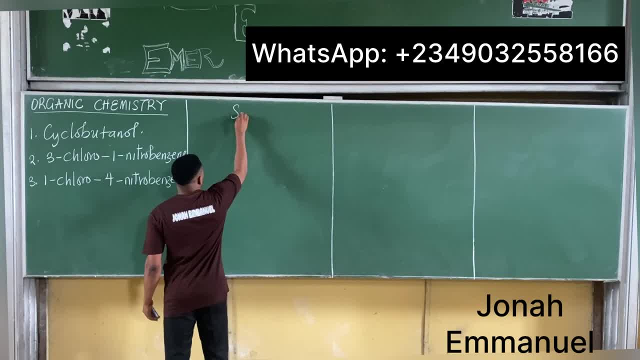 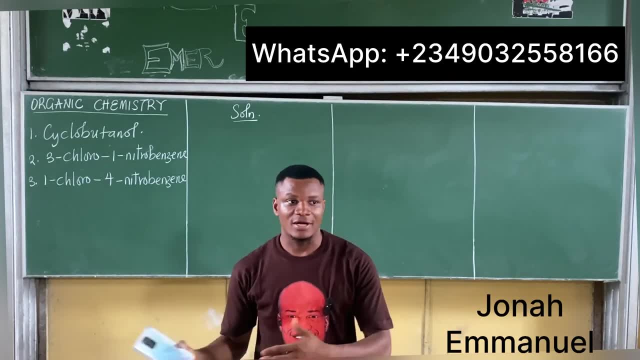 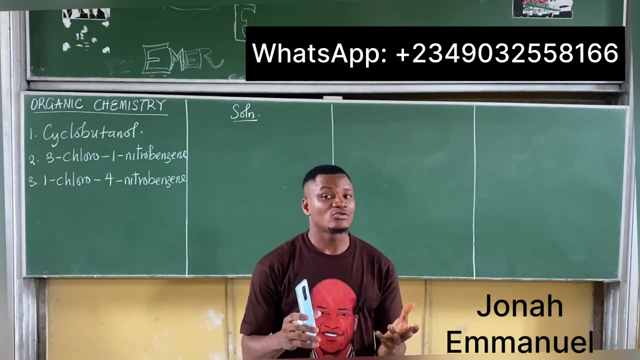 with this place? Um solution. if you're used to my classes, what I do is this: before I solve. I will allow you to attempt it first, Abhi, before I do it, But for time's sake, considering our scope, I won't do that one like that. 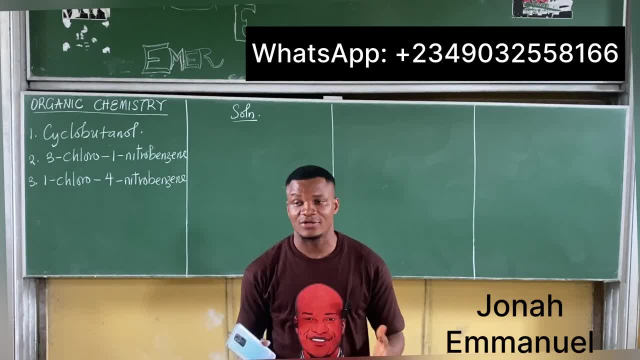 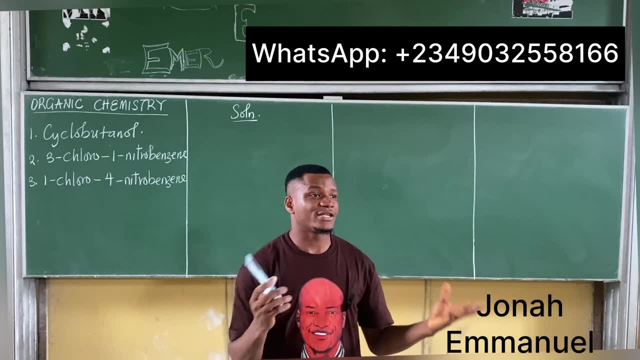 So I'll just go straight. If you have a question, just answer. Just sorry, ask right. I won't give you time to start trying again because of time. Um, I'll just be doing it. If the party don't understand, call my attention. 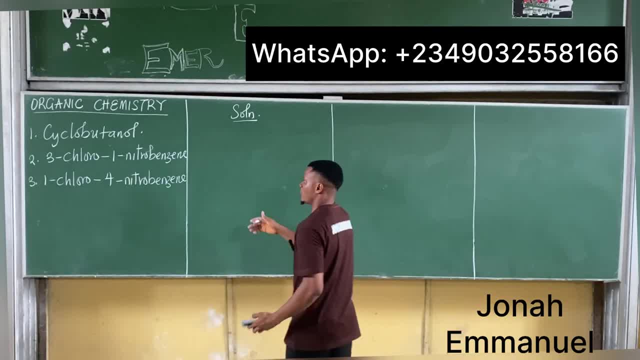 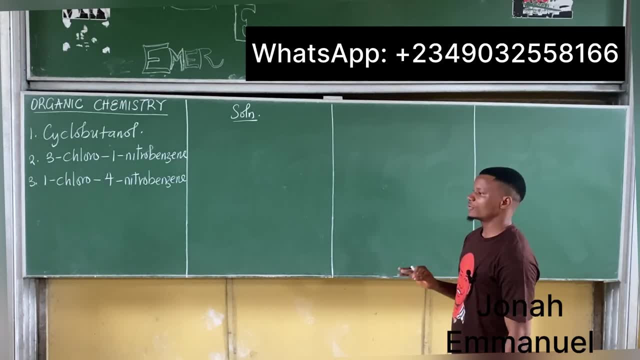 Just raise your hand, I'll get to you. All right, first things first. uh, we have to draw the structure: Cyclobutanol: three chloro, one nitrobenzene, one chloro, four nitrobenzene. 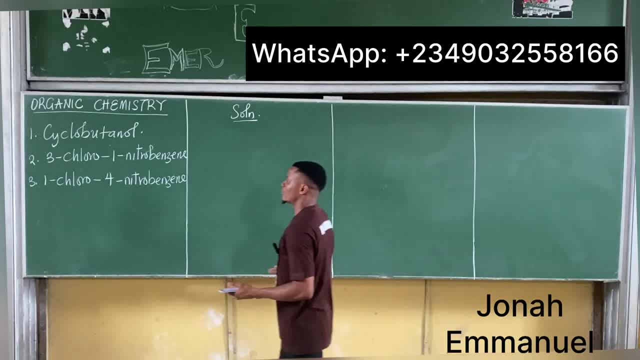 So here's the tax list. First things first. I have a cyclobutanol. The term there says cyclo. We've argued that when we want to compound it's cyclo. What does it mean there? It means it's what there? 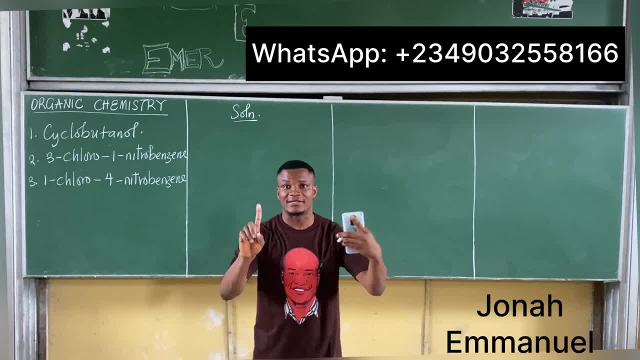 In a ring format. that's all. Cyclo means it's in a ring format. Next up I'm seeing a but Butanol When we say: but how many carbon there? One, One, Four carbon. So this simply means get four carbon. 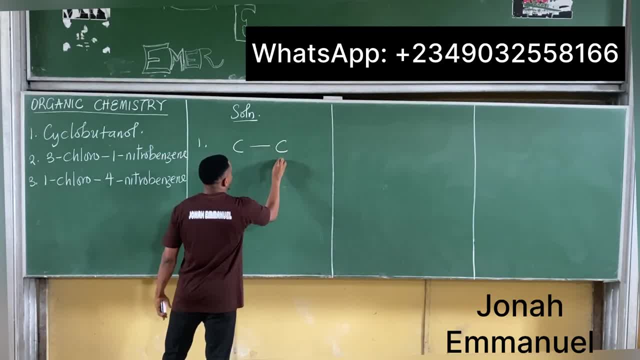 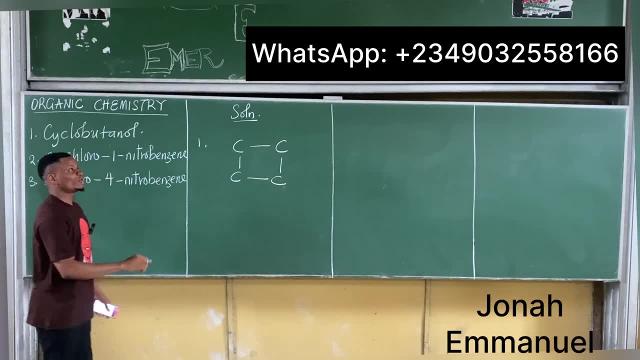 The first one there, cyclobutanol. get four carbon and it should be in a ring structure. This is cyclobut. This is cyclobut. The next tax that I have over there, an anol or arcanol. 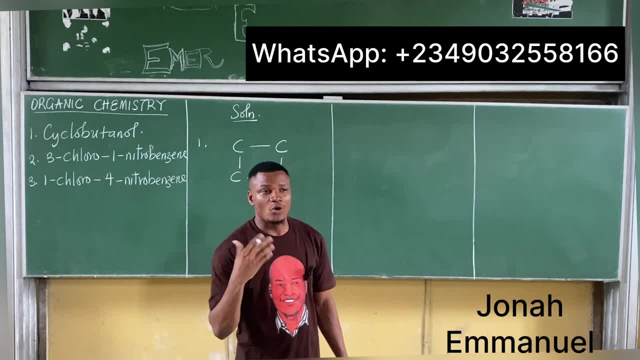 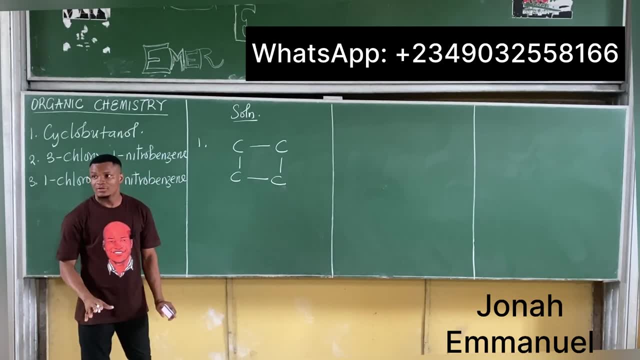 For your arcanol. how do you identify arcanol? The OH group? So it should now be: where do I put OH here? That's the question. Put it anywhere. So if I choose to put OH here, it's correct. 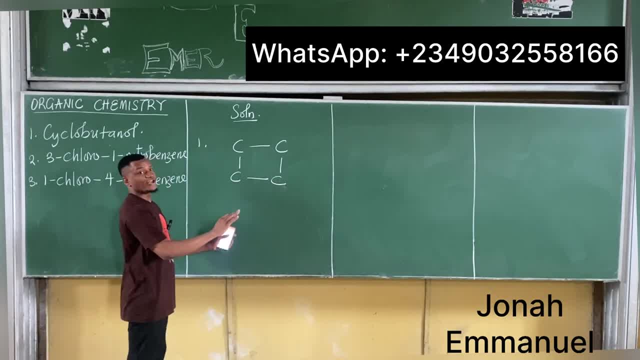 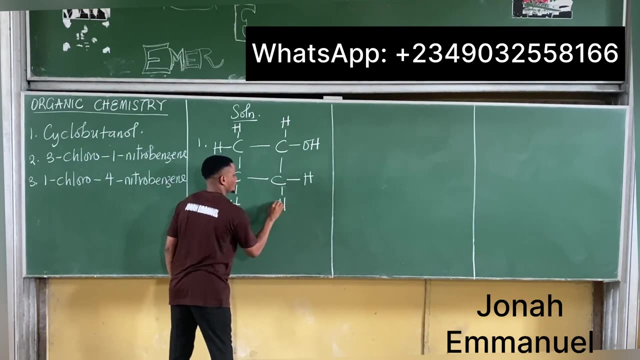 If it's here, it's correct. If it's here, it's correct, So put the OH anywhere, It's correct. So I'm coming here, I'm doing OH, I'm having All right, So that's all, please. 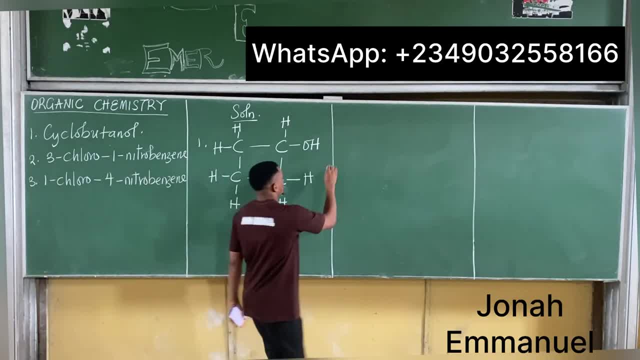 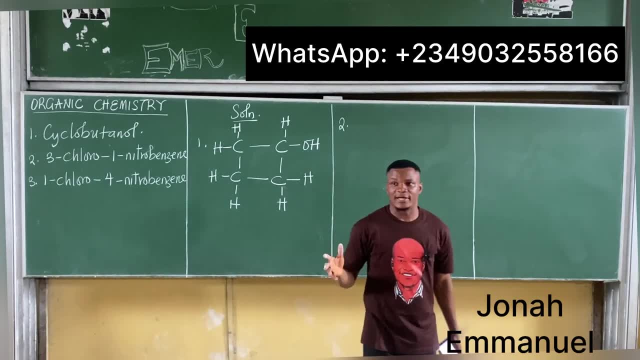 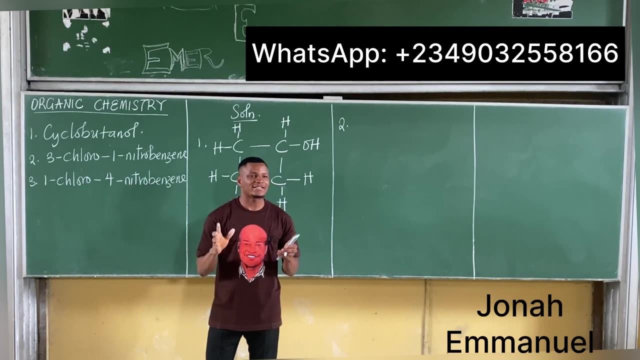 This is cyclobutanol. That's all. Number two: that's cyclobutanol. Number two: I have trichloronitrobenzene. Please, you are pleased to draw any structure Depends on noting which of them is the parent atom. 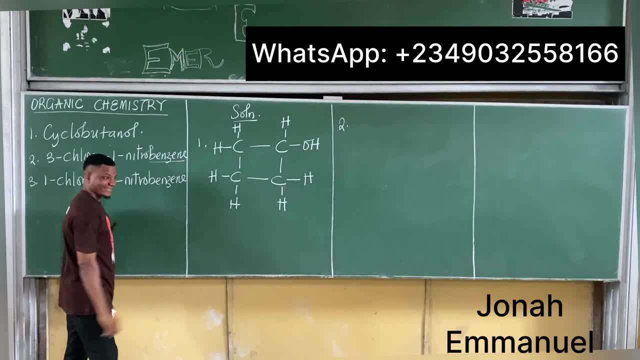 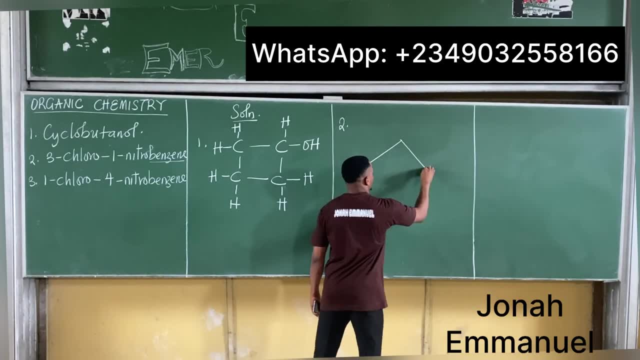 In this case here my parent. that's what Benzene? It's benzene. So first things first, draw a benzene ring. For my benzene ring I'm having this. this, So here is okay. it's not complete yet. 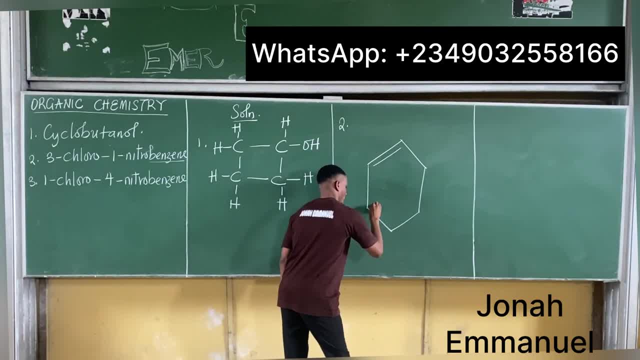 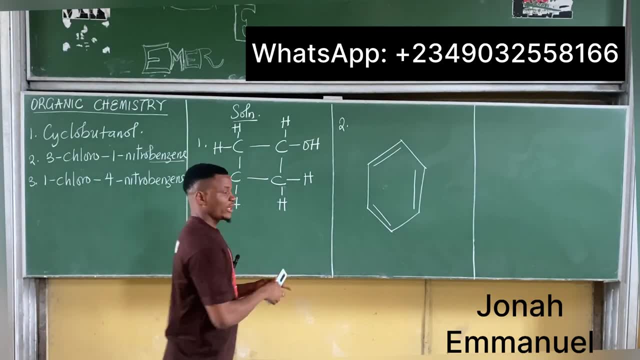 I'm having here, here, here. So here is a benzene ring. So this is called Kekulé structure. You can choose to put these two here and this one here. Is this correct? It's called the localized pi bonding. 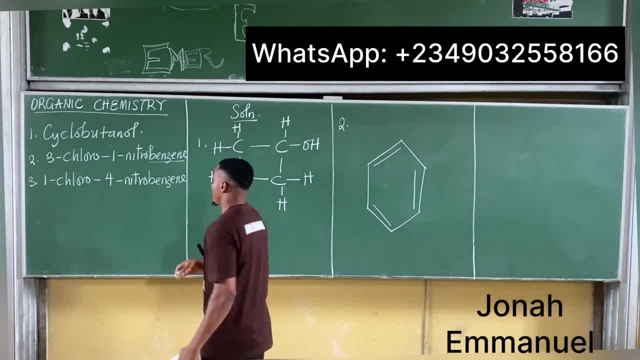 All right, You can take it at any position. So this is my benzene there Next up I'm having a look up this. I'm having a nitrobenzene- One nitrobenzene please, So put your nitro. 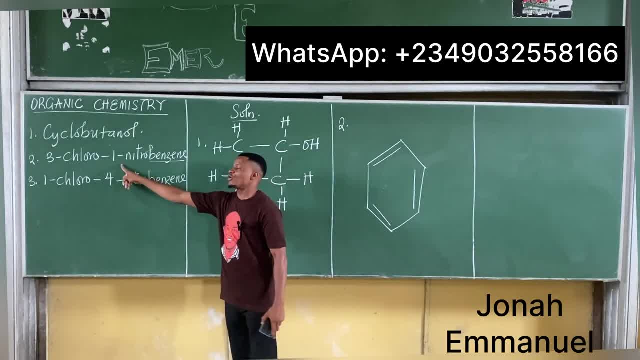 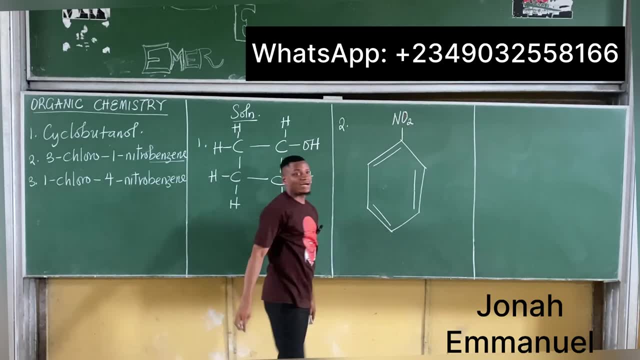 Your nitro is usually NO2.. I want to now say one nitro. It means that nitro comes here. I'm having this as NO2.. So I have one nitrobenzene. Finally, I also have over there three chloro. 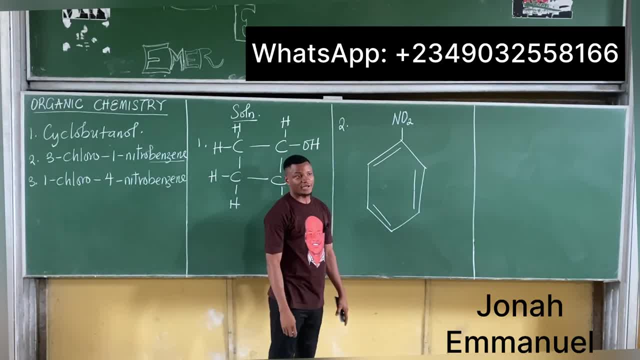 So it means: from here, count three and put chlorine. So it also depends on how you want to get your answer. You can choose to count from here- Here this has one, two, three and put chlorine. here It's correct. 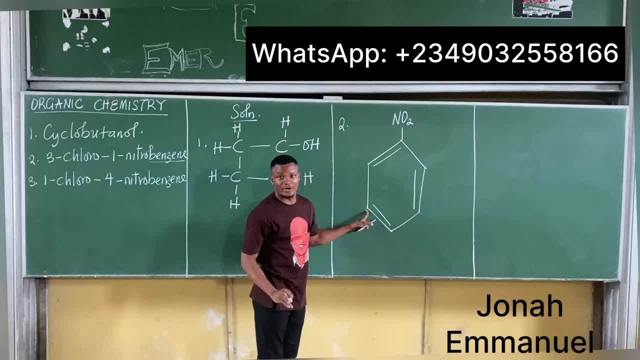 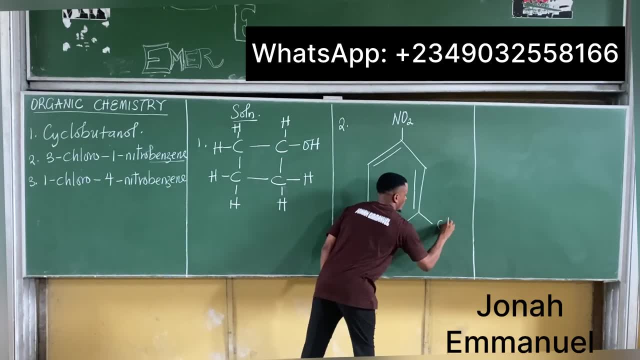 You can choose to do one, two, three and put chlorine here. You're correct. So whether you put the chlorine at this position or this position, it's correct, But I'm choosing mine here. So this now becomes position one, two, three. 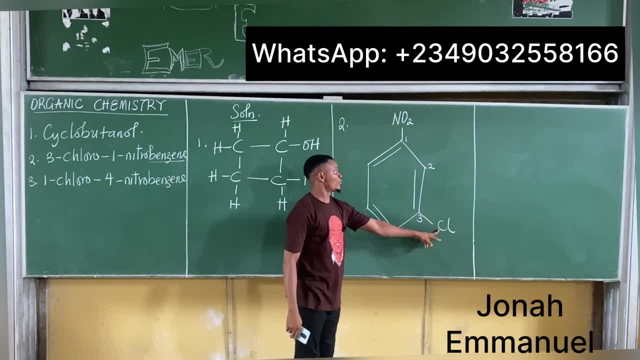 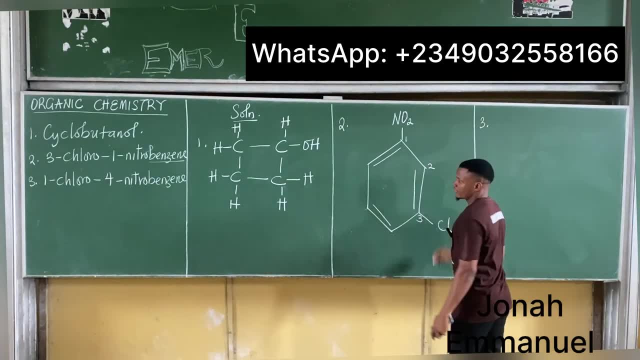 So it becomes three chloro, one nitrobenzene. That's all Number three. Number three is not really the regular. It's not really the regular, But let's see how it goes. So they said one chloro, four nitrobenzene. 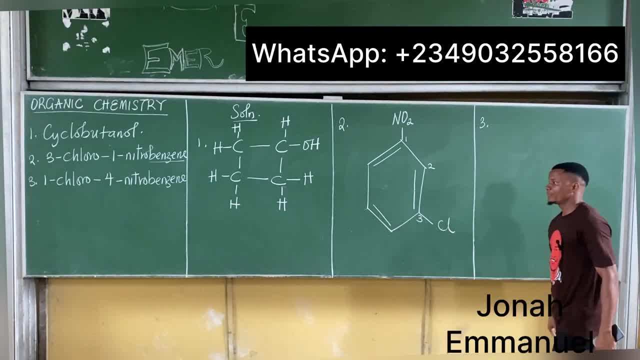 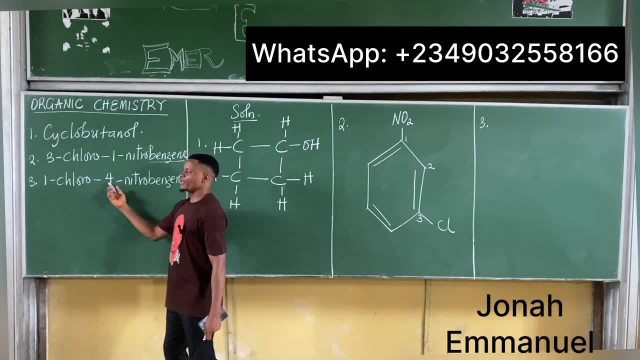 That's quite wet, But then, Okay, I think the name is actually wet, Right, I think this naming is wet. How can the four be the nitro? Right? But then, if I'm going to take this description, it means chlorine is at position one. 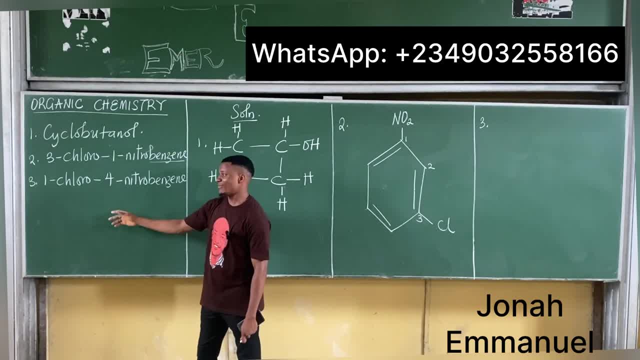 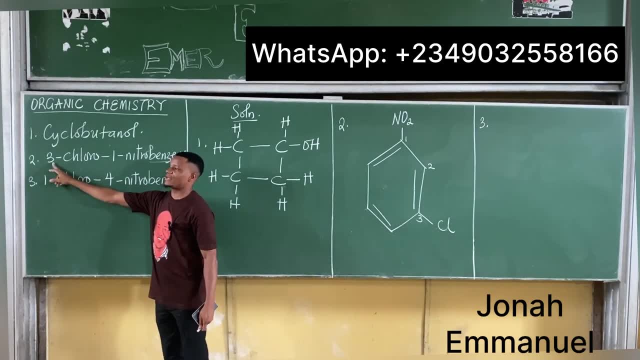 Nitrogen or NO2, is at what? there Four. But I still feel this is a weird name. A weird name. Usually the substituents should take the bigger number and this one should be closer. But fine, Let's use this. 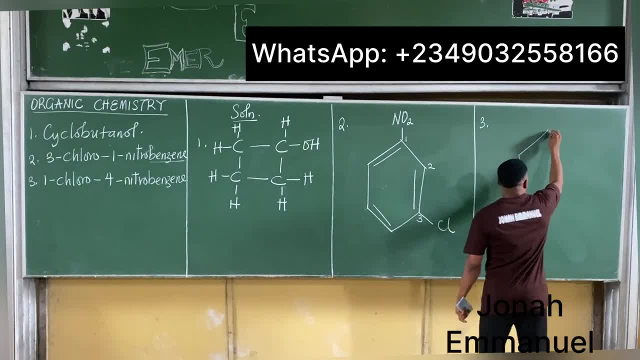 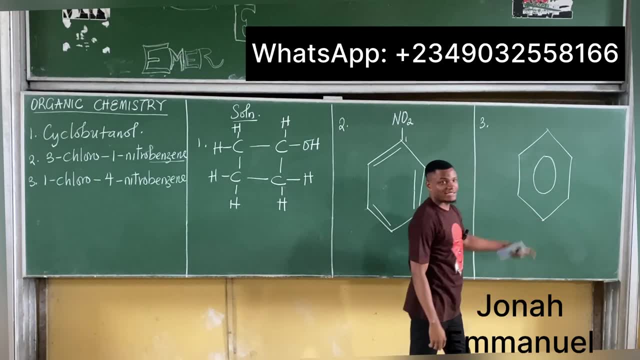 So I'm having my benzene ring again. I'm having my benzene ring again. It's still okay for you to do this. I've said it before, So I explained this in our last class: how to do benzene. This is still a benzene. 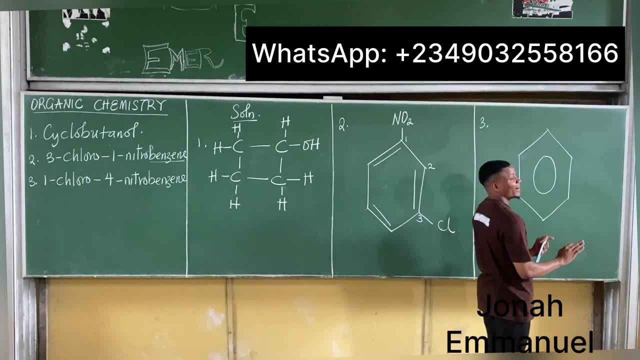 It's okay, You can use a circle desk- Okay, But then let's make it as formal as we can, And by that I mean put this as this, this and this. Alright, so I have this Next task. 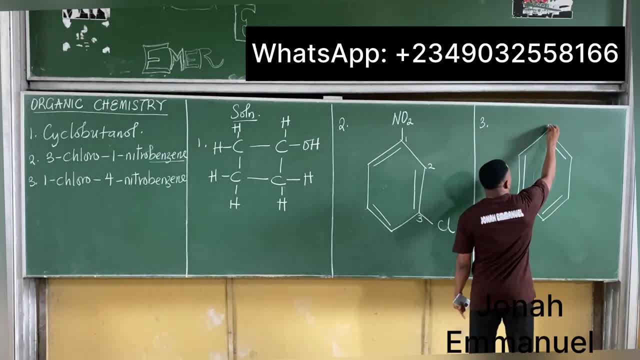 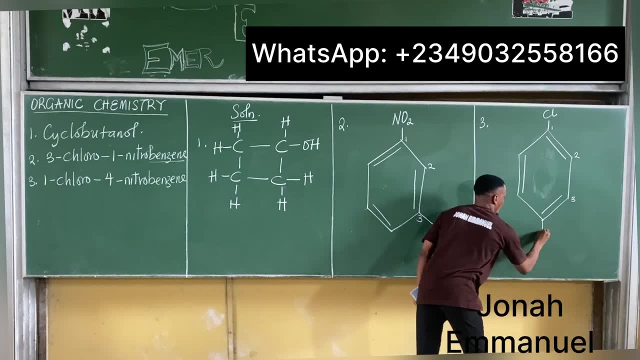 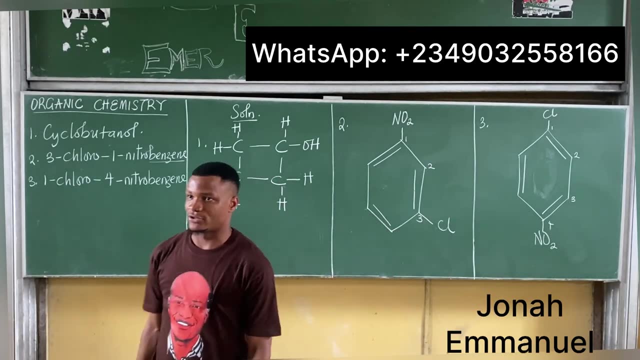 Let me get my one chloro. So if it's one chloro, that means chlorine should be at position one. So one, two, three, four NO2.. Here comes one chloro, four nitro benzene. So that's all. 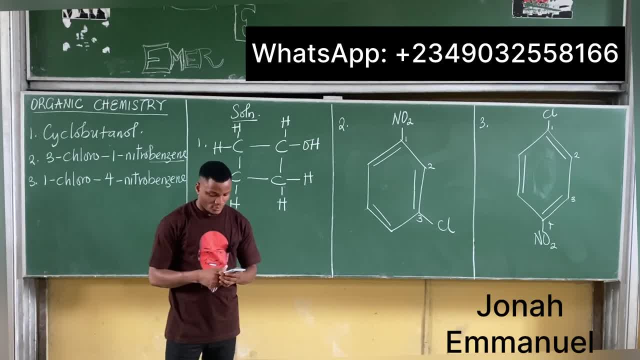 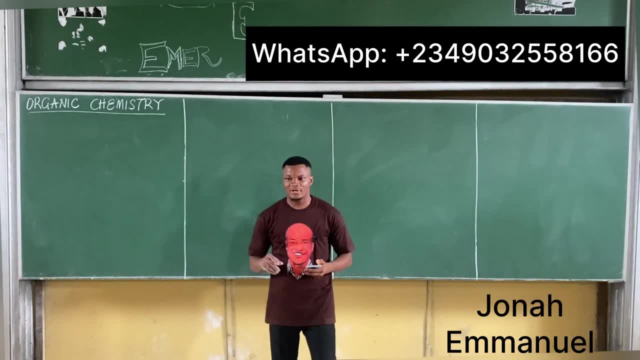 So this is how you draw these structures, please? Alright, Let's move on. Any questions, please? Alright, Next up, please. Let me highlight some few things to note about isomerism, or isomers, And let's proceed, please. 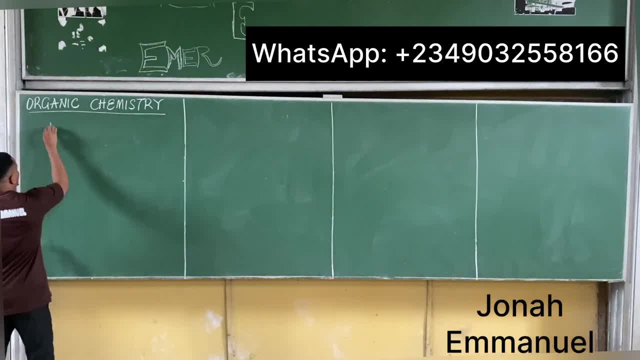 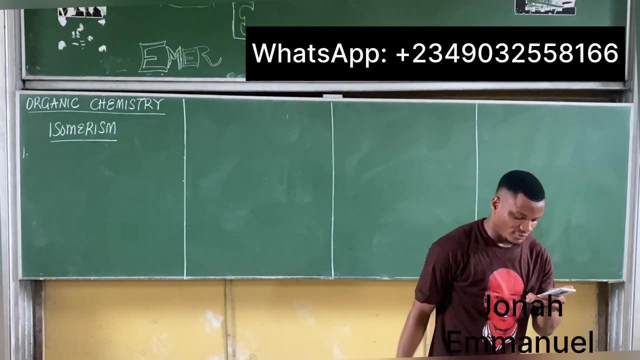 So let's look at, let's highlight isomerism a bit. Please note the following: please, Isomerism or isomers. Note the following, please: Number one, Number one, Alkenes, Number one, Alkenes. Alkenes are isomers of cycloalkanes. Please note this one first. That's the first thing to note. We've defined isomerism before now. We've talked about the types- Chain, functional, geometric- But leave that one now. 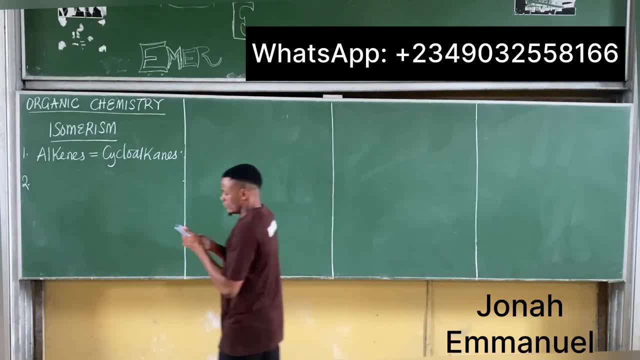 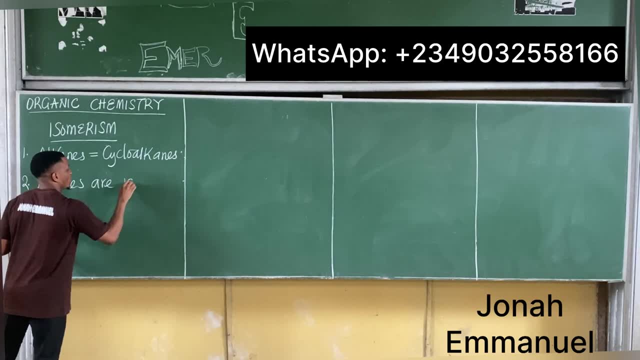 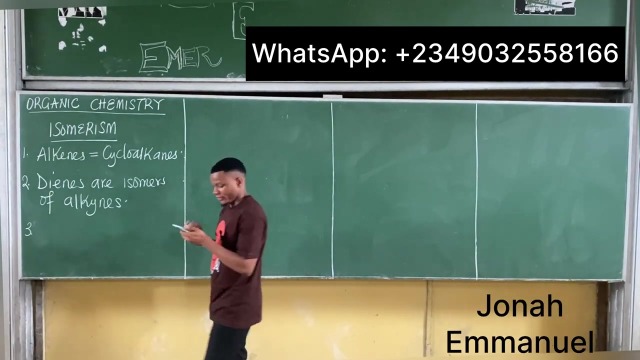 Let me just highlight some few points. Number two: Note that dienes. Note that dienes are isomers. Isomers are isomers of alkynes Are isomers of alkynes. That's number two. Number three: Note that alkanols. 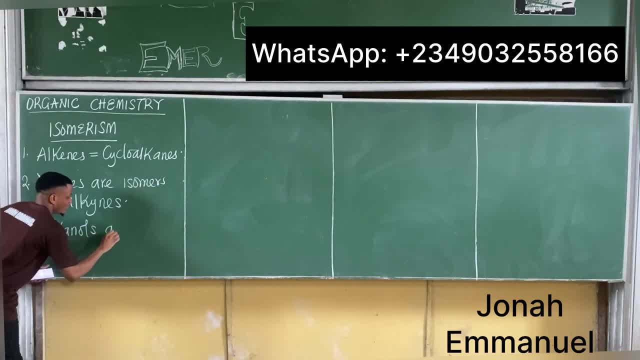 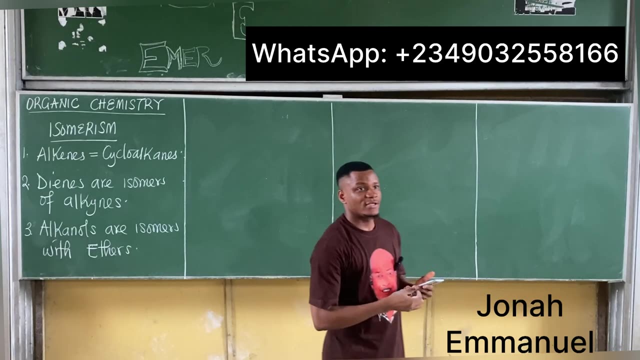 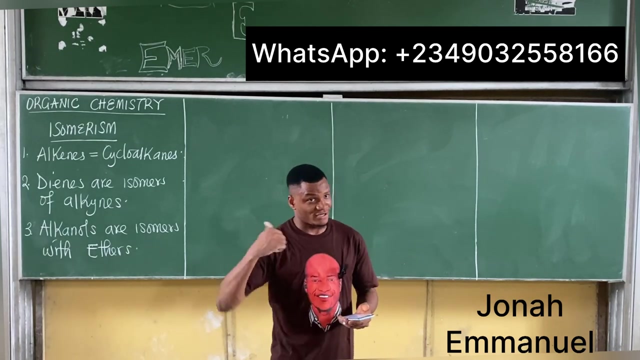 Note that alkanols are isomers: Does with ethers. So if you know the three things, there is nothing to give you an isomers. but you can know the three things. I didn't mention these three when we did isomerism in class. 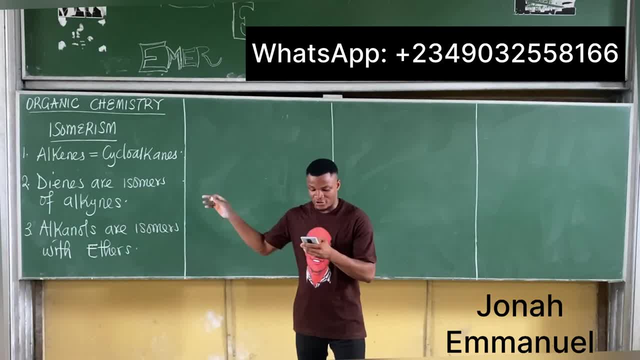 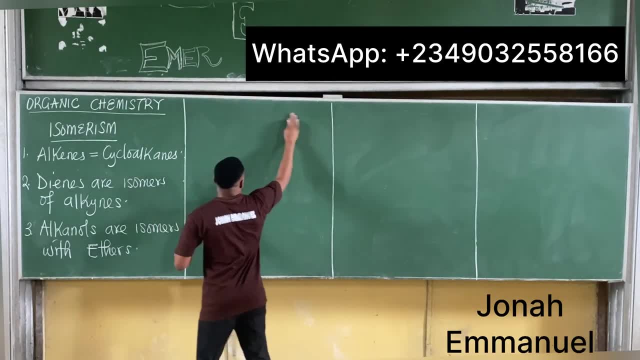 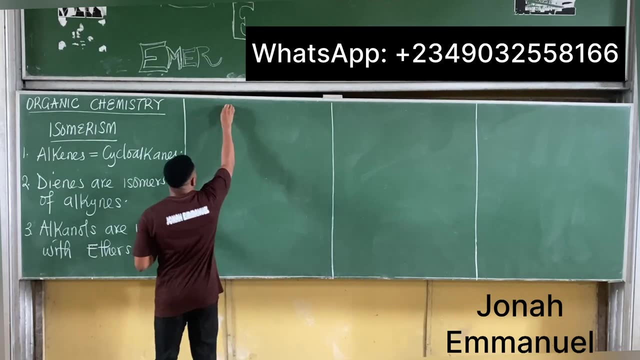 But now I'm giving you now Let's use this concept to answer a lot of past questions. Take that: please Give the names. Let's try this question. please Give the names and two structures for the following: Give the name and two structures for the following: 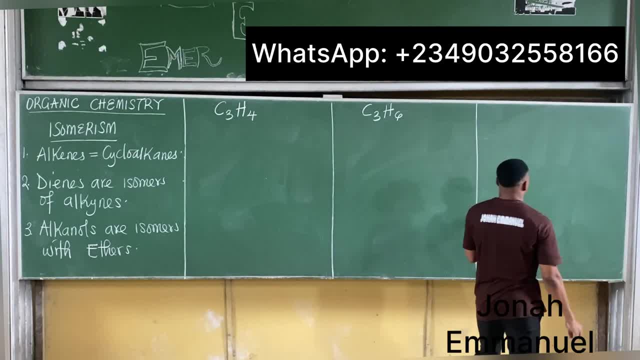 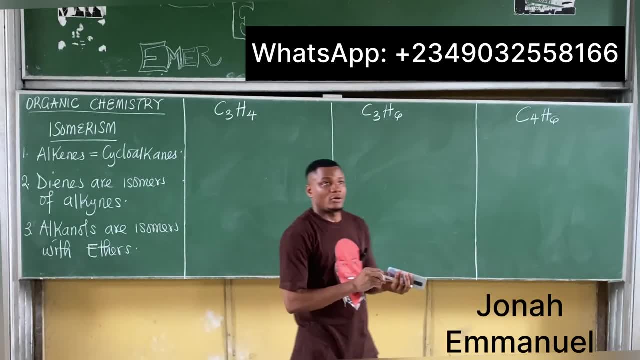 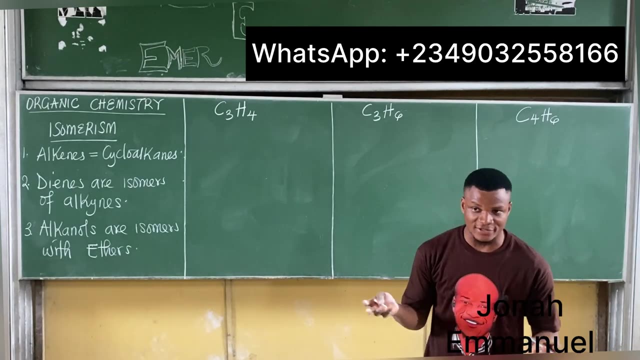 Give the name and two structures for the following For the following: All right, look up, please. So this question here is actually to test your idea about isomerism or isomers. First things first, I'm giving C3H4.. 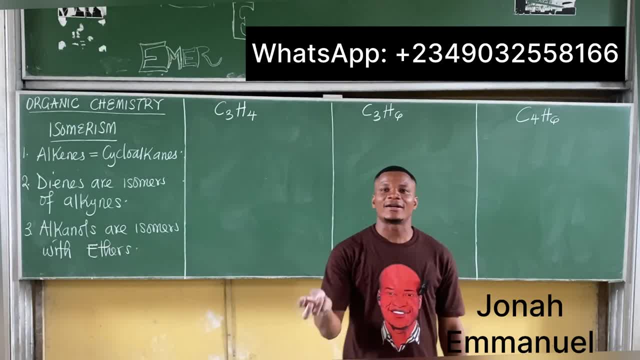 My first task would be C3H4,. is it an alkyne, alkyne, alkyne, alkyne, or which of them? Ah, I'm having alkyne, I'm having alkyne. 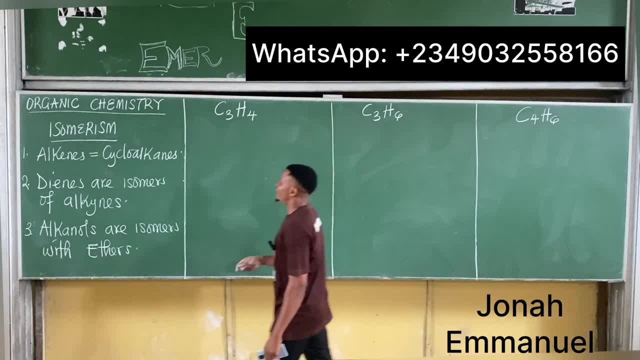 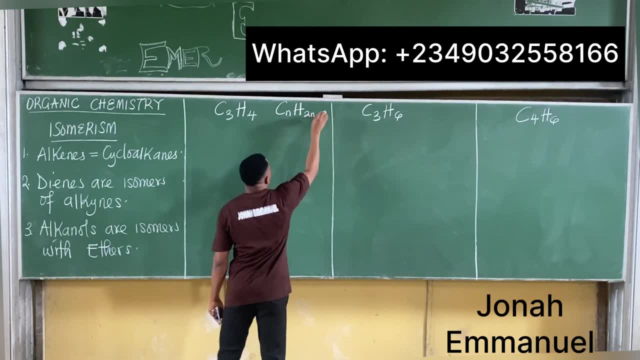 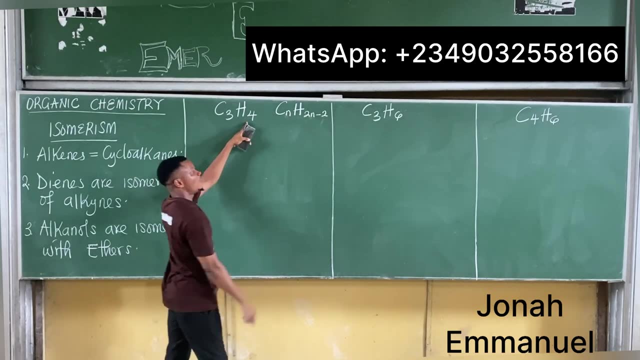 Is it an alkyne or an alkyne? Of course, check the formula For alkyne. I have CnH2n-2.. So when it's 3 here it becomes C3 into H2 times 3, 6, minus 2, 4.. 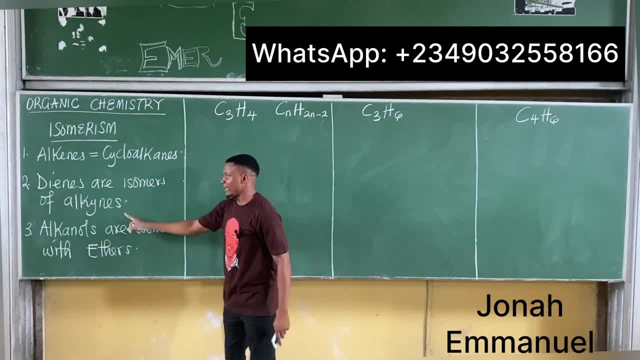 So it's an alkyne. If you say, give 2 isomers, just simply what's there, come here, that's it. That means I'll create an alkyne and what's it in there? A diene. that's simple. 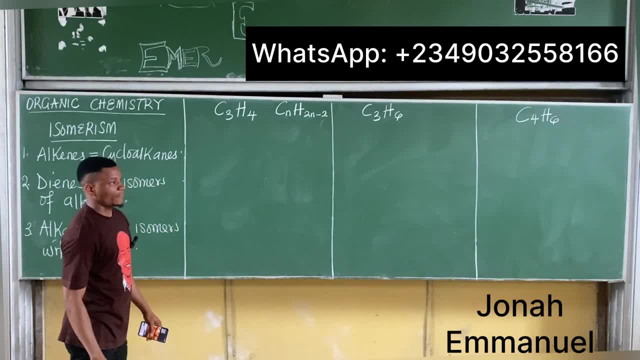 So first things first my alkyne. All right, so I'm creating an alkyne with C3H4.. First things first my C3 carbon. there, 1,, 2, 3, that's C3. 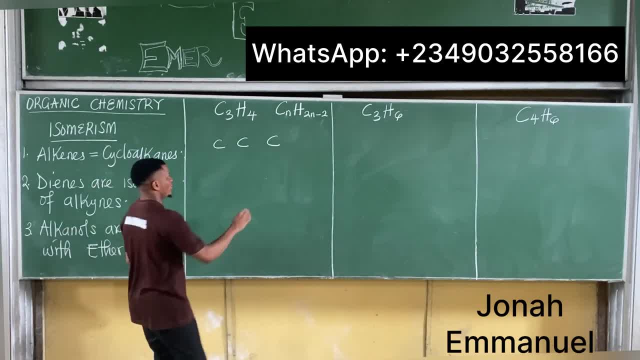 So maybe it's an alkyne. it means I have to put what there? A triple bond, So it becomes 1, 2, 3. Automatically, this is now an alkyne, Of course. balance this up. 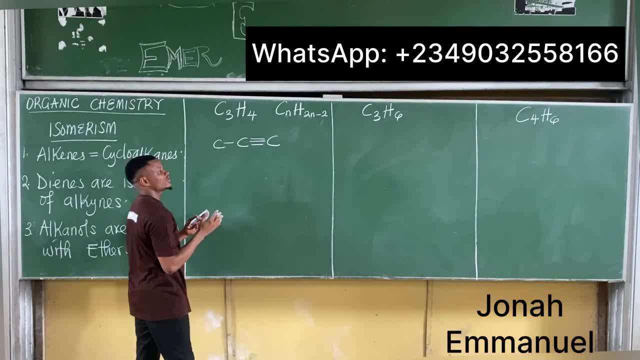 How do you balance it? 1 here We said, for this stuff to be balanced there, each of them must have 4 bonds. This one has 1,, 2, 3.. This makes it 4.. This has 1,, 2, 3.. 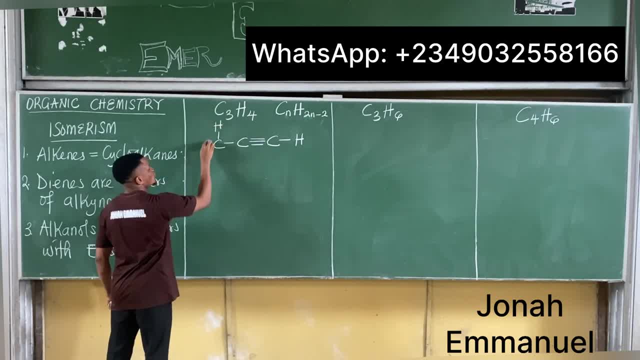 This makes it 4, balance. This one has 1,, so 2, 3, and 4.. So check this out. I'm having 1, 2, 3, C3,, 1, 2, 3, 4, H4.. 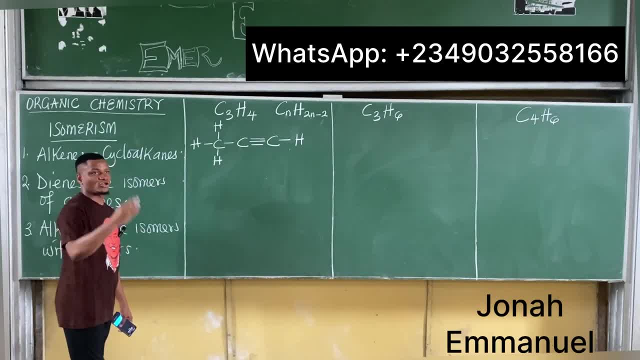 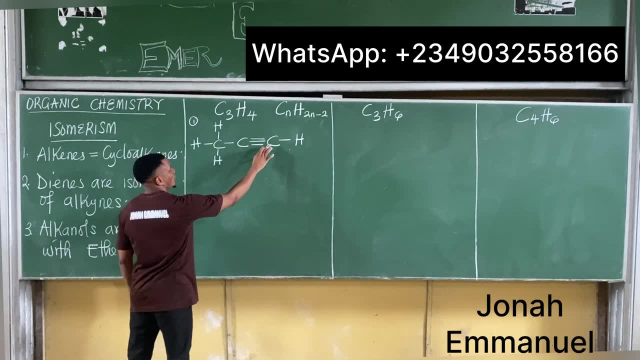 Balanced. I've got my first structure. They said: provide the name and the structure. I've got my first structure. That's 1 there. Let's get the name. What's the name of this compound there? Huh, Propane. 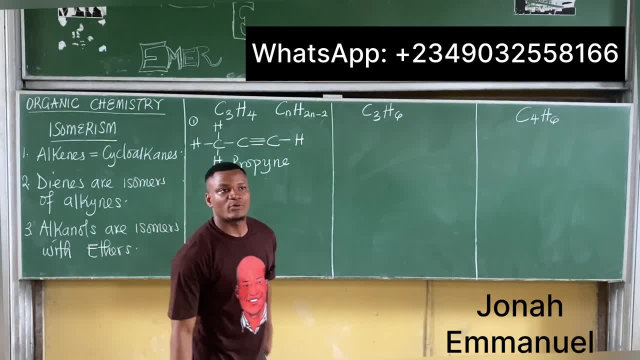 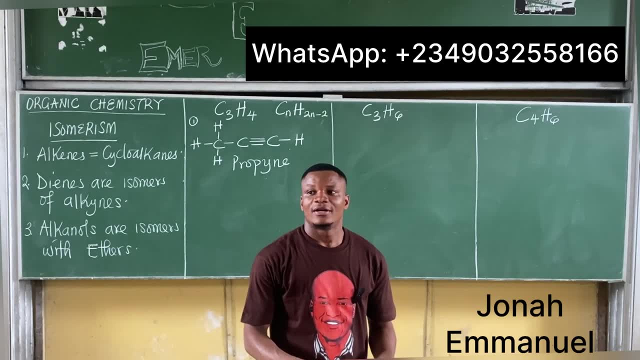 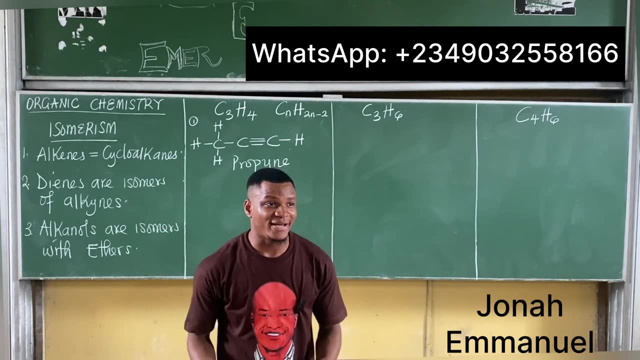 Propane, Please. is it propane or 1-propane, Propane or 1-propane, 1-propane, 1-propane- Where is it now? If you are here now. like I said, propane and 1-propane are the same thing. 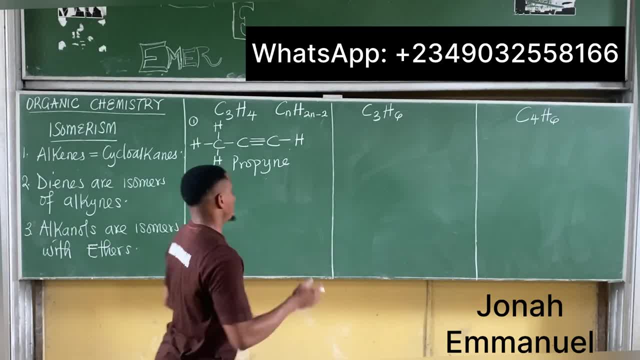 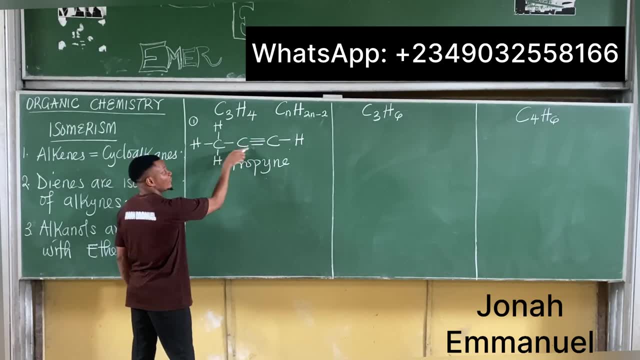 Why? Because there can be no 2-propane. If this man is here, I'm counting 1 before the source is 1-propane. If I choose to move the triple bond here, I'll still have to count from here. 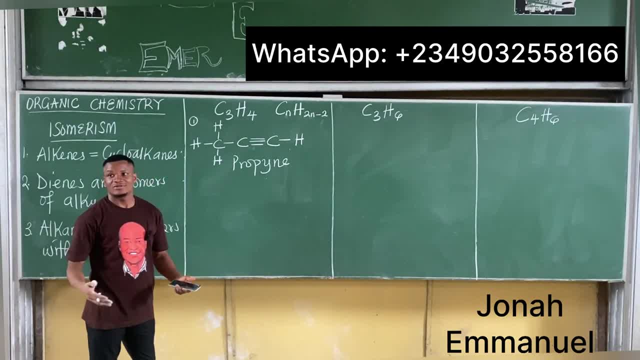 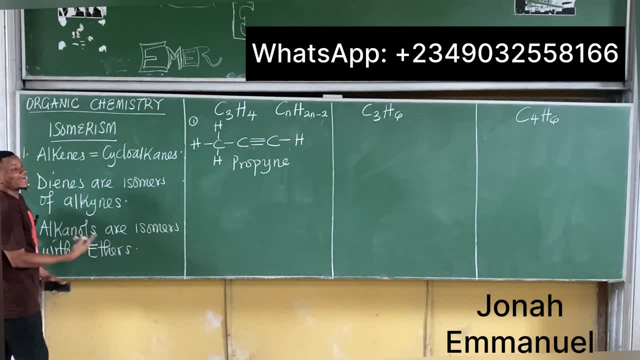 So, whether here or here, it's 1-propane, So it becomes 1-propane. I've got my propane, my alkyne. My next step would be to form a diene, So the second one. 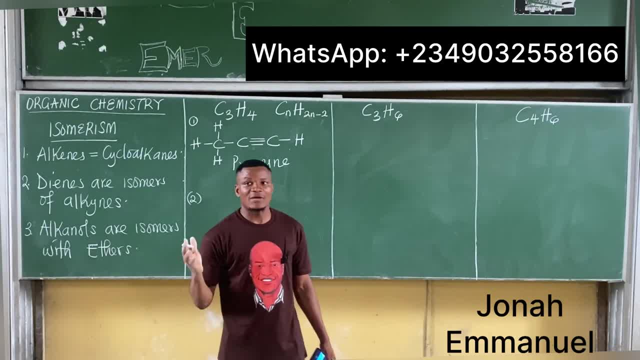 I want to form a diene. What's a diene Here? When it's called a diene we said dienes are simply compounds that have over there 2 double bonds. It's telling you a di and an in. 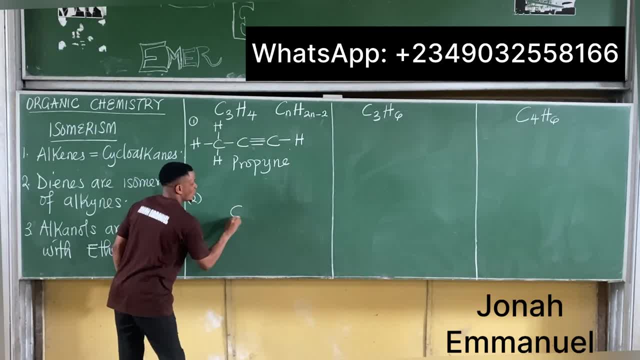 So 2 double bonds. So it means create the same 3 carbon compounds: 1,, 2, 3.. Make this a diene. How Put 2 double bonds Between these 2,? I'll put my first double bond. 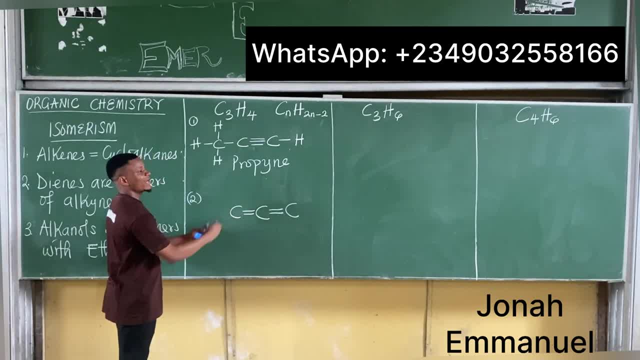 Between these 2, I'll put my second double bond. Balance of the structure. This one is now 1, 2, 3, 4. Balance: This one here is 1, 2.. 3 and 4.. 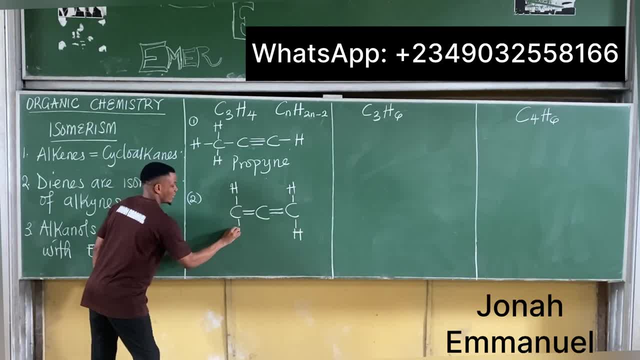 Balance. This one here is 1, 2,, 3 and 4. Balance. If I count, I have 1, 2,, 3. C3, 1, 2,, 3,, 4. H4.. 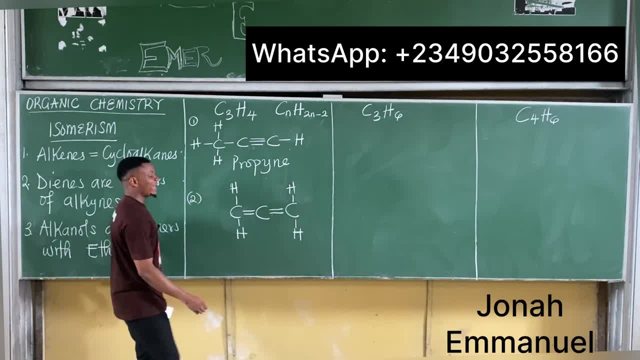 That's correct. So name this compound. Of course, what I choose to number, from right to left or left to right, the same thing. So let's number it. I'm having 1,, 2,, 3.. So how do we name the dienes? 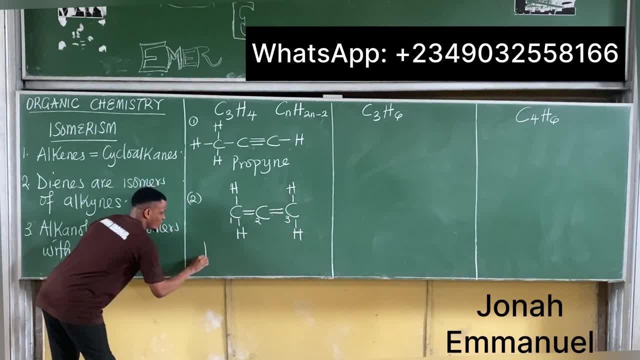 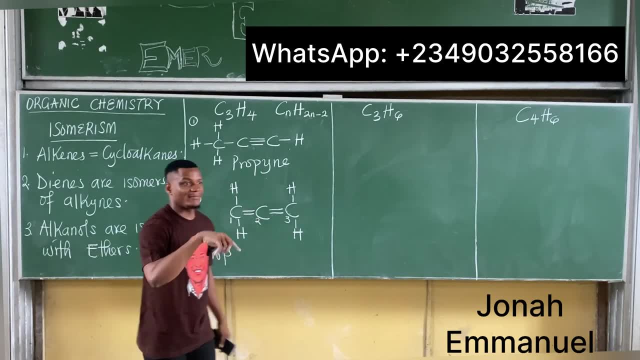 For this one. here I'm having 1,, 2, 3.. 3 carbons is a. what there Probe? But we said for dienes it's an A, are we You can remember? So this is not just probe. 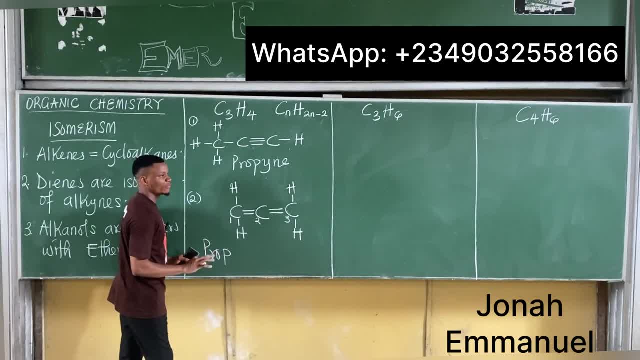 Okay, hold on, This is not just probe. If I want to get the position of the double bond, my first double bond, from my numbering, my first double bond, if I'm counting like this, so I'll count carbon 1 before my first double bond. 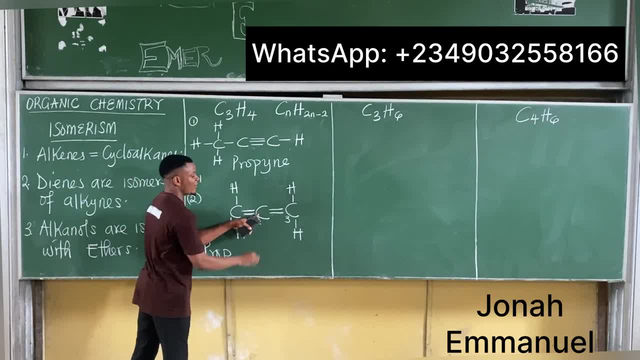 so it becomes 1.. Moving on, if I go this way, I'll count carbon 2 before the double bond. So I'm having 1,, 2.. Now note for dienes. you don't say probe 1,, 2, diene. 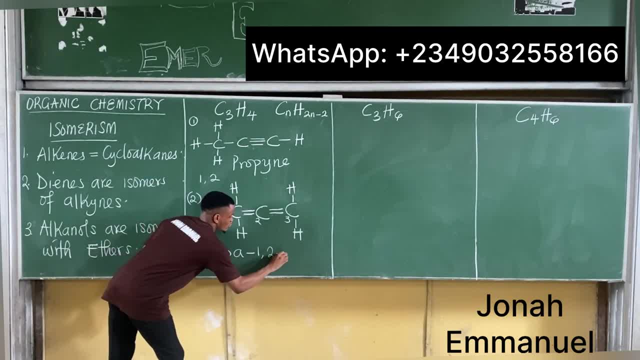 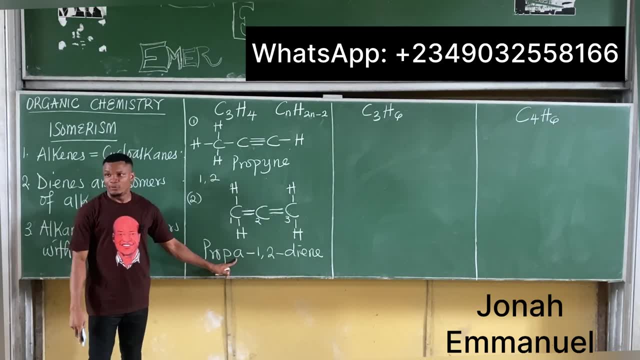 What do you say there? Probe 1, 2, diene. Please go check your notes. So for the dienes, there's always an A there. If it's boot, it's not boot 1, 2, no. 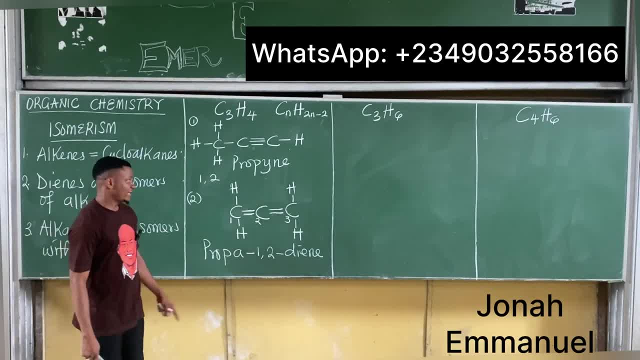 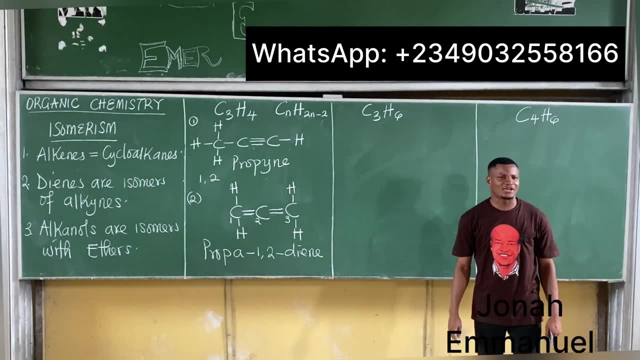 It's boot 1, 2, diene. That's the idea. Alright, I'm done with the first one. Let's come to this one here, C3H6.. C3H is what there? An alkene right. 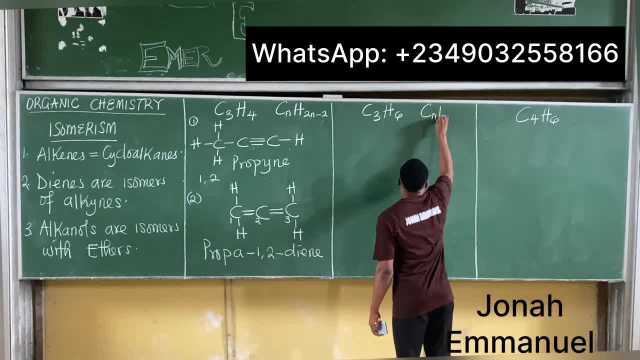 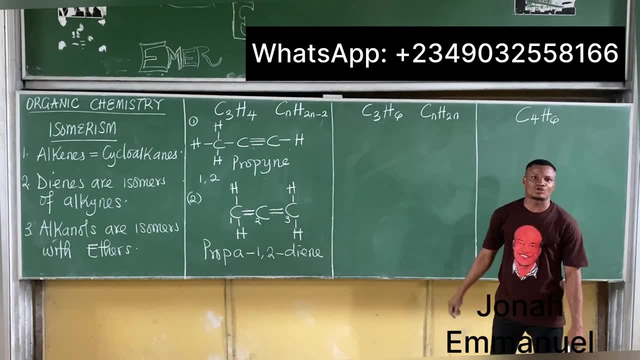 Yeah, alkene. Alkene General molecular formula is CNH2N, So 1 is 3.. It becomes 2 times 3, 6.. My tax number, they said, create two structures for my alkene. 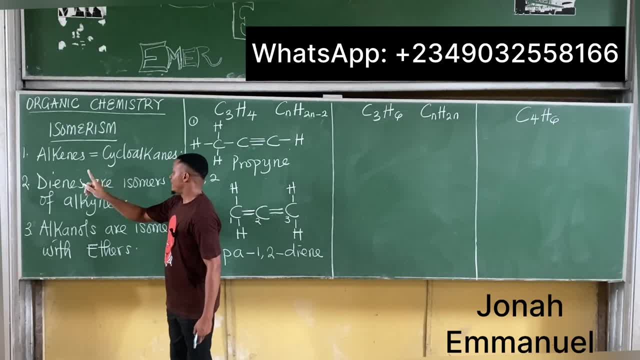 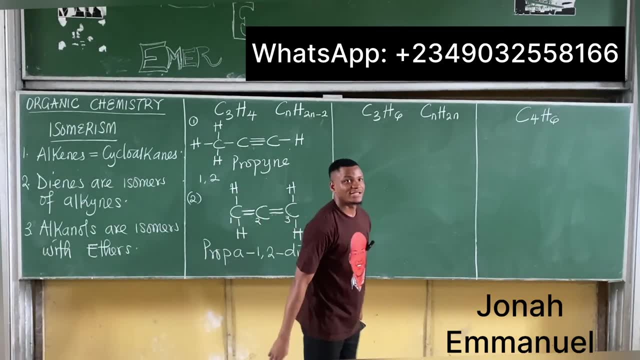 Look at it here. So I'm saying that alkenes are what there, Isomers are what there, Cycloalkene. So the first in there form an alkene. Secondly, form what there, The cycloalkene. 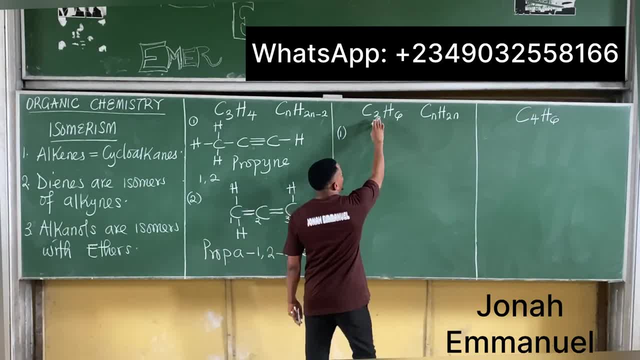 So first is first number 1.. Let me form an alkene For this one C3,. I'm having 1,, 2, so make this an alkene. Put what there, Double bond. So I'm having 1, 2.. 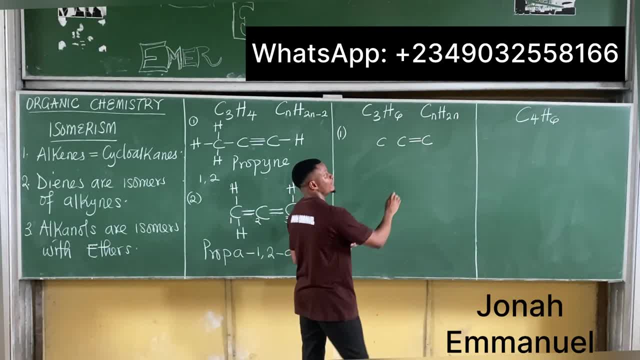 This qualifies this as an alkene Balance of the structure. I'll put 1 here, So this one is now 1,, 2,, 3, and 4.. 1,, 2, 3. This makes it 4.. 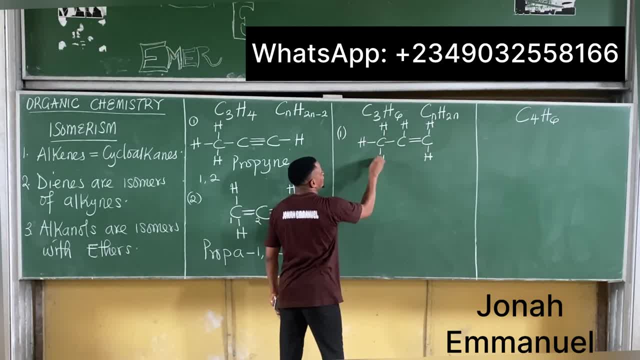 1,, 2,, 3, and 4.. 1,, 2, 3,, C3.. 1,, 2,, 3,, 4,, 5,, 6,, 8,, 6.. That's correct. 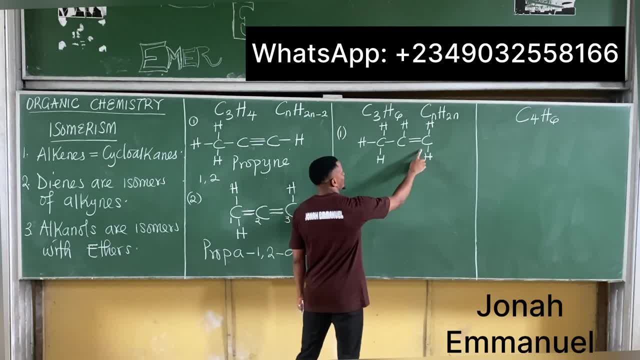 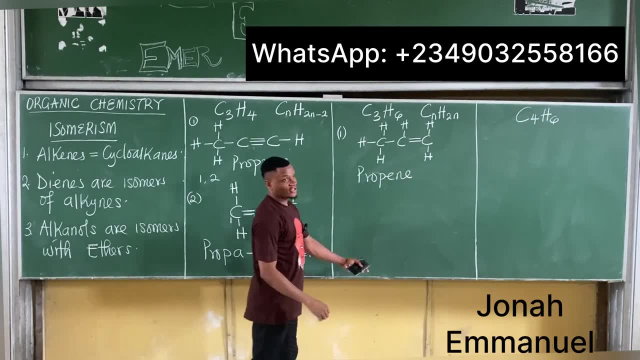 So name this compound. How do you name this? Which compound is this? Propene? If you say prop-1-ene, note that there's one there. no prop-2-ene If you want to say 1-propene. 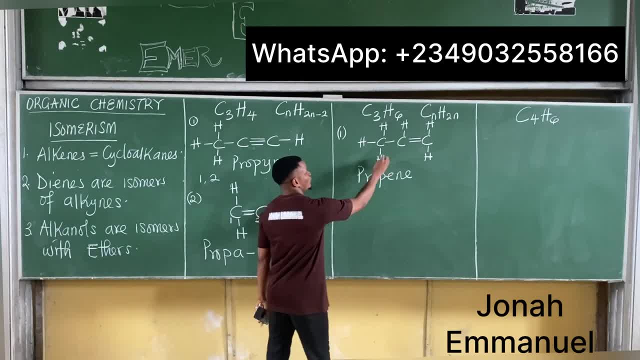 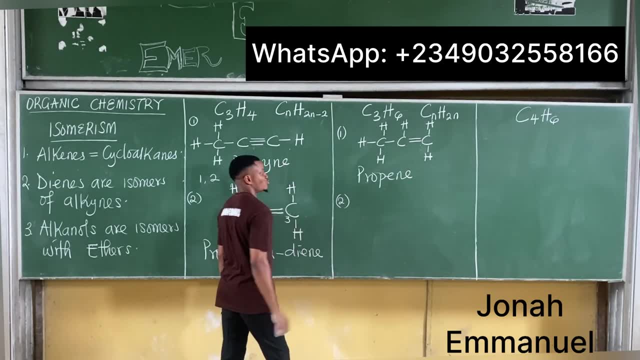 or prop-1-ene, no problem. Or you can say propene, Because prop-1,, 2,, 3,, 3-carbon prop and then double bond alkene, My second structure. we said propene and cycloalkene. 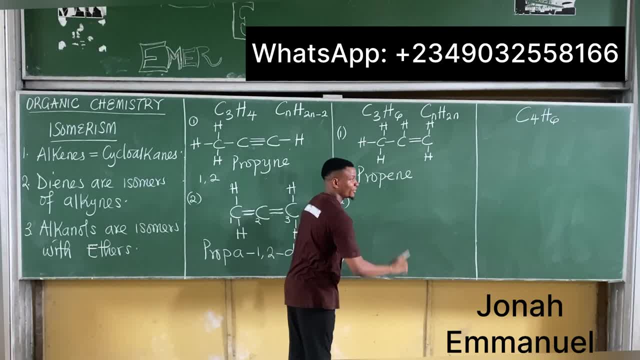 So it's as easy as use 3 to form a cycloalkene. For the fact that it's a cyclo, it means to be what there? A ring structure. So I'll now arrange 3-carbon to give me ring structure. 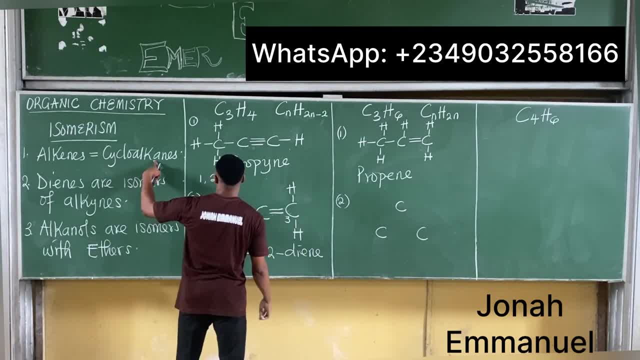 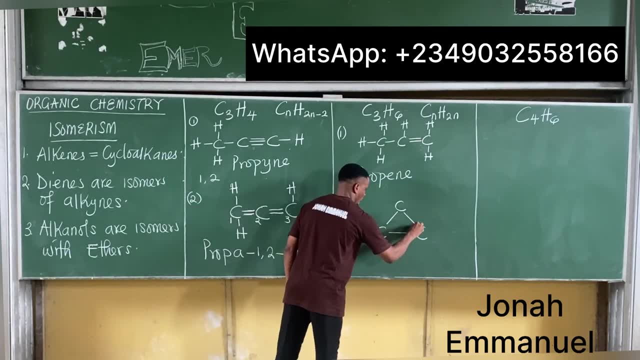 like this. Of course, it's a cycloalkene For an alkene, I expect a single bond to become single bonded, single bonded, single bonded. So I have this Alright. so here's now a cycloalkene. 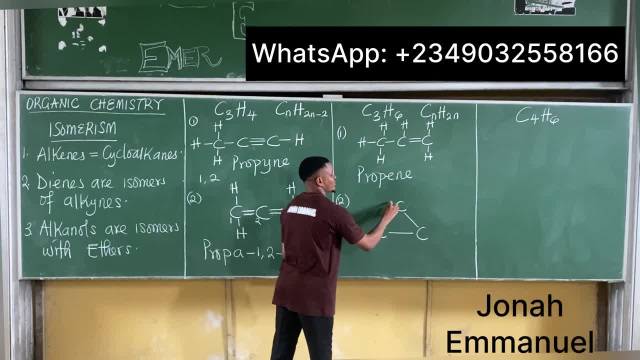 Balance this out. I'm having 1,, 2.. You can just put your R there or say H2.. It's correct. So 1,, 2,, 3, 4.. 1,, 2, H2.. 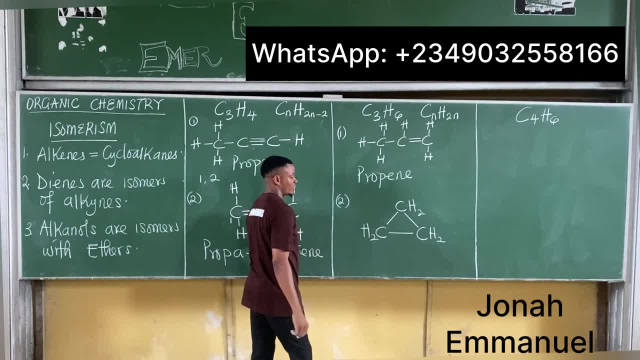 3, 4.. 1, 2, H2.. 3, 4.. So it becomes 1, 2, 3. C3,, 2, 4, 6. H6. This compound becomes: 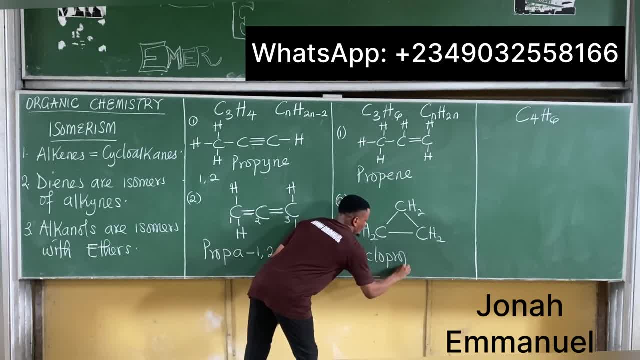 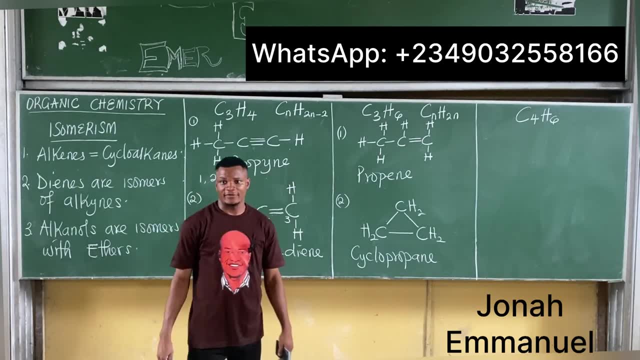 cyclo-protein. Please, get this man done on your own, please, Very fast. Get this man done on your own, please, Very fast. Get the third one. Cut it down. Get the third one done on your own, please. 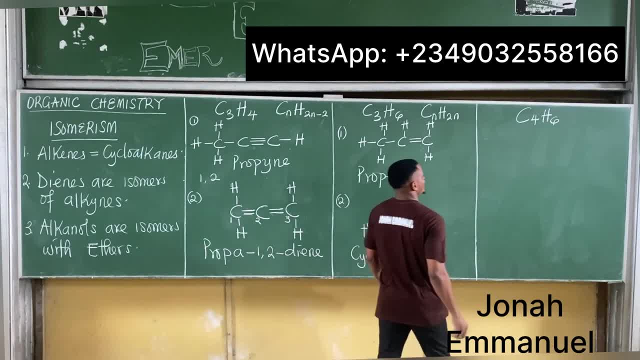 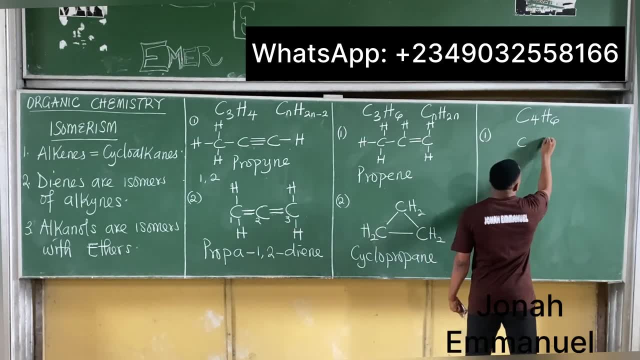 Very fast, Very fast, By the way. let's get this done, please. So here's an alkyne. Here's an alkyne. First things first: 4-carbon: 1,, 2,, 3,, 4.. 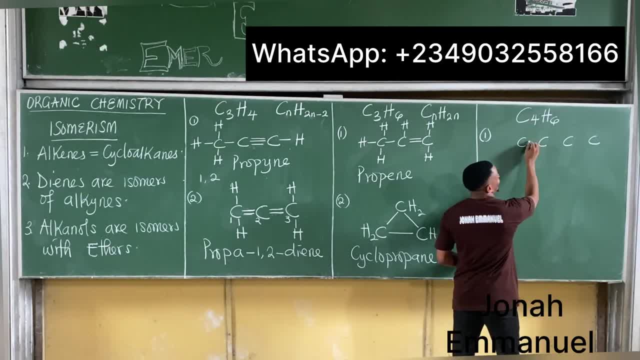 Make this an alkyne, Please. you can choose to put your triple bond here or here. For this case, let me use here. I'm having this and this and this, So this one becomes 1,, 2,, 3,, 4.. 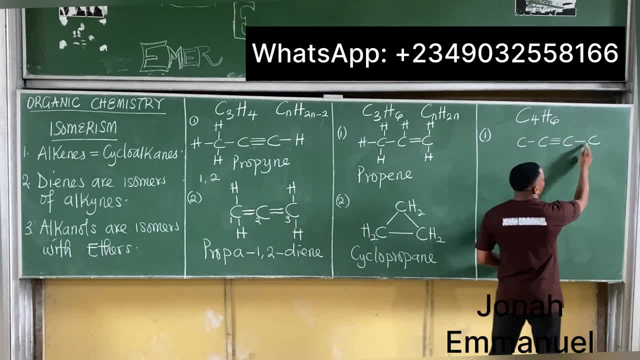 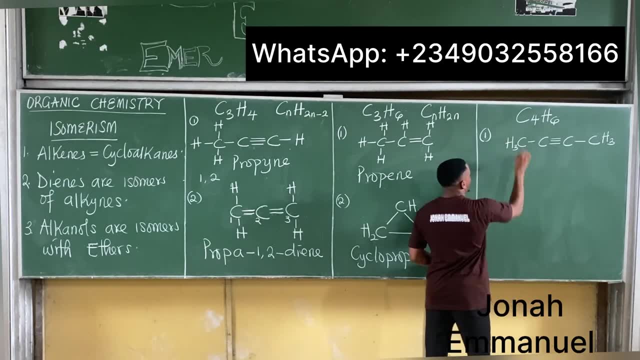 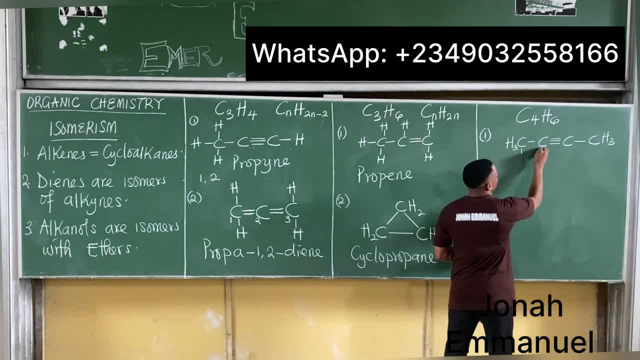 I'm still correct. How do I name this? This is 1,, 2,, 3,, 4.. 4 is boot, So it becomes boot. The triple bond is attached to carbon 2.. So boot 2, iron. 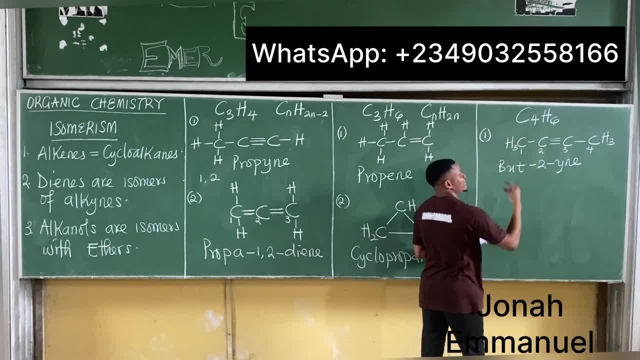 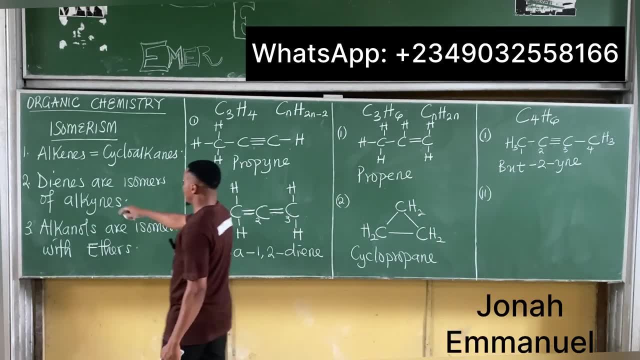 If you want 2, you can bring this one here So that it becomes boot 1, iron, They are both correct, all right. number two: we said our kinds are isomers of what they're, dienes. all right, so let's get a. 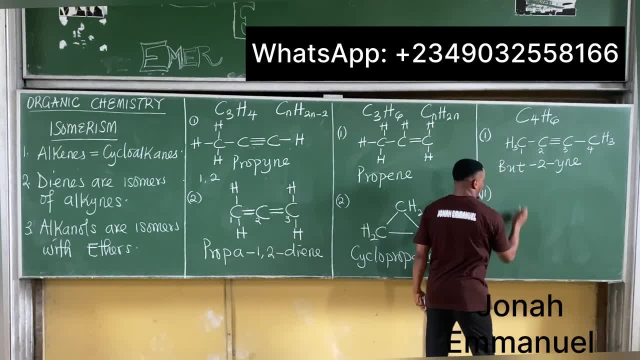 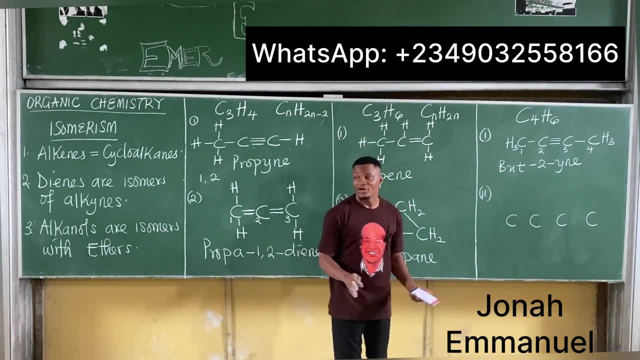 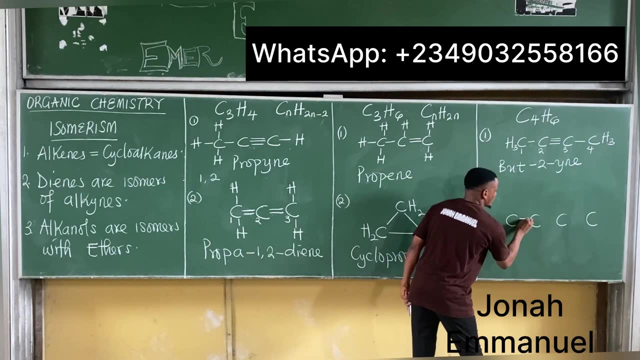 diene equivalent. so first is 4 carbon 1, 2, 3, 4. it's now at your own discretion to put your double bond for a diene. it means i'm having two double bonds. put your two double bonds anywhere. you can come here and choose one two as the first one also here. one two and second one is correct, you can. 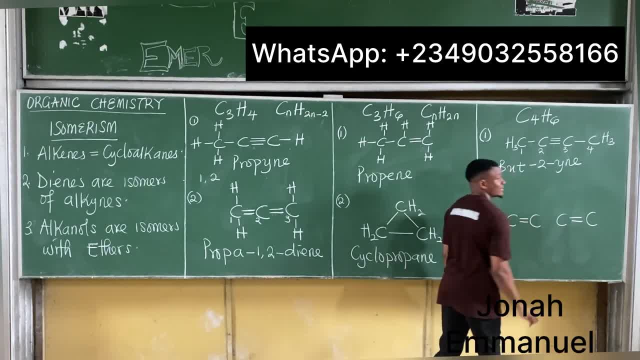 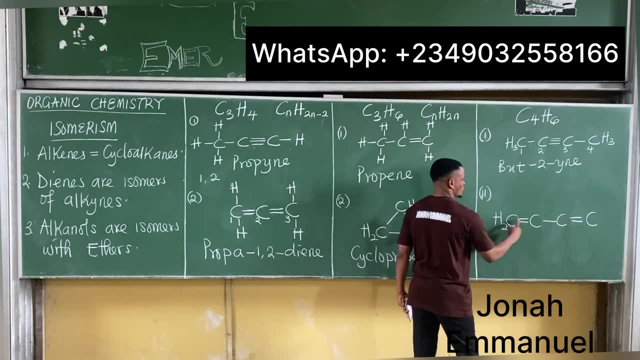 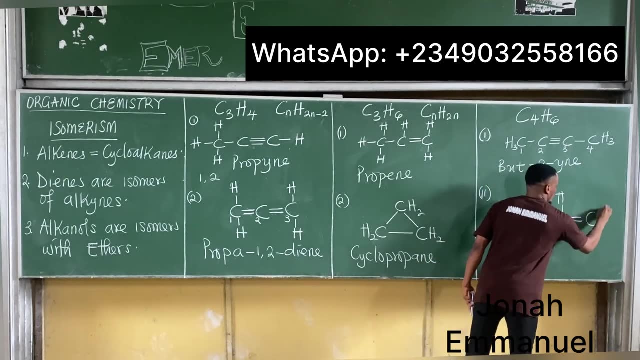 choose one, two here and one, two here is still correct. any one complete this single bond here. so this is one, two h two. one, two, three, four. one, two, three h. one, two, three h. one, two h two. so one, two, three, four, c four, two, three, four, five, six, eight, six name this compound one, two, three, four, four is good. 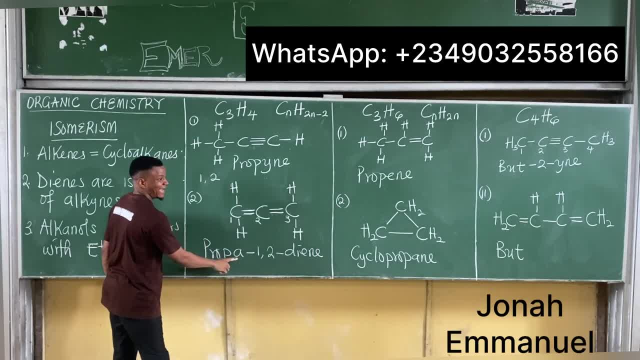 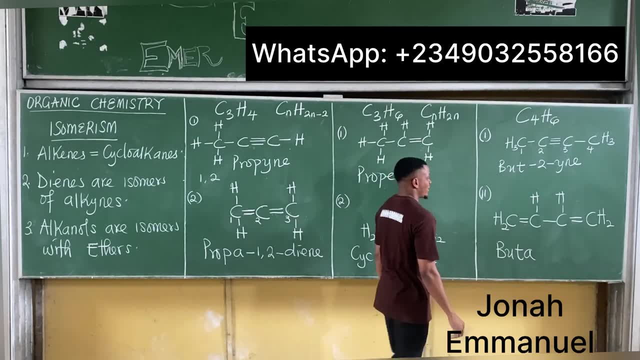 and i said: for your double bond, what is it now? buta and an? a. so instead of proper, instead of boot, it becomes what there? buta. all right, buta. do your numbering one, two, three, four. the double bond is at carbon one here and then carbon three here, so becomes one, three. 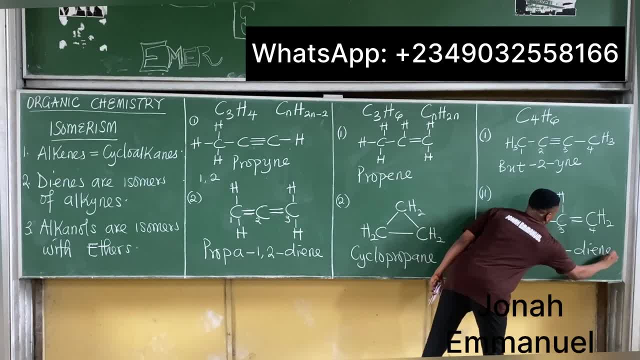 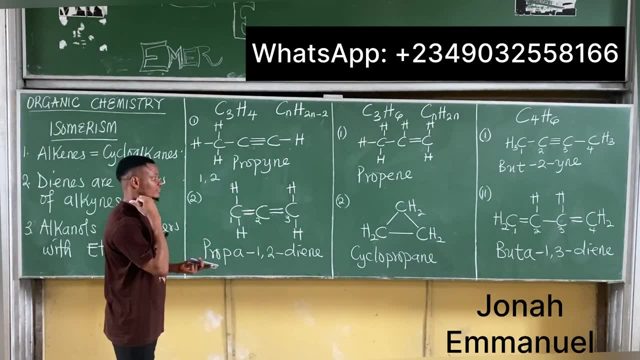 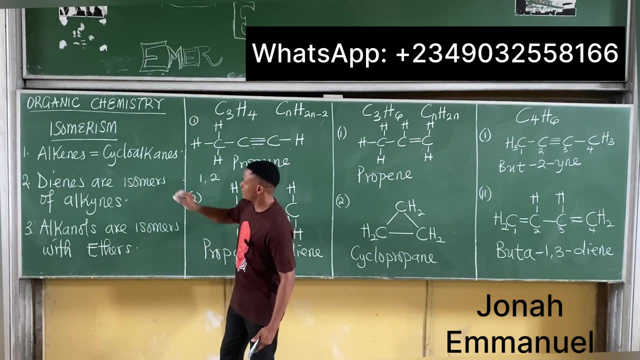 buta one three da in. so i have this. so that's how you get this stuff here. buta one three da in, uh, before we move on, please. before we move on, i have tested these two. uh. let's see if you can test one with this. let me give you one with this. let's see if you can test one with this, please. 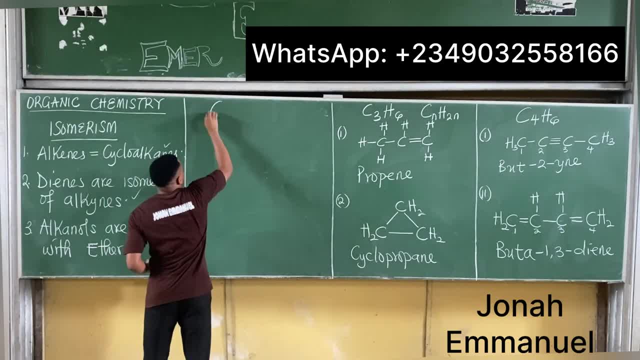 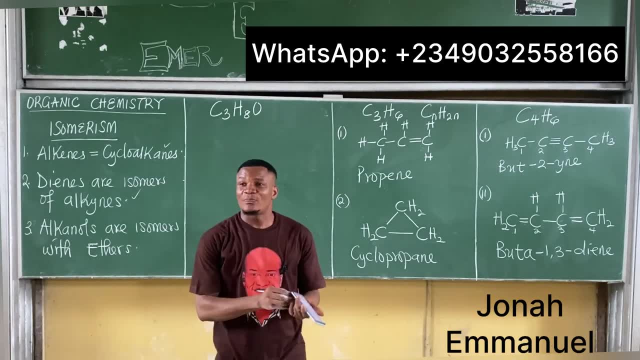 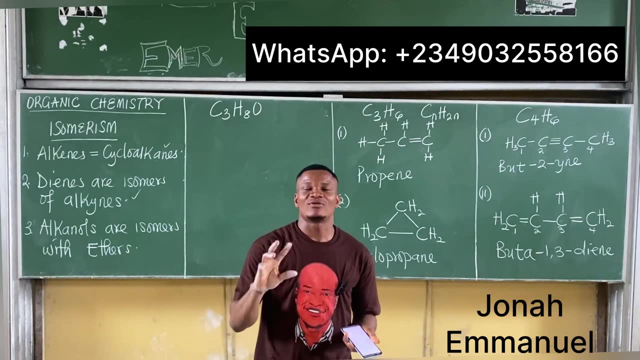 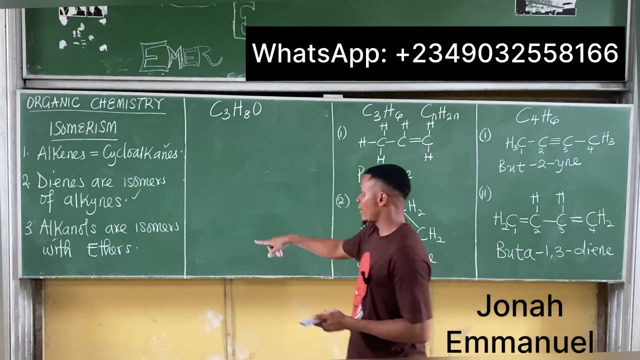 um, c3, h8, o, yep, so use this to name. so please see the different one. i now use c, h7 and 8, for 7 is most likely what you have most likely will be your um, R canal and R canal or your aldehyde and ketone for alcohols or R canals. you have this, so please see if you can. 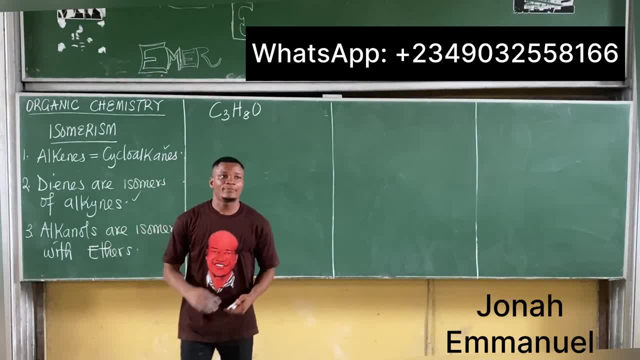 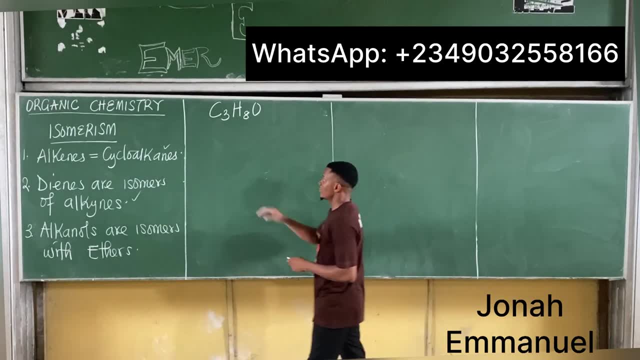 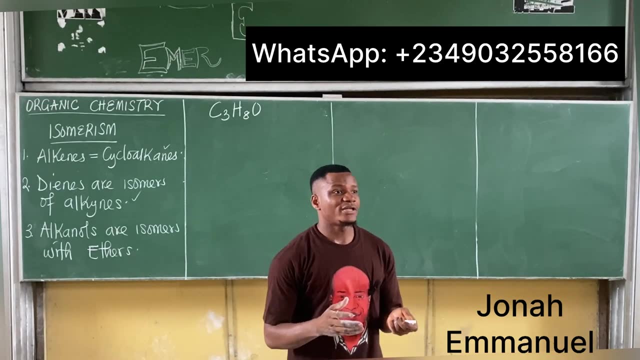 get two structures of this. let's move on here. so look up, look up, let me answer this and let's proceed. let me answer this, let's proceed, please. um, first things first for this one here. they won't tell you it's an arcanum. you have to be able to identify it and that's why the general molecular formula idea is important. 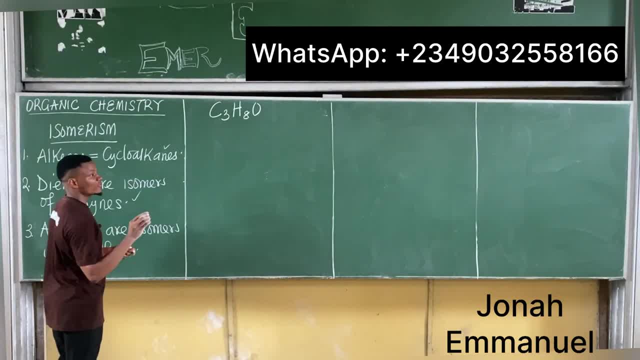 if i know my general molecular formula, i know that for the arcanum what i have is cn, h2n plus one. what again there? oh h. if i look at this, becomes c3 h into two times three, six plus one, seven plus this one here, eight, and then, oh, that's right there. so this is an arcanum. i can get an. 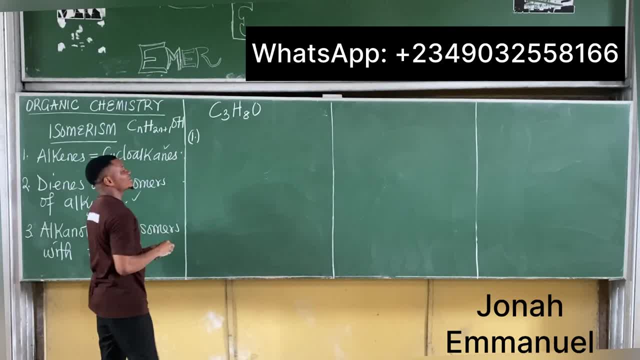 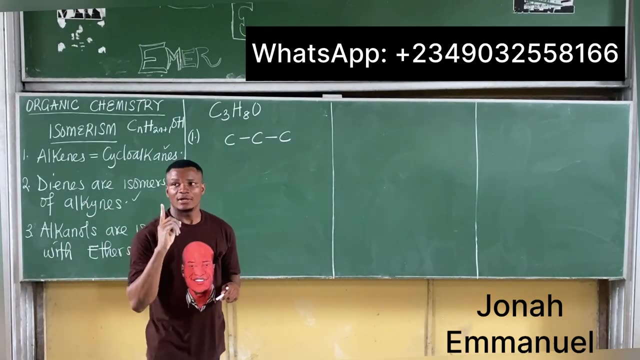 arcanum from this. so if that's true, that means let me get a three carbon arcanum, so it becomes one, two, three for an arcanum. we say: put what there. oh h, now, now, listen carefully, listen carefully. i said what we did after this example. i said: there's nothing. 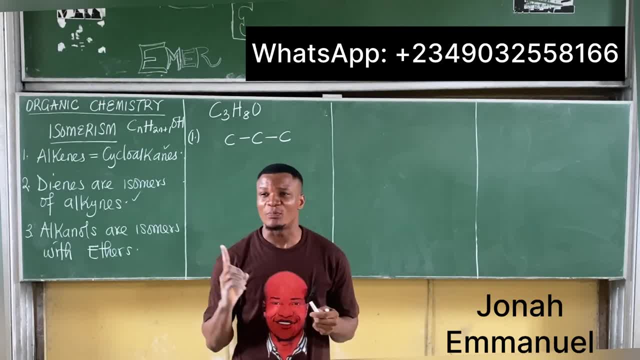 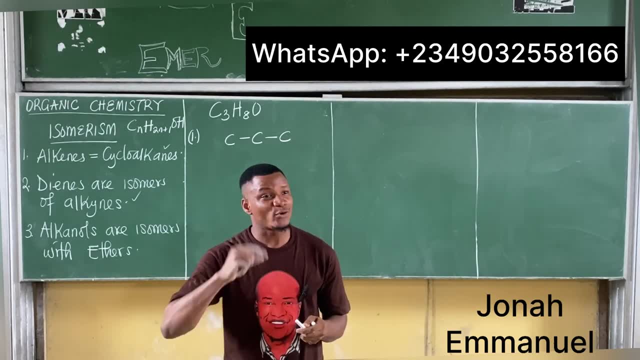 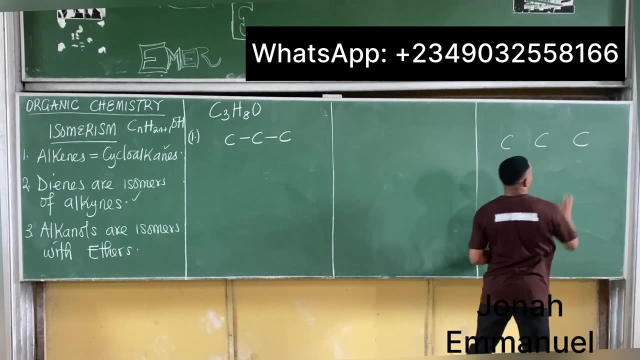 like what there like um, one propane and one propene for the arcanum. there is something like one propanol. please get a difference. look at this very well. i'm having three carbon here. let me explain something. i'm having three carbon here. let's say i want to use double bond. if i put double 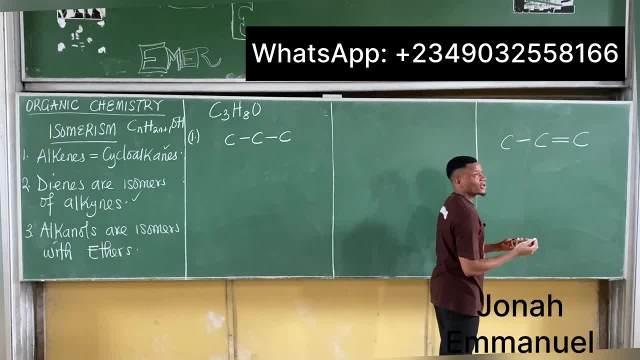 bond here and this for my numbering. we said number from this part, so i'll come to double bond first, so it becomes one, two, three, so it becomes propane in. let's reverse it. if i reverse it, bring these two here. it becomes this way. and then this from my proper numbering: i'll have to number one, two, three. 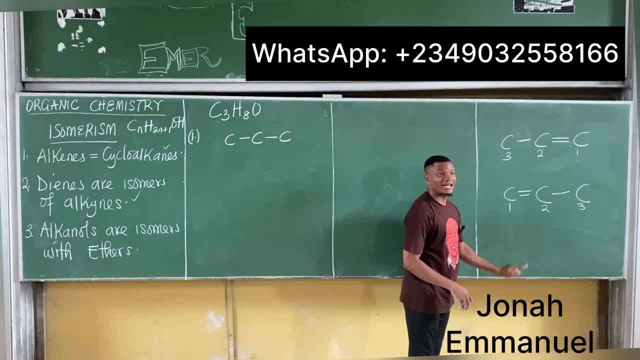 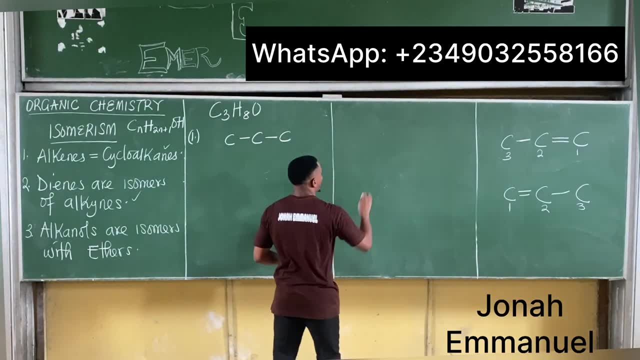 so it still becomes one, whichever way you number it. now, this is for an alkene and alkyne, so i'm gonna for an arcanor, it's not. so what do i mean for an arcanor like this one here? if i now choose to put the oh, 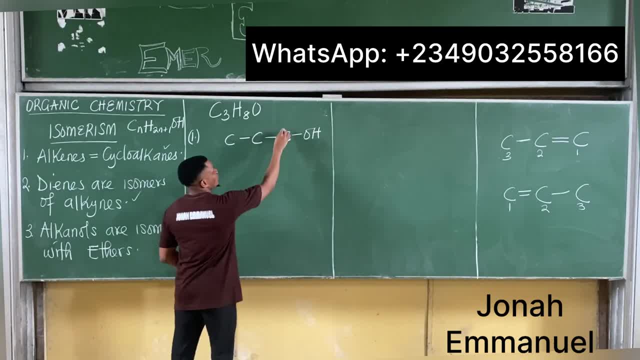 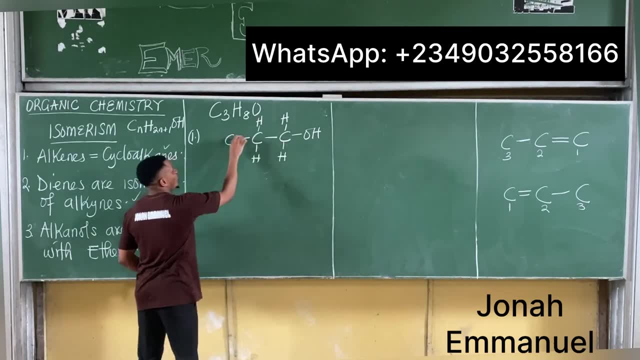 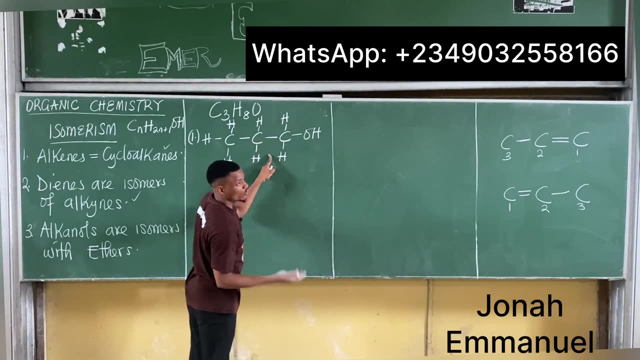 at the extreme, this one here, oh, and i now do: uh, one two, three, four. one two, three, four. one two, three, four. what i have here should be called not just propanol, but what there, propan-1-or why? because if i change this one here and bring it here please, it cannot be. 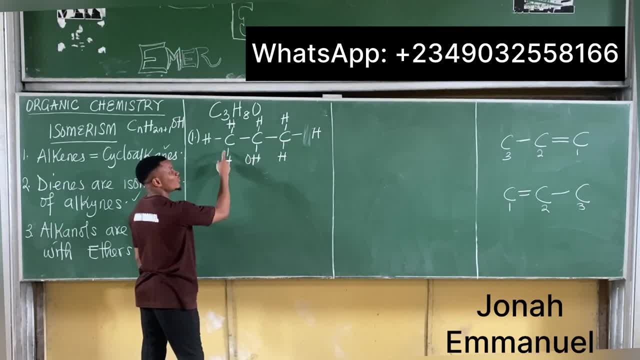 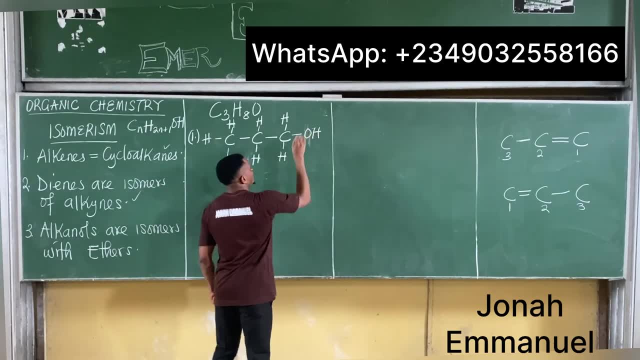 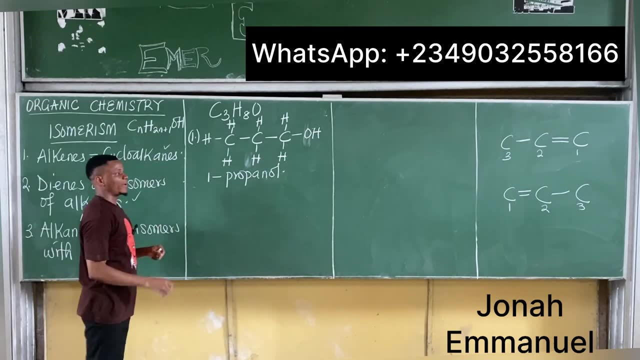 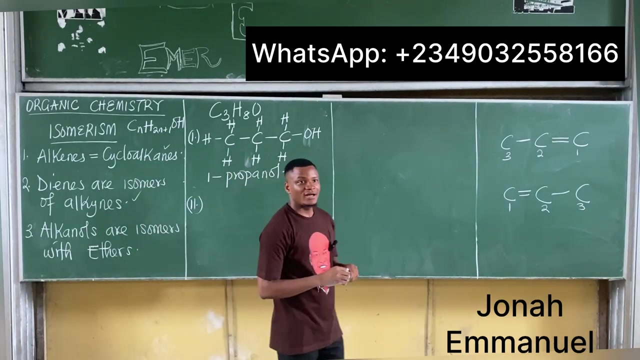 the same thing, because at this point now, if i number, becomes one two, so a two exists. all right, so bring this one here. this now becomes a one propanol or a propan-1-or. that's the first one there. number two: let's get an eta. what's an eta? 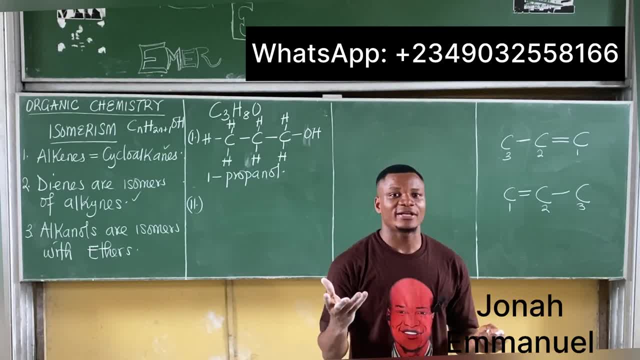 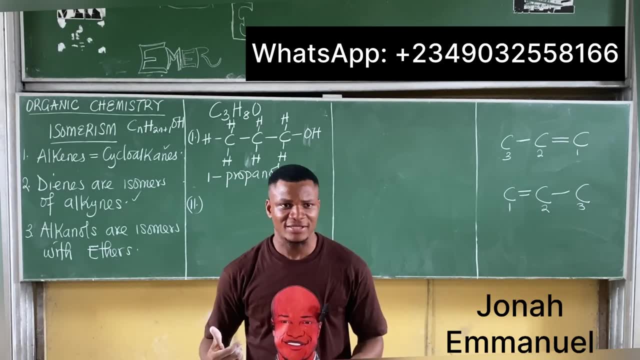 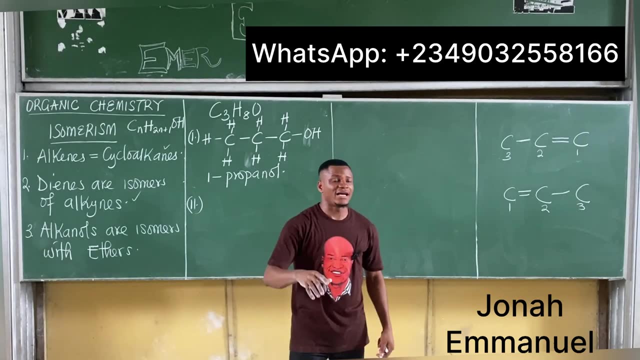 huh, what's an, what's an eta? we'll do etas. i think, yeah, i think we did etas in our previous class. all right, last week, right, we did etas. all right, yes, we did. if you're like, last week we did etas. but don't worry, look up if it's your first. 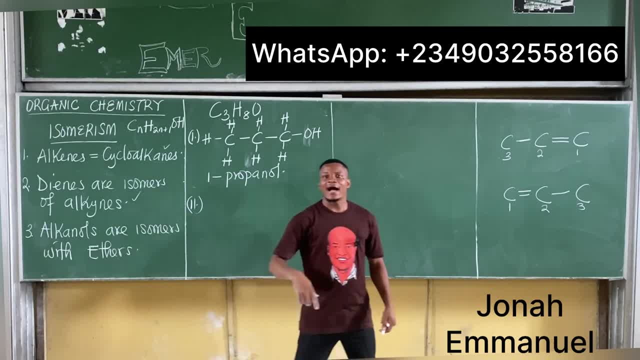 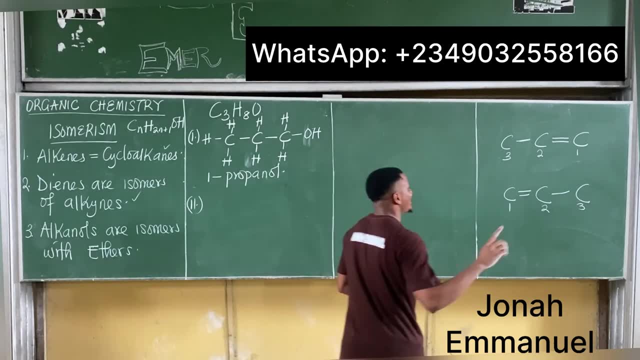 time. go to our first class, our very first class. i give you a table: serial number, homologous series, general molecular formula and functional group. please check. you had eta there. i said for eta you had r-u-o-r. abby, check, you had this. so look up please. what does it mean? look up, please it. 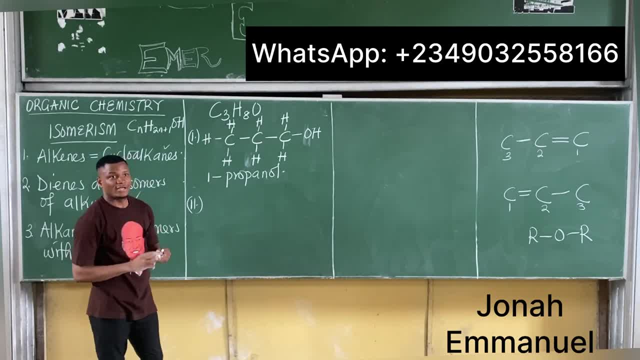 means if i want to form an eta here. so listen, this one can have two answers. if you choose to write one propanol, it's okay. if you choose to use two propanol, it's still okay. let's get the eta for the eta here. my task will be this: 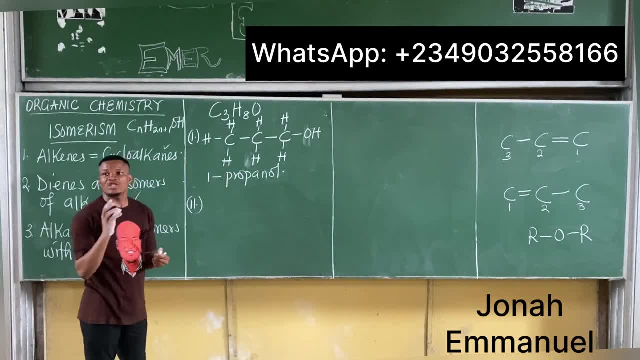 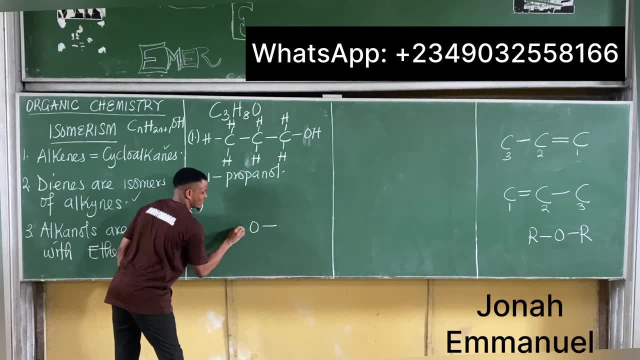 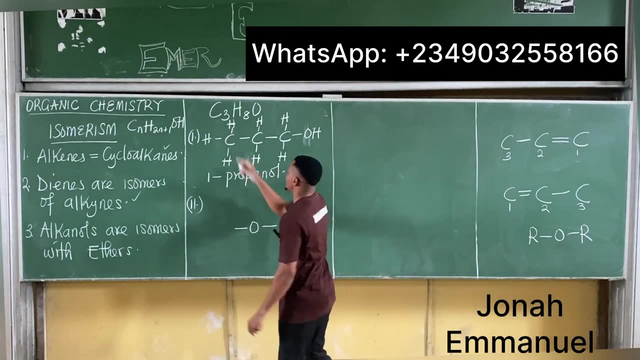 i'm having r-o-r and i think the the most important part there is the o, or the oxygen at the center. so i'm having o at the center here, this and this. what this r means, it's just simply a chi group. if i'm having three carbon, it means form. 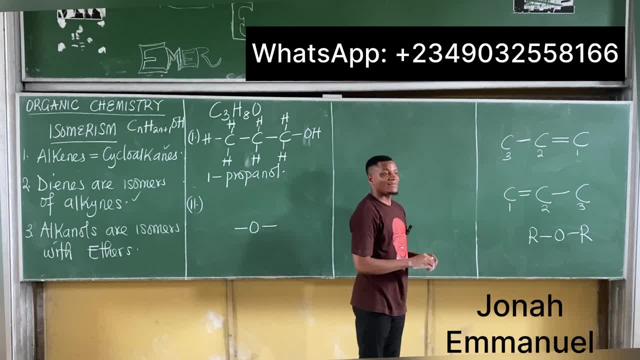 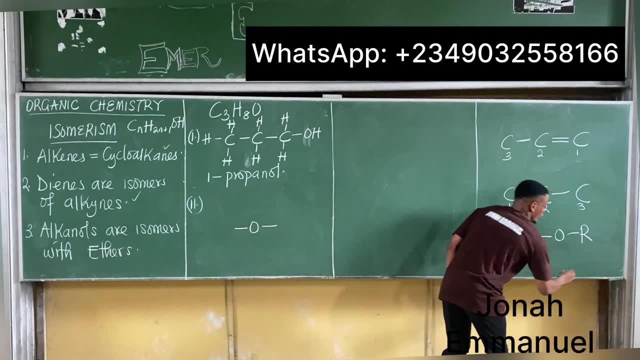 three carbon are chi group from both sides. that means i can have ch3. that's what they're making for ethyl. what's your formula there? c2, h1, there, right, you can have this. so this is methyl, this is ethyl. if i combine what i'm having, look up please. if i combine, i'm having c and c2. 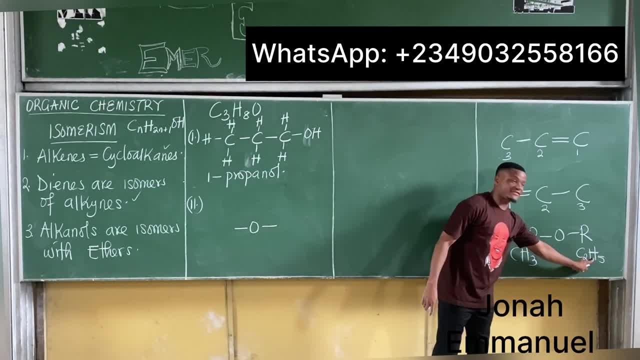 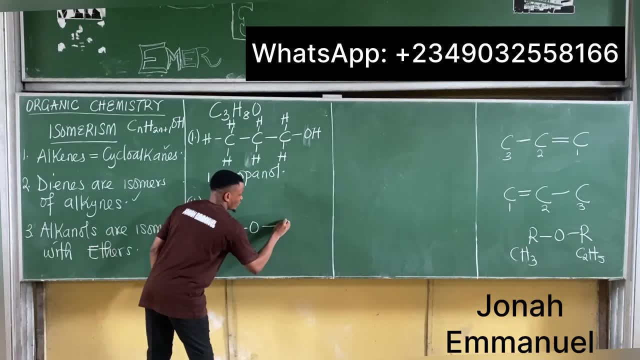 in total c3, h3 and h5, h8, and then, oh, so it's correct, that means for this. i come here, i see c, h3, c2, h5. you should know how to draw this in full right: ch2, ch3. how do you name this compound? 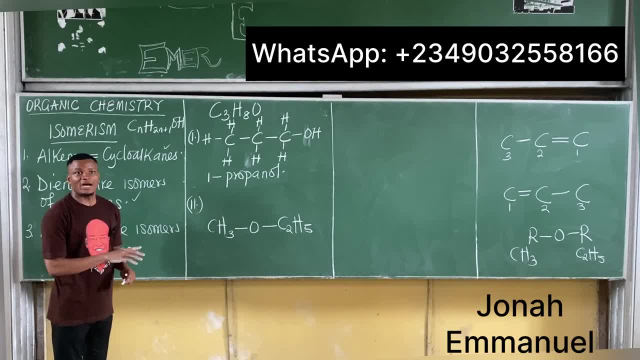 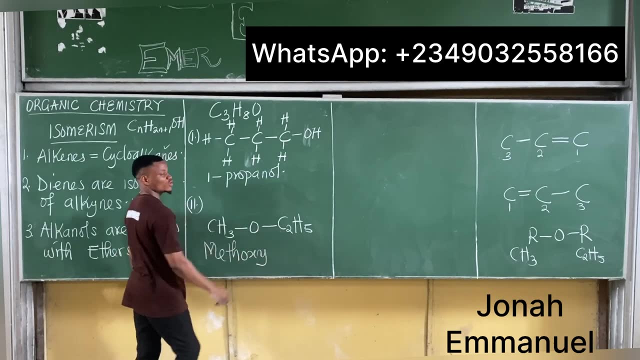 now listen. i showed them how to name this last time. how do you name this? i'm having one carbon. one carbon is what there. one carbon is what it becomes metz. then this one becomes an oxy. this one is sullin 2.2ll. it's not codice used there. 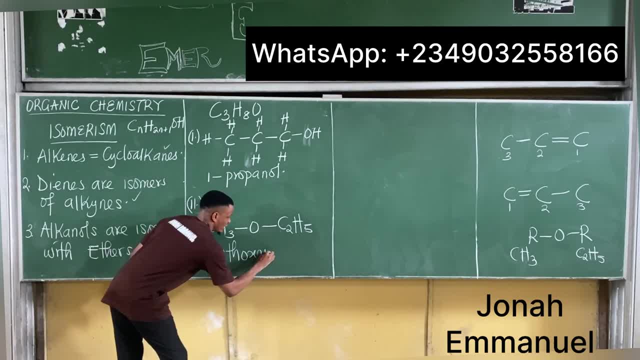 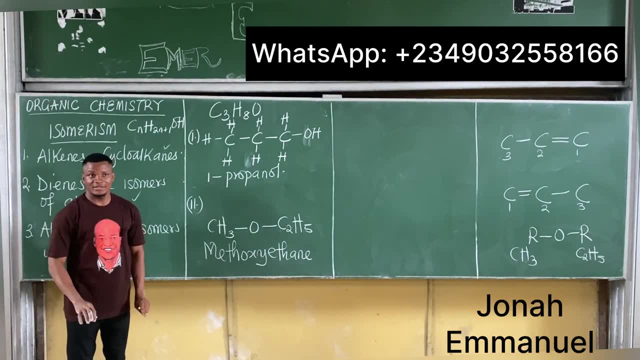 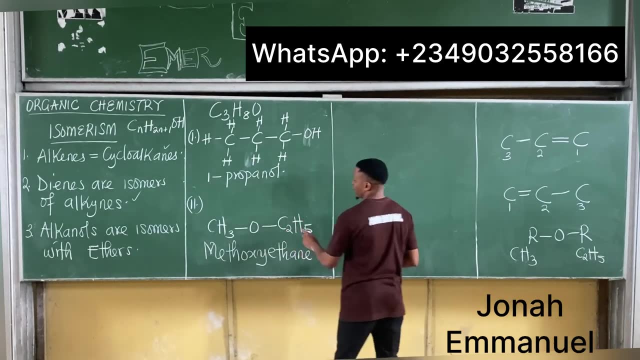 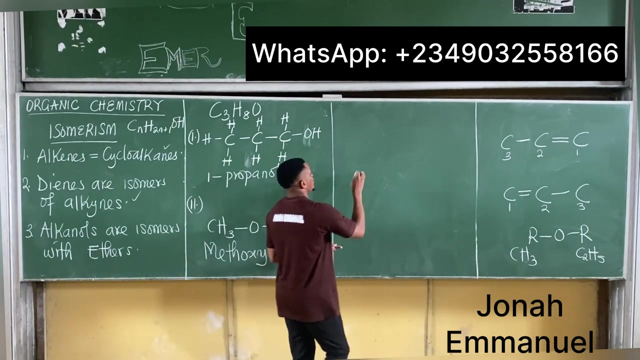 earth. you call it as an arcane, it becomes what there it is called metoxy. et. now keep it pending. what if you choose to flip it? if i flip it, that means this one comes first. so i'm having now listen, listen, i said better still. if you want see, if i flip it, it should be something like this: c2. 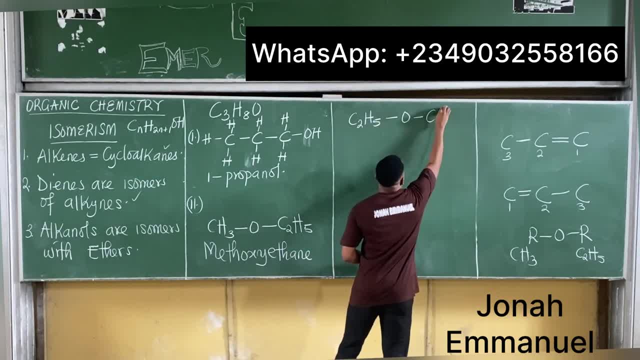 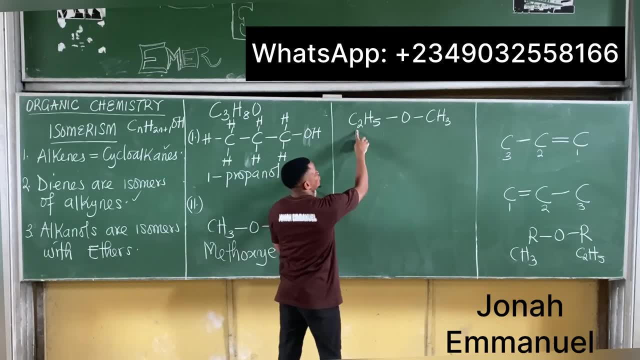 h5, o and then ch3. i flipped it. but this salt, this stuff here is not proper. it's not proper. so arrange it. if i have c2h5, please arrange. this is a molecular formula. arrange it in condensed form. only be there. ch3, are they ch2? what again there? oh, what again here? ch3. so i have. so c2h5. 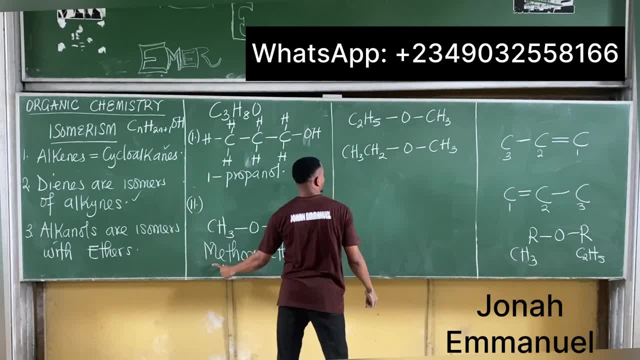 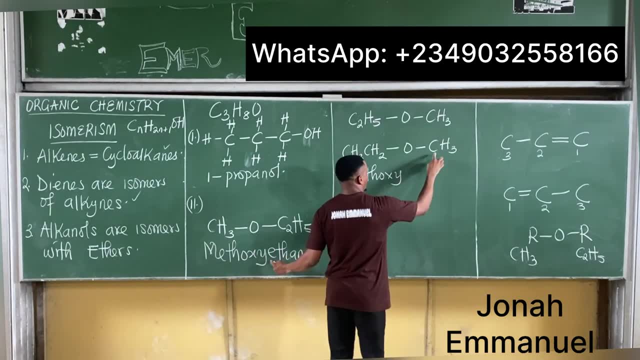 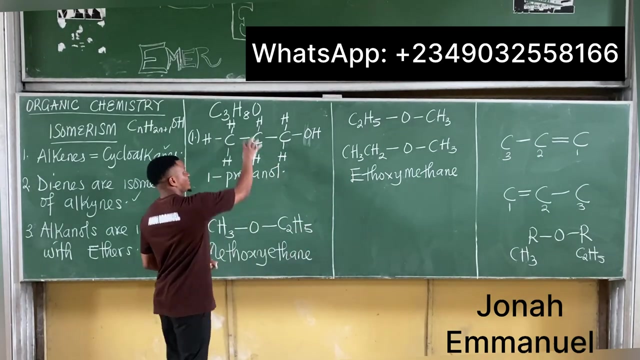 how do you name this? please observe: it was met two. carbon gives you what there, x, so it becomes etoxy. what there? it doesn't. what methane, please? methane, because it's one carbon, etoxymethane. so the idea is simple: x, oxy, then methane, so they say: name two. you can just pick this and this or this and this. now hold on though. 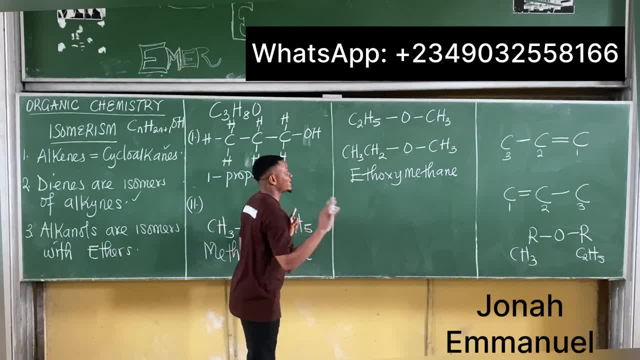 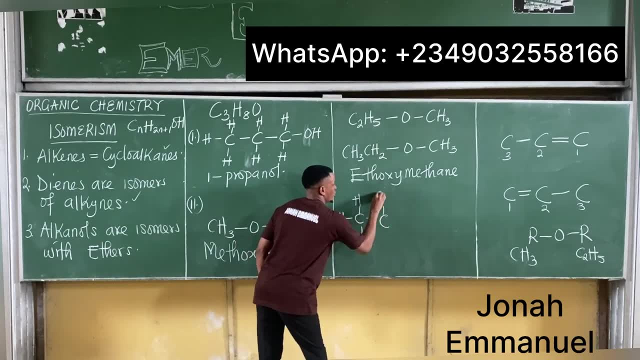 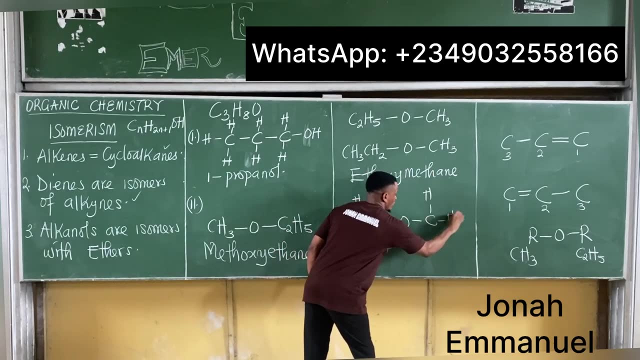 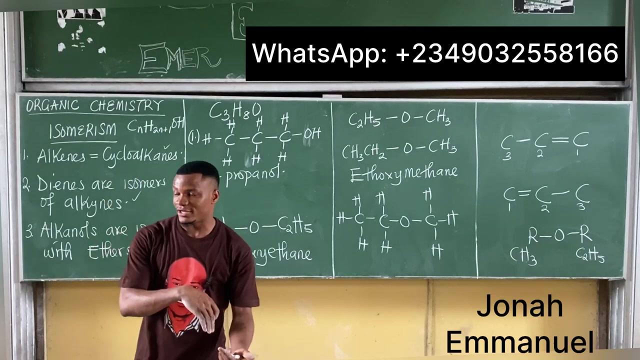 since they say: draw the structure, don't give it like this, give it like this instead: um, this one comes: c one, two, three, ch2. c one, two, oxygen, o c, c one, two, three. so here is what you should have, so the difference between a metoxy ethane and an etoxy methane. all right, yes, question. 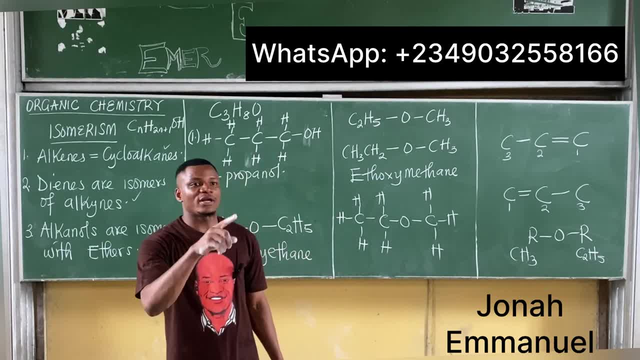 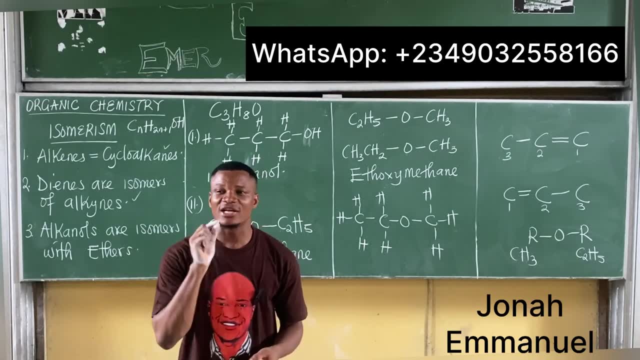 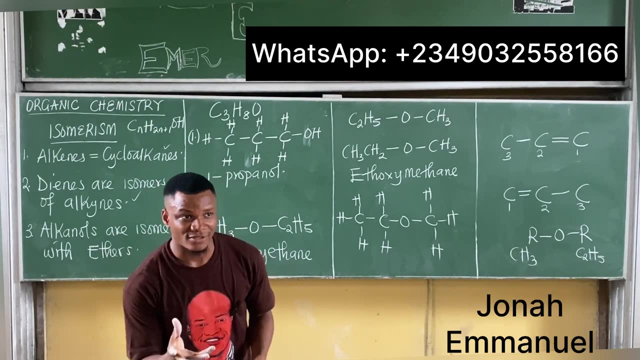 yes, uh, is that also an archive group for your level? yes, class, we'll do other things too. archives are what they're. substituents from water are kings. by what? the loss of one hydrogen. next we look at a second type called the phenyls or the benzene. what's a benzene? a benzene is a substituent that you get from a benzene. by what? 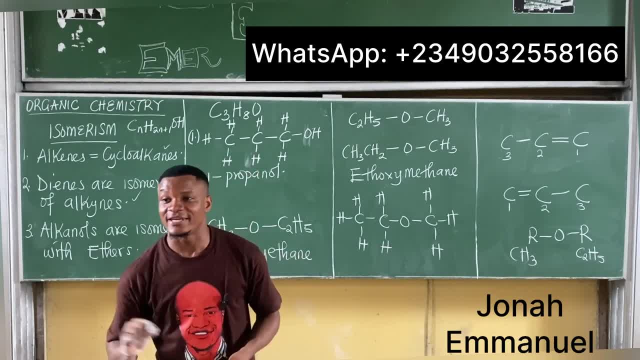 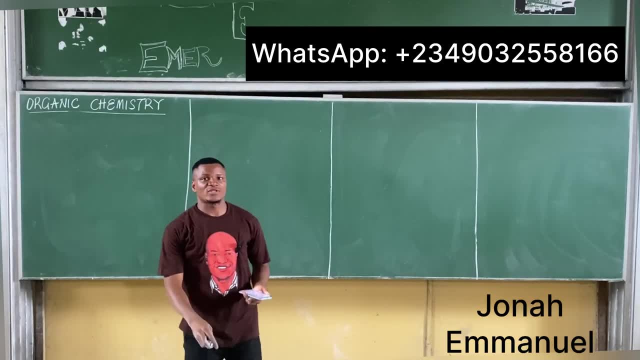 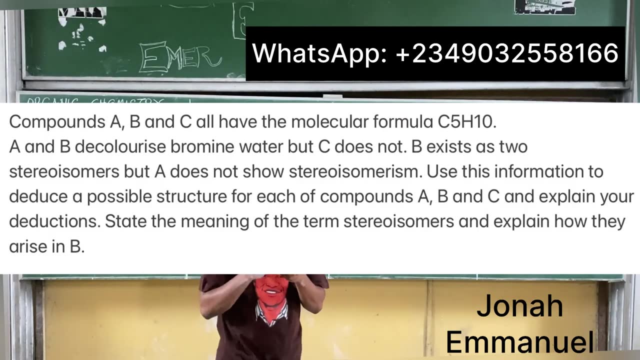 the loss of one hydrogen example, phenyl. we'll treat in the next class, but for now just hang on with this. all right, for recording purposes. please check your question, please. compounds. let's try this question, please. compounds: a, b and c: all have the molecular formula c5h10. full stop a and b. 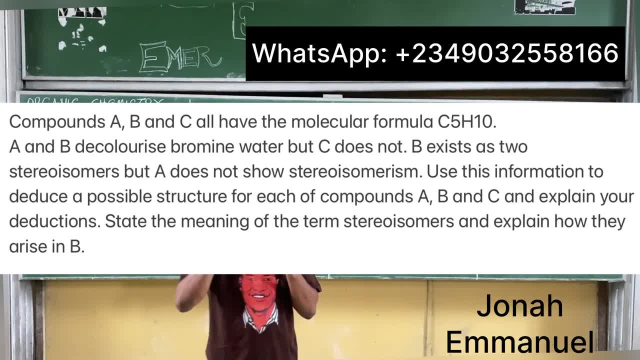 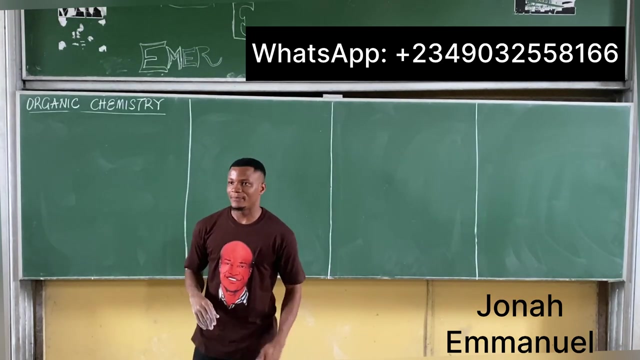 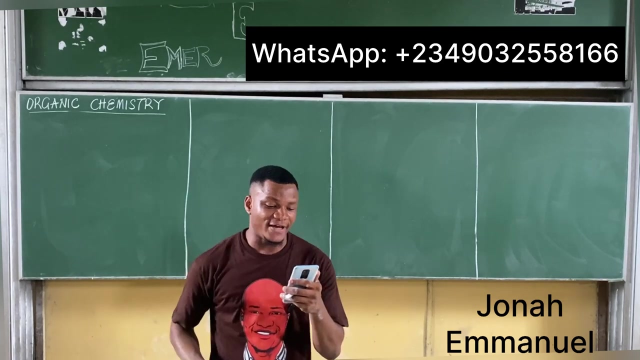 decolorizes bromine water, but c does not full stop. b exists as two stereoisomers, but a does not show stereoisomerism full stop. use this information to deduce a possible structure width of nitrogen and hold them together as its Banchal. 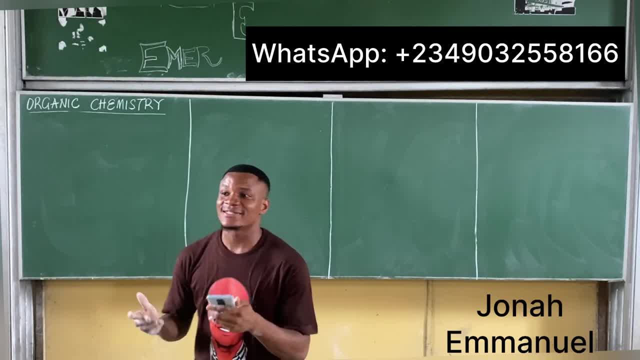 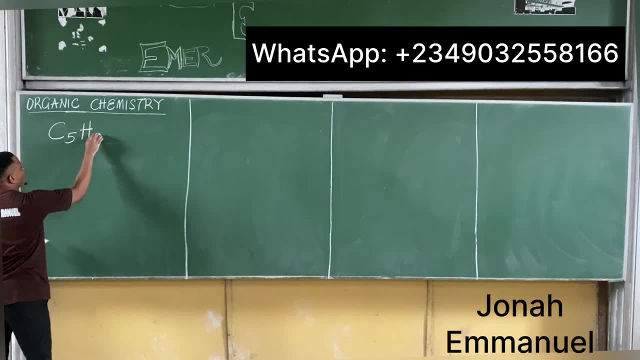 of each of their compounds say they have one there. molecular formula: what c5h10, PROP3s고qualivingc10, THO cookies? there we go, something like that. anything you can do here, as you can see now C5H10, all right, so let's say it's done. I'm having a C5H10, so that's my first task, okay, so what next? 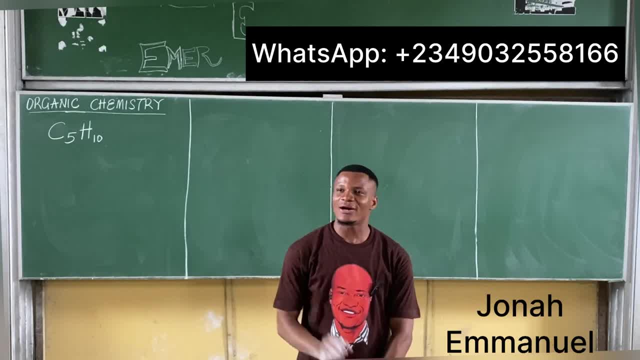 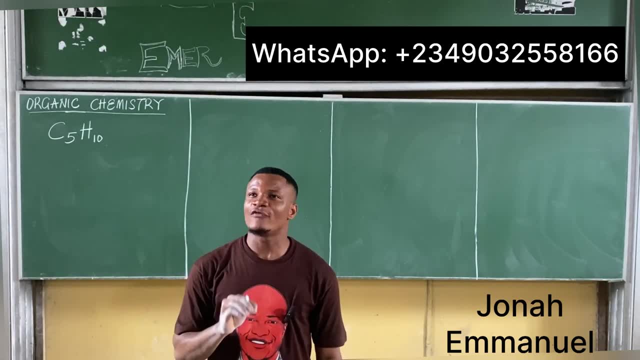 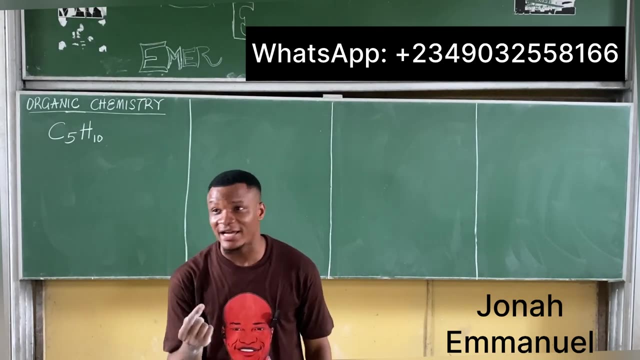 they said an A and B decolorizes bromine. now, hold on, I have, when you do your practical, when you do that bromine, something which of the homologous series decolorizes bromine. was it just alkene? it was alkene. I want there alkyne. that decolorizes bromine. so if they say A and B decolorizes that, 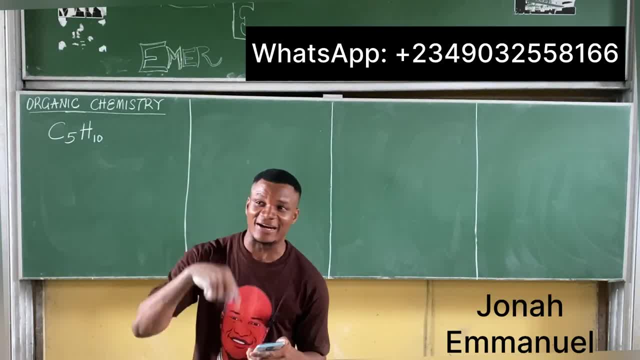 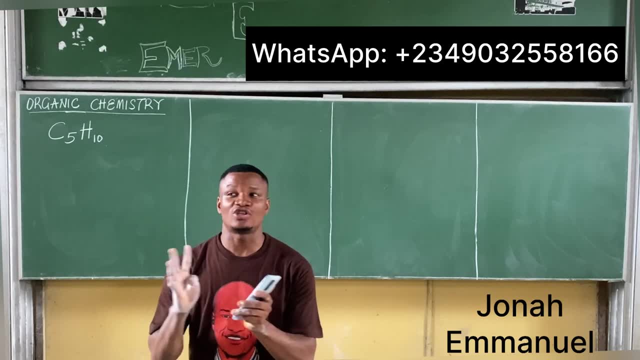 mean most likely A and B. I want there either alkene and alkene, or alkyne and alkyne, or alkene and alkyne. whichever way, my first deduction or my first hypothesis or my first inference is that A and B are most likely alkene alkyne. keep it pending, let's move on. they said. 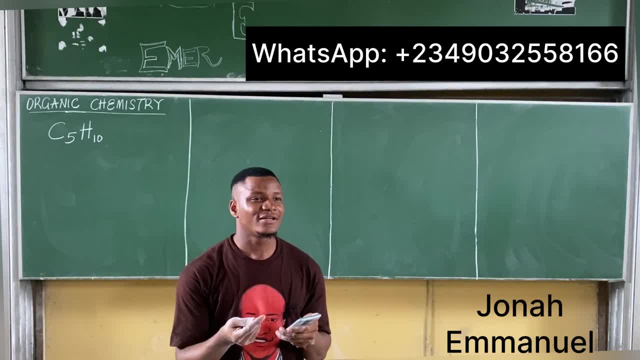 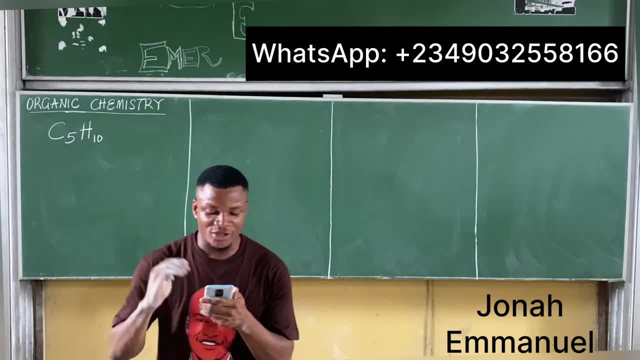 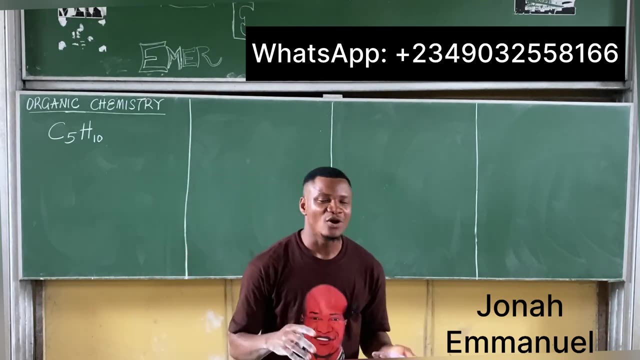 but it does not. which of them does not? so cis and alkyne. so see, I'm doing it now. so A and B is most likely alkyne, alkyne, cis and alkyne proceeding. they said B exists as what? there? two stereoisomers. let me break it down to the simplest form. when we say stereoisomers, what we 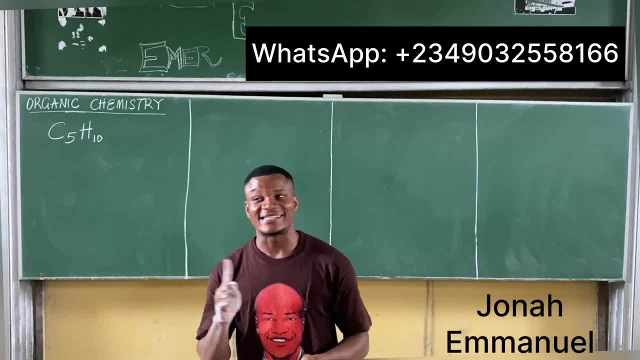 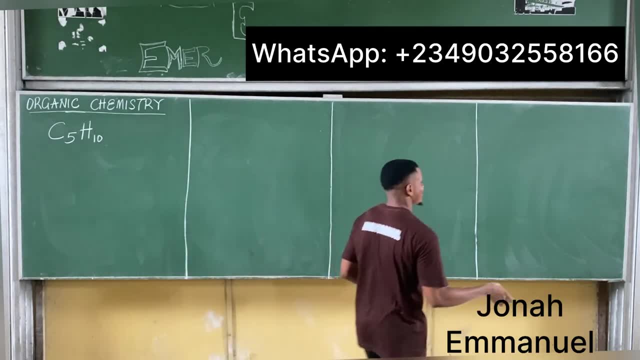 mean in the basic sense, is your cis and trans system cis and trans? now, if you remember how we do cis and trans, it's something that looks like this: cis and trans trans looks like this, something of this nature are we? yes, this is cis and trans system now. 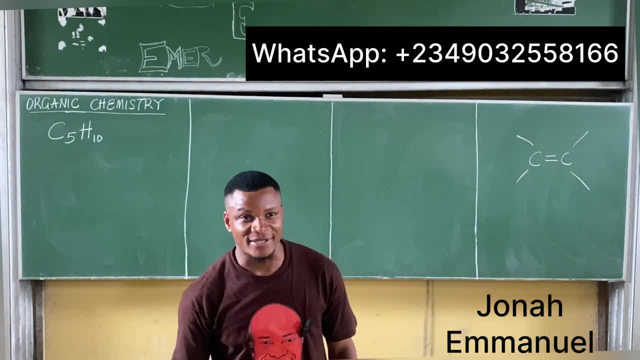 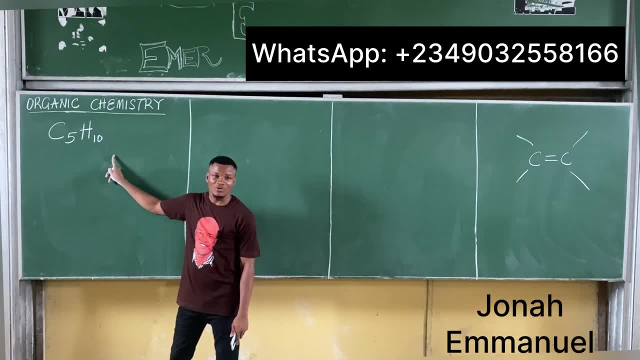 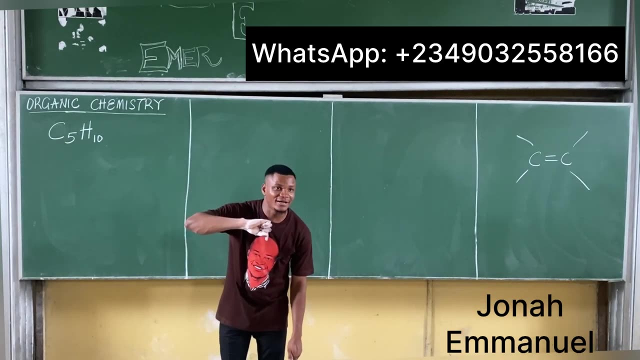 let's see, get something right. let's get something right, please, considering this formula c5, each step, please. can this be a alkyne? huh, no, this cannot be a alkyne. this can be what an alkene Trans throw, strapping a syn 102. 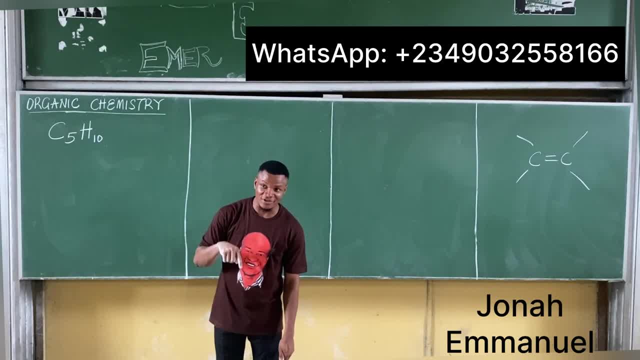 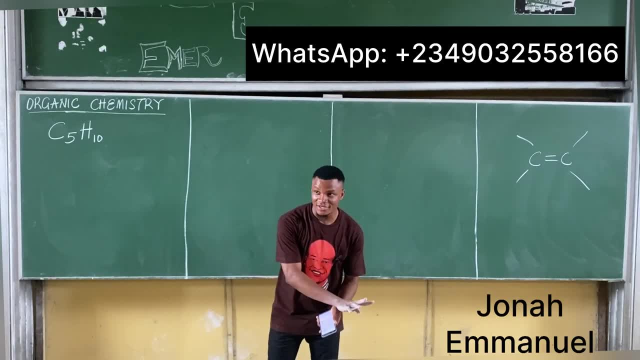 чис where A falls under cycloalkene. Remember, we said A was an alkene And we know that the isomer of an alkene is what there, Cycloalkene. So we've gotten A, But keep it pending for now. 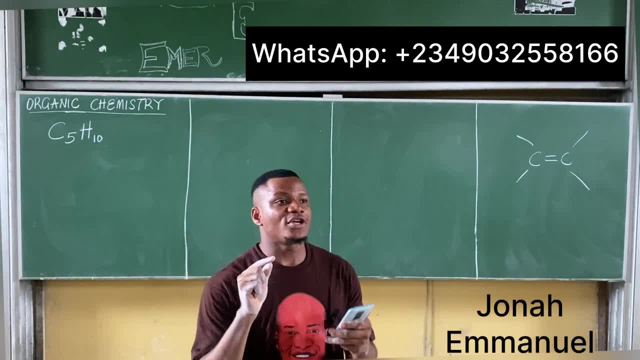 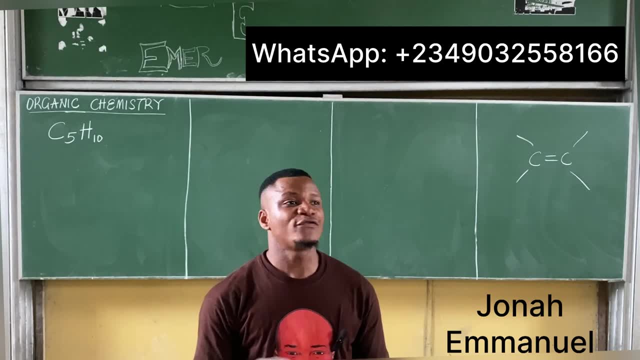 So listen again. Initially we said A and B should be what there, Either alkene or what there Alkene. We've just said: alkene is not possible, Abhi. Yes, Because of what there? The formula. 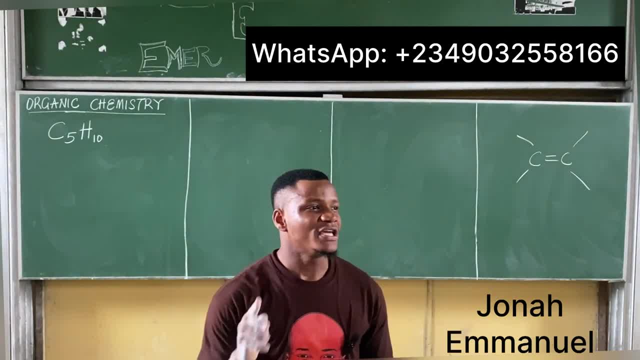 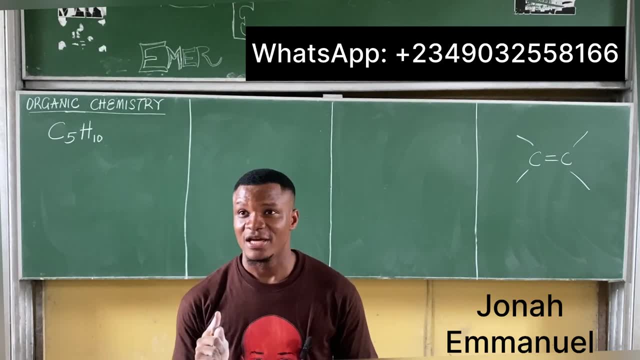 So if that's what it means, what does it mean there? It means that what there, A and B are both what there- Alkenes Or alkene Double bond please. It means A and B are both what there. 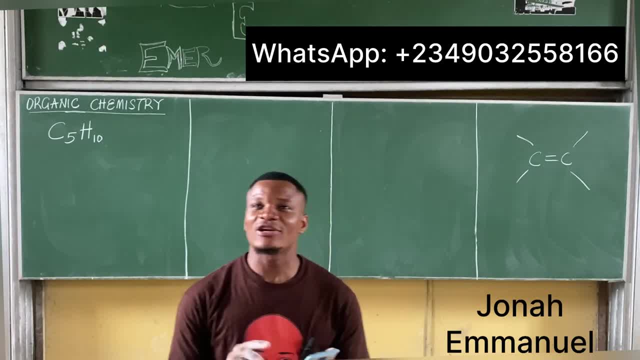 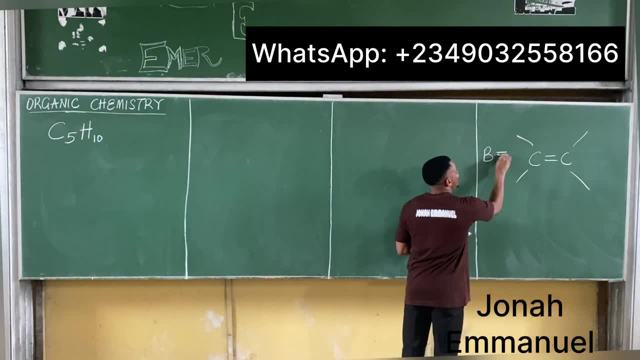 Alkenes, Because they decolorize what there Bromine. So what kind of alkene? It has now specified that B. is it B? Yes, It says B exhibits what there- Stereoisomerism. But see what there. 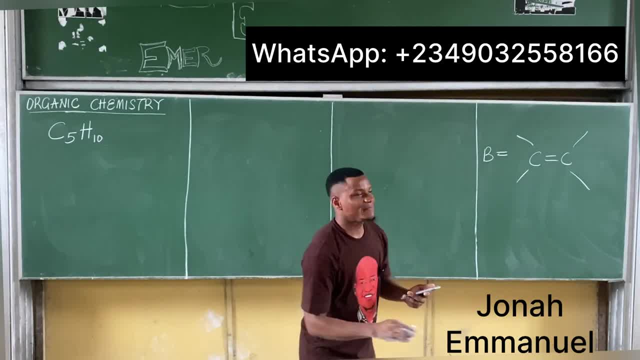 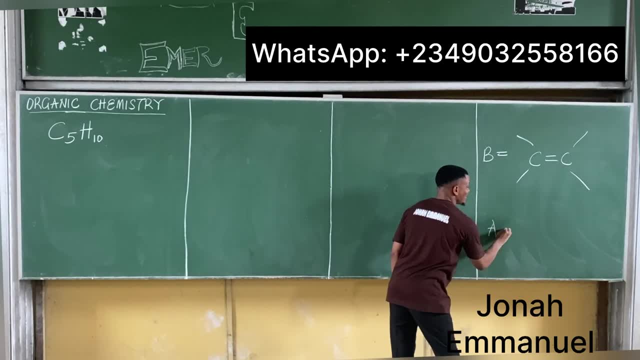 But A does not show. So here's the thing: It means that B is an alkene that exhibits stereoisomerism, while A is still an alkene, but it does not do what there Exhibits stereoisomerism. 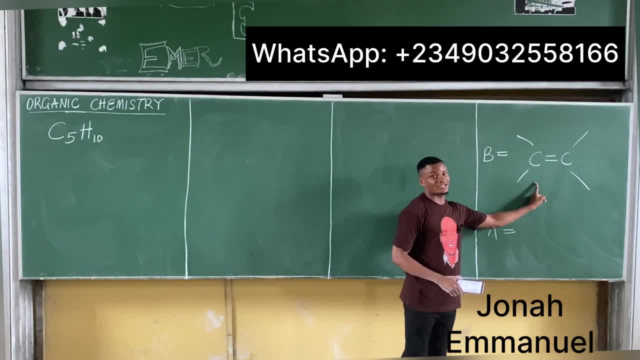 A and B are both alkene. B is showing C strands, A is not showing C strands. If A is not showing C strands, what does it mean there? It's what It's straight carbon. All right, let's proceed there. 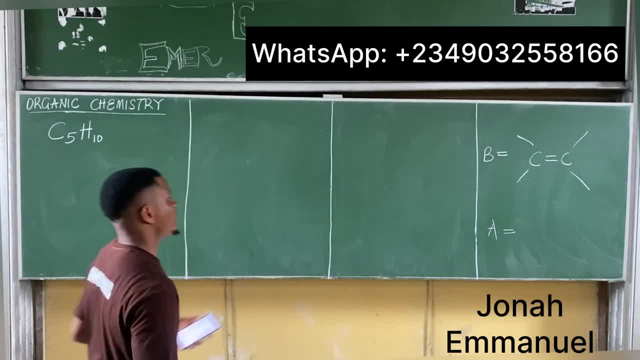 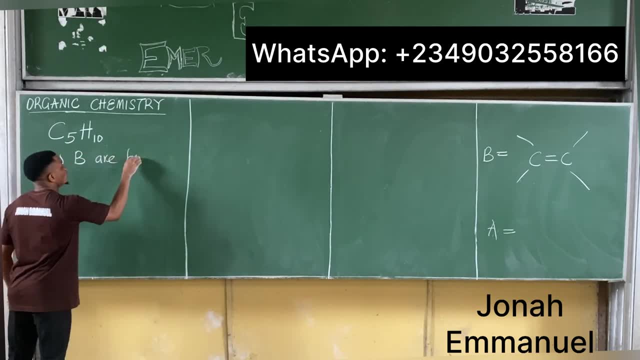 All right, you said information Okay, so let's get this done, please. So first things first. we know that A and B are what there. They are both alkene. That's what we know, While C is what there. 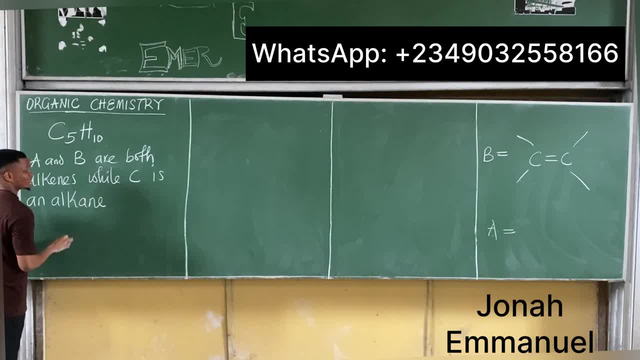 An alkene. Why an alkene? It doesn't decolorize bromine water. So which alkene will have C5H10? The cyclo of it. We just said that. So let's get a cyclo alkene with 5.. 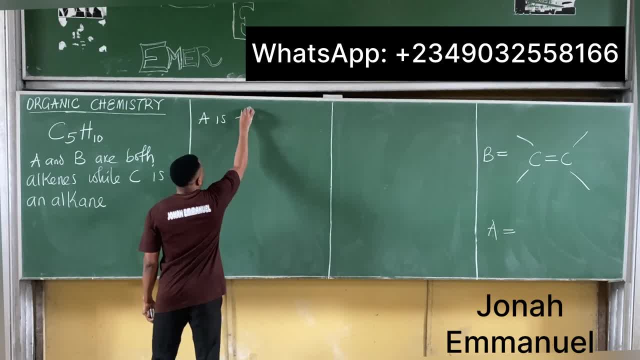 That would be so. A is therefore, I'm having 1,, 2,, 3,, 4, 5.. So I'm having 1,, 2,, 3,, 4, 5.. That's a cyclo. 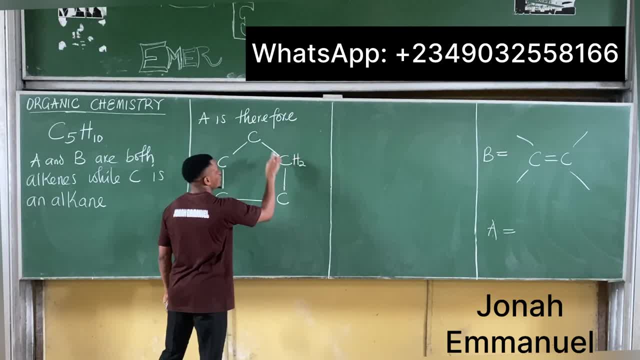 Let's use an alkene: C, H2. C, H2. C, H2. C. 1, 2, H2. C. 1, 2, H2.. So here's an alkene that has 1,, 2,, 3,, 4,, 5.. 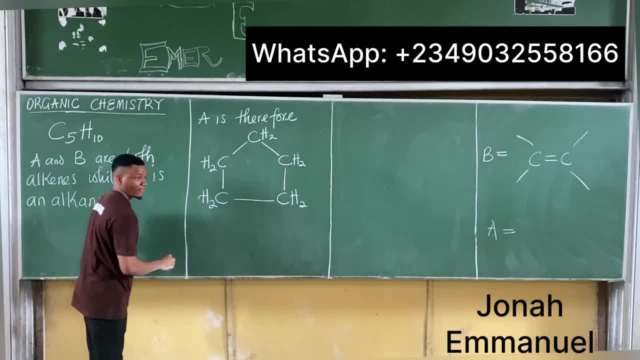 C5,, 2,, 4,, 6,, 8,, 10.. H10.. So therefore, It's what Cyclo, what? Okay, it's A, It's C, Sorry, sorry, sorry Right. 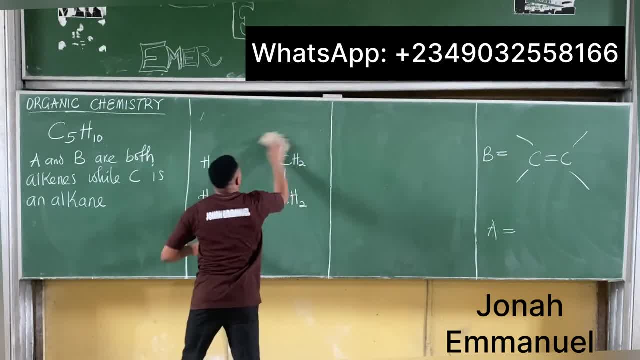 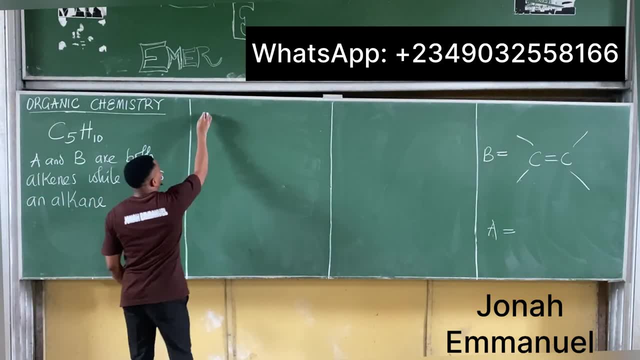 So let me repeat this with you, sorry, Sorry. yes, You said C is the alkene, please, So C is therefore. C is therefore a cyclo alkene. That's 1,, 2,, 3,, 4, 5.. 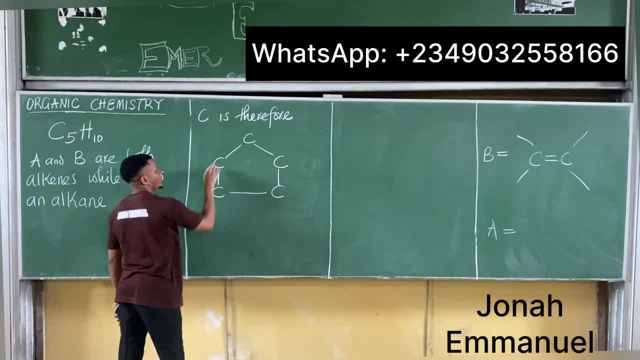 So, here, here, here, here here: 1, 2, H2.. That's 1,, 2, H2.. That's 1,, 2, H2.. That's 1,, 2, H3,, 4, 5.. 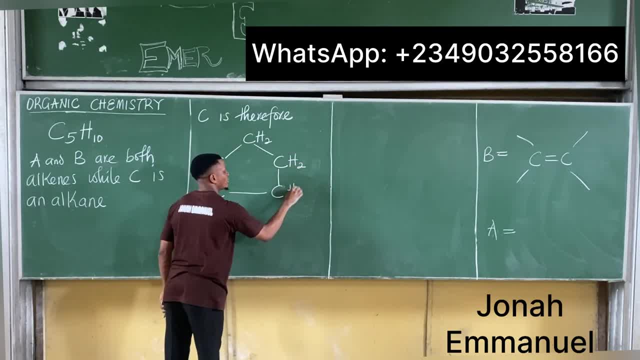 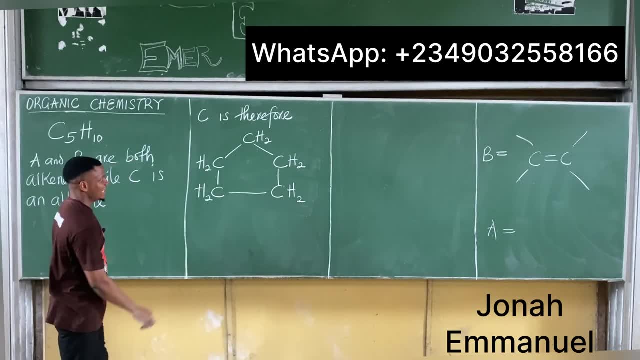 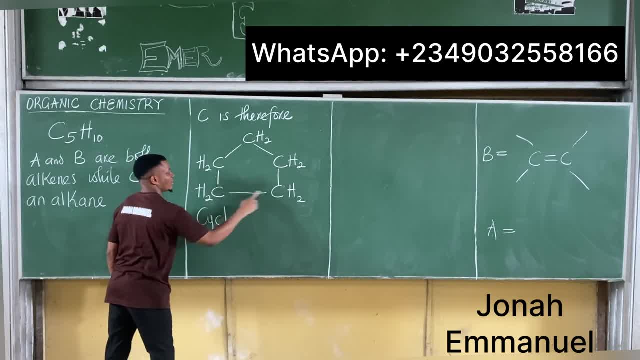 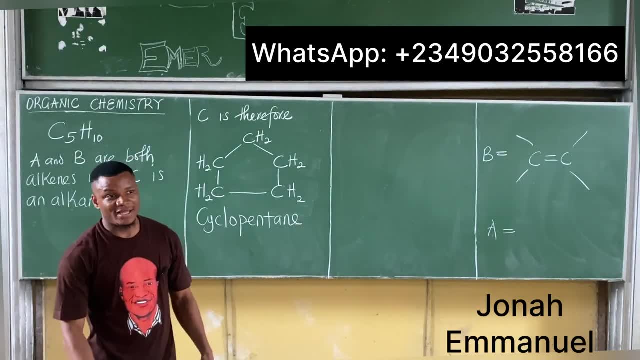 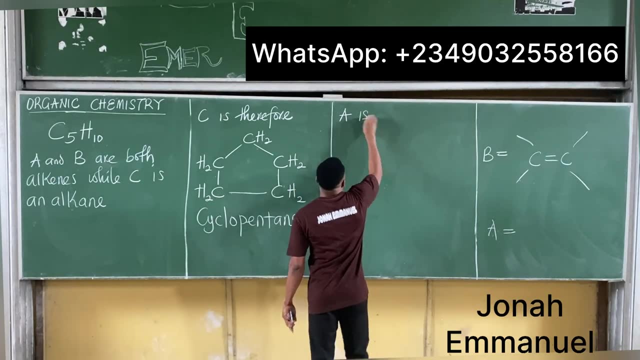 a word there: cyclo: 1, 2,, 3,, 4,, 5,, 10,, 10,. I have deduced C. I'm left with word there: A and B. let's get A for A. what will A be? A is an alkene. now we said we know what. 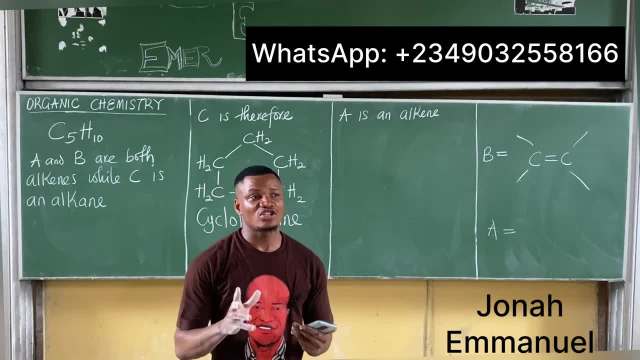 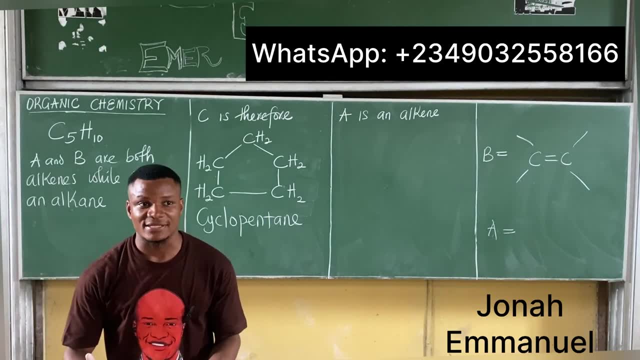 A is an alkene. but it said: A does not do what there. it doesn't do what there exhibits sterilizing medicine. so we are having an alkene that is not cis and trans. if it is not cis and trans, what does it mean? there it is straight alkene. so I'm having C5, it. 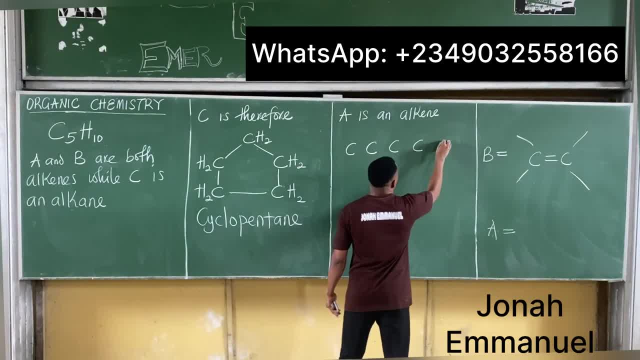 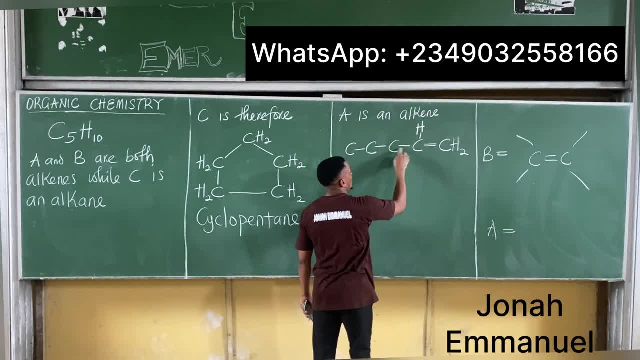 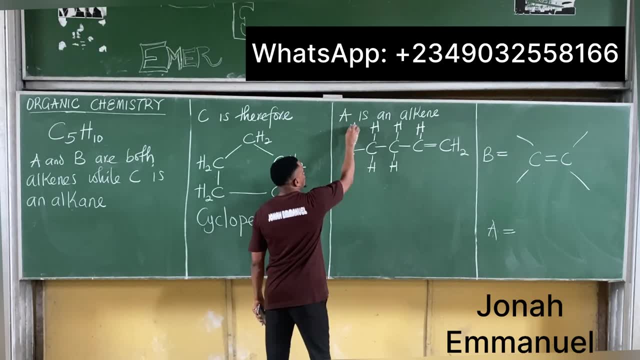 H2, 4,, 1,, 2,, 3,, H 1, 2,, H H 1, 2,, H H 1,, 2,, 3, and 4, so how do you name this this? 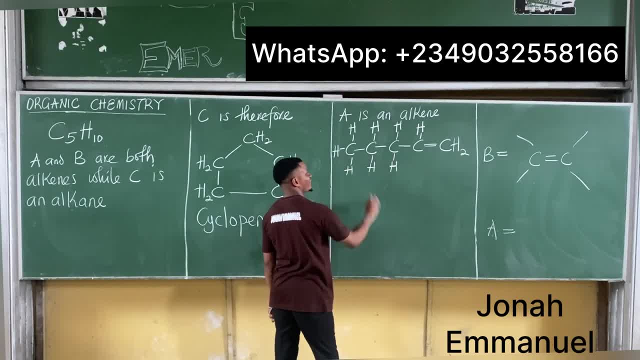 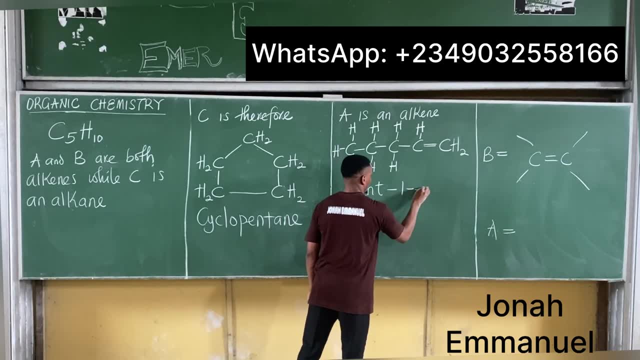 is what 1, not B 1,, 2,, 3,, H 1, 2,, 3,, 4,, 5.. 5 is what Proof Pent, Please, pent Pent 1 in. 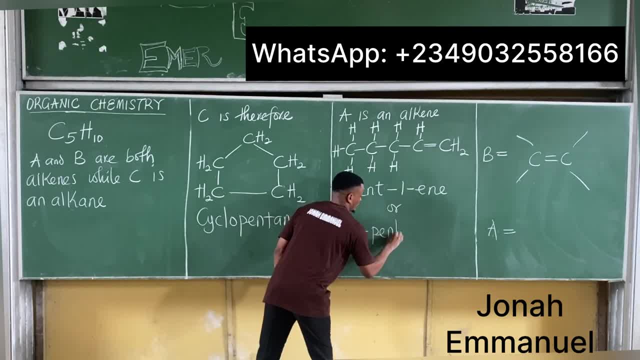 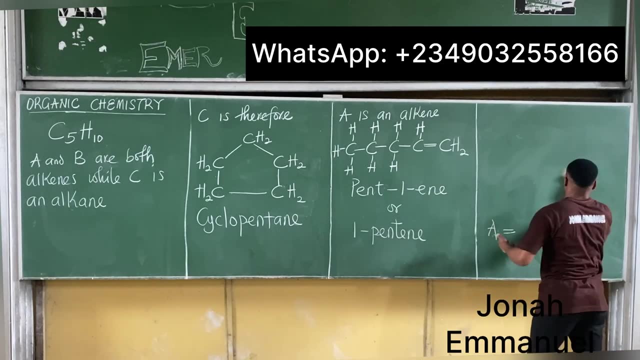 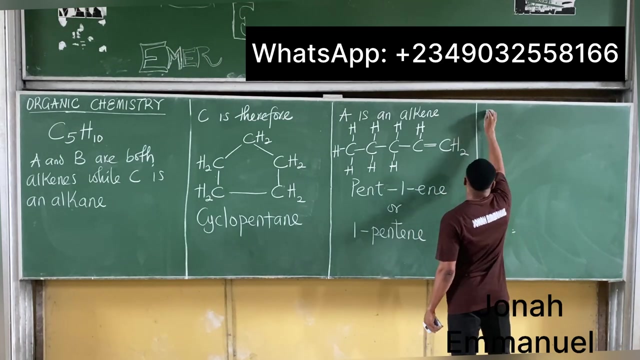 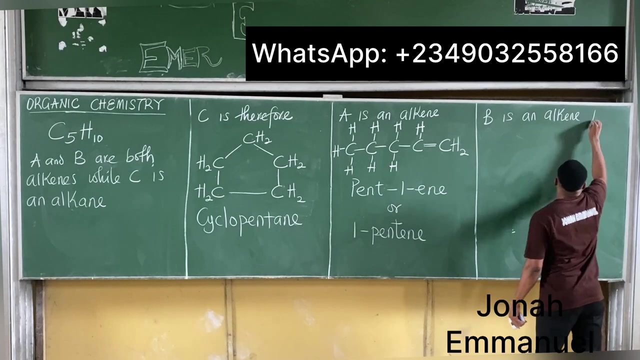 Or 1 pent in. B is also an alkene that exhibits stereoisomerism. So because of what there Cis-trans concept? So let's get B, So let's get B. So B is an alkene, that is a. 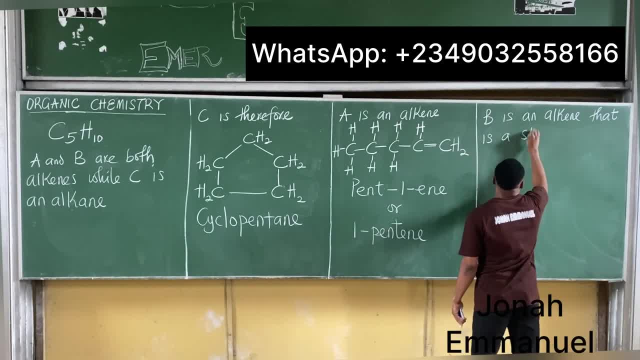 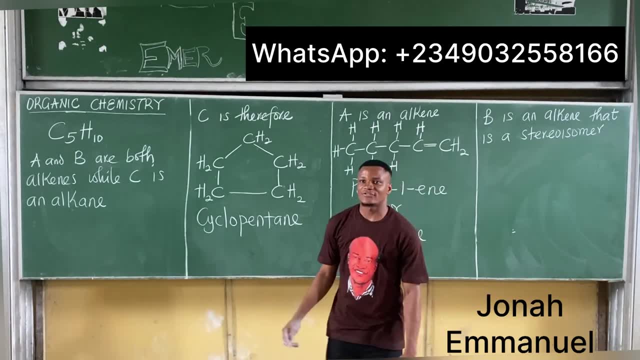 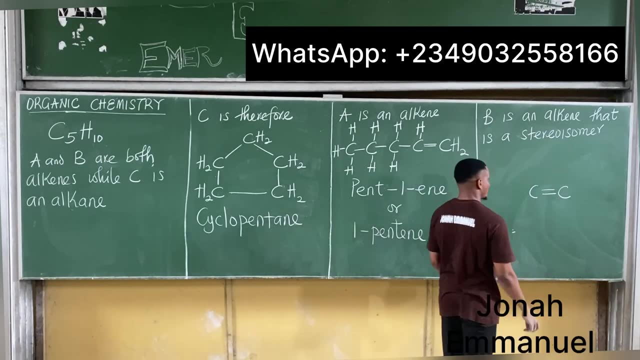 that is a stereoisomer. That means form a cis and a trans from this. So for my cis-trans, my first case is to get these two carbons first and then complete it C5.. You can see C, of course. C, I'm having 1,, 2,, 3,, 4.. 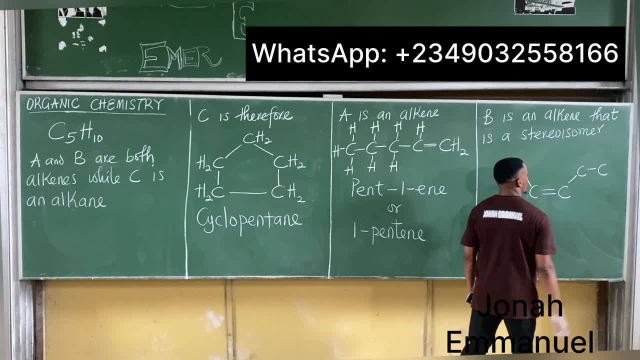 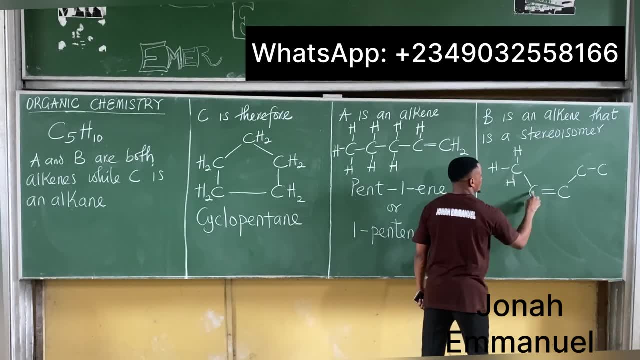 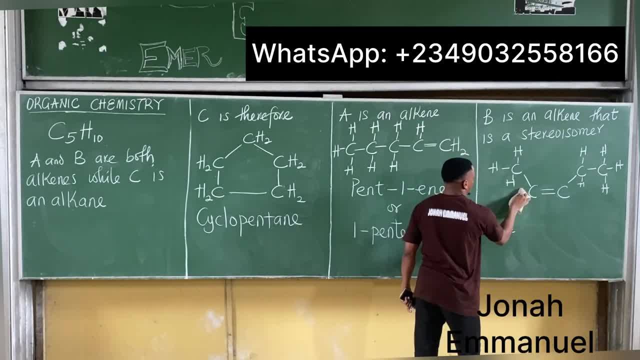 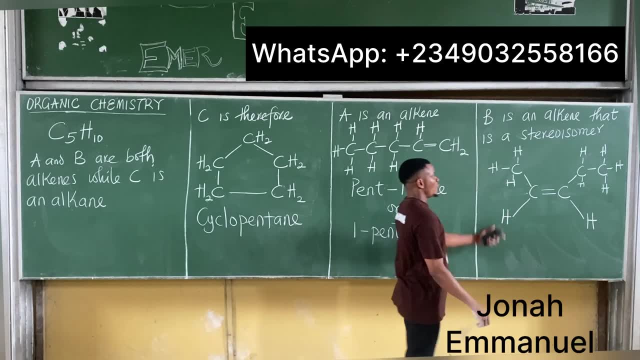 For this one here. for this one here. we know how they should look like. Are they Yes For a cis-trans? I'm having this, What I have on the board. please Let me make this H bigger. I'm having this. 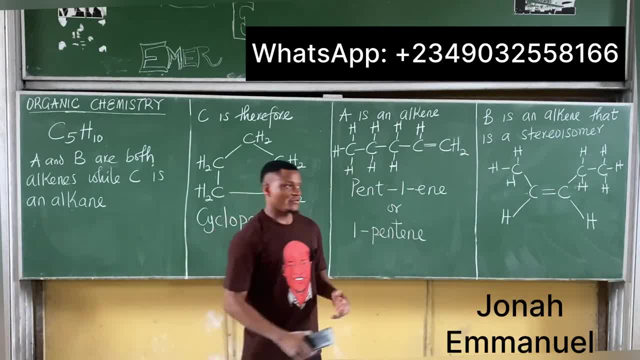 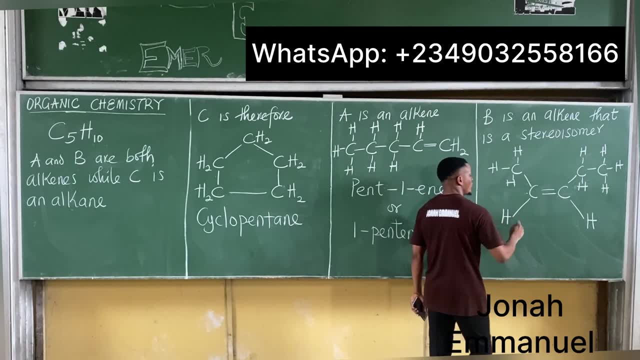 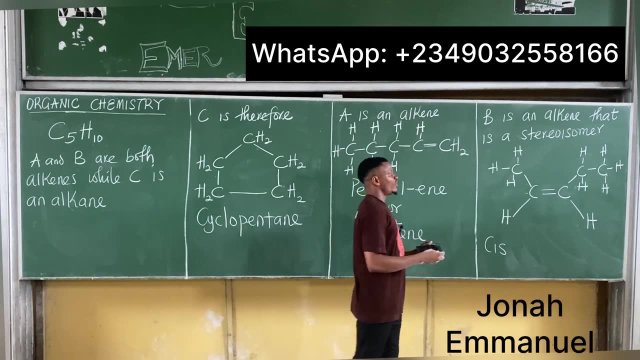 Is here a cis or a trans? Obviously cis. Is that for cis, The two hydrogen will be what? there, the same plane like this. so gives you cis, so cis what. this is cis, cis, what. how do you number? which of them gives you the shortest distance to double bond is from left. 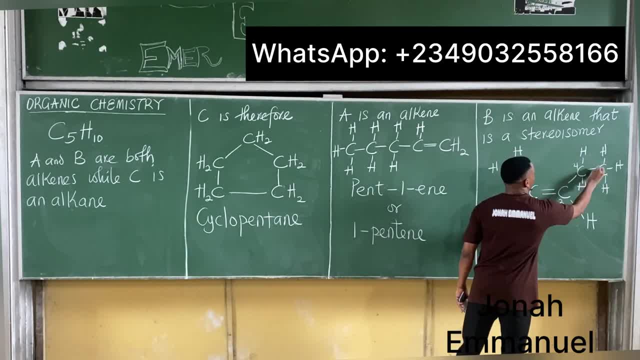 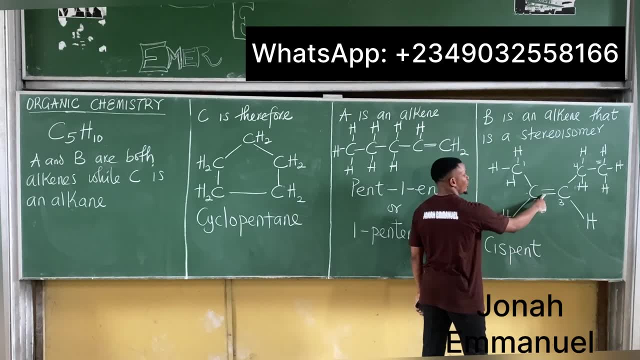 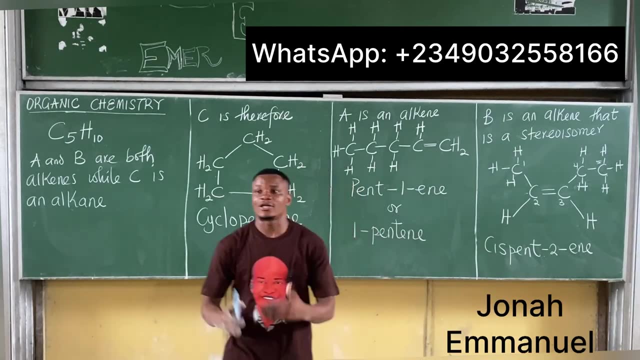 so i'm having one, two, three, four, five. all right, so name this becomes: cis pence five, carbon pence- what there? double bond is on carbon two. cis pence two, what there in? i have this. if you want to use this trans, it's still correct if you want to use the trans. 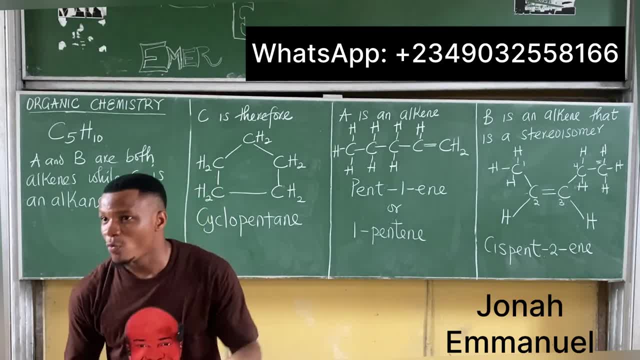 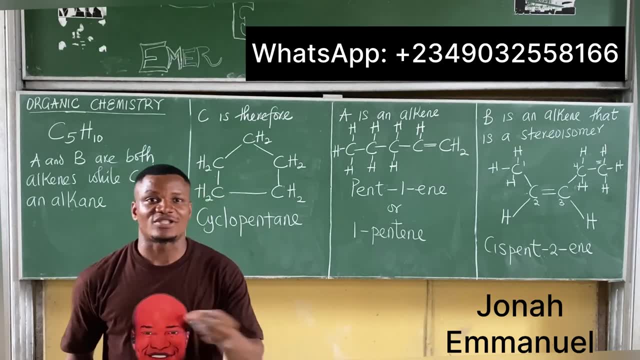 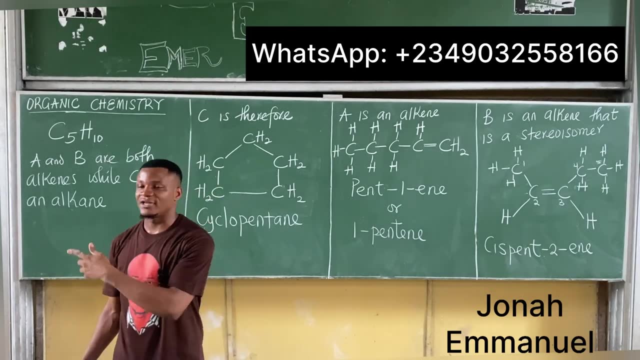 it's still correct. that's what i said. deduce a possible what's possible here. cis is possible here, trans is also what there possible here. so if if your neighbor is doing trans and you're using cis, put a few words there. correct, that's it. i have the mark scheme. i have one of these marks in there. 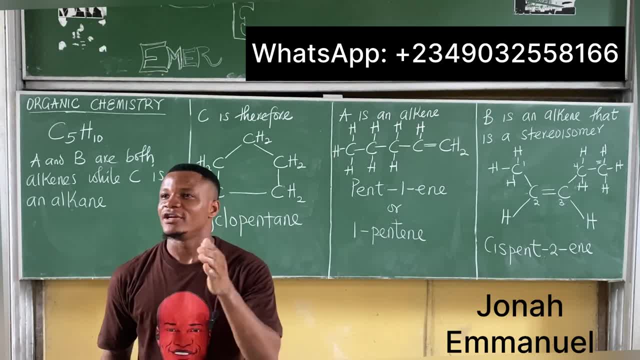 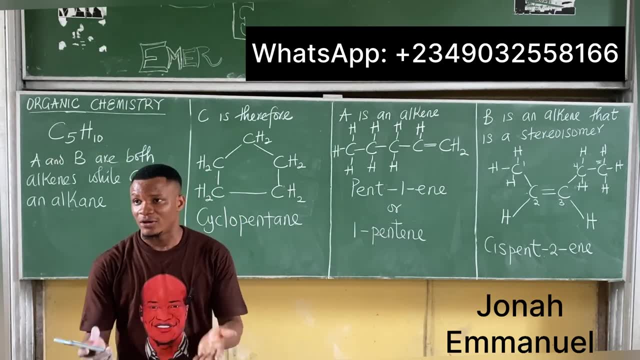 for the maximum they give. they will give a question. they'll give list of possible answer. so while you're doing a cis, the method might be one there, a trans. both of you are there, correct? so that's how we get this done. that's how we get this done. 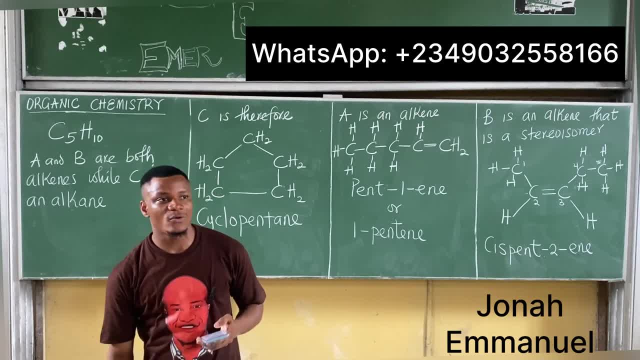 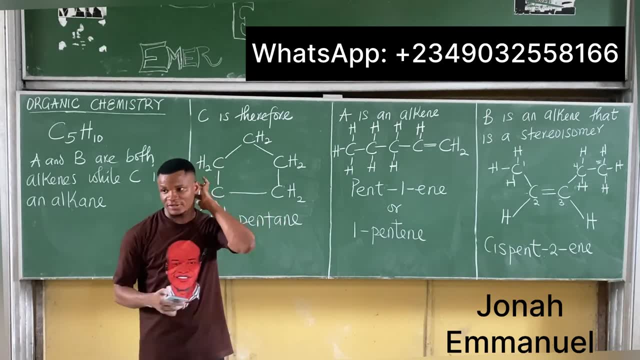 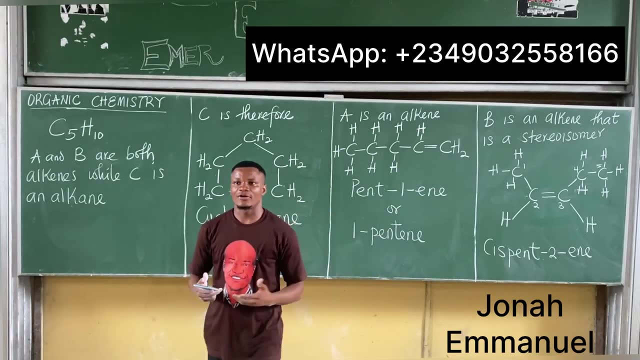 last thing that says states the meaning of stereo isomerism. all right, copy down. let me give you a definition of stereo isomerism and then we can proceed with. so the next thing that says: what is stereo isomerism? here's the definition, please: stereo isomerism or spatial. 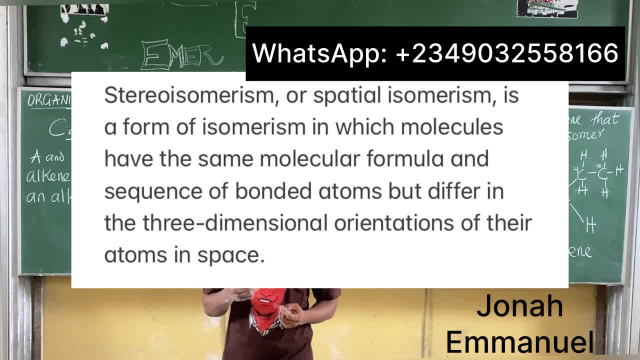 or spatial isomerism, is a form of isomerism in which molecules have the same molecular formula and sequence of bonded atoms but differ in the three dimensional orientations of their atoms in space. last thing that says: and explain how they arise in compounds. and explain how they arise in compounds. and explain how they arise in compounds. 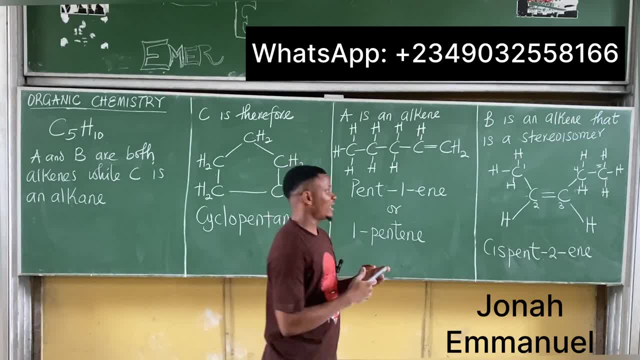 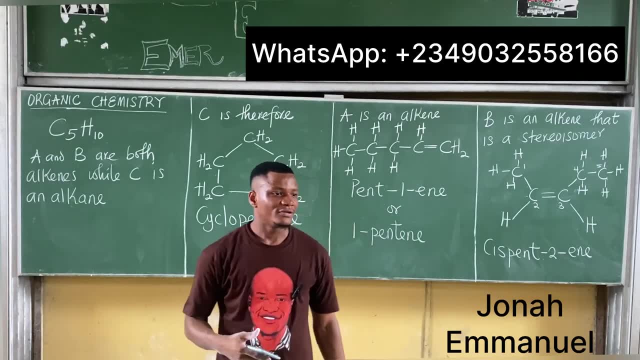 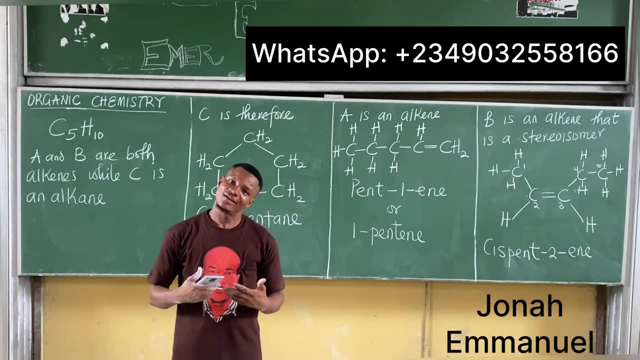 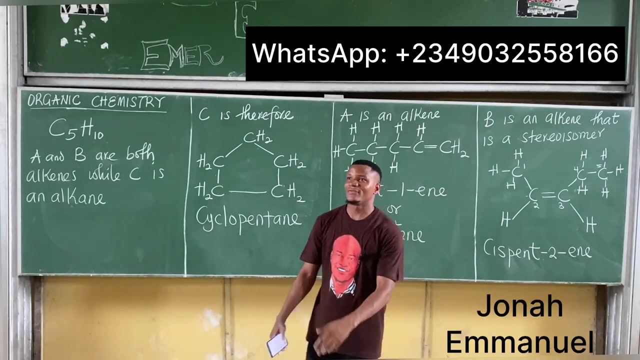 b and explain how they arise in compound b, what would you say? huh, how? and explain how they arise in compound b, what would you say? so you can just say: give them a simple man's concept. we said: denounce him. for stereo isomers there are basically two types, which are what are there? cis and trans. 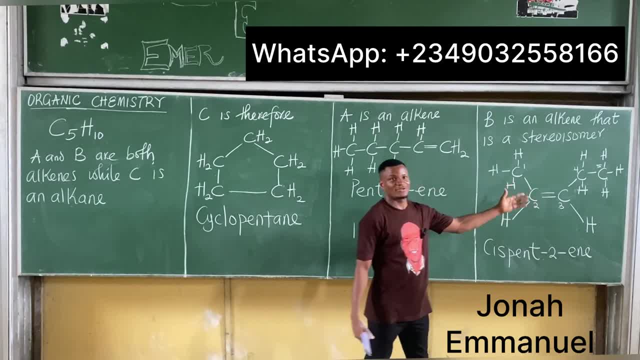 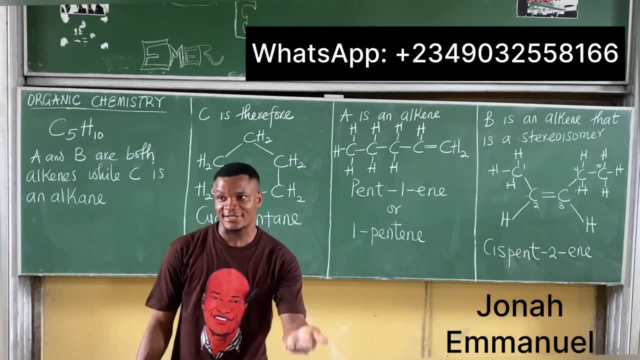 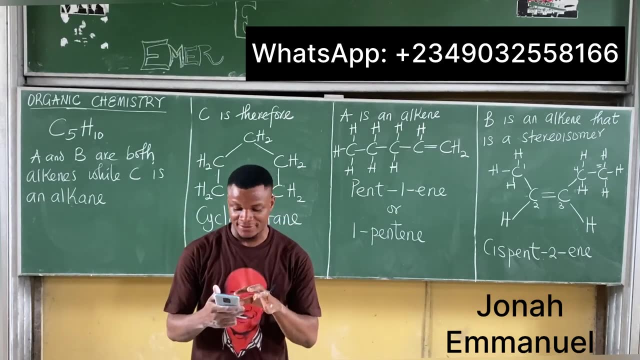 and hence b becomes a cis structure. so that's how it arrives in b. now, since b is a stereo isomal, then it is either a cis or a trans structure. so hence you have that's just like um, a very simple of putting your answer, all right. so that's that for that. let's proceed, all right. 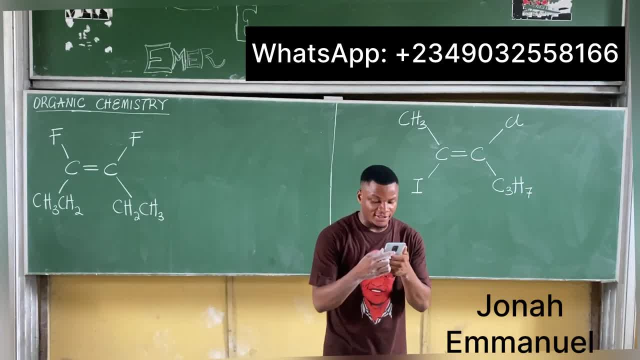 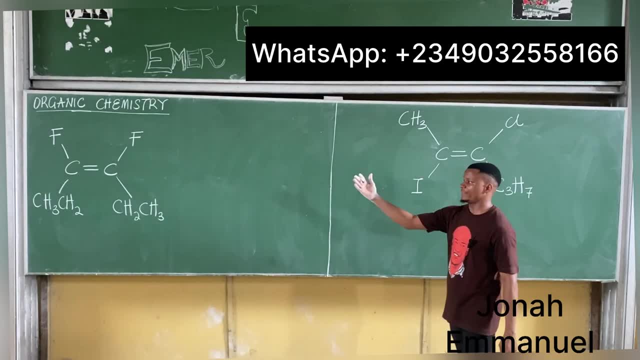 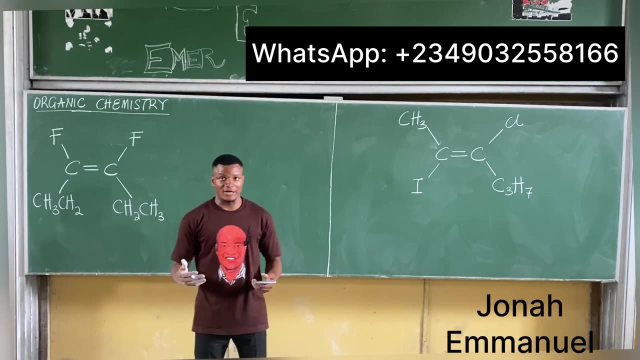 so here's another class question here. this one says: give the names of the geometric isomers below. give the names of the geometric isomers. so you have this and this. let's name this. how do you name this first? first things first, do your numbering. now listen, use your eyes, see that. 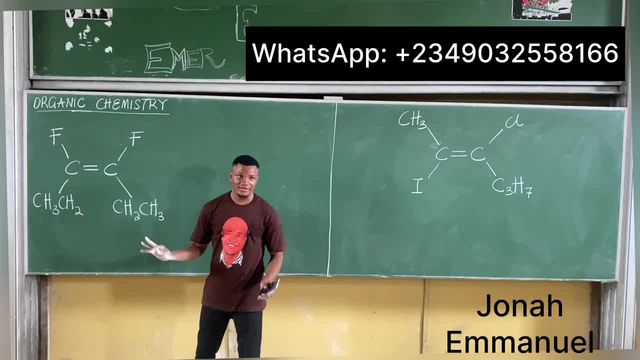 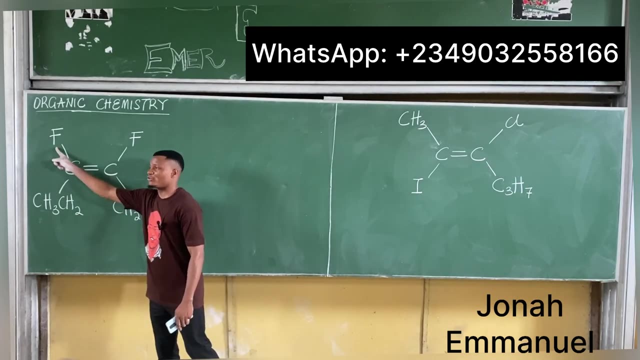 if i choose to number from here or from here, the same thing. so that means this one here is not a deciding factor. i'll now switch over to my substituent. observe that the substituents are both what they're: chlorine and fluorine. what does it mean? 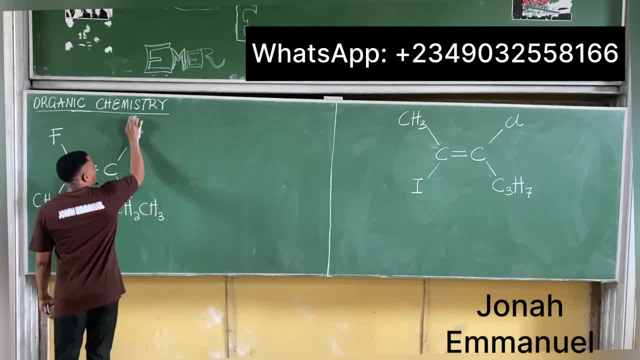 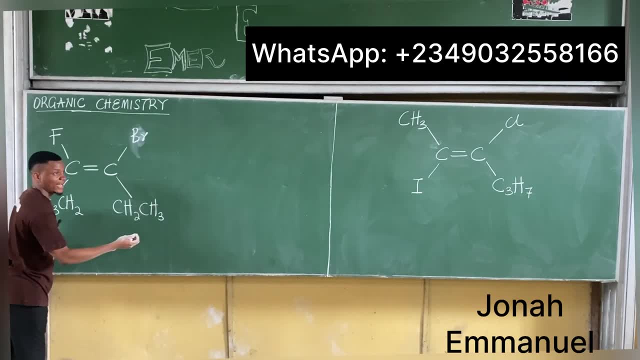 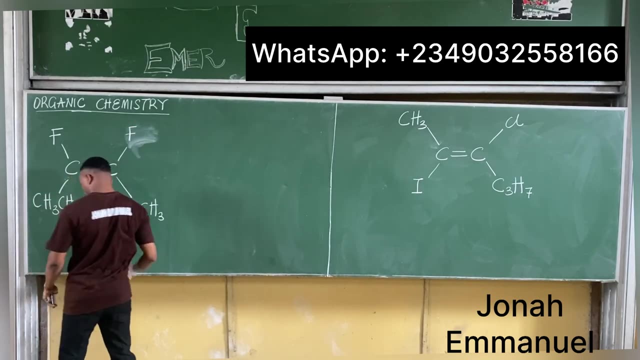 start from anywhere. in other words, if this man was a bromine now, i would have to start on this part here. why, from alphabetical order, is b before f, that's, by the way. so from here i'm having um, chlorine, chlorine, let's name this please. i said number from anywhere. if i count this way, it becomes: 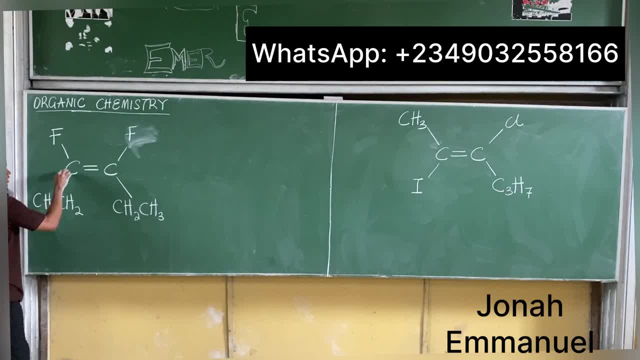 please. in total, how many carbon there? 1, 2, 3, 4, 5, 6, 6. is what there next? number two: look at this. i have a double bond, so it becomes one there and r king. number three: here is a geometric isomers. 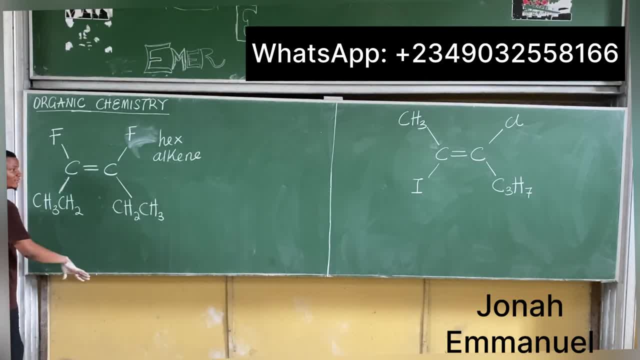 this structure here. is it a SIS or a TRANS? he says SIS, since these two are on the same thing, like this: so the sig. so so they become sis and sis next up. let's do that in two, because these two are on the same thing, like this: so this is to become cis and cis next up, let's. bring this Sob. is it a SIS? is it is a trans? these are proclaimed trans or trans trans, trans B that times combined articulation frequencies disease. the next try to indicate is this word is: you can add performers. you can take my cap中共 at this time and fill in some. prove you. 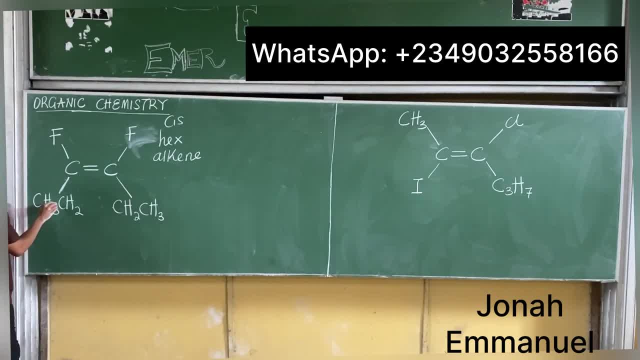 What I'll you, you will find out theuce, so I'm going to copy at that point. so today, Next up, let's do number please: 1, 2, 3, 4, 5, 6. It means the 2 fluorine. I'll cover what there: 3 and 4.. So what's the number of this compound there? No, No. 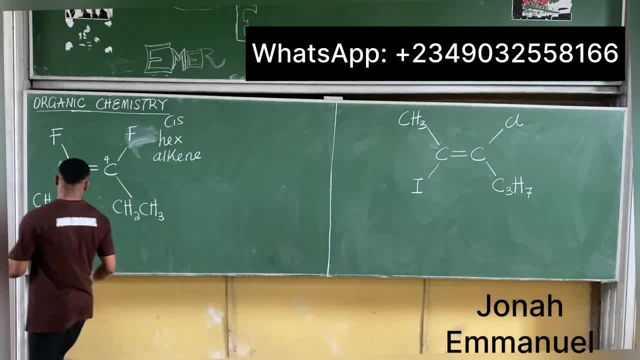 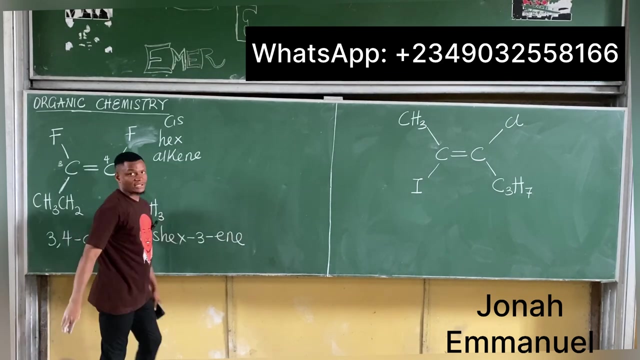 So substitute, and first 3, 4.. Yes, that's true. So 3, 4, di-fluoro cis, not 6-hexane, 6-hex, what there? H3-ane, Please, careful, Careful please. 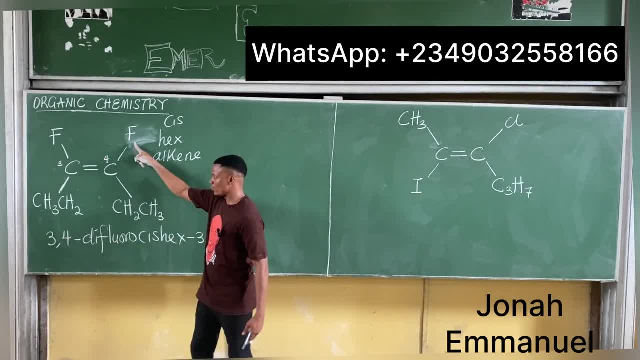 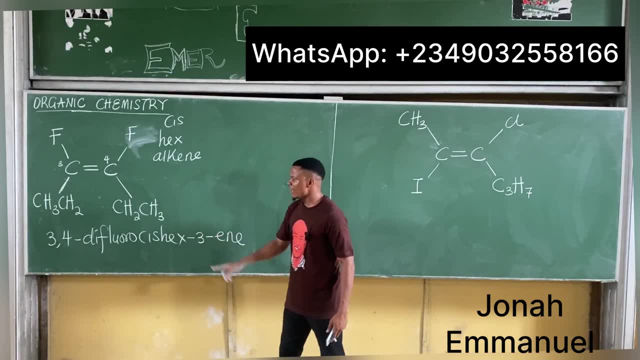 3, 4.. 2, di-fluoro. So it's always a substituent before parents now. So okay, so assuming you had mentioned 6, where would I put fluoro? So imagine that you're now saying cis-fluoro, Cis-fluoro No. 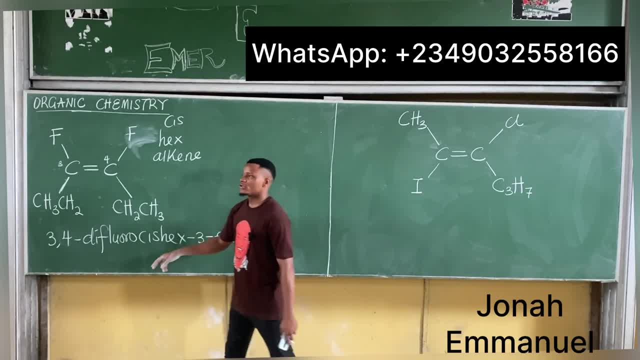 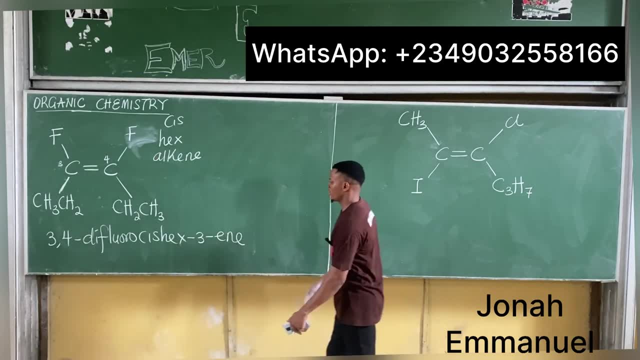 So I'm having this, please. Alright. so, cis-hex, You also have to show the carbon-bearing double bond. It's carbon-3 that bears double bond. So 6, 3-ane. Alright, this one here. let's get this done. 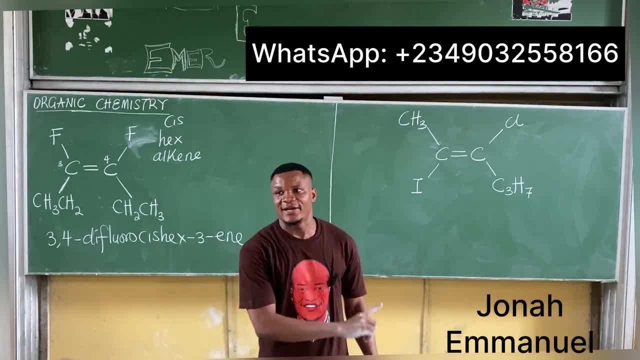 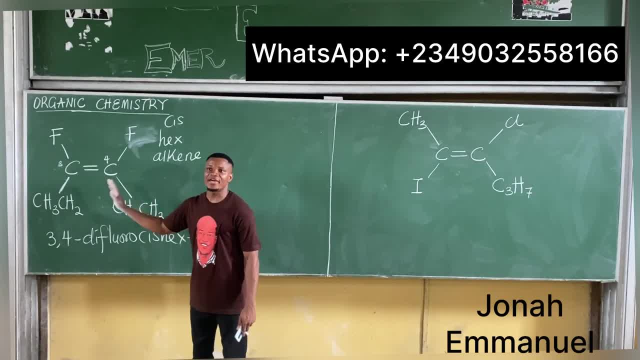 Subtituent, Subtituent, Listen, Listen In this one here. the reason why I started from any side was because 2 of them gives you what there? The same numbering. I will number 1,, 2, 3 before double bond. From here I'll have 1,, 2, 3 before double bond. 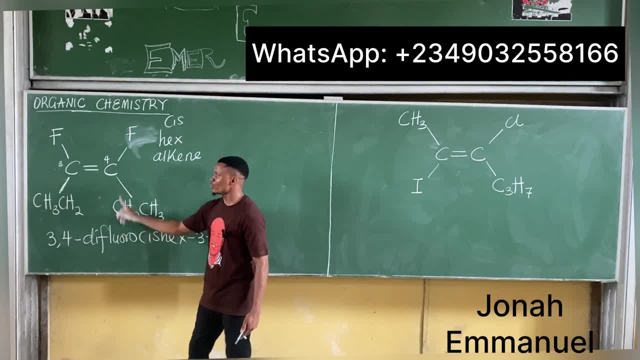 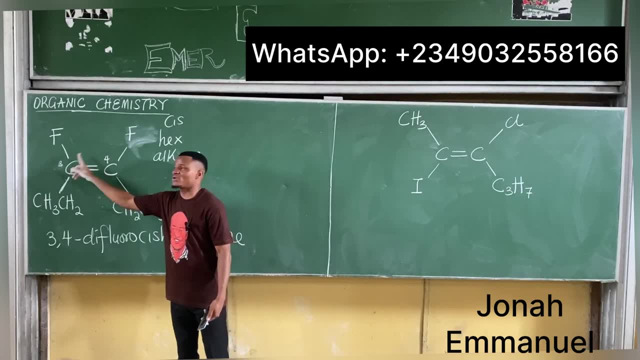 Subtituent, Subtituent, Subtituent, Subtituent, Subtituent. I have double- Rapid double bond. That's why I had to switch my focus toward there. Subtituent, But somehow substituent was still the same thing, So I did my stuff. In this case, your focus is always in double bond. first, 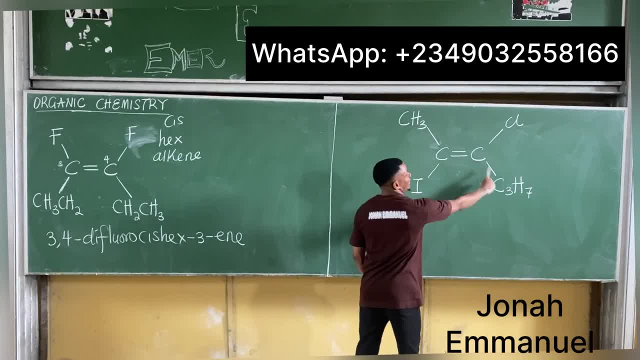 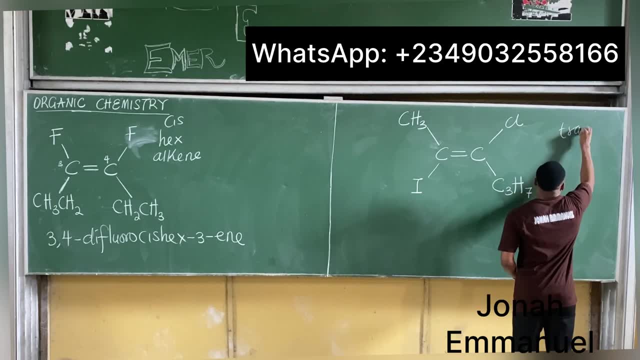 If I move from, of course I'm going this way here, this stuff here, Is it a cis or a trans Trans? So the first thing there is trans. That's the first thing. Number 2, how many carbon in total? 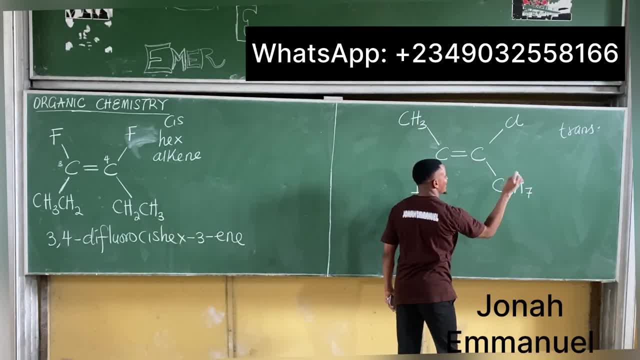 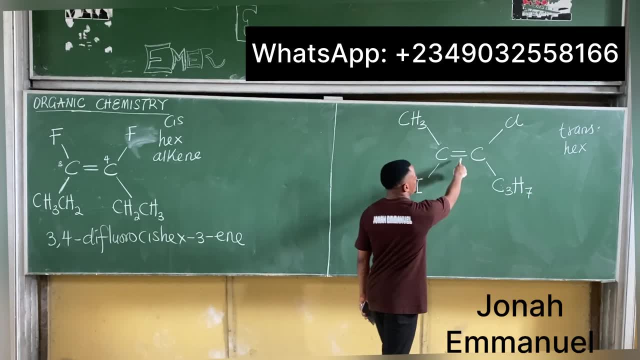 One, two, three, four, five, six. that gives you what there x. number three: functional group: your functional group is a double bond that becomes what there: alkyl. so how do you number this? observe that if i move from here this way and from here this way, they are not the same thing. so the question is this: which direction gives you? 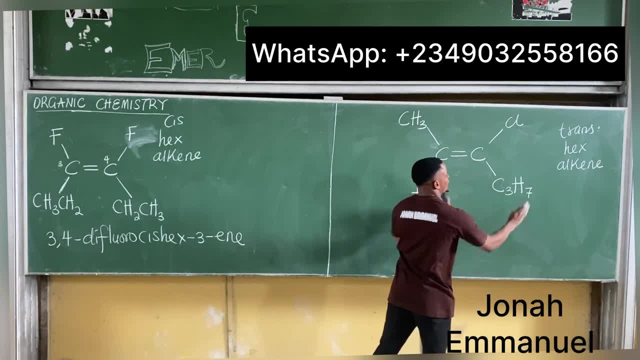 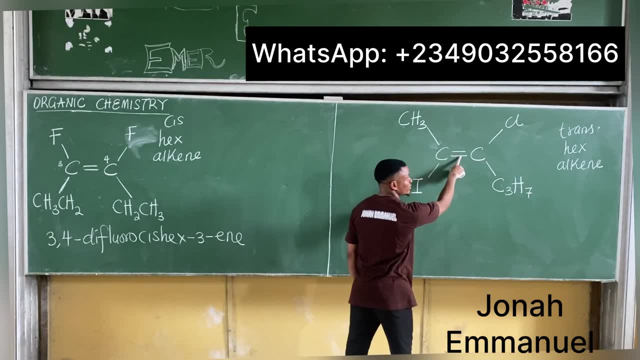 shortest possible distance to double bond. is it from left to right or from right to left? it's from left to right? from left to right, i have one, two, come on two beers double bond. from right, i have one, two, three and then four. so between two and four, the simplest one. that's what. 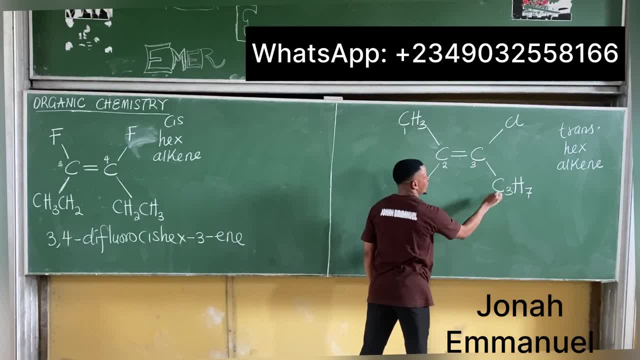 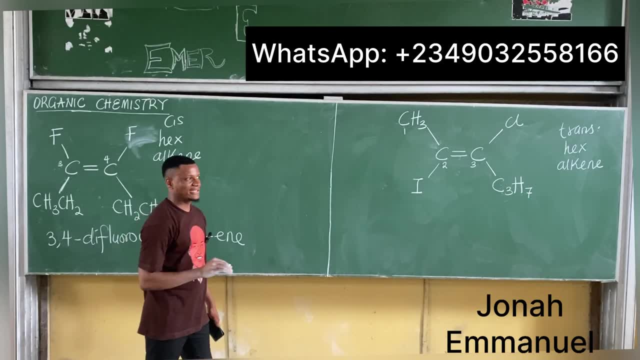 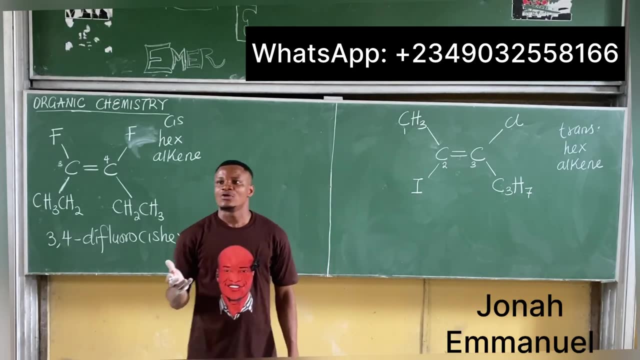 two. so one, two, three, four, five, six. all right, with that, one done. first things first, pick out your substituents. my substituents are what there- chlorine and water iodine- we said for a case like this, we consider what there, Alphabetical order: 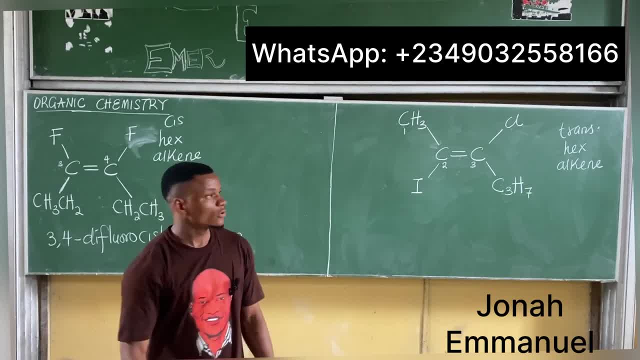 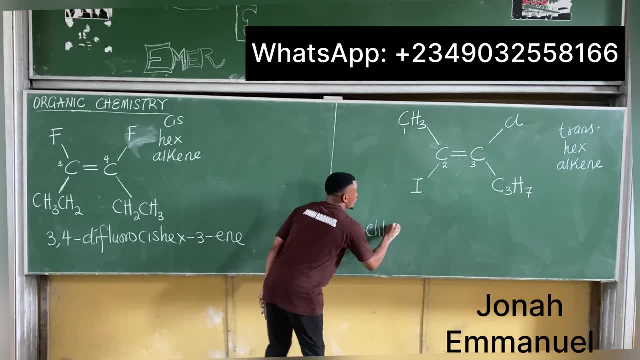 Between chlorine and iodine, which one comes first, Chlorine? Chlorine is attached to what number there? So it becomes what there? 3-chloro- 2-iodo- what do you say in cis Trans? 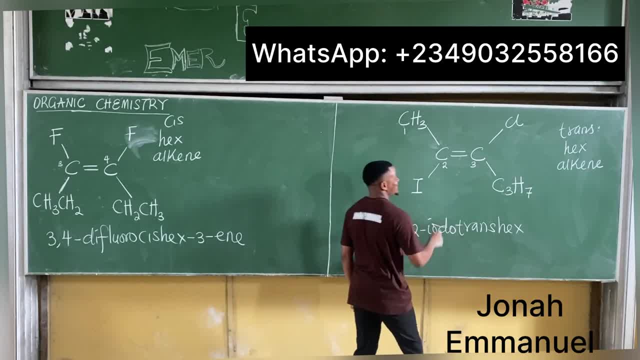 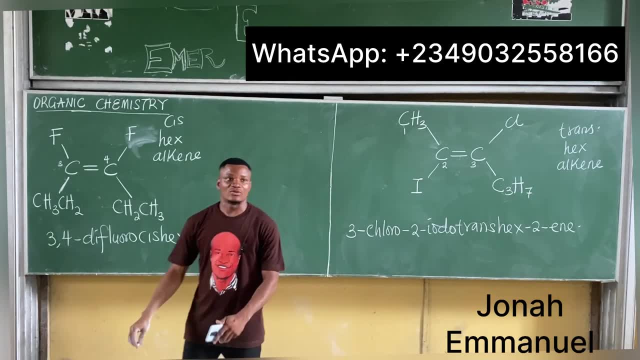 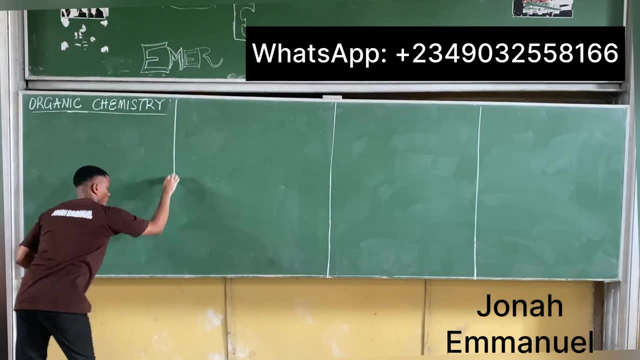 Trans, what there? 3-hex-2-e, Trans-hex-2-e, So that's it. I'm trying to name as many as I can and not skip some stuff, So I'm having this. Let's look at something about. 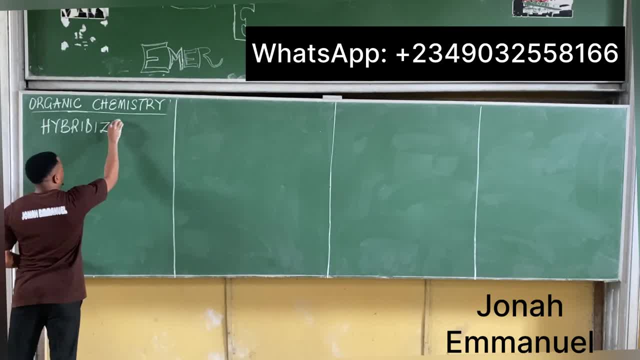 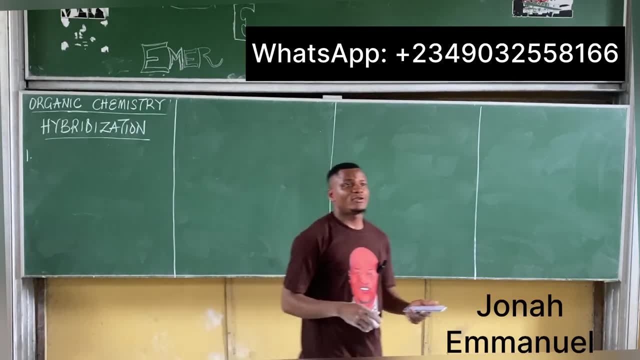 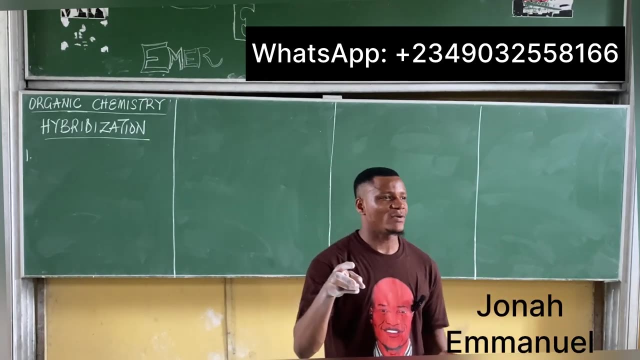 hybridization, Hybridization. Now listen, Listen. We've done this math before. in our previous class We discussed three types Abhi: SP, SP squared, SP cubed. SP is for which of them, SP is for which of them. 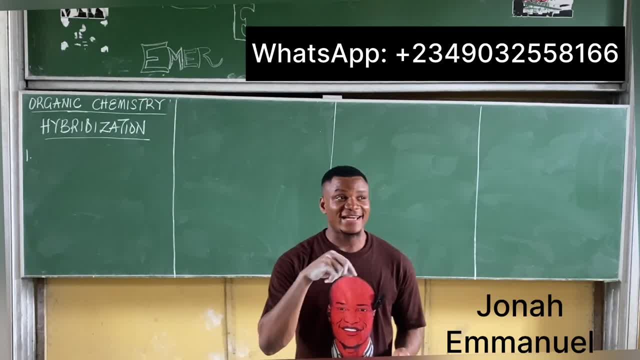 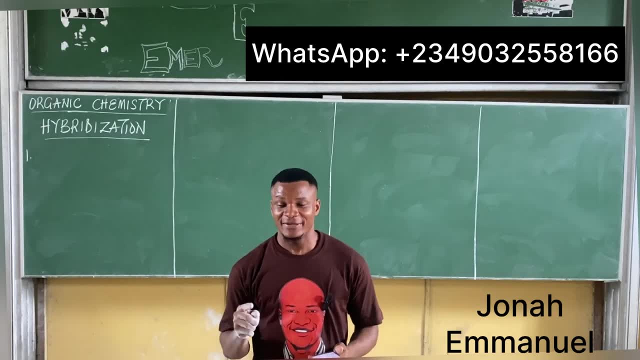 Alkyne Abhi alkane. SP is for alkane. SP squared is for what there Alkane SP cubed is for what there Alkane. Apart from these three, there are still other ones I want to show you today. 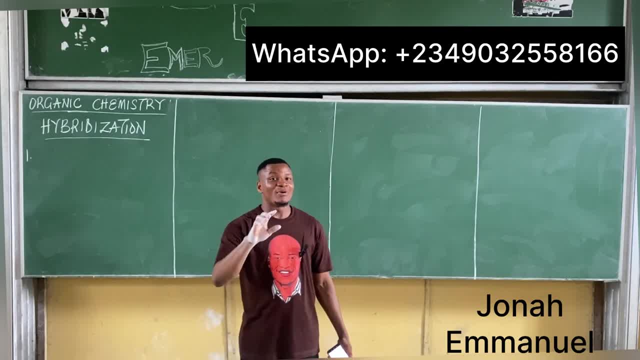 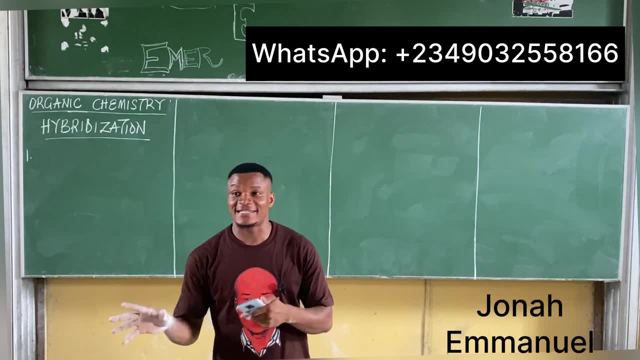 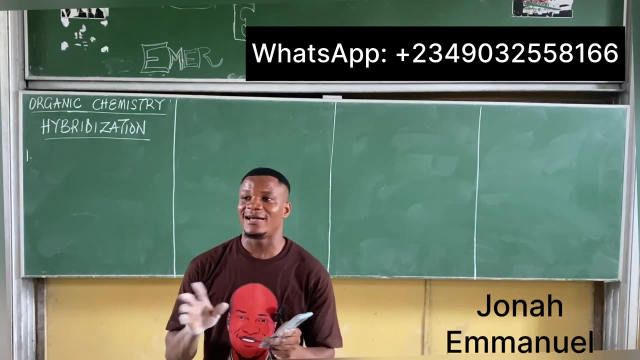 But before then, so we know those three, let me show you about two new ones today. There's an S, there's a P, which we've not done, but I think they passed through before, so let me bring it up now, But before then. so I'm not going to define what this means. You already have. 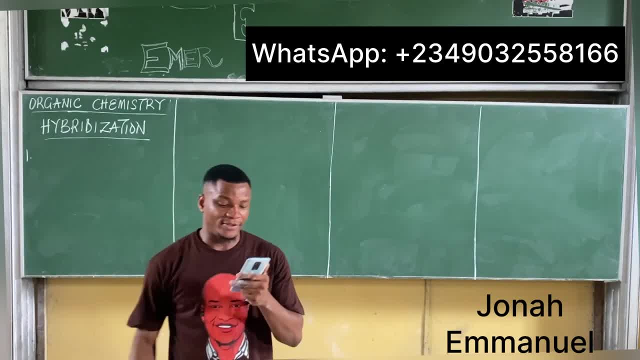 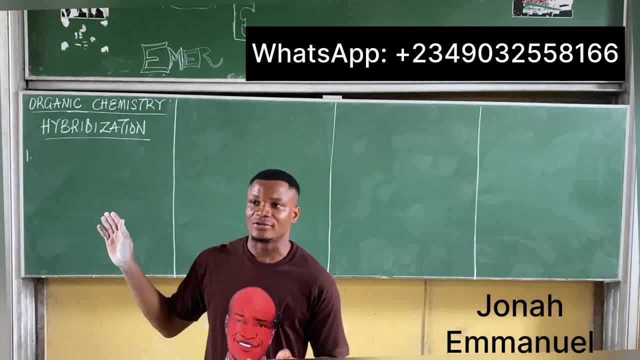 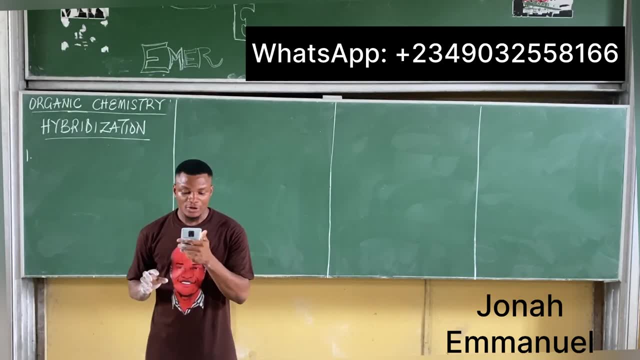 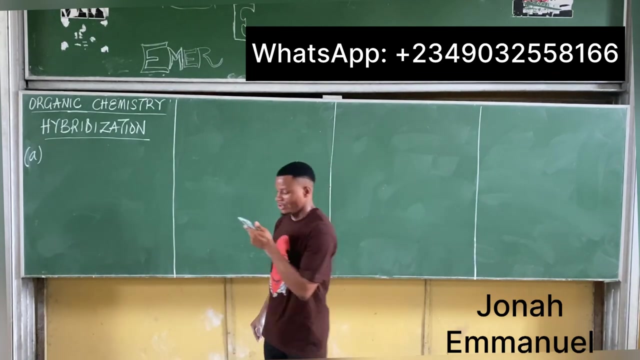 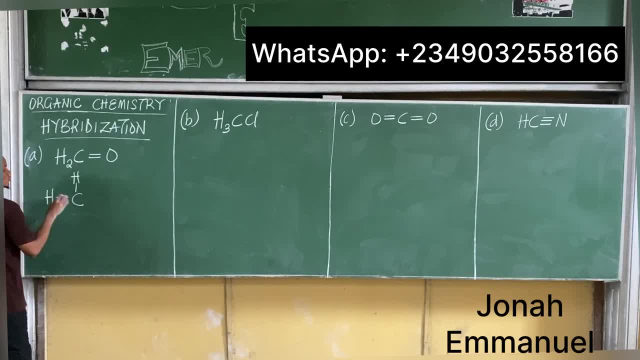 um, h, h, ch2, double bonded to o. all right, first things first. what is the hybridization pattern? is it sp, sp squared, sp, cube, sp, whatever? what do you have there? so i'm having a double bond, because what that sp squared hybridized? what is the geometry? 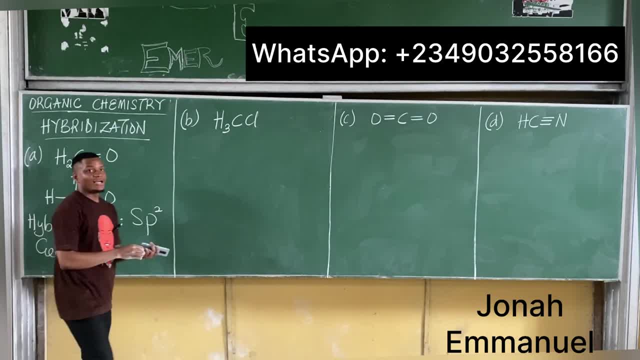 um for geometry. here's how i get the geometry clean. it is three-sided, it's called a trigonal. that's all by three-sided i mean. that's why i said: draw it in full. if i draw this in full, i can now see this. look at this. now i'm having here, here, here, here here, straight line here. 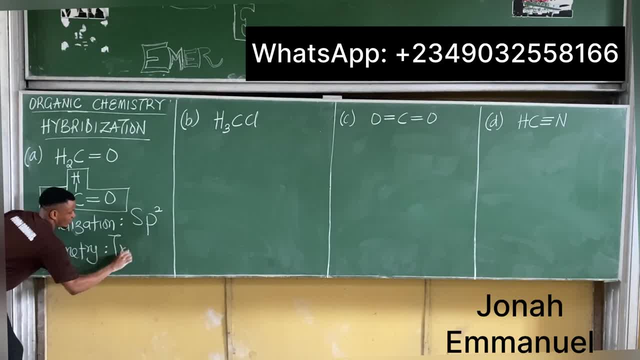 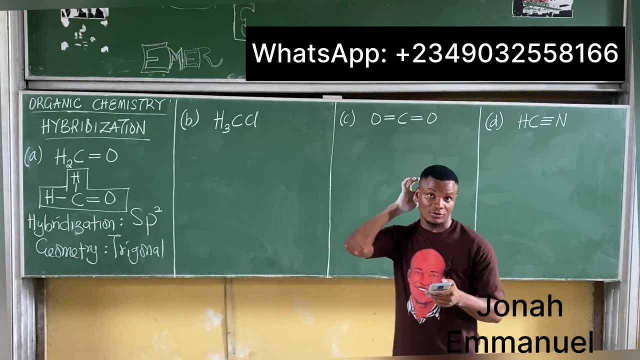 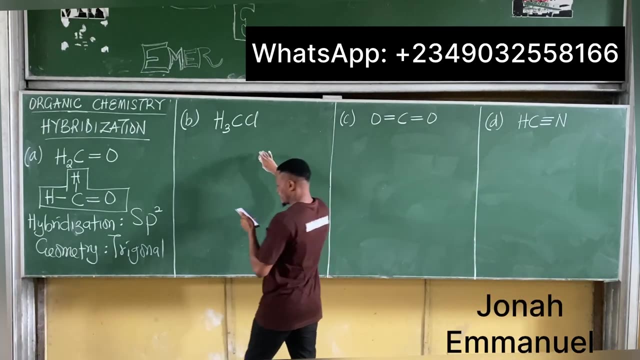 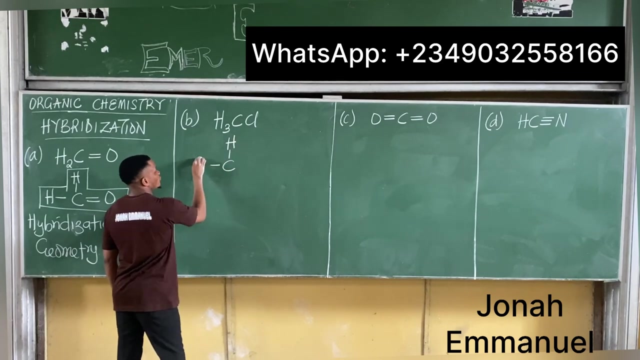 here. so observe the three pattern. it's called a trigonal and how geometry is a trigonal structure. that's how you get the geometry. so draw it out and you'll see what it looks like. let's get this one done. so first things first draw the structure c three: hydrogen one, two. 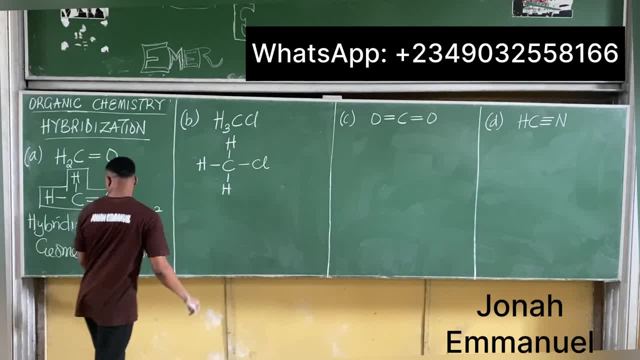 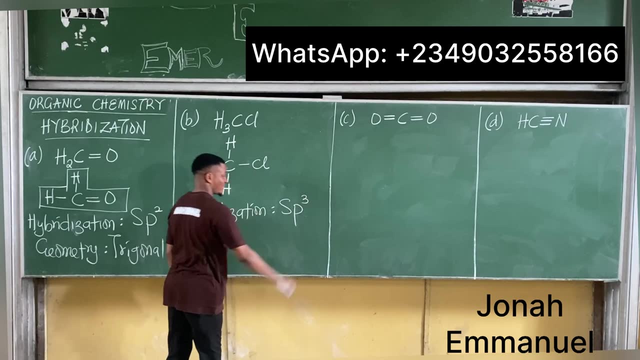 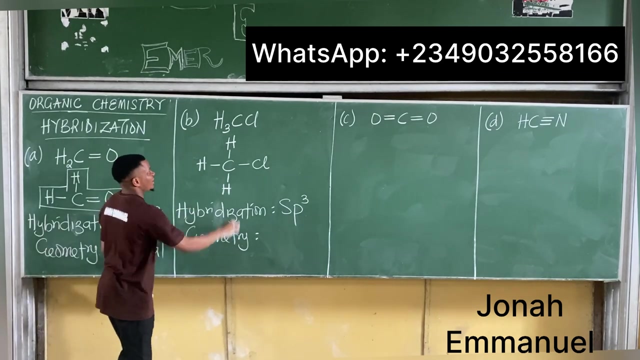 three, and then chlorine. i have c? l. let's get hybridization for hybridization, because what do you have here? sp cube, please not here. what's the geometry? if i look at this, this is now one, two, this, this, this. this looks like a cross. all right, so it's four. four is called tetrahedral, called tetrahedral. 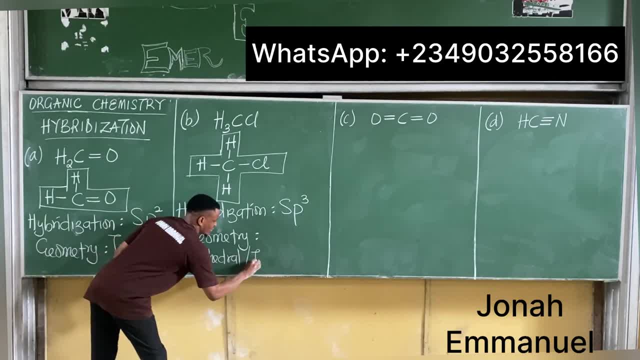 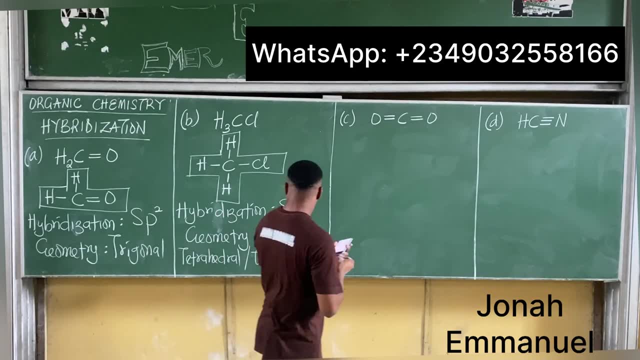 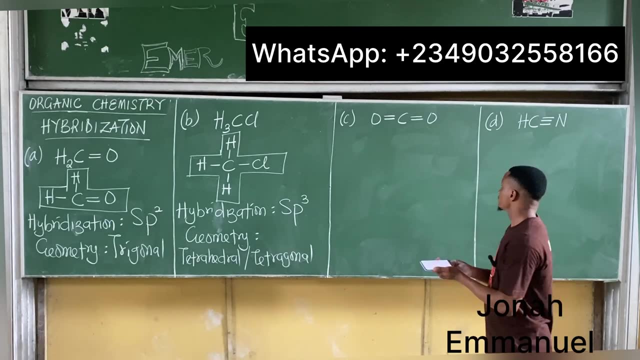 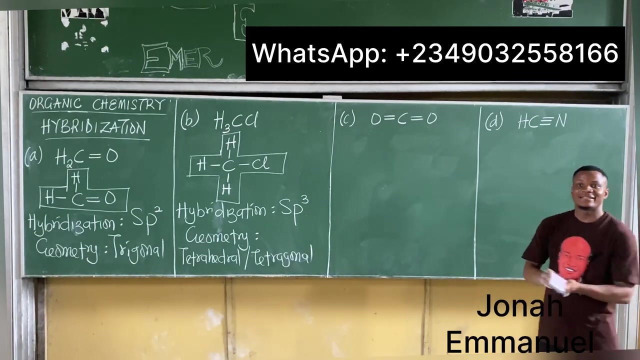 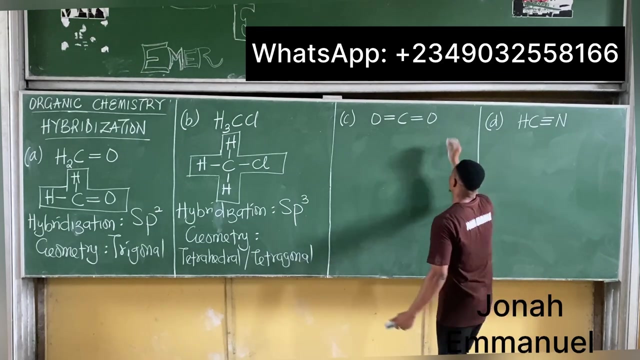 slash four, a tetragonal. so tetra four, tetragonal. for this one i don't have to start drawing structure again now, listen. um, for this one they were kind enough to give us co2, because usually they'll give you the molecular formula as well. there, co2. 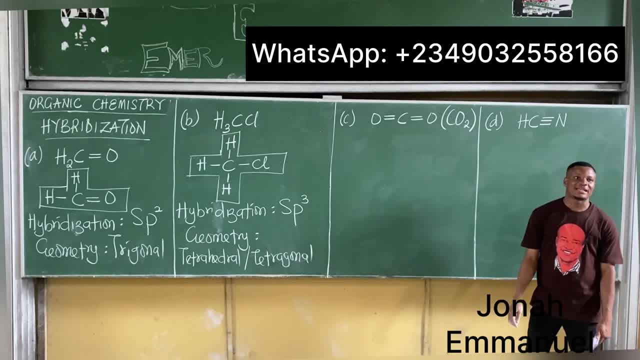 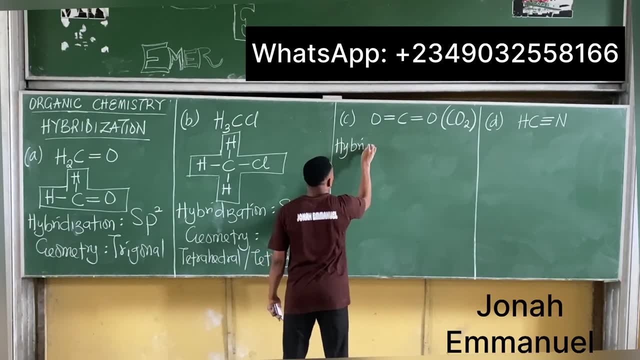 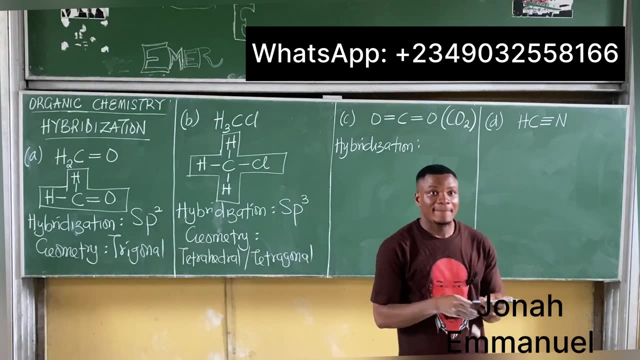 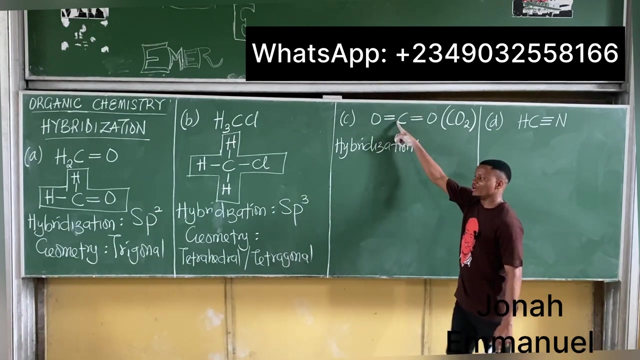 is now left for you to be able to draw the structure, but then again, they are nice enough to give us structure. so, for a case like this, what is the? what is the hybridization pattern? please listen, oh listen, listen. normally it's a double bond, and for double bond we expect an. 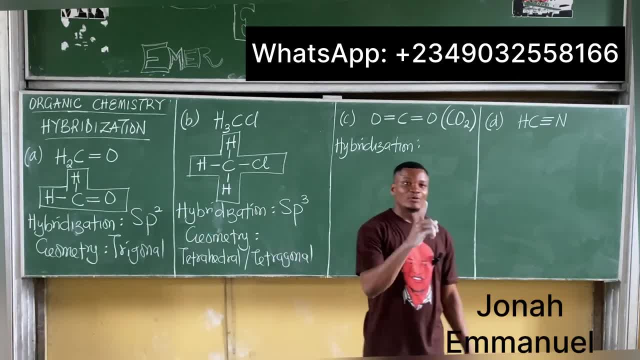 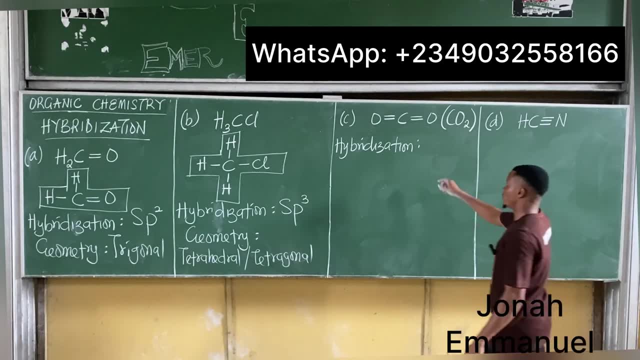 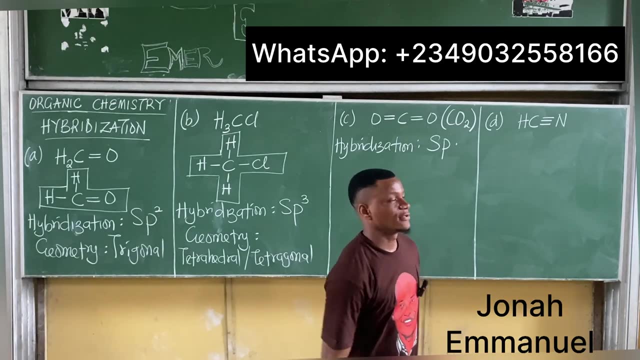 xp squared hybridization. but when the double bond is now double, as in the case of a dying- because we're there and sp, so please take note, please. when it's now double, it becomes no longer sp squared but sp hybridized. so please take notes. that's like a small difference. let's get out the geometry. 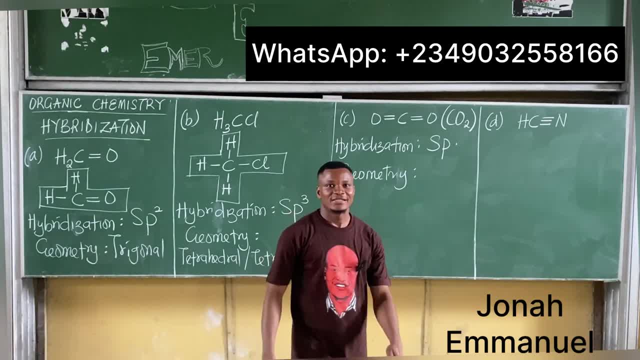 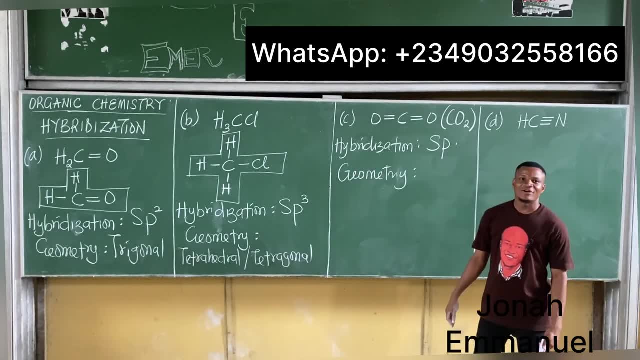 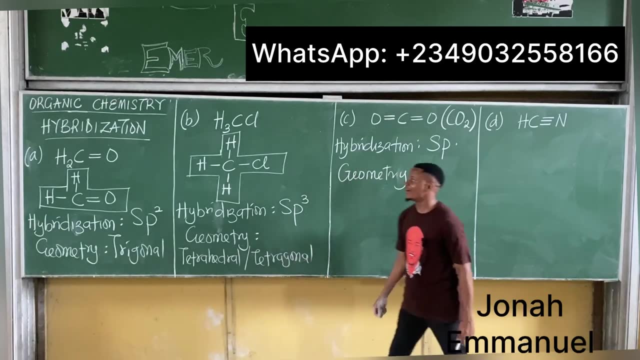 let's get our geometry for this. what do you think this will be? that's a linear structure. uh, should i go now? tetra or tetragonal? what will it be? see pattern now. see pattern three. try, go now four. tetra. go now two. only that, because we're there. 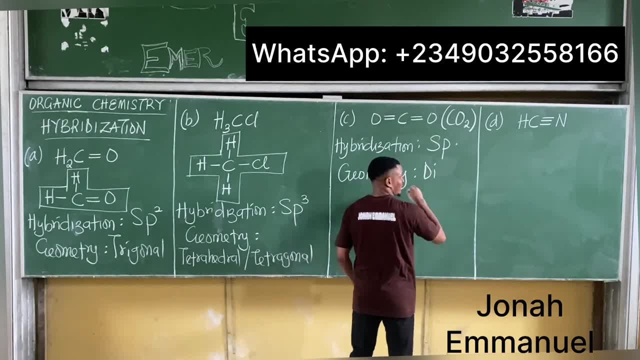 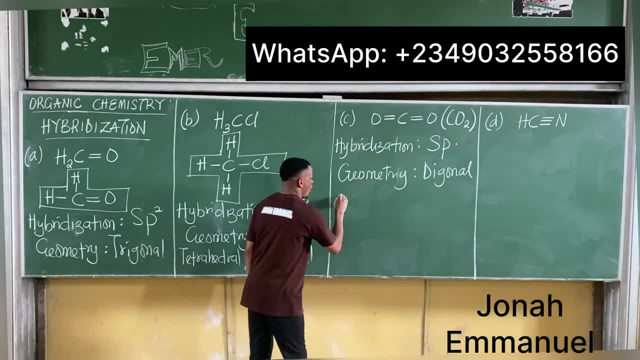 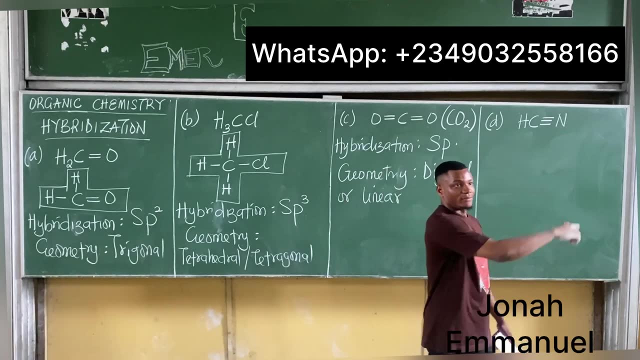 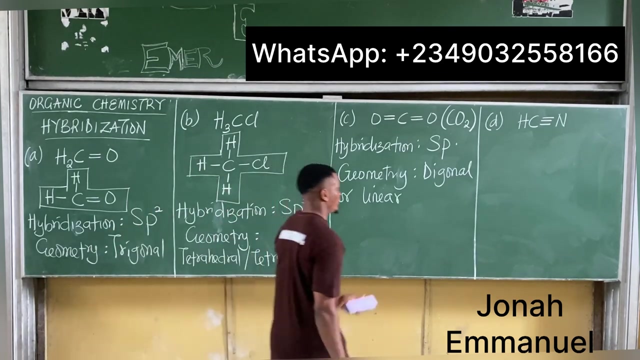 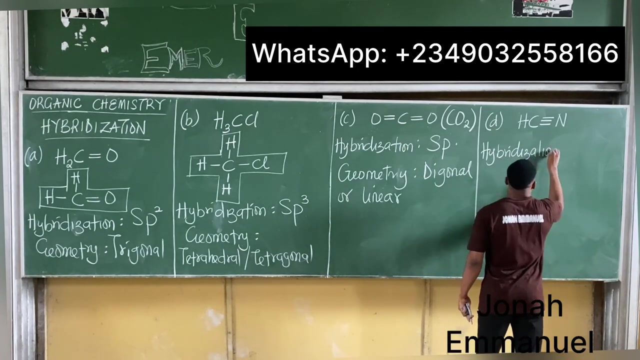 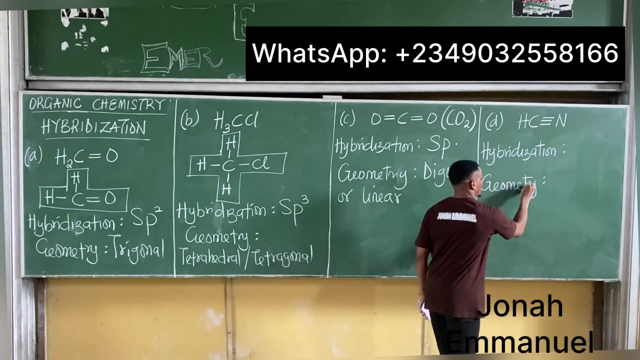 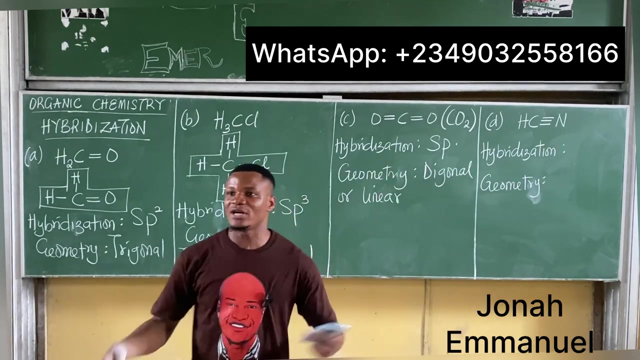 we're not gonna. it becomes a diagonal or diagonal. what that linear structure, please? for the fourth one, get out the hybridization as well as the geometry. for the fourth one: get out high breathe, die. they shun pattern as well as you, as well as geometry, please, fast, fast, fast, fast, fast. what do you have for the first one? 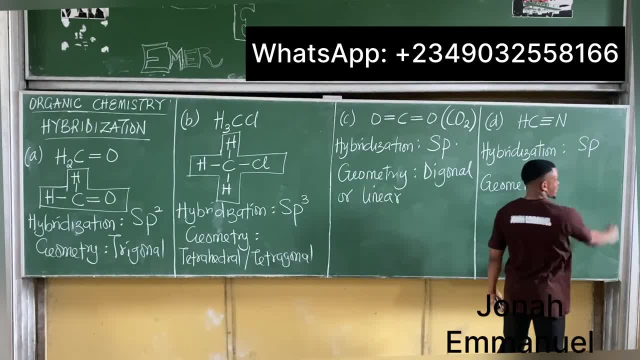 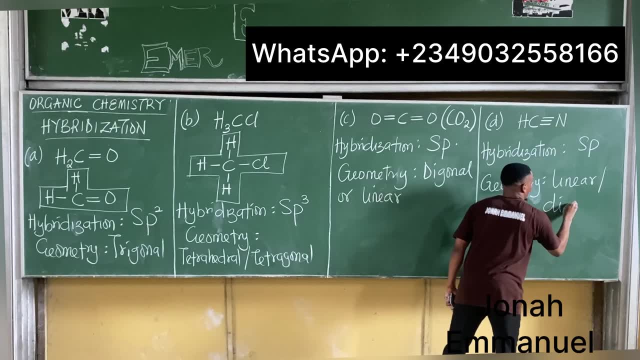 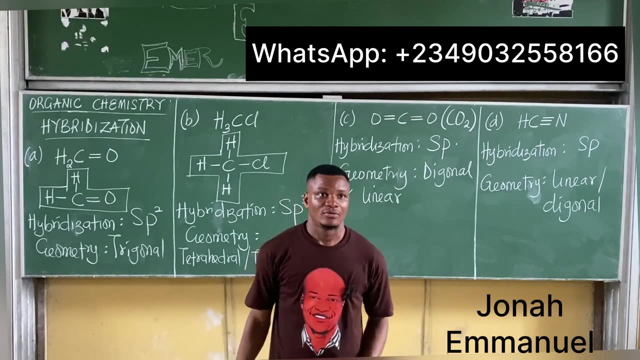 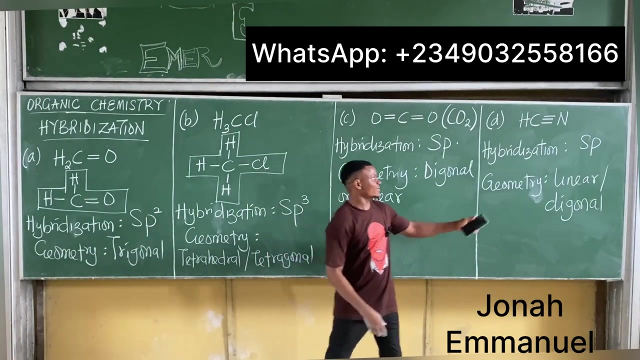 speed is triple bond, sp is triple bond sp. geometry linear or what there, please, it's not diagonal, is diagonal, not diagonal. you're not dividing two, two, all right, so that's how we get this man done. so, please, your. he was asking why this is sp, please. we've mentioned before. we said: 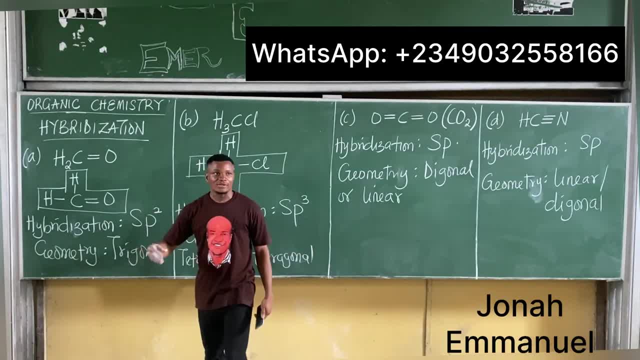 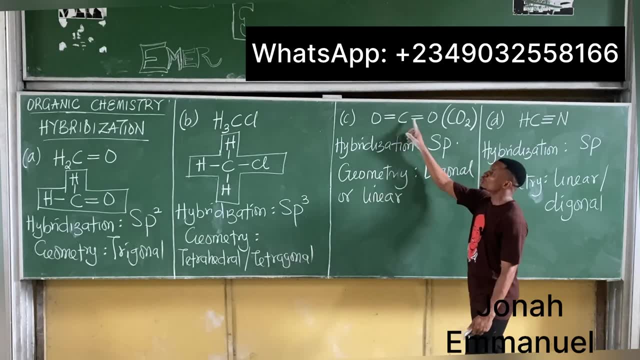 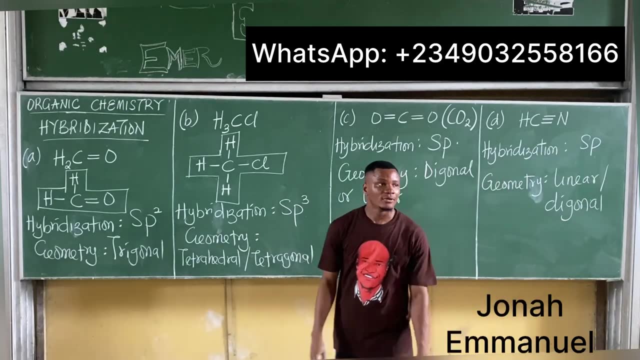 when it comes to double bond: for double bond, this is sp. hydration pattern- is sp. squared for single bond is sp. cube for a double double bond is sp. for a triple bond is sp. that's how it's done. yes, so far, so good. i've given you three. 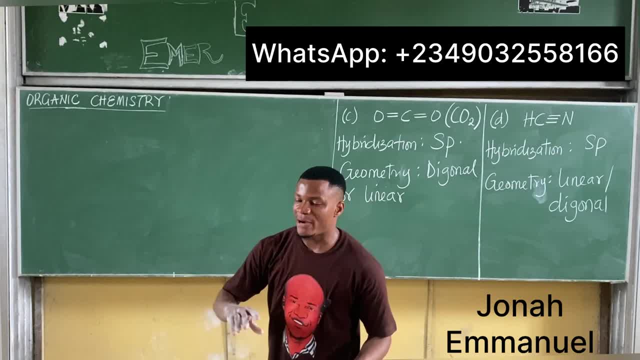 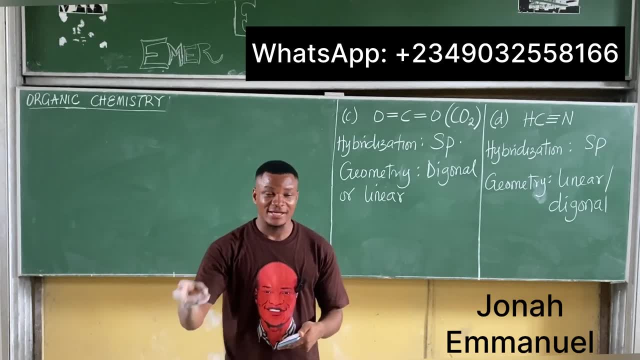 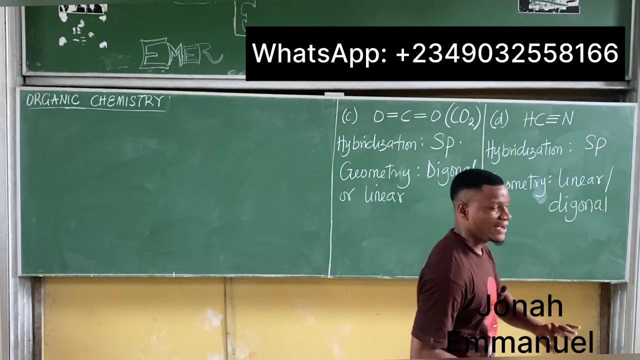 hydration pattern: sp, sp square, sp, cube. but apart from that one, there there's an s and there's a p, so now there's five. now s, sp squared sp, sorry, s, sp, sp squared sp, cube. and then p. take down. please take down, please aside the three major hybridization pattern in brackets: sp, comma, sp. 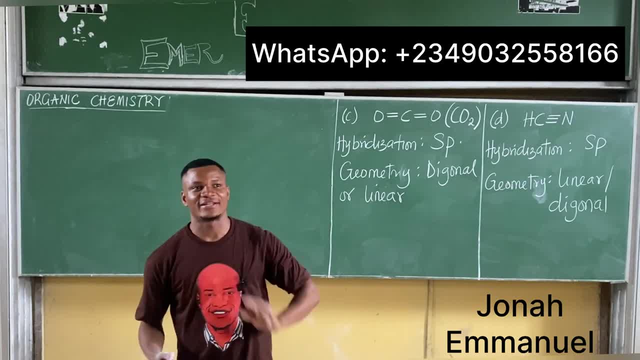 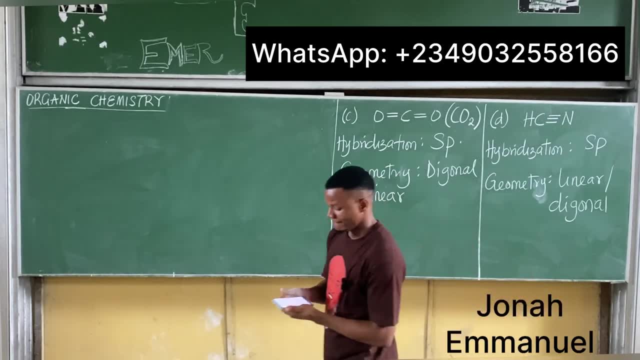 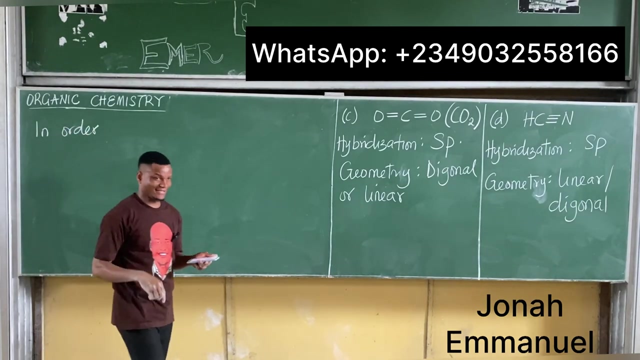 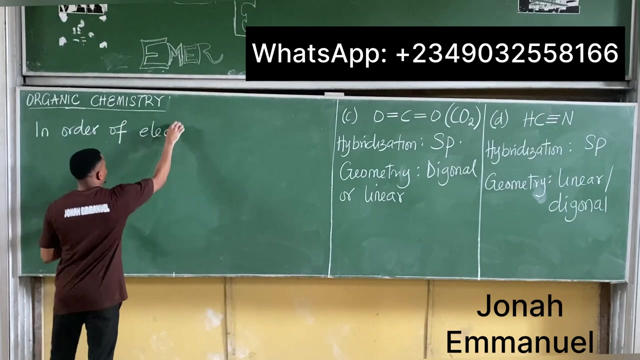 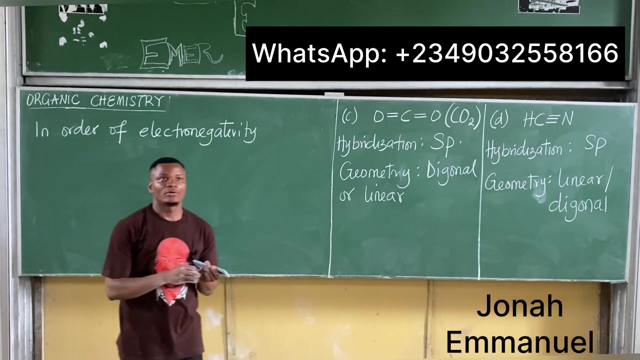 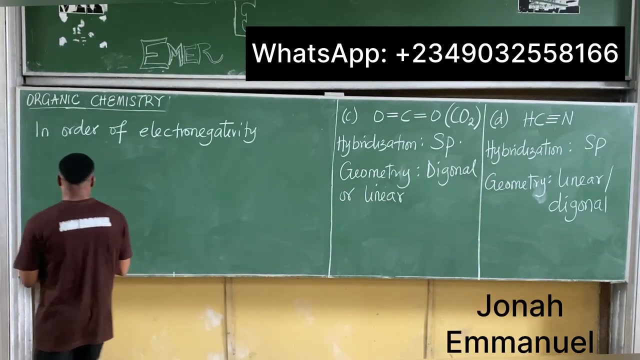 squared and sp cube. close the bracket. aside the three major hybridization pattern does um sp, sp squared, sp cube comma. there exists two other hybridization pattern. there exists two other hybridization pattern in brackets s and p. s and p. to stop in order of electronegativity. 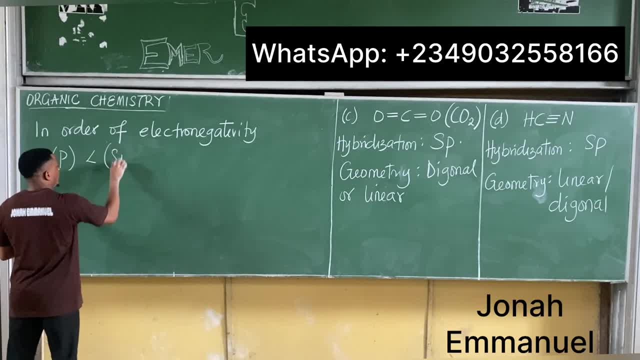 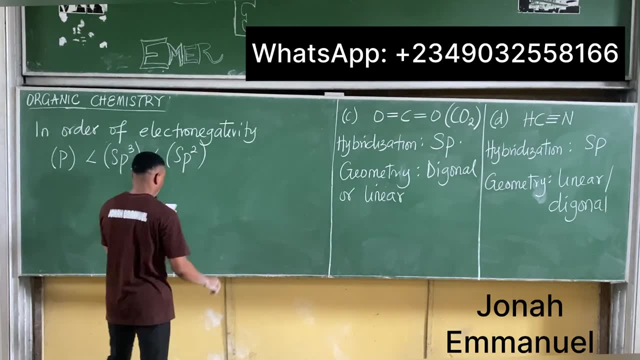 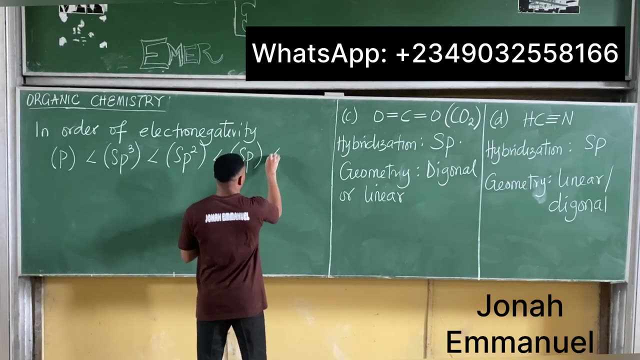 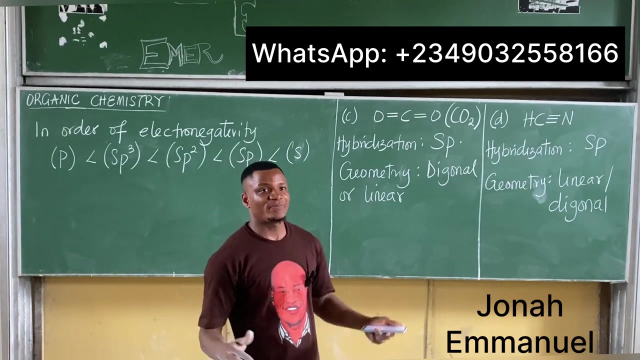 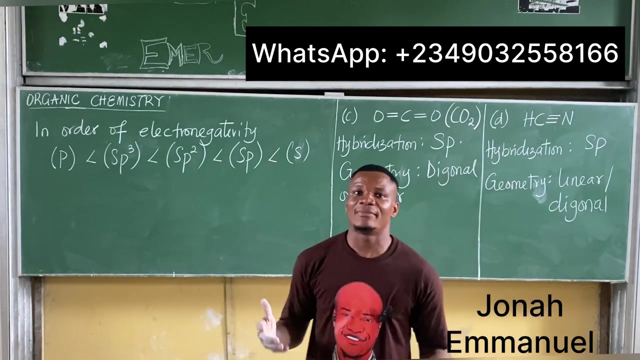 in order of electronegativity. in order of electronegativity, these diabetes patterns are arranged thus. so please copy this template. so i'm trying to say this in your year: one don't bother about trying to know what exactly s and p are. no, just notice thing. this is like this how they always access. 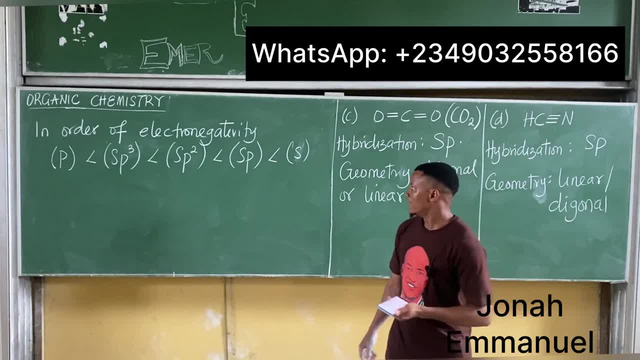 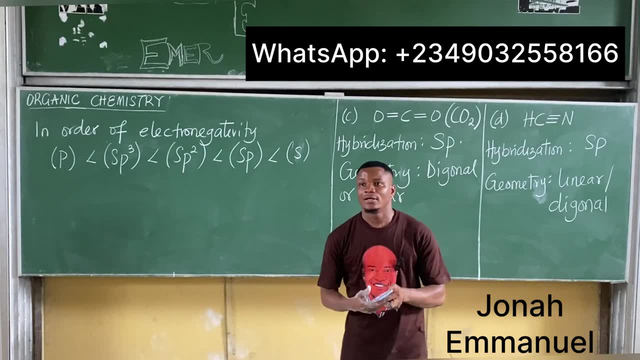 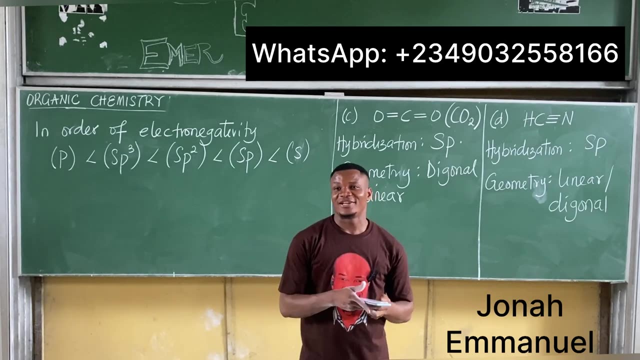 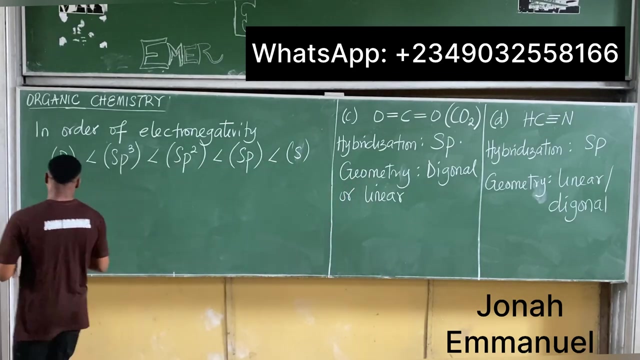 you see, arrange the following in order of electronegativity: so we're having this, it'll be increasing electronegativity. you have this all right. so that's like the new thing there. so now i'm telling you they are. they are five. but then i get to you two. now here they're no longer five, they're now seven, so perhaps you 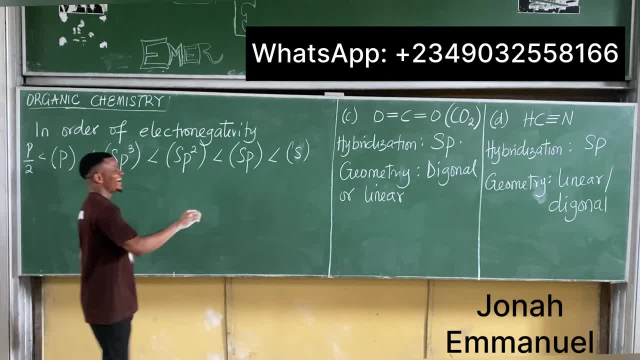 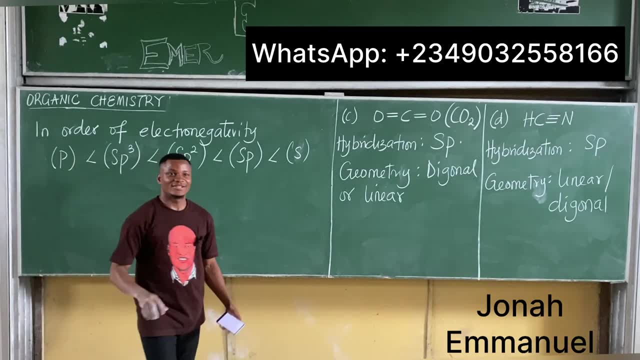 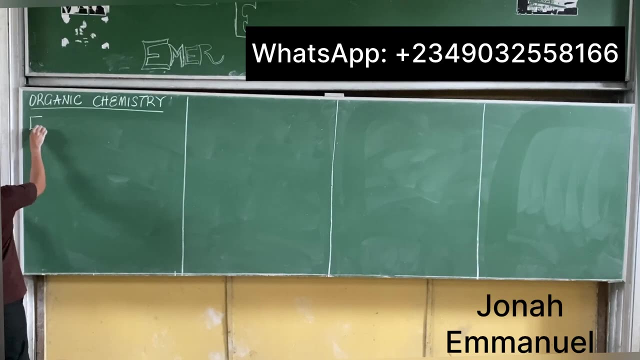 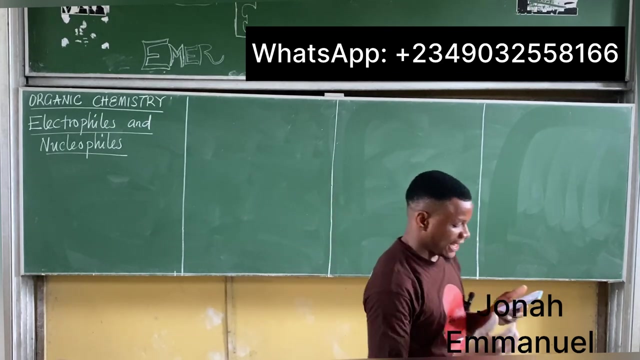 now have p over two. and then, because i'm kidding, though i'm kidding, the idea is just keep an open mind. you keep learning and learning, and learning. all right, next concept, please: electro files and nucleophiles. all right definition. i said, electrophiles are electron deficient species and can accept an. 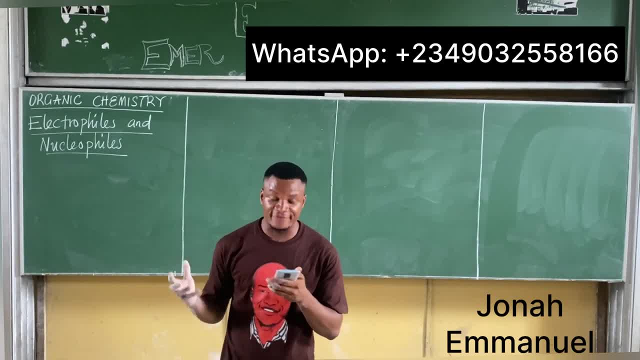 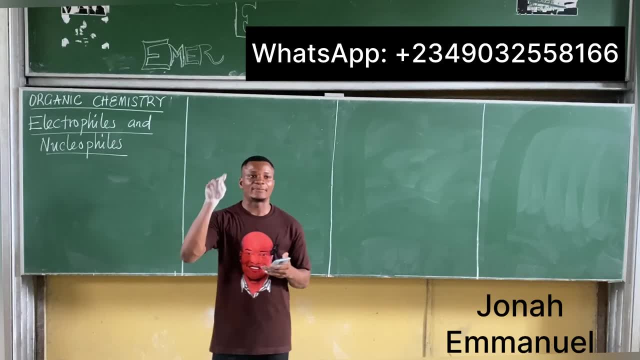 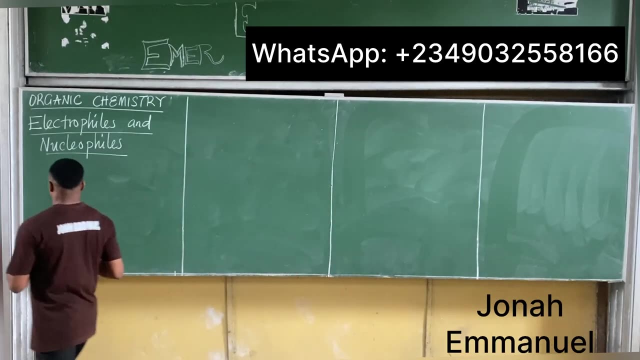 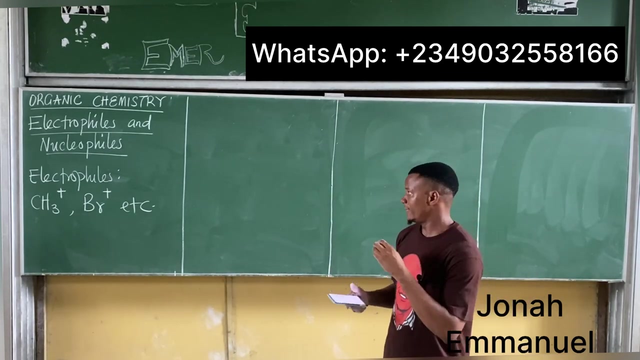 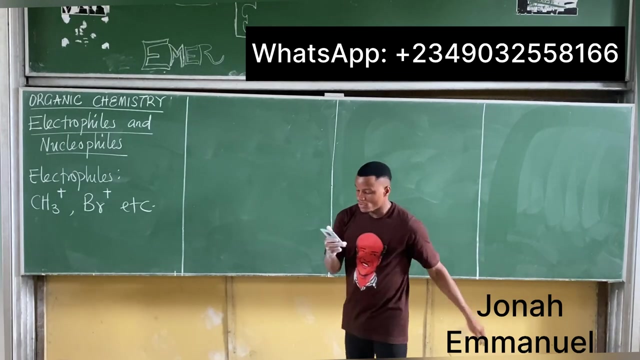 and can accept and can accept an electron pair from electron rich species full stop. they usually have a positive sign in bracket plus. they usually have a positive sign in bracket plus plus example, example, example. you have this. so electrophiles, electrons deficient plus so atc. while nucleophiles, while 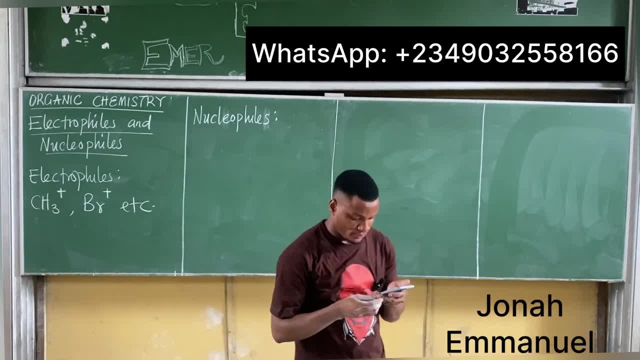 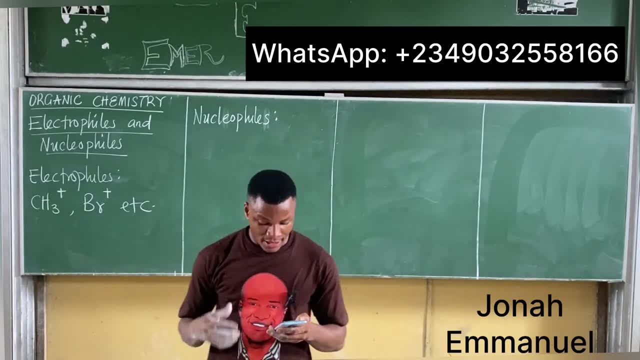 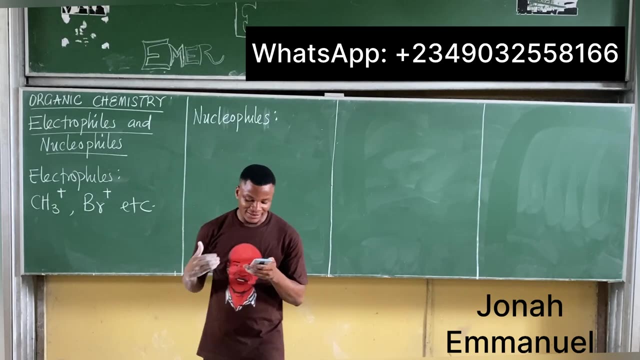 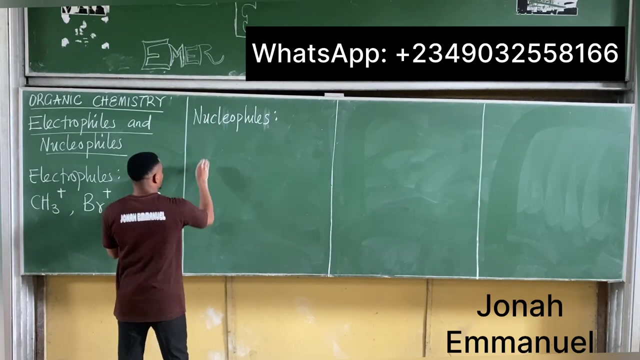 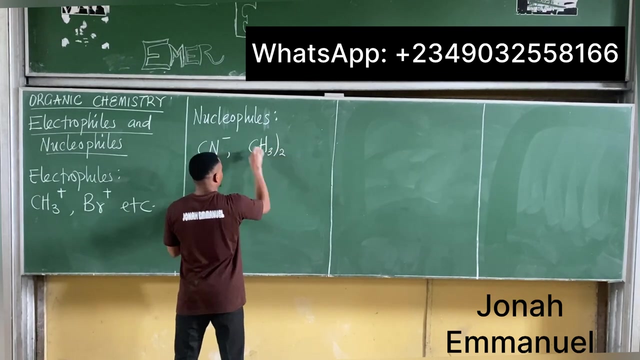 while nucleophiles are electron rich species, nucleophiles are electron rich species and they donate electron pairs and they donate electron pairs: electron pairs- p-a-i-r-s pairs to electron deficient species. to electron deficient species. p-a-i-r-s pairs to electron deficient species. to electron deficient species. to electron deficient species. 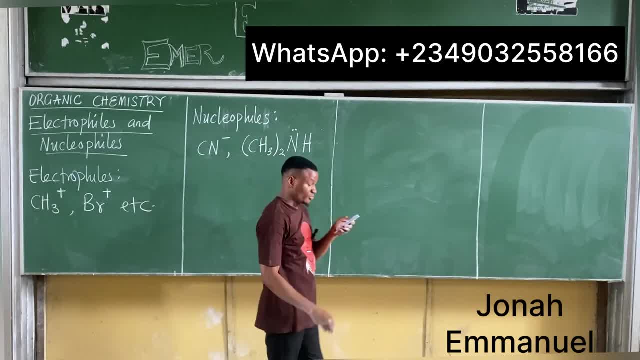 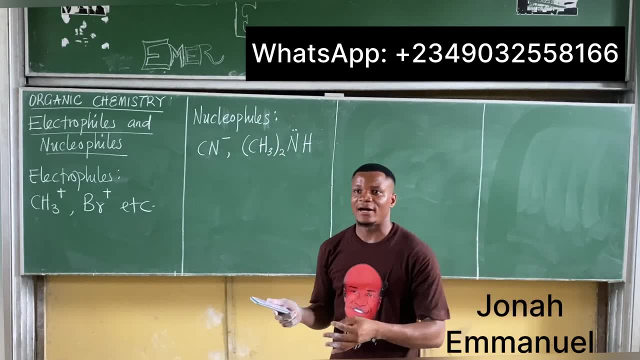 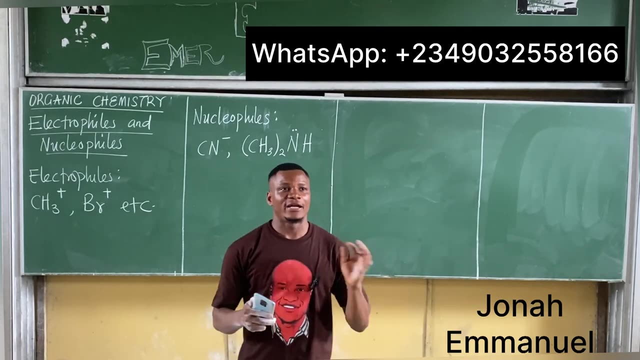 example. this is to see in your, in your test. what you should focus on is: how do you define electrophile, how do you define nucleophile? or they'll give you a subject. you said um, species which are electron deficient are called dash. the answer is: what there? electrophile? 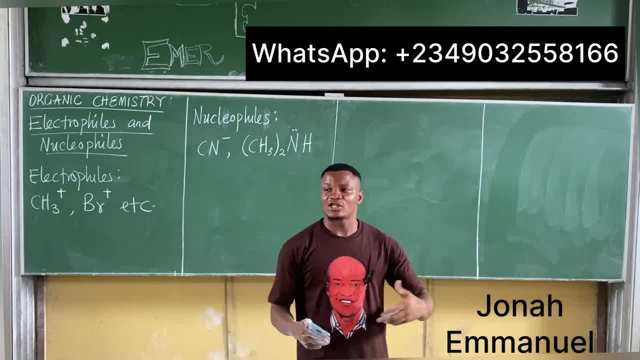 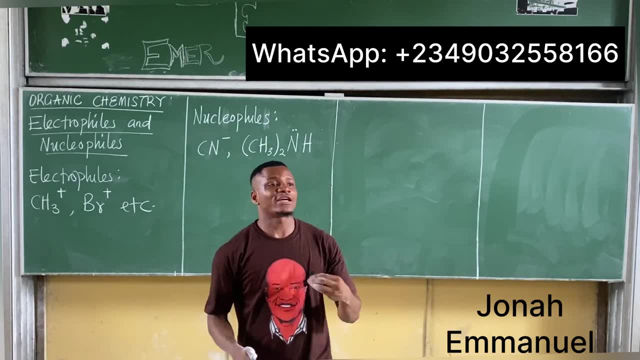 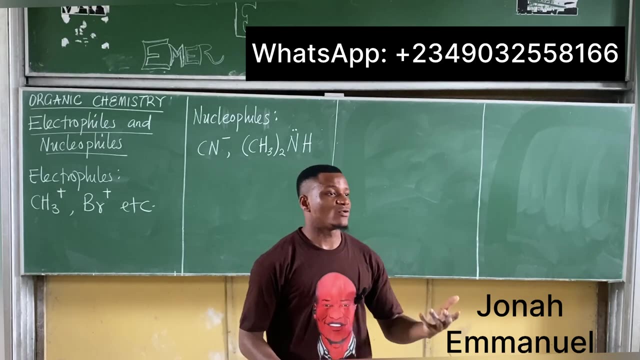 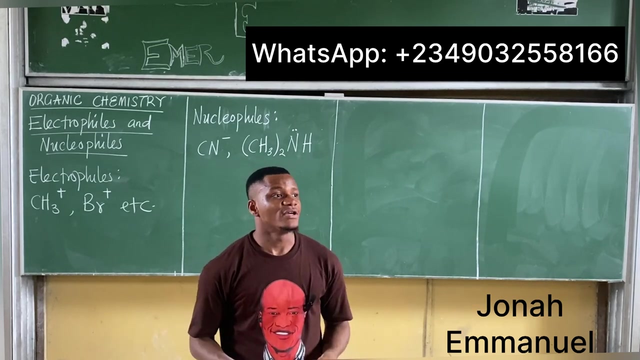 are called what there dash, that becomes what their nucleophiles. that's one pattern. an alternative tile is that to list out a number of ions, therefore number of ions. you see, classify the fullness weren't there. electrophiles are what they are: nucleophiles. it's very simple. if his 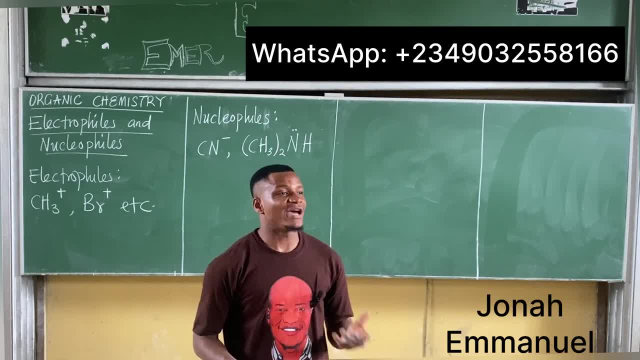 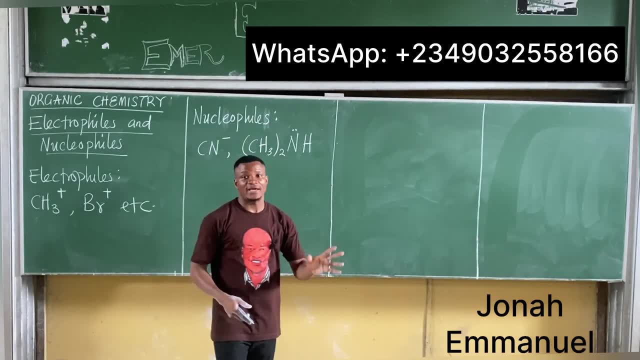 Lewis structure. if it's Lewis, what do I mean? it has what they're dots. so if it's Lewis, it becomes what there? nucleophile. so that's that's about what you be asked there. just note it right: positive electrophiles, negative nucleophiles, dot. 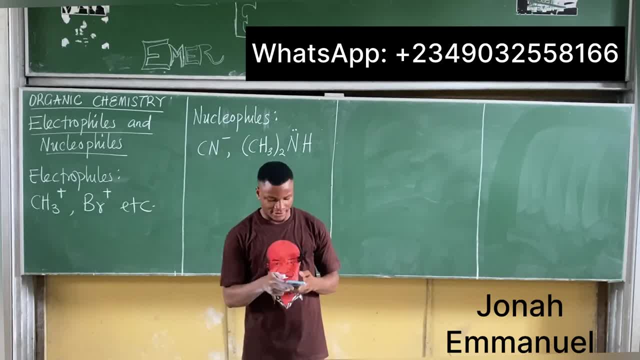 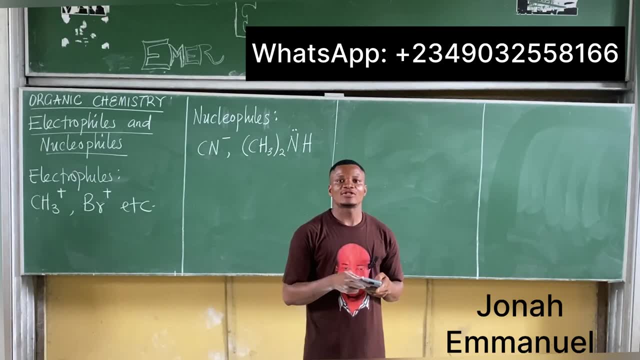 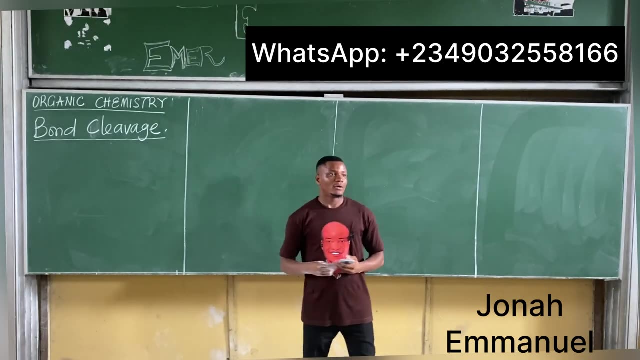 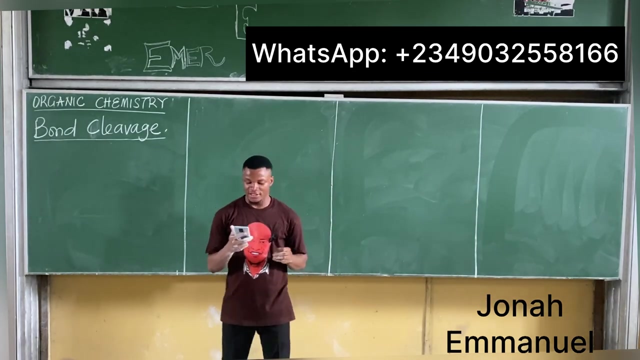 dot dot. nucleophiles. that's it. all right, let's move on. have you been taught bond cleavage in class? homolytic and heterolytic, all right. all right, let's look at bond cleavage, please. definition: bond cleavage: it is a breaking of bond between organic compounds, so bond cleavage means breaking of bonds between organic compounds. that's all, so very please. types: types of bond cleavage. types of bond cleavage: the person is called heterolytic bond cleavage or heterolysis or heterolysis. we define辛 Тыa in Python heterolytic bond cleavage or heterolysis in citing an ineffable fact. 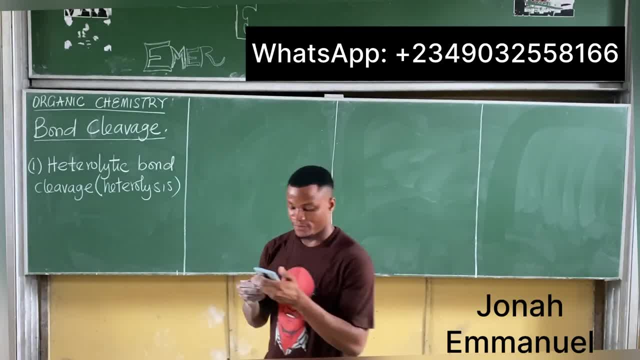 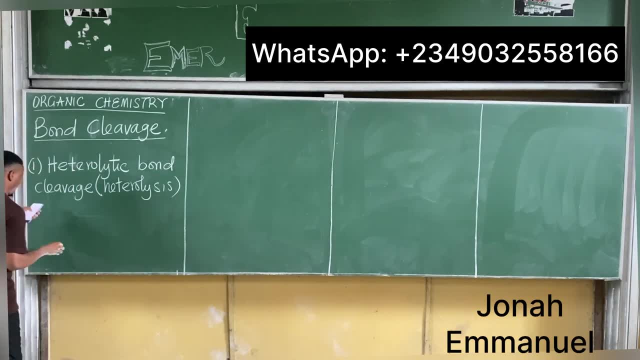 it is the breaking of a single bond in confusing information. it is the breaking of a single bond in confusing information, with two electrons in the bond, with two electrons in the bond distributor. it is not陶酱. it is the breaking of a single bond with the two electrons in the bond in confusion. 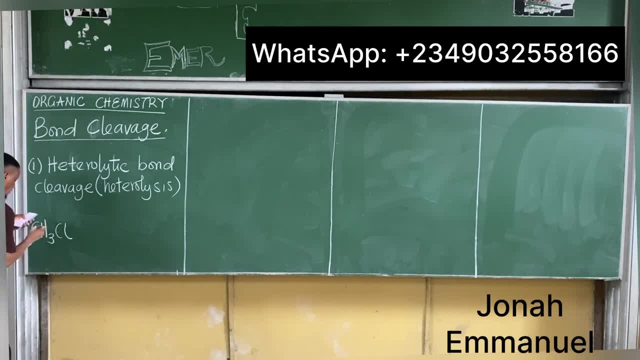 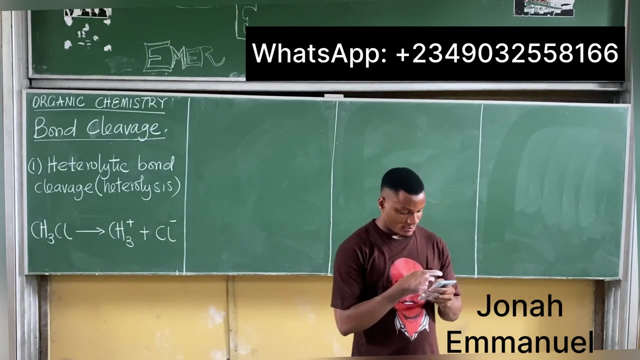 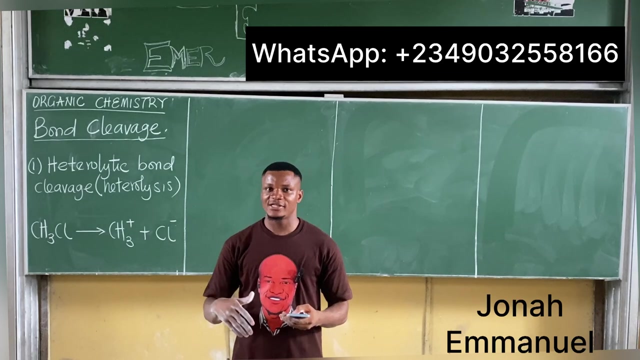 the two electrons in the bond in confusion, distributed unevenly with the two electrons in the bond distributed unevenly, unevenly or unequally, unevenly or unequally between the two bonds, between the two bonded atoms, between the two bonded atoms, or you can say between the atoms bound by the bond. 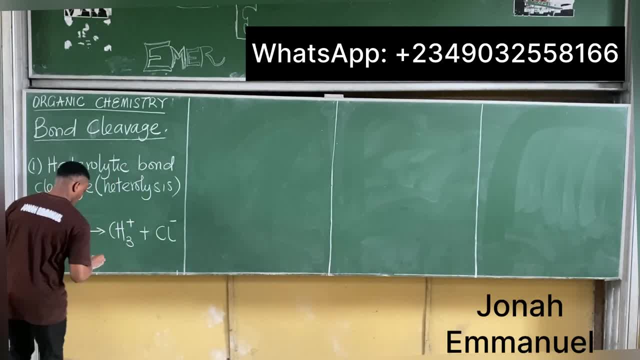 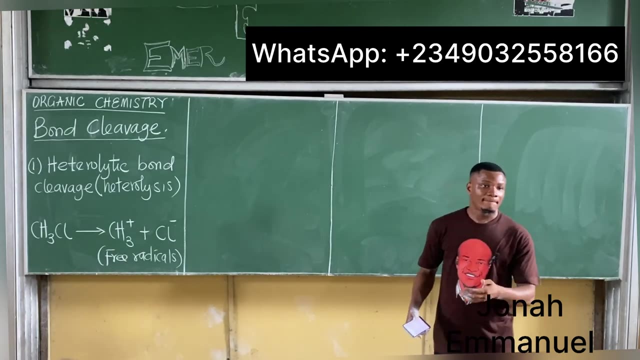 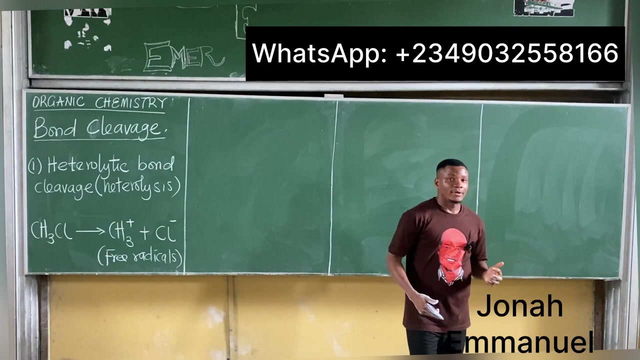 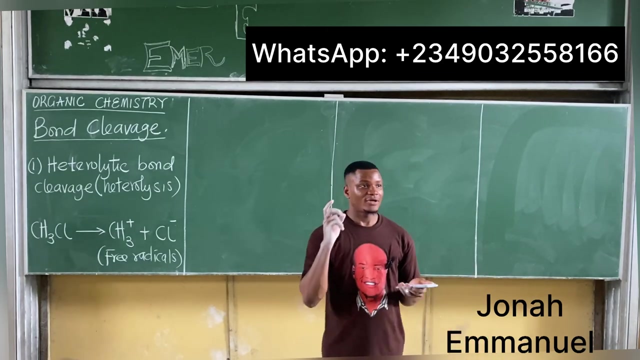 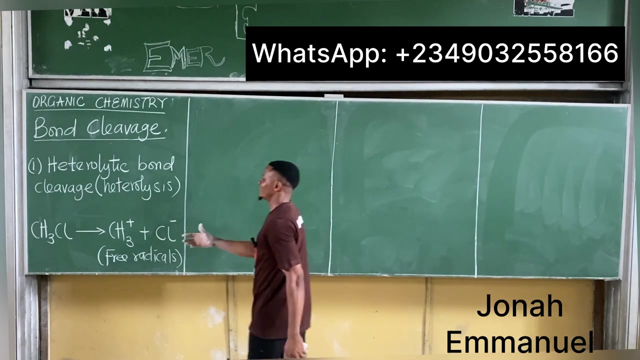 example, you have this, so listen, please listen. one way to easily spot heterolysis is that after the breakup in quotes I mean chemistry breakup, now do I break up. so after the breakup there, look at the products. if they are the same, it's a homolysis. 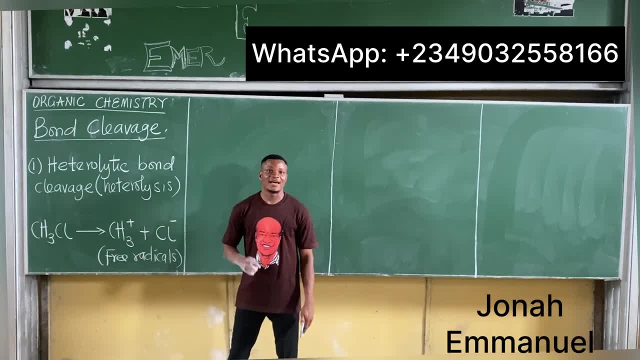 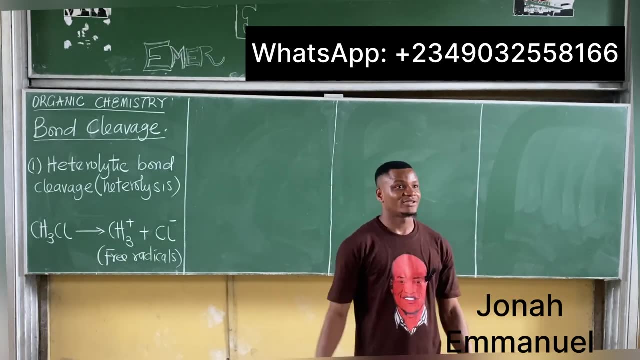 if they are not the same. as you can see here, it's heterolysis. note that what you get after a bond cleavage, it's called your free radicals. yes, they are ions, but the name there is free radicals. that's also a past question, to tell you. 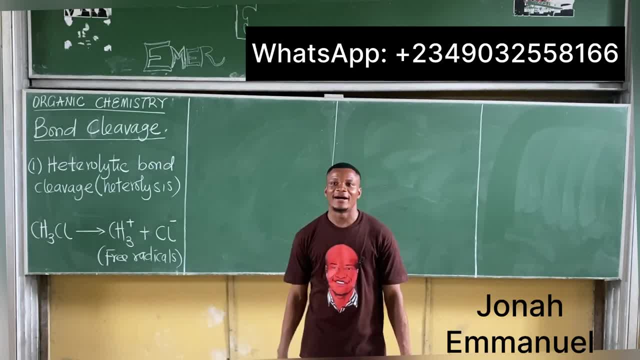 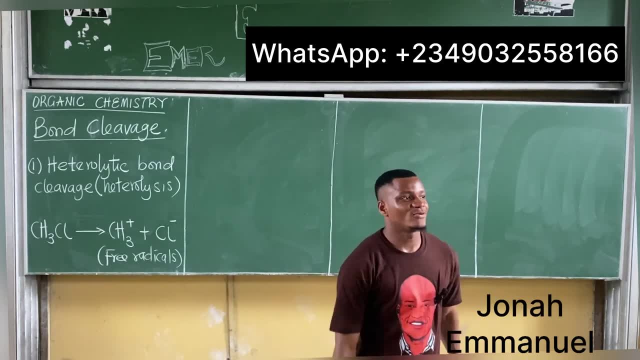 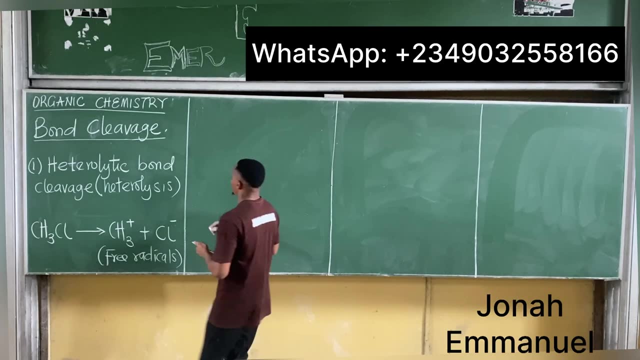 dash are gots by bond cleavage. we have that: free radicals. they are ions though, yes, but the chemical name there is free radicals. free radicals, they are free men, free men, all right. number two, that's the first number two: homolytic, homolytic bond cleavage. 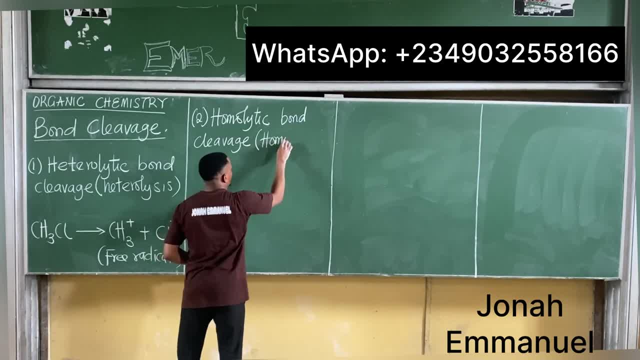 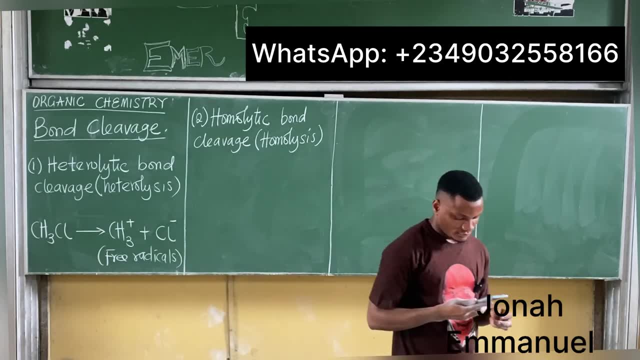 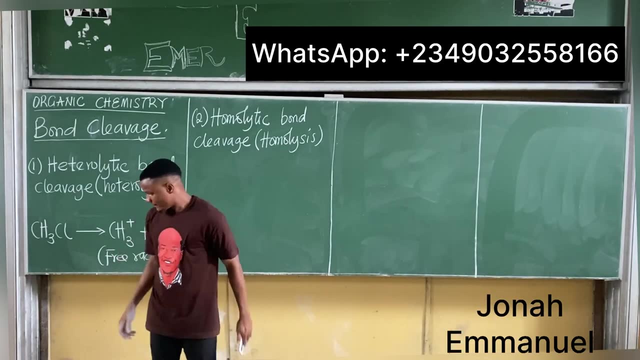 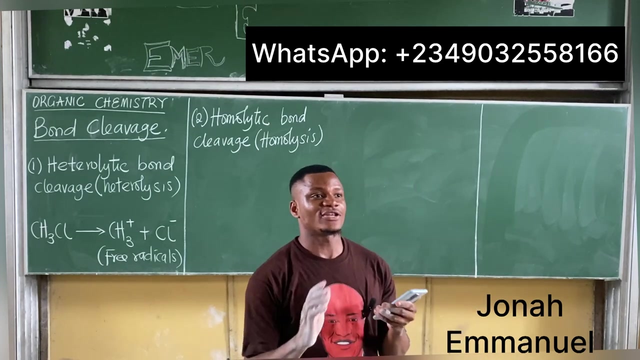 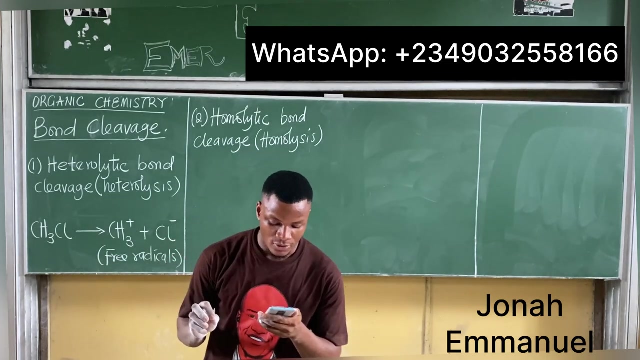 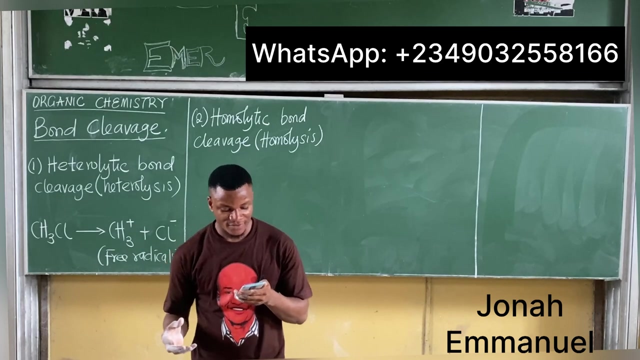 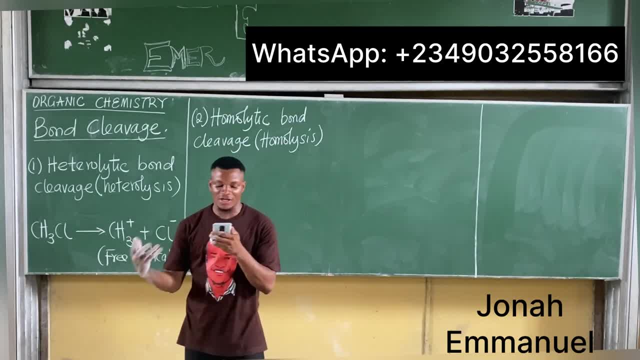 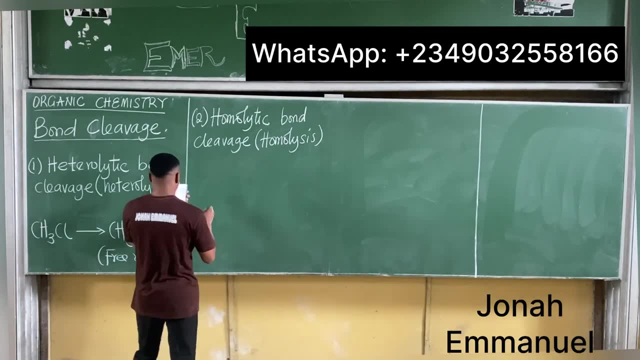 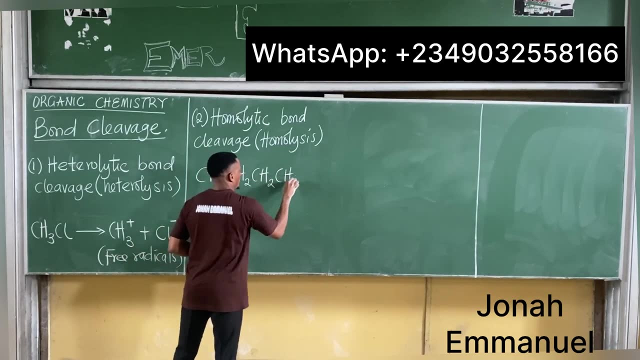 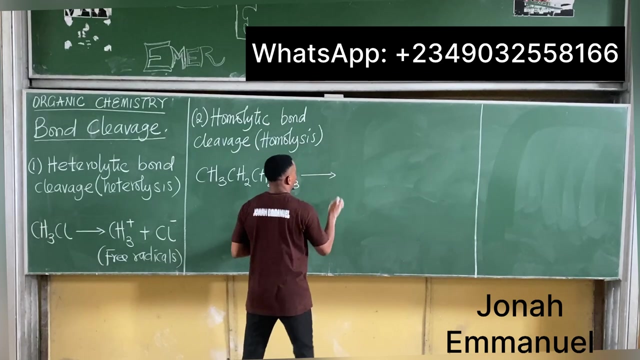 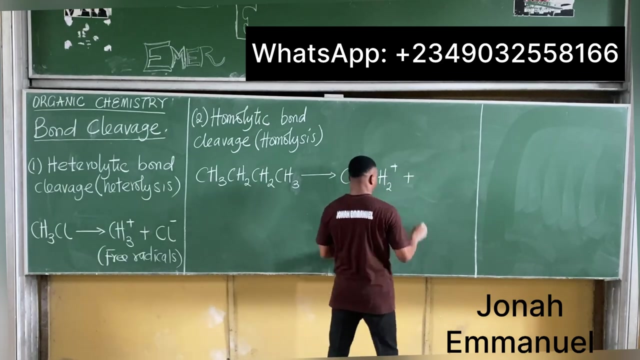 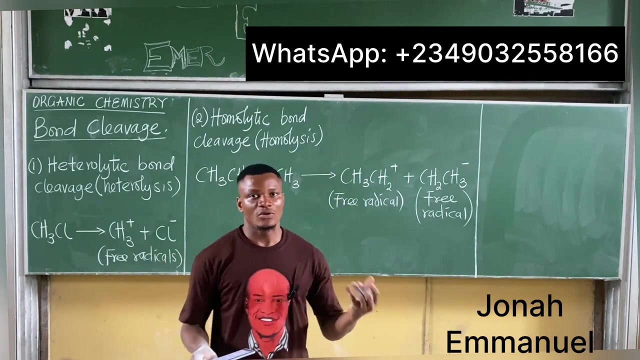 with the two electrons in the bond distributed equally or evenly between the two atoms, between the two atoms bound by the bond, bound by the bond. example, example. you have this. so i've said, the easiest way to know that it's a homolysis is that. look at the 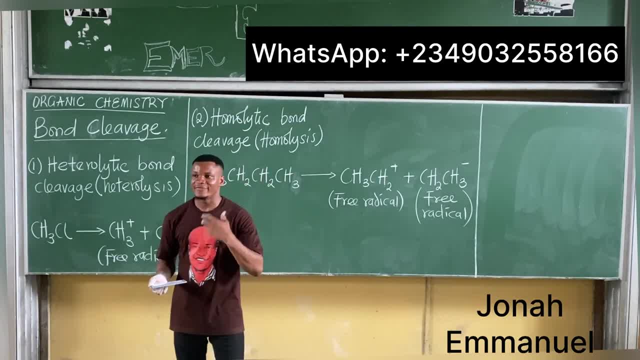 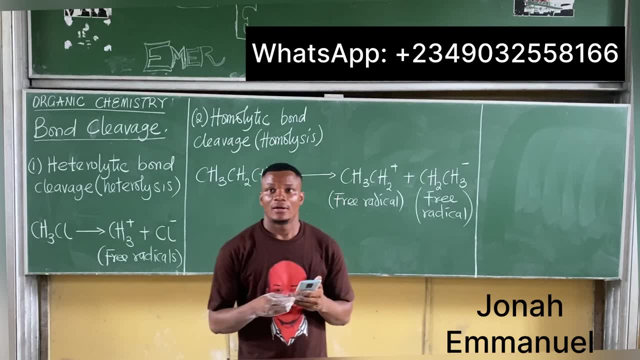 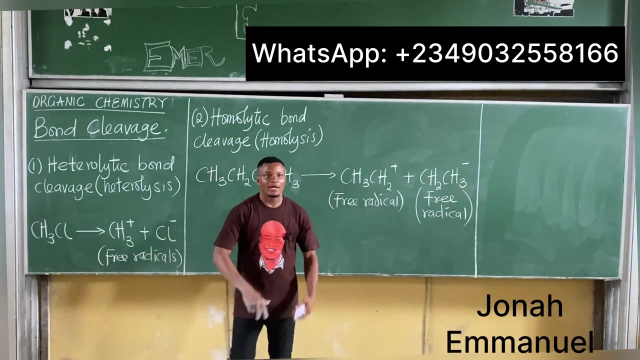 product. if they are the same, simple homolysis. they are different- simple heterolysis. it's that simple. so i said the easiest way to know is this. i said: look at the product. if the products are the same, is a homolysis homo same. if the products are different, it's called what they're: heterolysis. 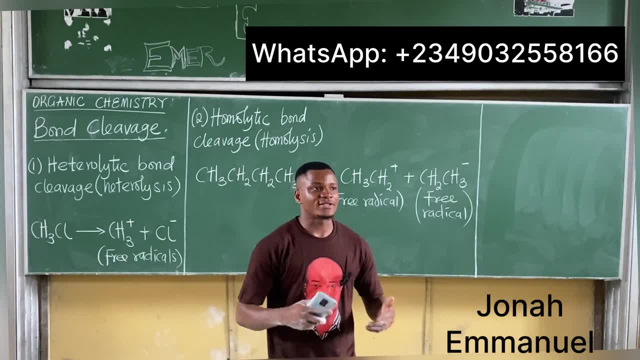 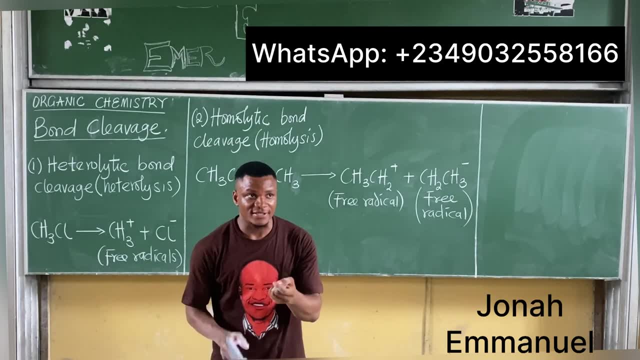 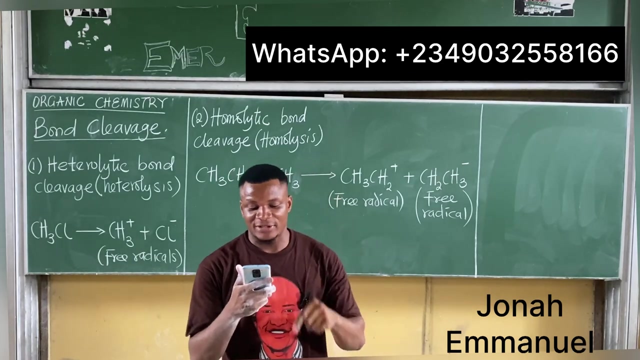 that's all. so for homolysis bond cleavage, so that it's shared equally or evenly between the free radicals. heterolysis bond cleavage, so that is shared on equally- i think that's like the keywords- equally on, equally free radicals, whatever. so here's a, here's a sample. um, here's some good test question practice example. or here's: 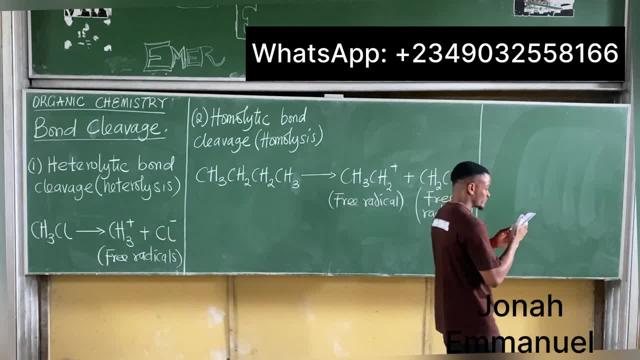 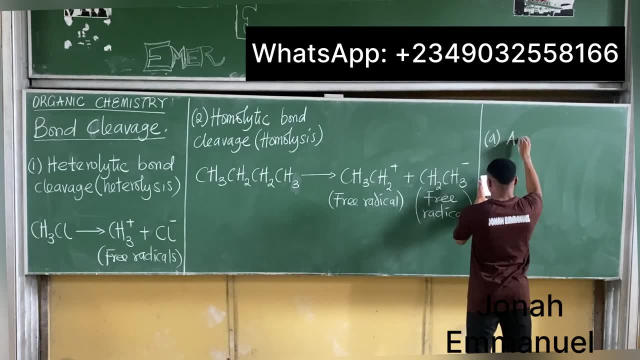 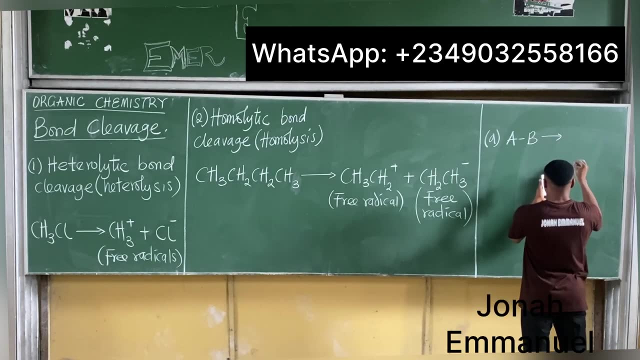 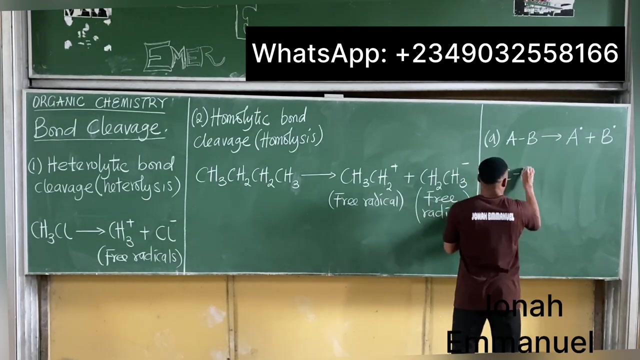 the test question. please identify the type of process. identify the type of process that has taken place. identify the type of process that has taken place in each of the following covalent bond, in each of the following covalent bond. so you have this. you have this. 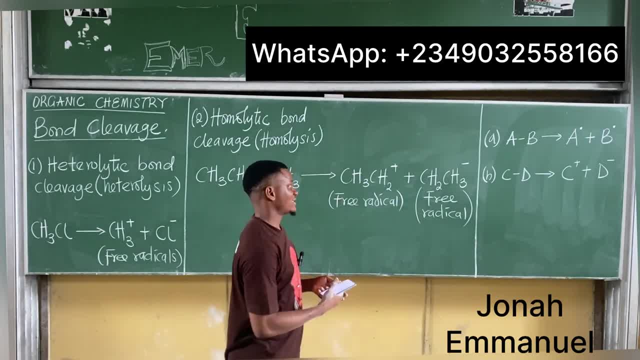 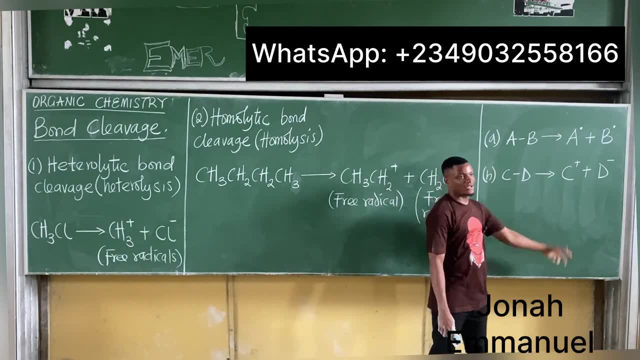 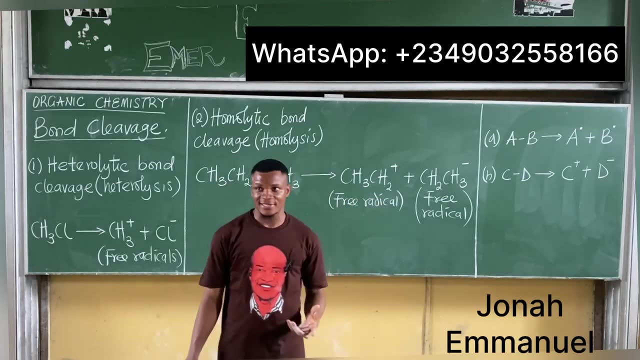 you have a and b. they say identify the kind of process. that's happened this? so the first you're seeing here is that this has broken down to a and b, this has broken down to c and d. which of them is homolysis, which of them is heterolysis? a is what there, homolysis, b is what there, heterolysis. so in 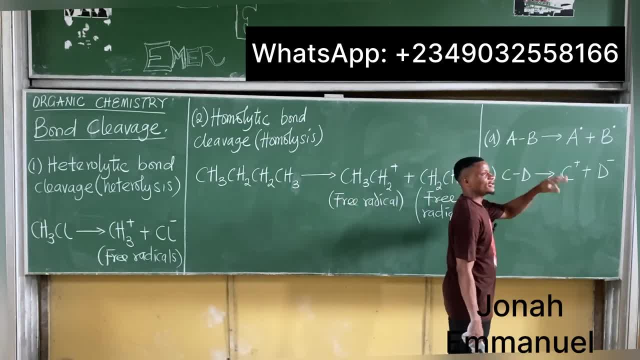 a case like this, where you're not having alphabet. there, your key task is not by looking if they are the same. they can't be the same. a and b cannot be the same. well, except in mass. you must now say: we are a equal to b. have it, that's math, but it's not. it's not chemistry. so what? you're not looking. 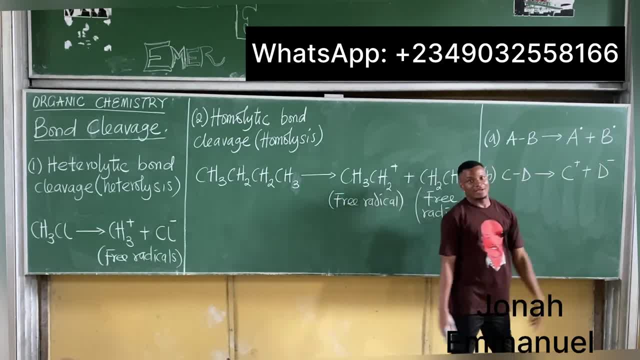 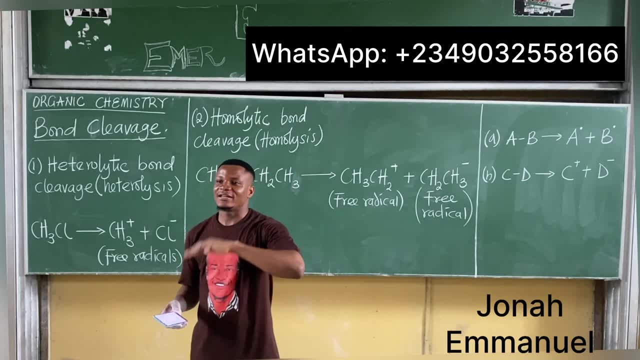 for this. the same thing there: homolysis, different heterolysis. this is a past patient also know this one here. all right, let's look how we do. we don't this one. let's not look at the next concept here. somebody's saying: how is it different? how is it different? i said: look at the product. 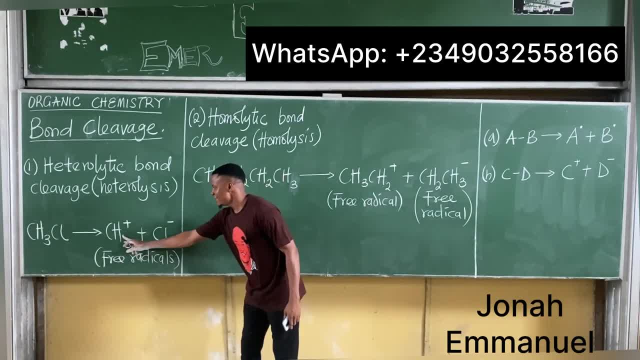 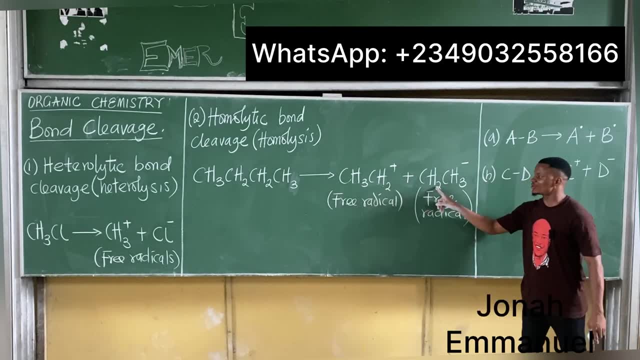 this product and this product are not the same thing. methyl and chlorine- hetero, don't stress. look at this one. here the products are the same how ch3, ch2, ch2, ch3. they're the same thing. that becomes homolysis. that's how it's done. so just look at the products. are the products the same? yes, homolysis, are they? 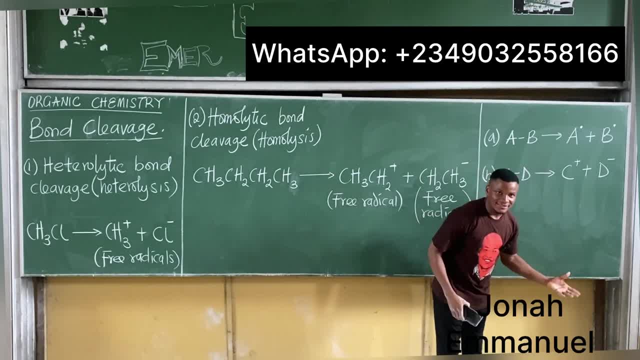 different. yes, heterolysis. in a case of alphabet i've said there's no way that a and b can look the same. how do you want to bend it at that point? now it's no longer if you look the same. now it's more of if the dots like dots, dots, that's like the key stuff there, dot, dot, the same thing. so homolysis. 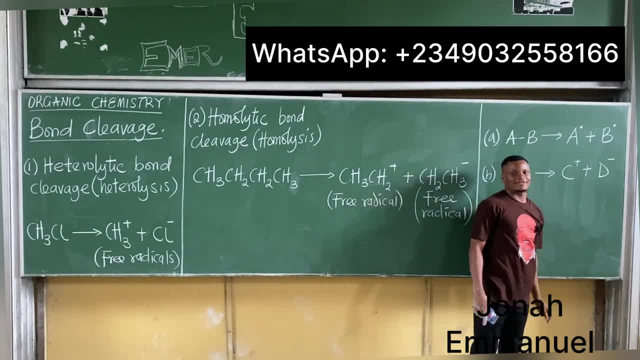 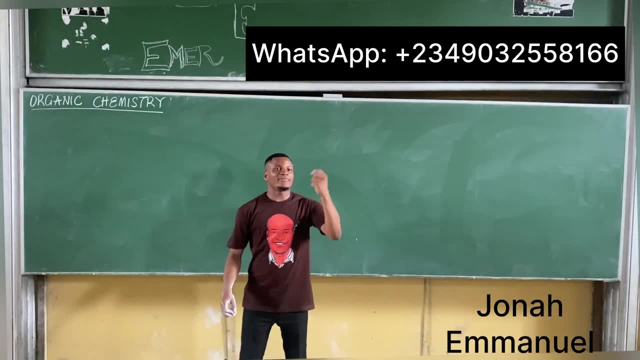 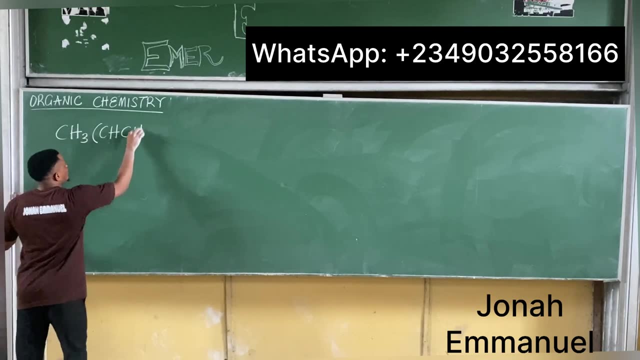 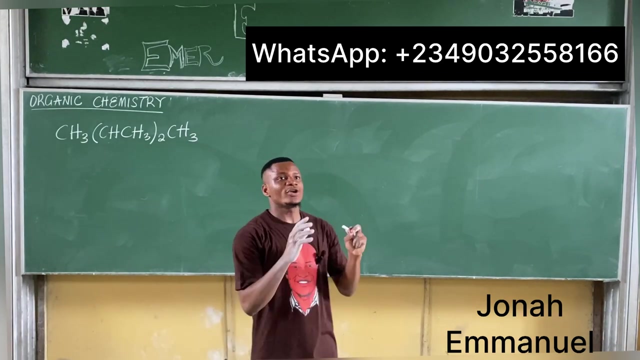 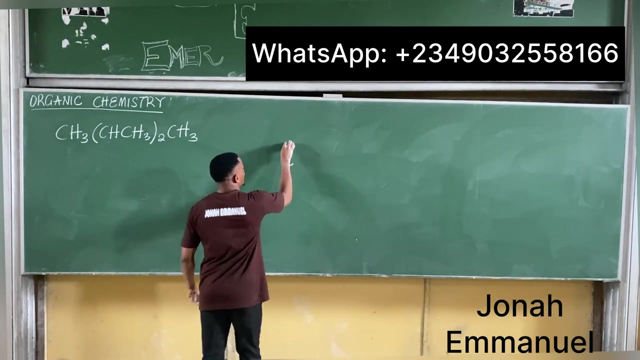 plus, minus, different thing, heterolysis. that's it okay, any question again. please give me that structure again, please. uh, how do i name ch3 into order? ch, ch3, twice ch3. i've said as much as you can to easily name compound. first of all draw the structure. start with this one here, ch3. so they come c, one, two, three. 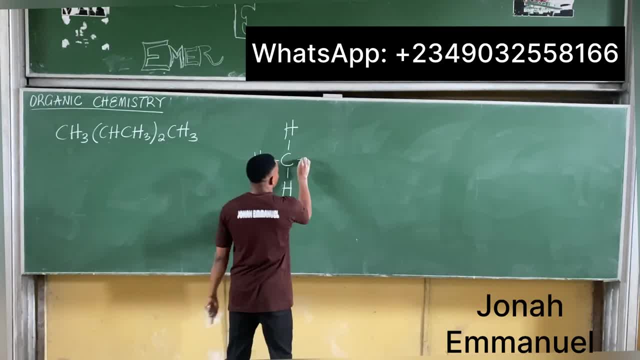 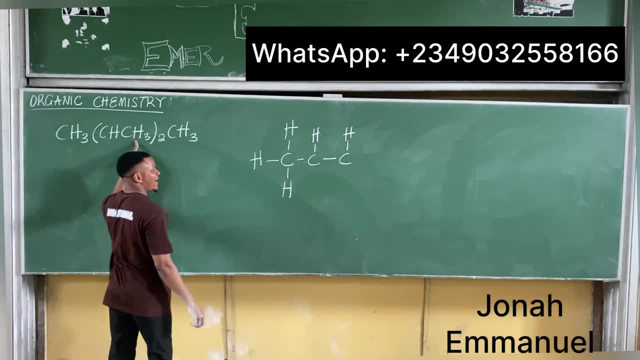 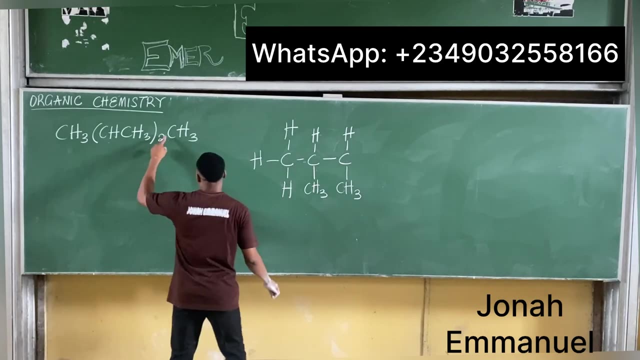 next up si h, two times, that becomes c h and then c h, next up c h3 twice. what will you come under? obviously here ch 3, here again ch3. finally to ch 3, that becomes c one, two, three. that's your compound 1..2..3. 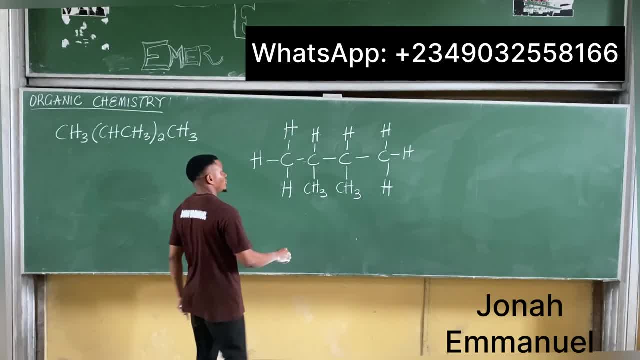 9. so it becomes of course. you get something else from here. first of all here. just remember that right three elements end up becoming ch1 and th3. ch2 will be following what? so what will you add to? if 100 c have better known, you get 150 c have 2cc. if 100 c have 3, but i, university have the other 4. of which you have in the lastати test. yes, let's do it. so it does look like it. if 분's are lilac, ch is far either. on this side, robin has i shared only about about 10 kph. the red color of the 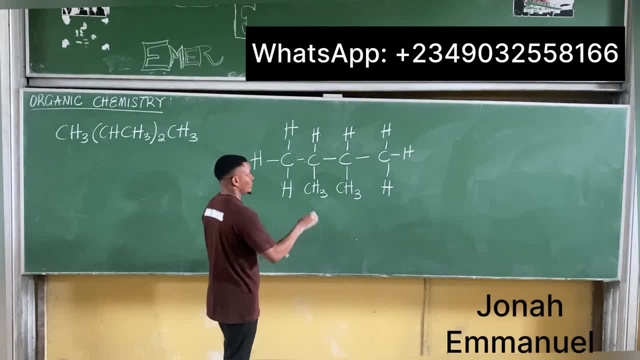 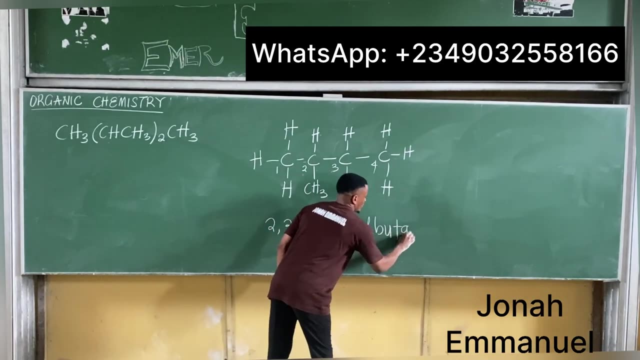 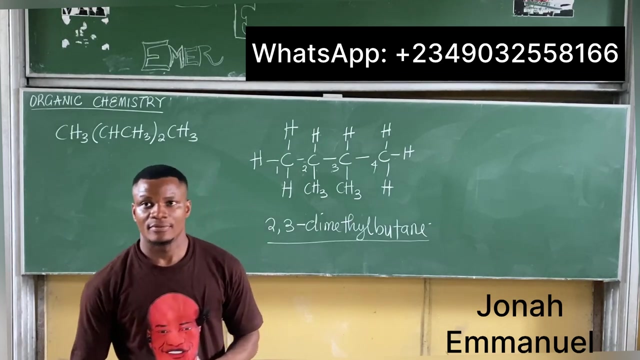 numbering from left and right. the same thing: one, two, three, four becomes two, three, two, three. what again there, di-metil? what there, butane? please open your eyes. these things, they exist. they exist all right. so let's take, let's see the same case in a skeletal form. let's look at this. 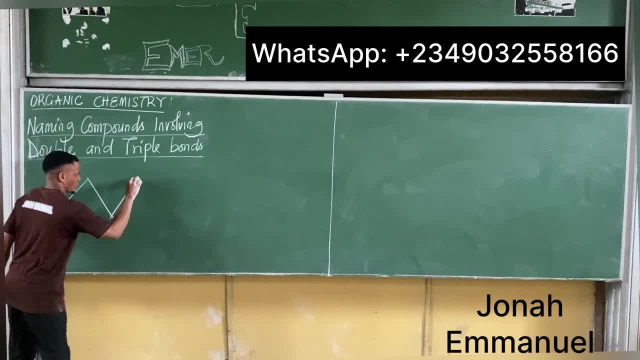 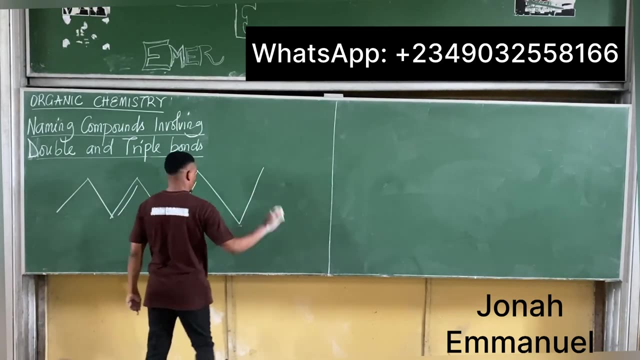 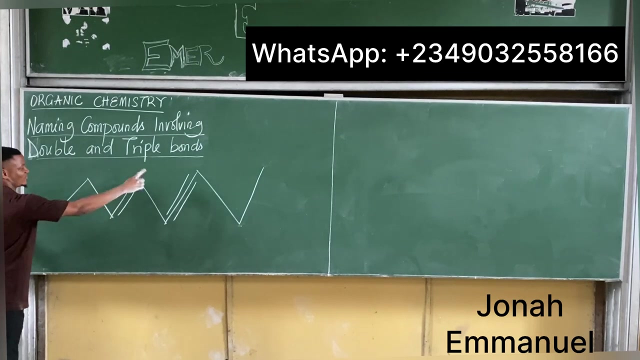 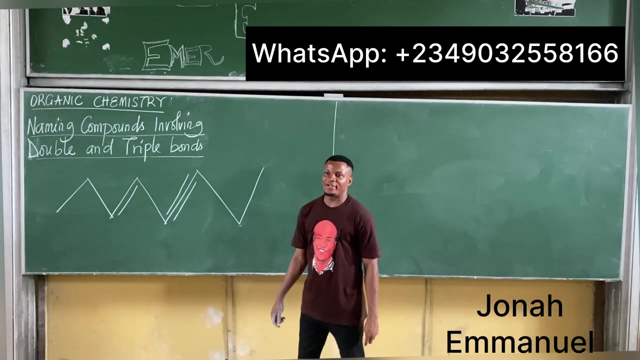 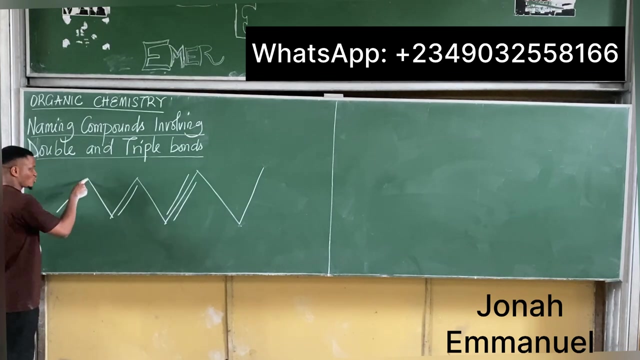 all right, please forgive my inconsistency. okay, in my triangle this one looks bigger, but you get the concept. how do you name this compound? huh, longest continuous carbon chain, how many? so we know that at every vertex is a carbon. so one, two, three, four, five, six, seven, eight, that's what there. 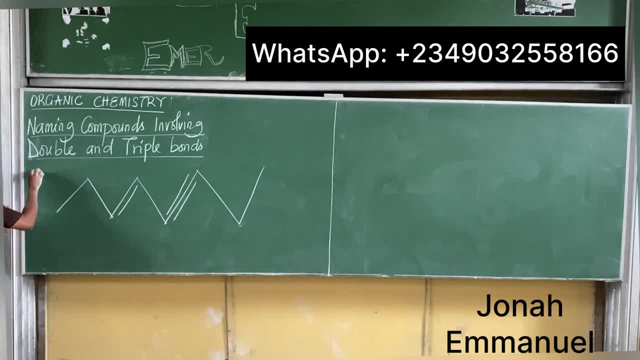 and ox Metals. let me make it a none again, let me make it a deck. aha, I'm having one, two, three, four, five, six, seven, eight, nine, ten, all right, so how do you name this first? obviously, the numbering that will give me the shortest distance to double bond would be like this: I'm having one, two, three, four, five, six, seven, eight, nine, ten. 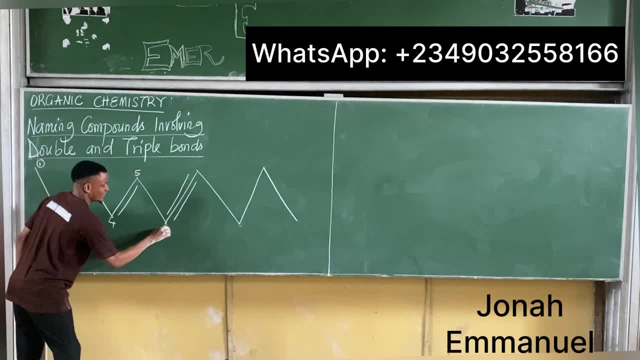 dark black one, two, three, four, five, six, seven, eight, nine. ten is a definitely a deck, 10 is a deck. so because what mourning start there, death coming in through it draw. and 6 y Descent. is it descent or decant Descent? 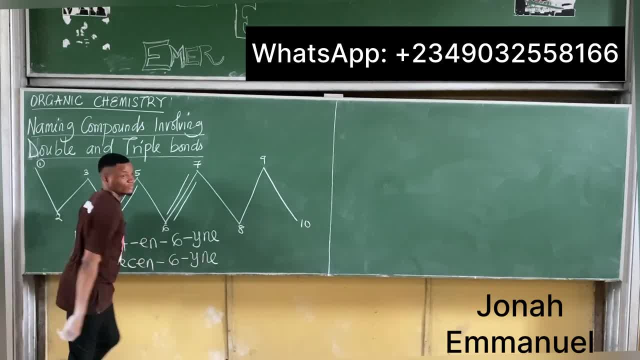 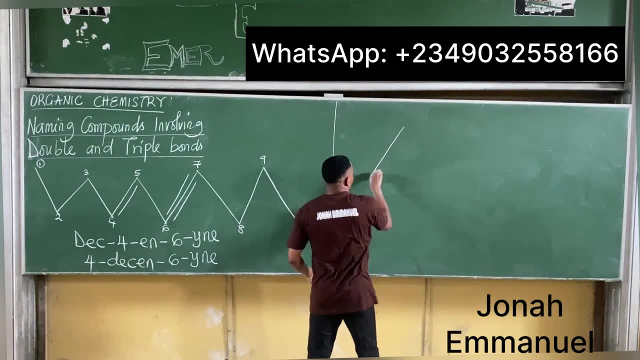 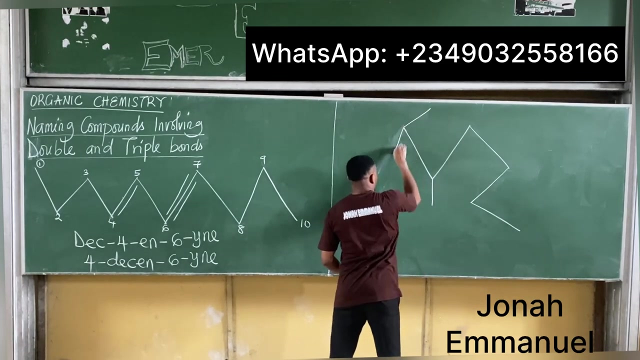 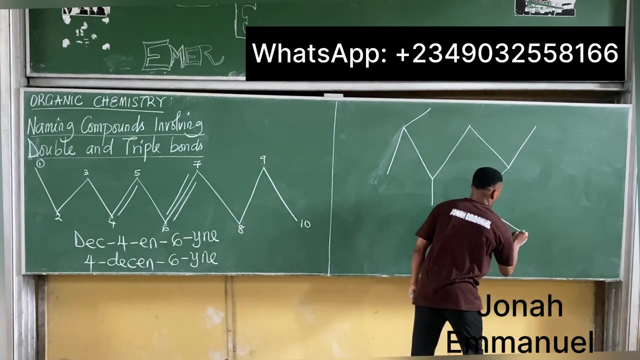 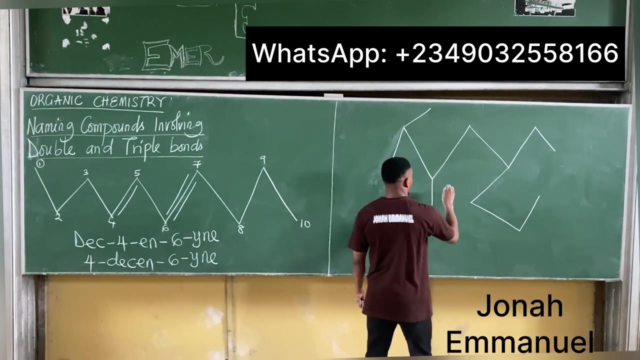 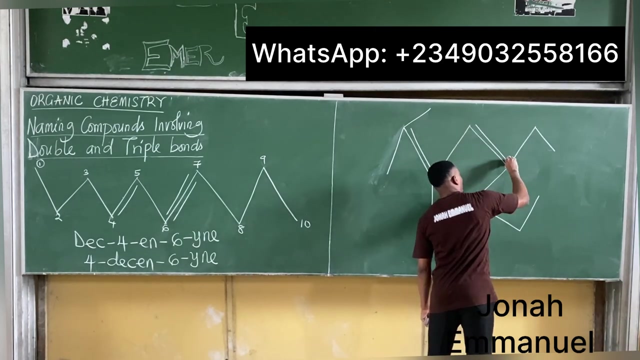 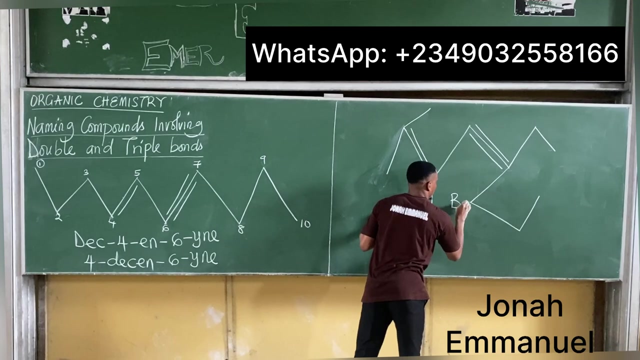 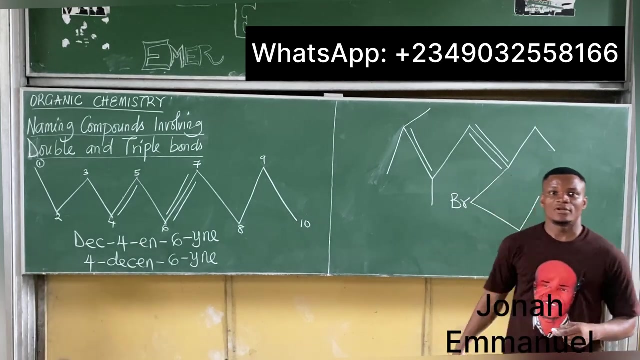 Okay. So that's this. Is that okay? Let me give one example. Let me give one more example. Let me include something else here. Let me include something else, Please. you have the next three minutes. please See if you can provide the name of this compartment. 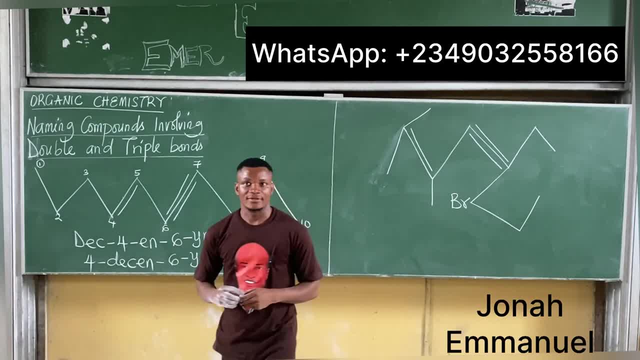 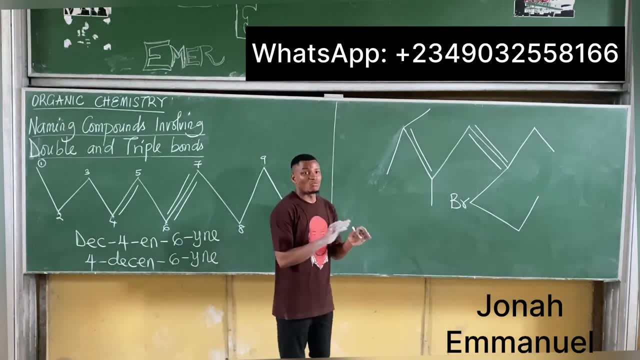 You have the next three minutes. See if you can provide the name of this compartment. All right, so look up, I want to name this. What do I do? Very simple, Longest continuous carbon chain. We've stressed that thing too much, so I'm going straight. 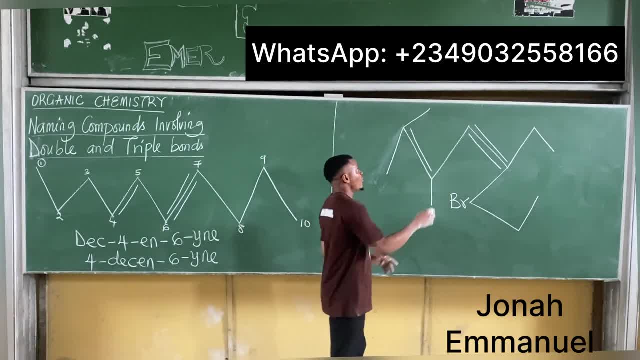 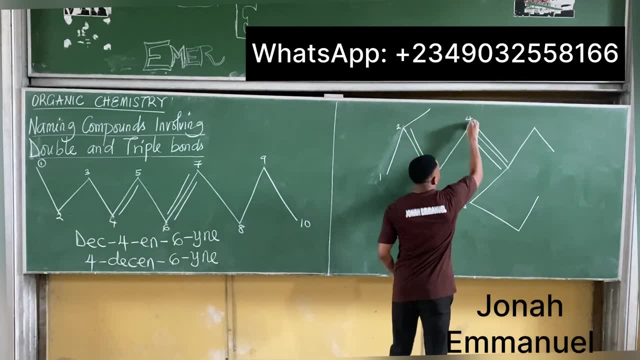 It has to be from here to here, Abhi, Yes, Or from here to here, The same thing, is it not? Yes. So I'm having one, two, One, two, three, four, five here, six, seven, eight. 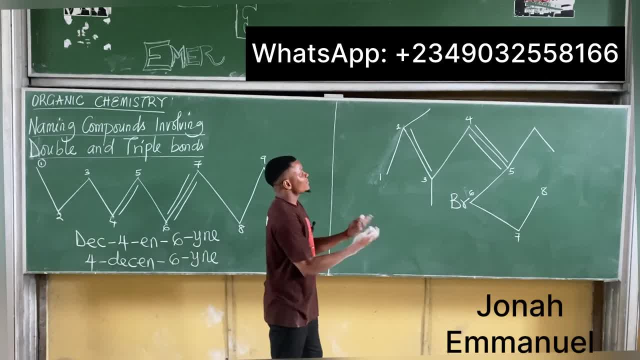 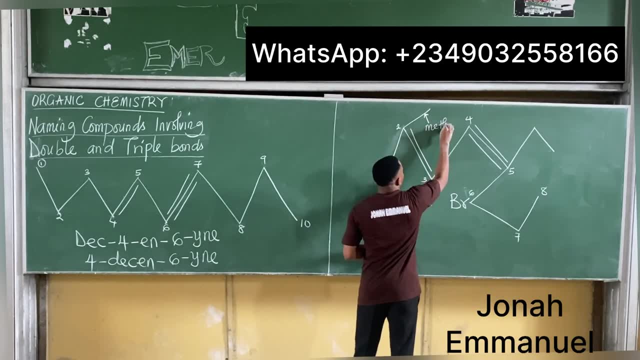 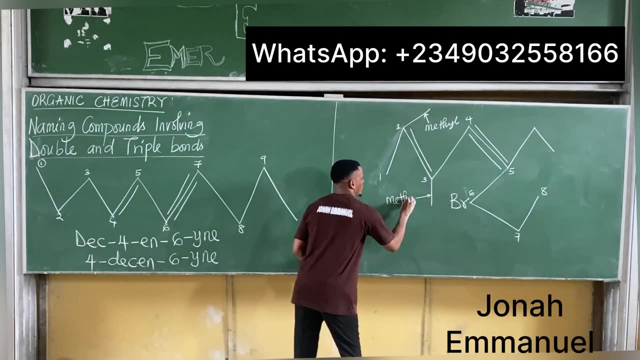 It's an oct compound. It has now observe that this one here is not part of the parent carbon, So it becomes what there Methyl. This is methyl. This one too is not part, So it becomes what there Methyl. 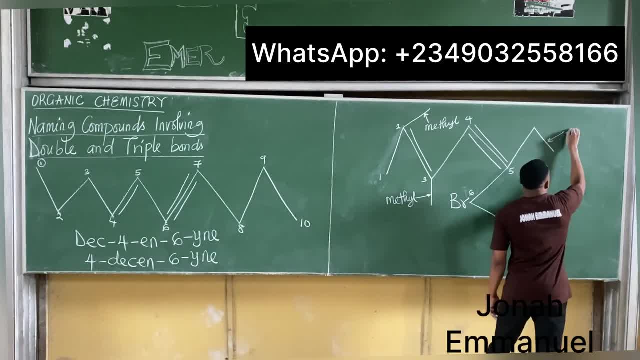 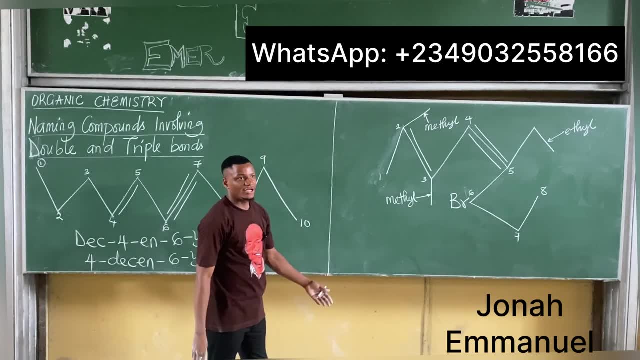 This one is not part. It becomes what there? Methyl, Methyl, Ethyl, One, two Ethyl. So first things first get inorganic. Inorganic is the bromo or bromine. So it becomes what there? 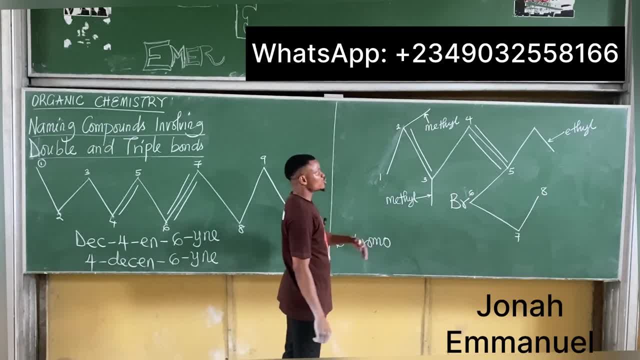 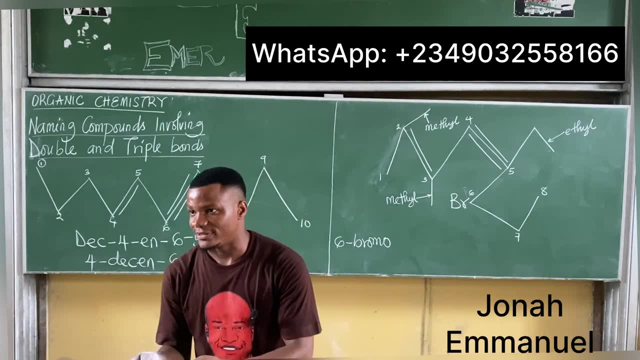 Six: bromo Bromine, attrition six. Now go to organic. I said for organic it depends on the author. So the author will say take position before alphabet. So we'll say take alphabet before position, But let's take alphabet. 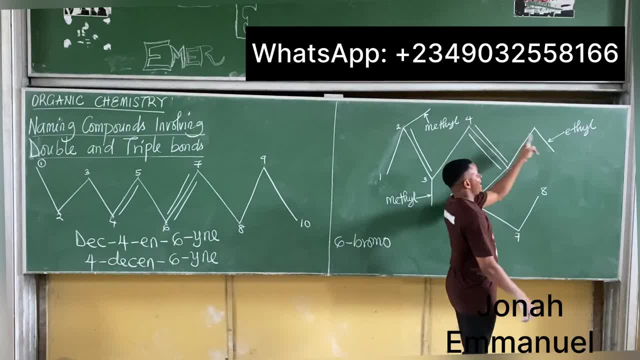 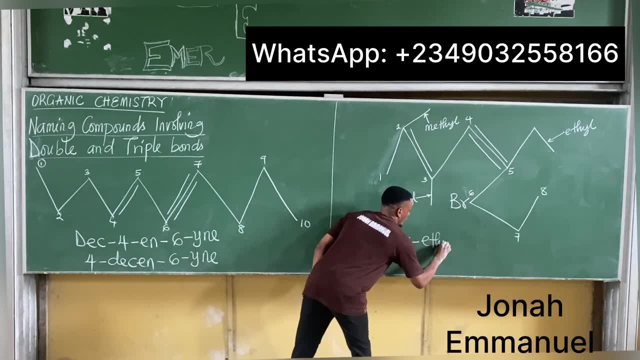 If I take alphabet, I'm going to take position before alphabet. I'll have E before M. Ethyl Carbon: what there? So it becomes what there. Five ethyl Come to methyl. Methyl occurs twice, Are they? 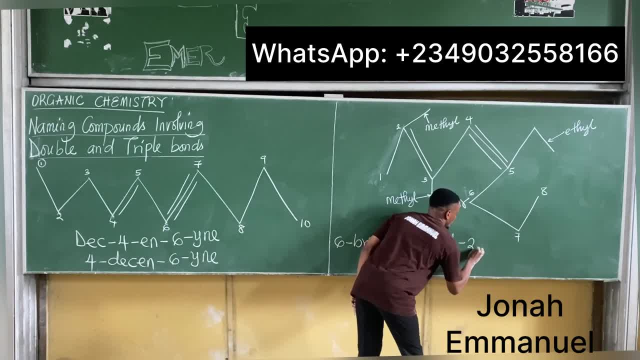 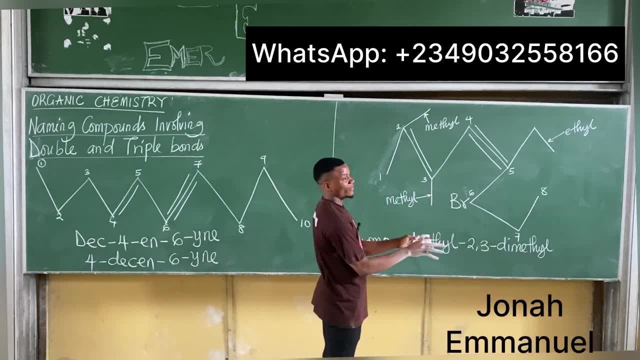 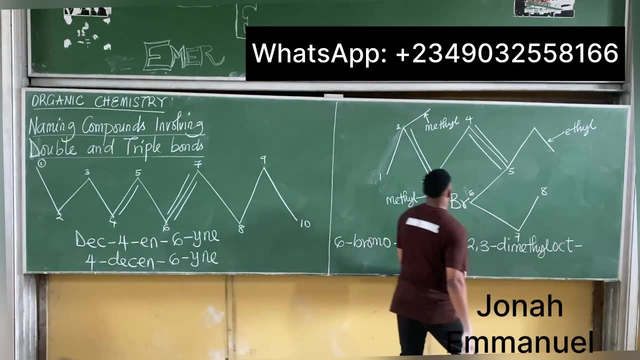 Where and where. So it becomes what there? Two, three di-methyl, Di-methyl. I'm done with sub-dituents now. Now take the compound as a whole. That's ox, Ox, ox. what there? 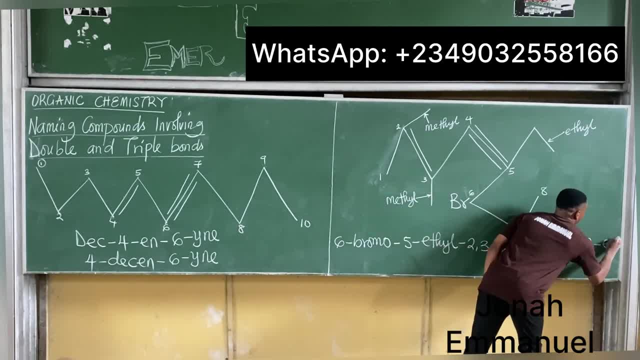 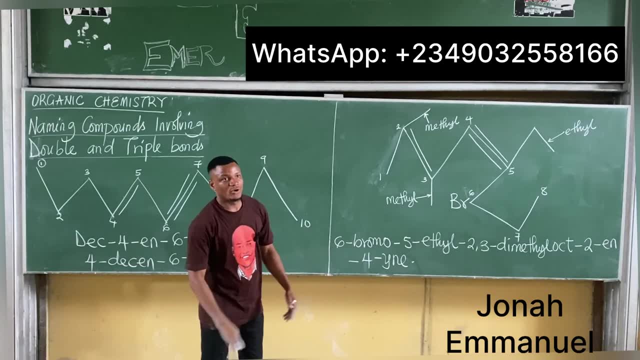 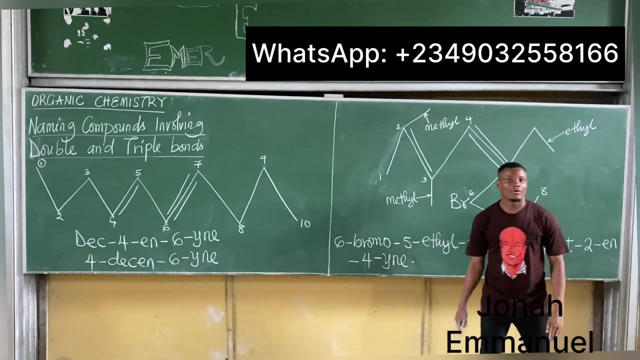 Two and next up four, all right, very simple. Or you can say at this point, at this point, you're not saying di-methyl two, octane four, all right, same thing, same thing. 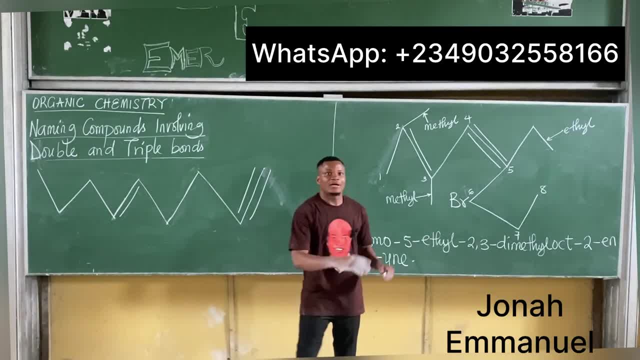 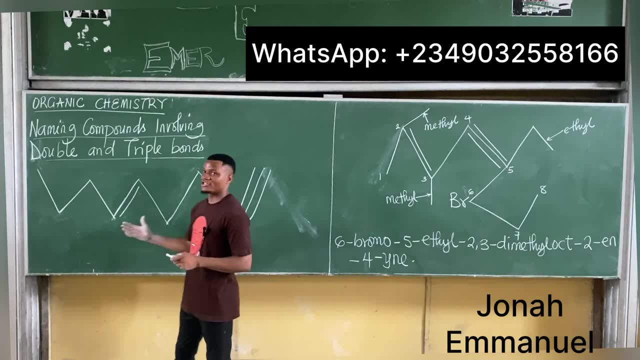 Now listen. look at this, let's get this thing done. look at this, Look at this, Look at this. So here's what I told you earlier. I said for a compound of this nature. here I said I am naming or I am numbering from. 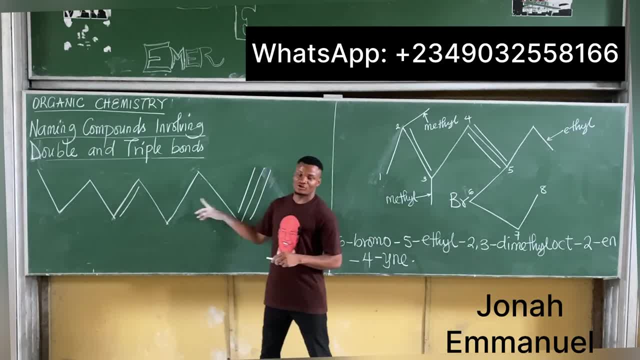 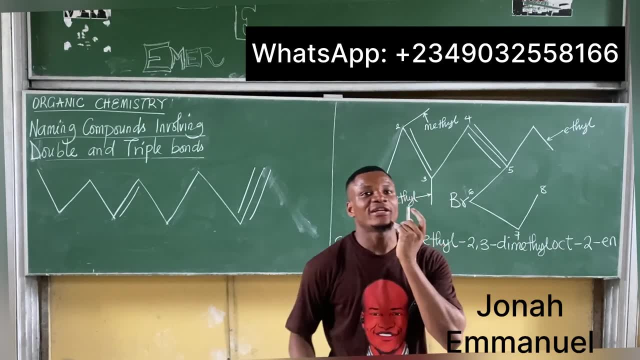 the position that gives me what there? double bond first before triple. Now, what if it's in a case like this? right, We can still do that pattern. or alternatively, if you look at what they are saying, right, There's a pattern that they said. I think it just came to my mind now. 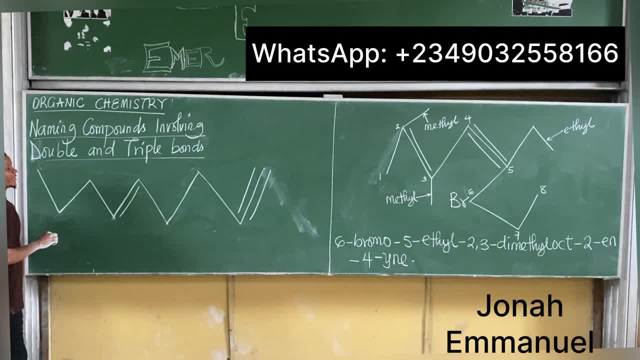 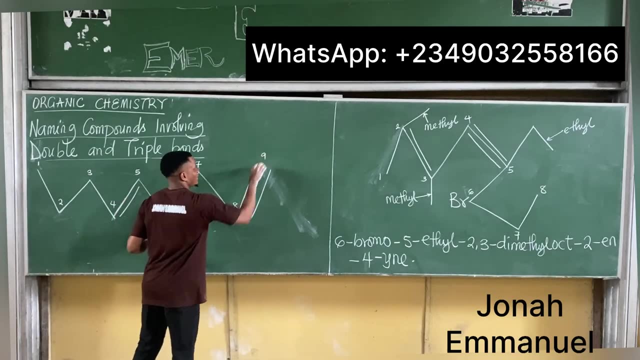 Here's an alternative way. Look at this. please Let me do a numbering here. If I number this, I'm doing both upper and lower numbering. So I'm doing upper numbering: one, two, three, four, five, six, seven, eight, nine. 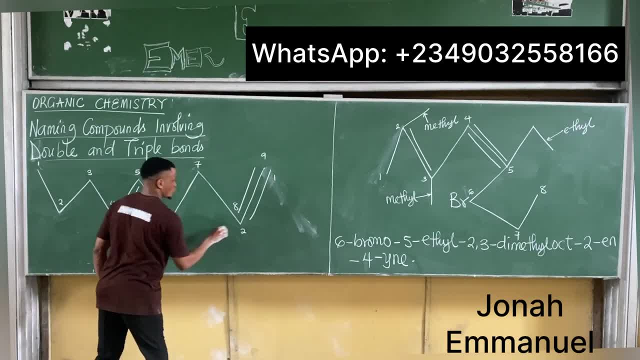 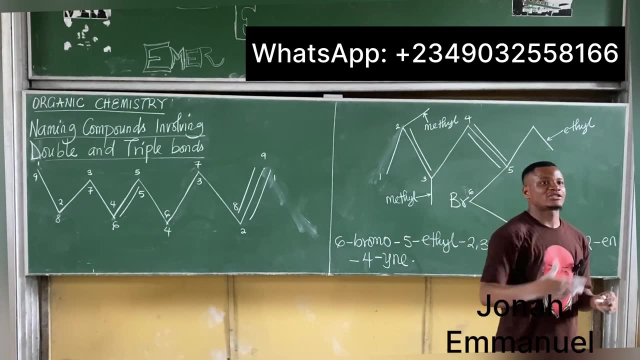 Lower numbering one, two, three, four, five, six, seven, eight, nine. So please watch this. This is another concept of naming this. Let me do one that the lecturers have been using. So here's the pattern here. 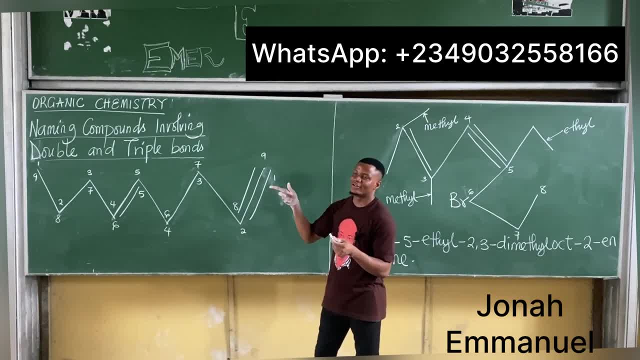 So for a case like this where they said this one is in quote: terminal, that means close to the end. So if I want to number this, what do I do? So the other concept of naming this here would be, if I go with upper, numbering from upper. 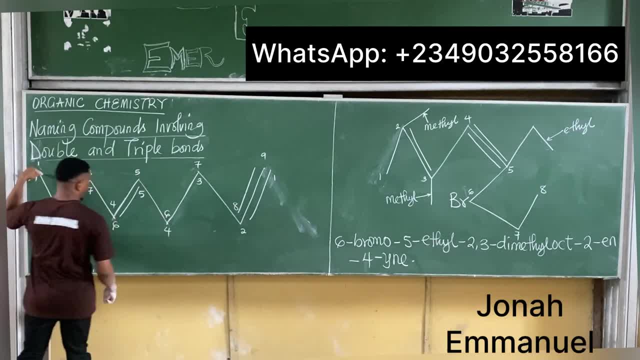 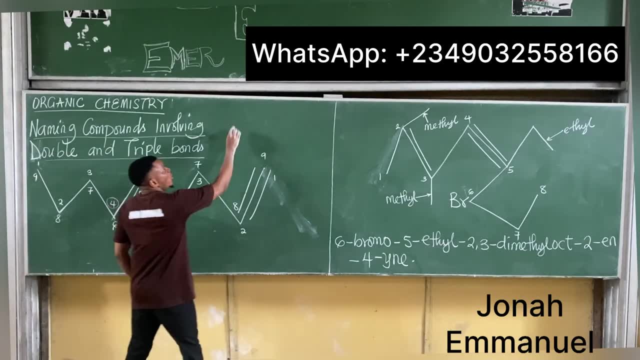 numbering, my two numbers would be upper numbering. observe that double bond occurred at carbon four and then I want to get in there eight. So from upper numbering, If I go with lower numbering, I have four and eight. If I go with lower numbering, from lower numbering, if it comes from like I'm having what there? 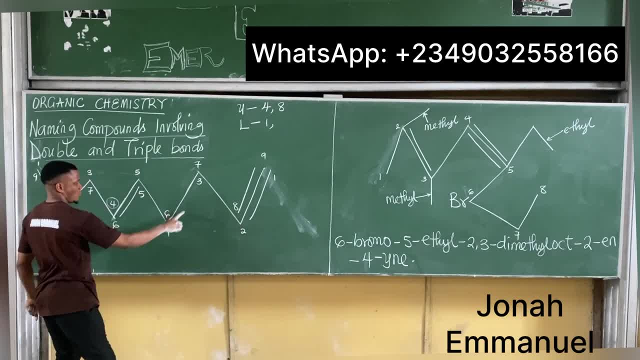 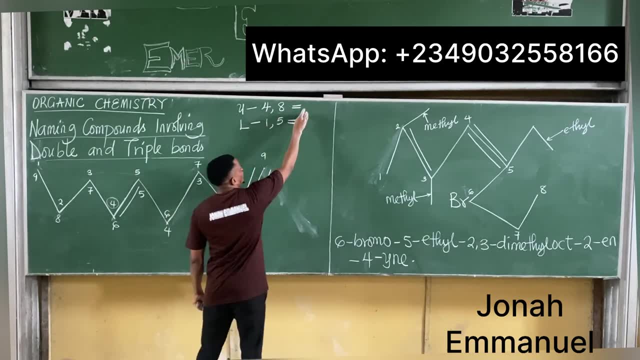 One, one and what again? there One and five for double bond. One and five. So we'll do a summation. If I sum this to gives you what there 12,. sum this to gives you what there six. 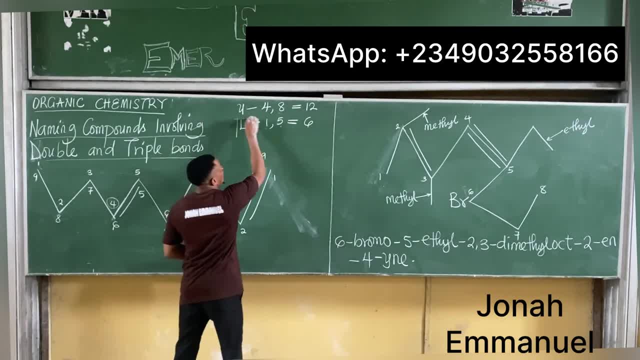 And now I'm saying: you now take the one that gives you the lowest sum, which is six, Because these two here, if I sum one and five gives you six. So I'll now take the one that gives me the lowest sum in quotes, and that's which of 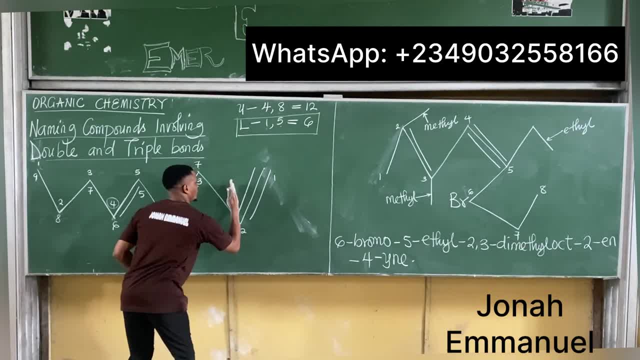 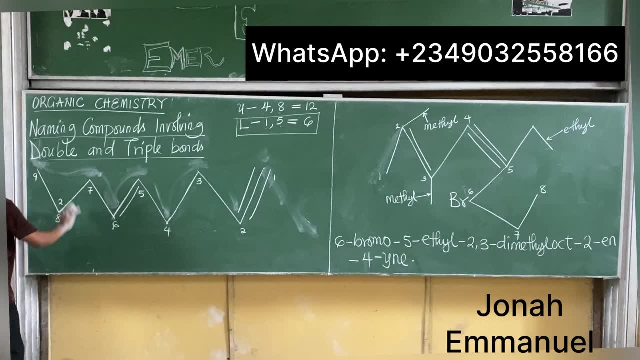 them. Lower numbering, that be. So I'll now take off the upper numbering. So what would this numbering be there, which? okay, that becomes what there? Nine is what None, So none. what there? Five, One and one and 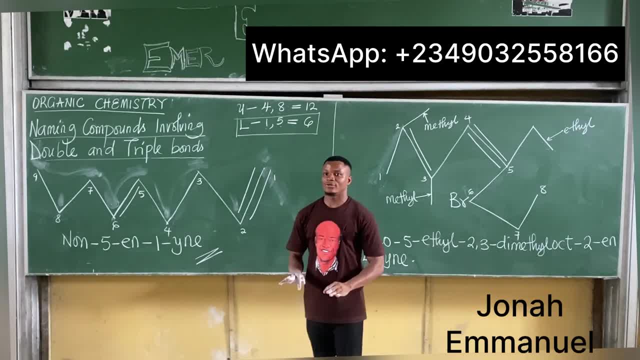 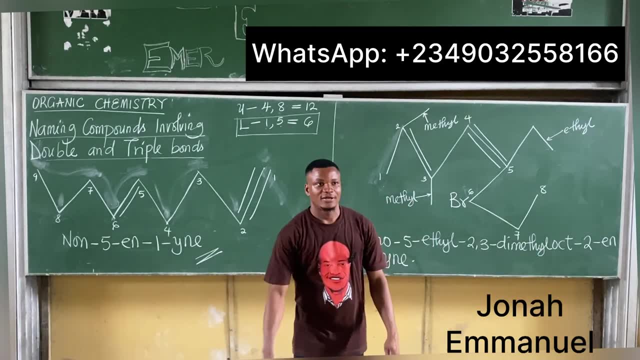 So that's another concept. Hold on, hold on, hold on, So that's another concept of doing this. All right, So listen, listen, if a lecturer said you should use this one, no problem, So you can use this one too. 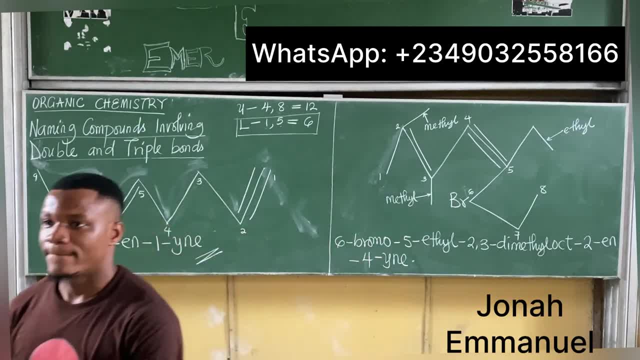 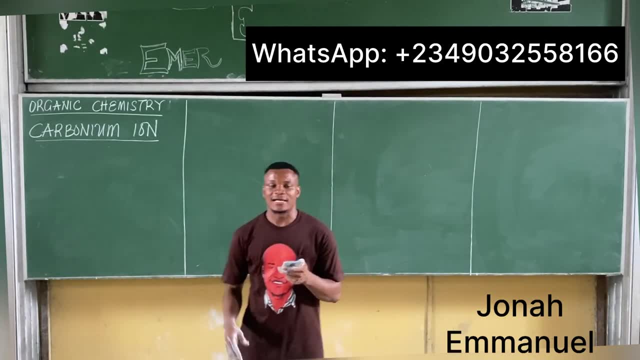 That's a pattern. Yes, Steve, let's hear you. Next concept: let's look at carbonium ion Definition. we said a carbonium ion is an organic cation in which the positive charge is located on a carbon atom, Full stop. 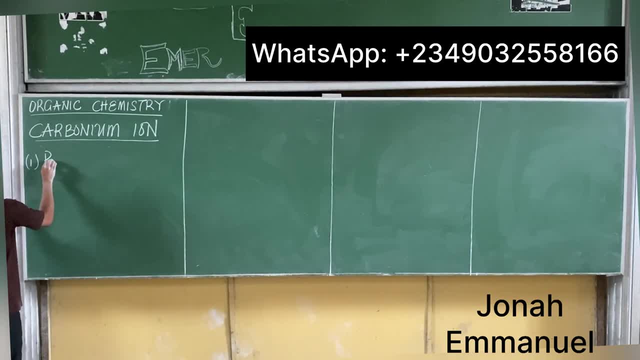 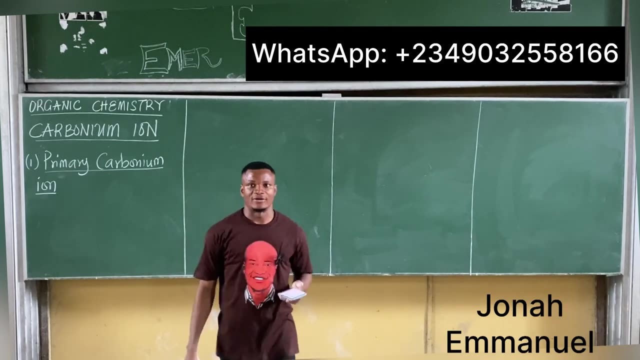 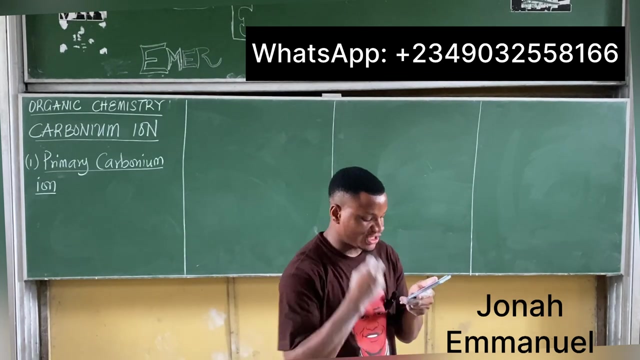 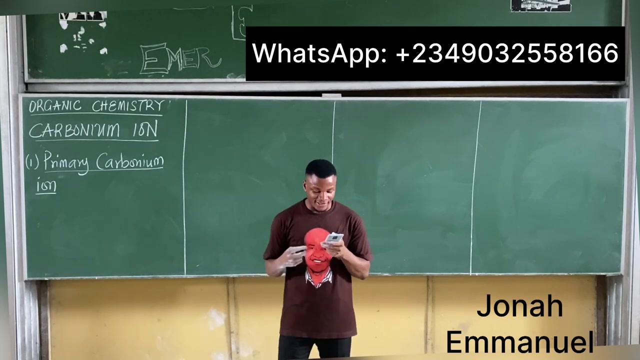 Take that, please. Types: Types Number one: Number one: Primary carbonium ion. number one: primary carbonium ion. take that, please. here the carbon which carries the positive charge. here the carbon which carries the positive charge. here the carbon which carries the positive charge. 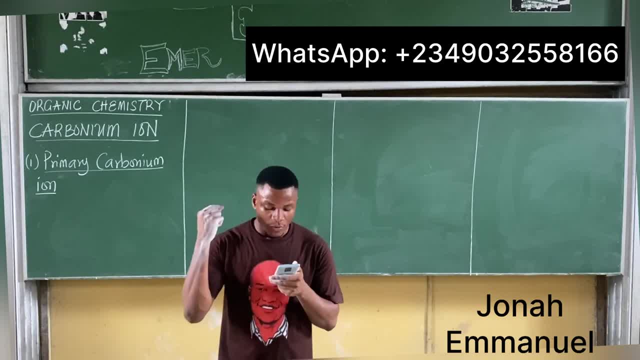 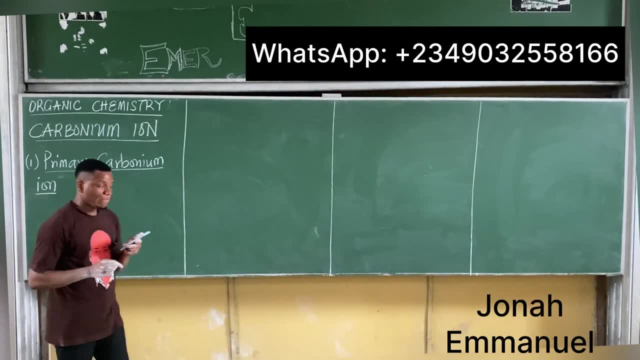 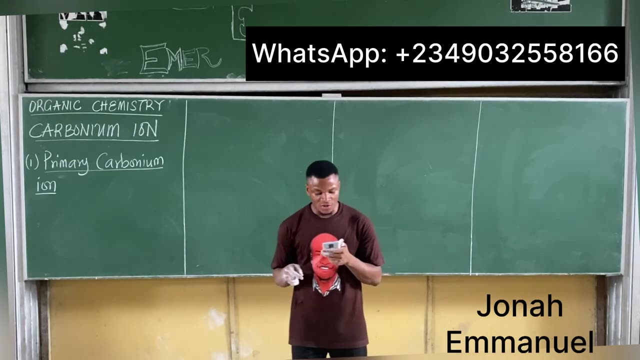 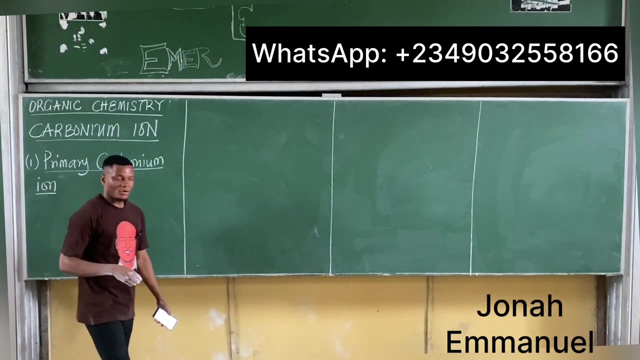 is attached to only one archive group, is attached to only one archive group, to only one archive group. or just hydrogen, or just hydrogen, or just hydrogen. so please look up, please. so i'll do the first ones. subsequently, you should be able to name it on your own, please. so the first one there: um carbon bearing the plus sign. this this now becomes: 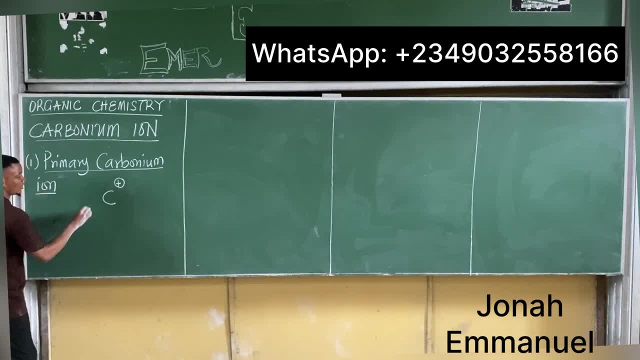 look up. please attach this to look up. please attach this to one archive. it becomes: look at this. it one archive. it becomes: look at this. it one archive. it becomes: look at this. it becomes this, becomes this, becomes this. um. the least attachment i can have is ch3. 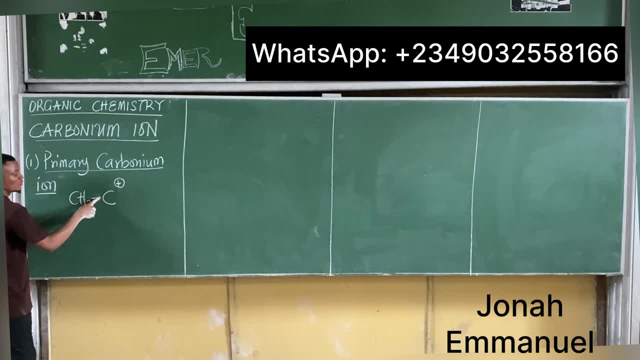 um, the least attachment i can have is ch3? um, the least attachment i can have is ch3. so attach ch3 here. so this man has one, so attach ch3 here. so this man has one, so attach ch3 here. so this man has one two. 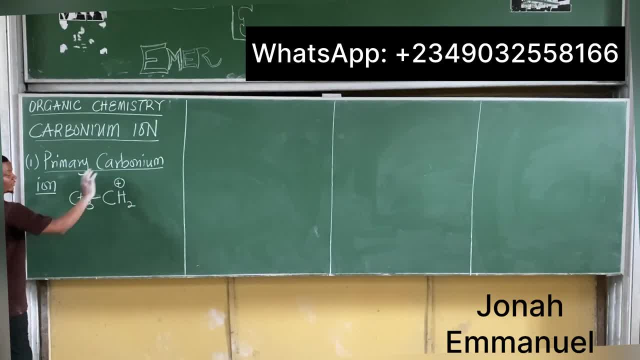 two. two h2 makes it four. this is a primary h2 makes it four. this is a primary h2 makes it four. this is a primary carbonium ion: carbonium ion, carbonium ion. why the carbon? why the carbon? why the carbon bearing the plus sign, let me bring it. 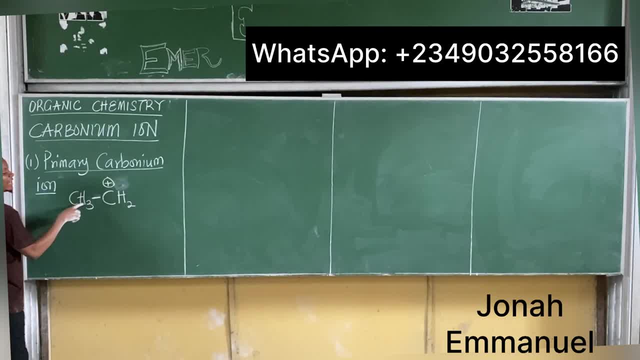 bearing the plus sign. let me bring it. bearing the plus sign. let me bring it here here. here is attached to just one archive group. here is attached to just one archive group. here is attached to just one archive group. and then this: so look at my balancing. and then this: so look at my balancing. 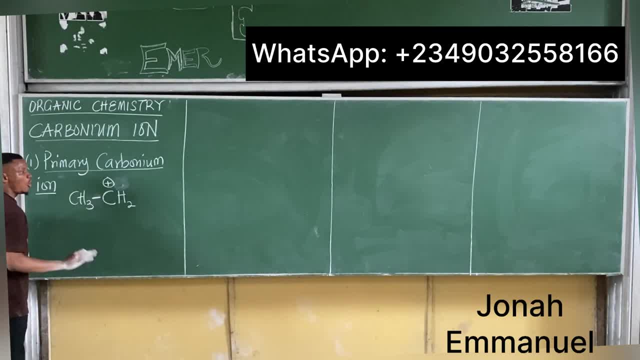 and then this: so look at my balancing. see here one, two, three, four. and we said: see here one, two, three, four. and we said: see here one, two, three, four. and we said: all just hydrogen if it is just hydrogen, all just hydrogen if it is just hydrogen. 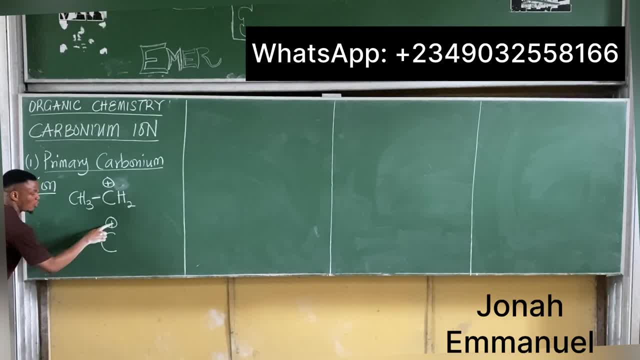 all just hydrogen. if it is just hydrogen, be be be carbonium ion having the plus sign. this is carbonium ion having the plus sign. this is carbonium ion having the plus sign. this is one. i think it was there one. i think it was there one, i think it was there- ch3. so see how this balances. 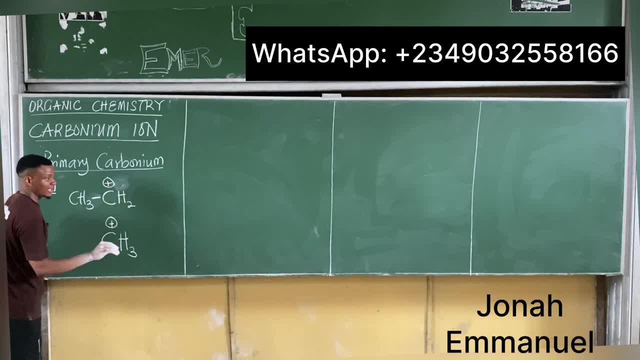 ch3. so see how this balances. ch3. so see how this balances. i'll tell you how this affects naming. i'll tell you how this affects naming. i'll tell you how this affects naming. of compound much more later, but please. of compound, much more later, but please. 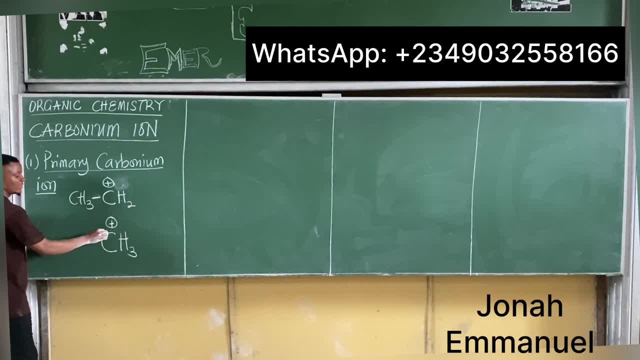 of compound much more later, but please notice, this is called a primary notice. this is called a primary notice. this is called a primary carbonium ion because this carbon is carbonium ion, because this carbon is carbonium ion, because this carbon is having having having just hydrogen, or perhaps it's attached. 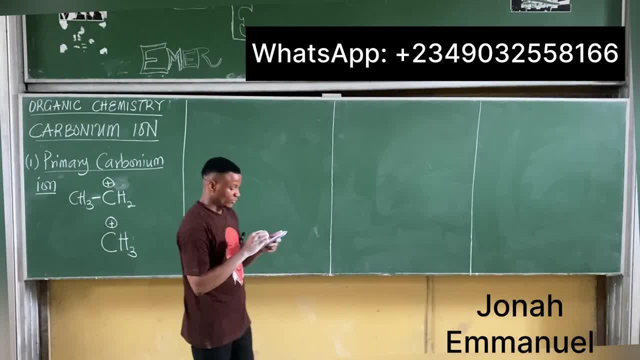 just hydrogen, or perhaps it's attached, just hydrogen, or perhaps it's attached to just one archive, to just one archive, to just one archive. so that's the example, just keep it. so that's the example, just keep it. so that's the example, just keep it pending. i'll show you. 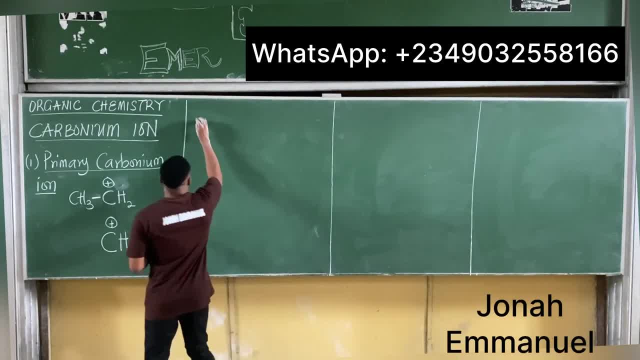 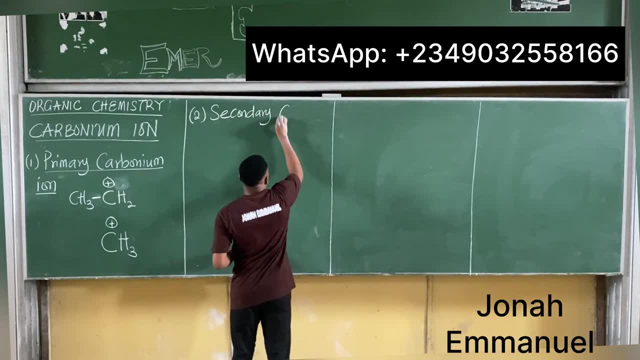 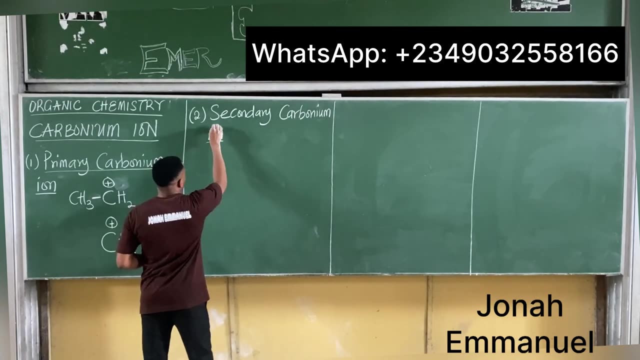 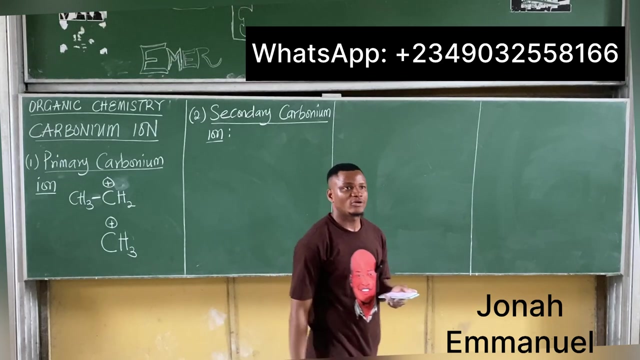 pending, i'll show you, pending, i'll show you. more things there, more things there, more things there. let's do secondary, let's do secondary, let's do secondary. carbonium ion, carbonium ion, carbonium ion: here the carbon which carries the. here the carbon which carries the. 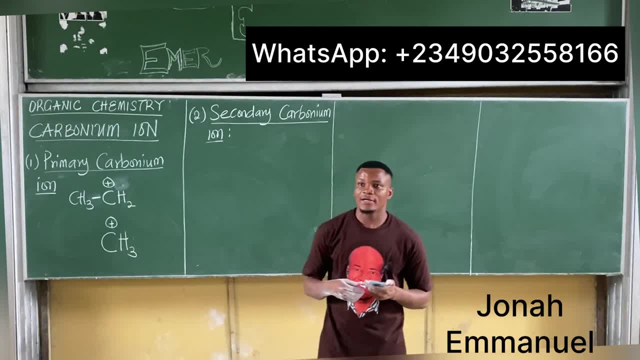 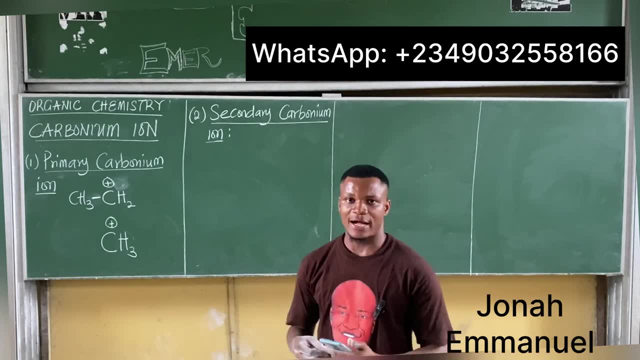 here the carbon which carries the positive charge. positive charge. positive charge. here the carbon which carries the. here the carbon which carries the. here the carbon which carries the positive charge. positive charge. positive charge. is attached to two. is attached to two. is attached to two. archive group. archive group. 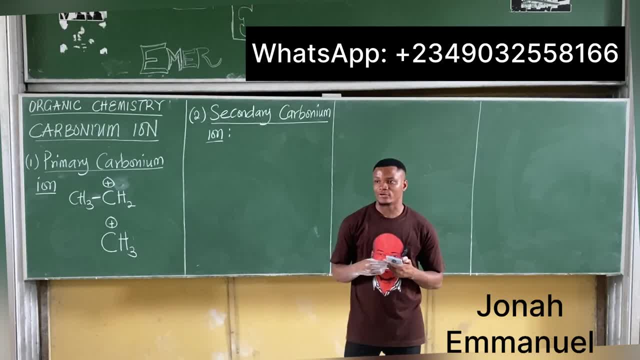 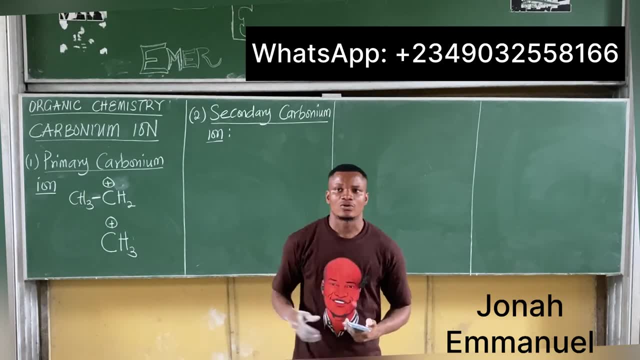 archive group is attached to. two is attached to. two is attached to two archive group: archive group. archive group is attached to. two is attached to. two is attached to two archive group, archive group, archive group. so i'll do this one on my, i'll just. so. i'll do this one on my, i'll just. 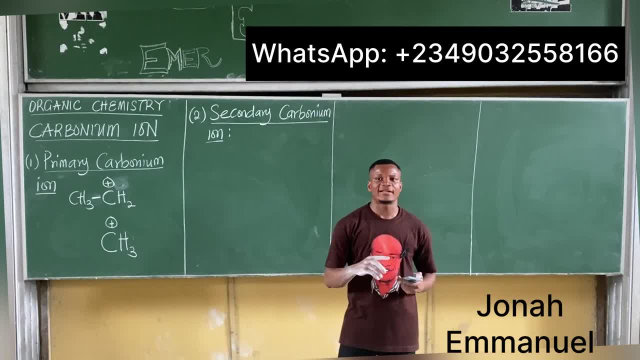 so i'll do this one on my i'll just show you how this one is done. show you how this one is done, show you how this one is done, and then you go, do you define tertiary. and then you go, do you define tertiary. and then you go, do you define tertiary and give out the example. 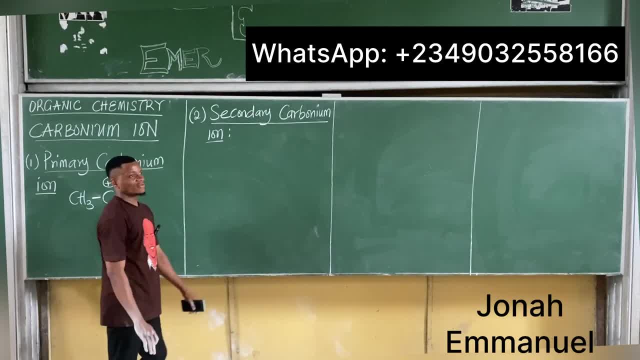 and give out the example. and give out the example. so look up, please look up, how is this? so look up, please look up, how is this. so look up, please look up. how is this done? very simple, done, very simple, done, very simple. they'll give you a list of carbonium. 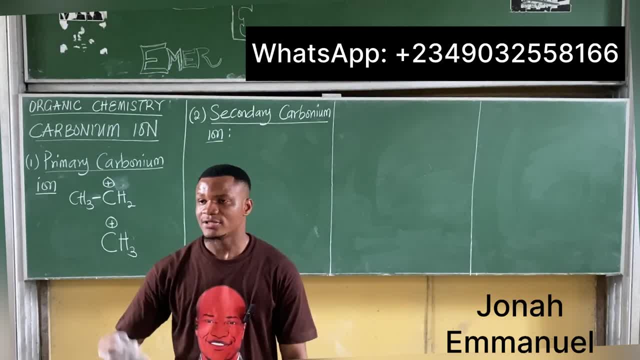 they'll give you a list of carbonium. they'll give you a list of carbonium ion. classify the following as primary ion: classify the following as primary ion: classify the following as primary, secondary or tertiary. for this one, it's secondary or tertiary. for this one, it's: 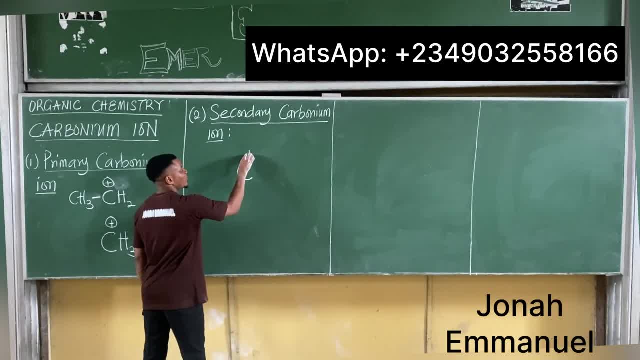 secondary or tertiary. for this one it's simple so first in space carbon. simple so, first in space carbon. simple so first in space carbon, bearing the plus sign, bearing the plus sign, bearing the plus sign. we said it's attached to two archive. we said it's attached to two archive. 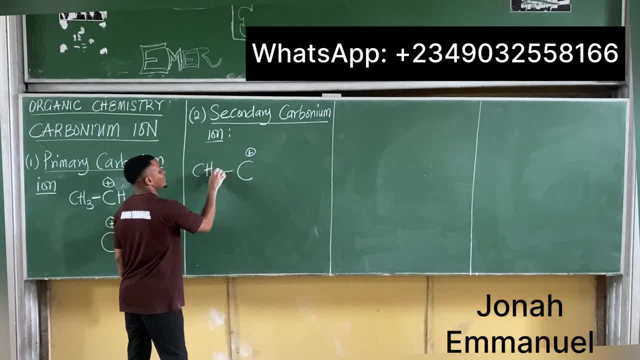 we said, it's attached to two archive group. the simplest of the archive group group, the simplest of the archive group group, the simplest of the archive group is ch3 metal is ch3 metal is ch3 metal. but perhaps we're using material too, but perhaps we're using material too. 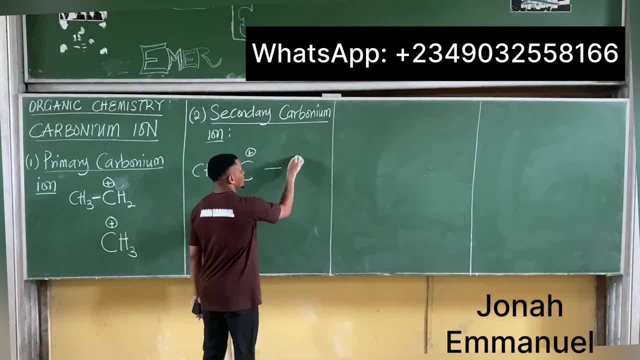 but perhaps we're using material too much so, let's now add something else. much so, let's now add something else. much so, let's now add something else. let's say profile c387- this one here. let's say profile c387- this one here. let's say profile c387, this one here becomes a secondary. 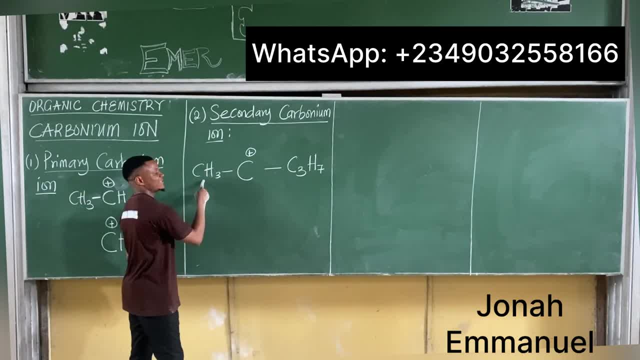 becomes a secondary, becomes a secondary carbonium ion, because this one is carbonium ion, because this one is carbonium ion, because this one is attached to two archive groups, attached to two archive groups, attached to two archive groups melted by the left and prepared by the, melted by the left and prepared by the. 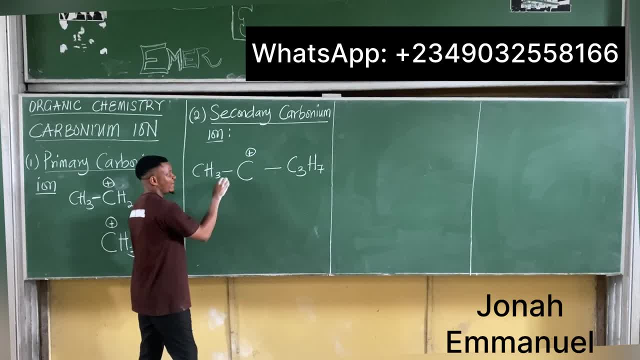 melted by the left and prepared by the right, right, right. obviously that this man is not balanced. obviously that this man is not balanced. obviously that this man is not balanced yet, yet, yet, i'm having one, two, three, one more h. i'm having one, two, three, one more h. 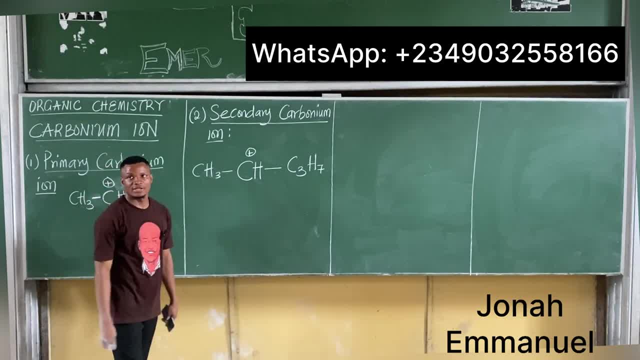 i'm having one, two, three, one more h that makes it four. so this one here is a that makes it four. so this one here is a that makes it four. so this one here is a secondary, secondary, secondary carbonium ion. please define tertiary on carbonium ion. please define tertiary on. 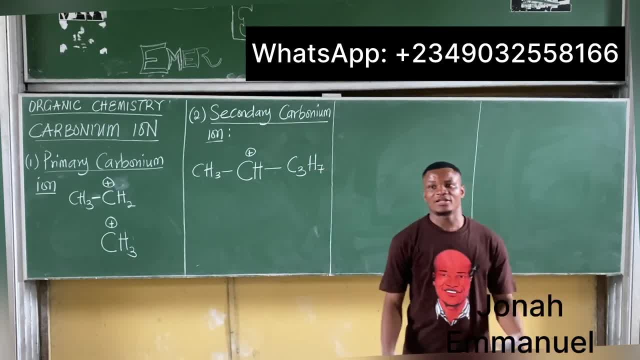 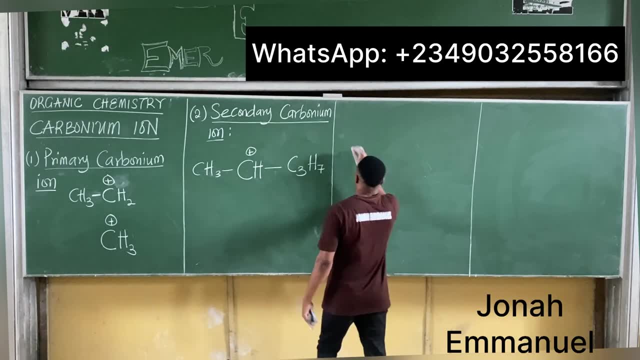 carbonium ion. please define tertiary on your own, your own, your own, and give an example. define tertiary on and give an example. define tertiary on and give an example. define tertiary on your own, your own, your own, and give an example. so the third one: there has to be tertiary. 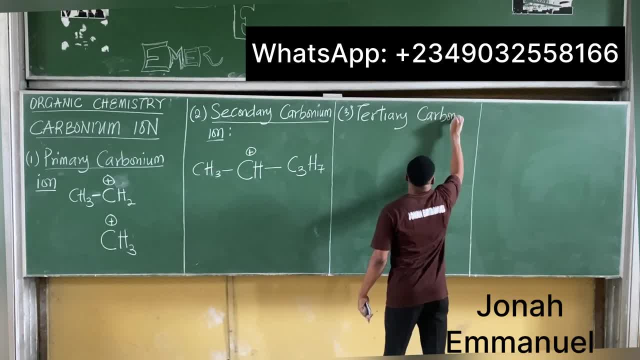 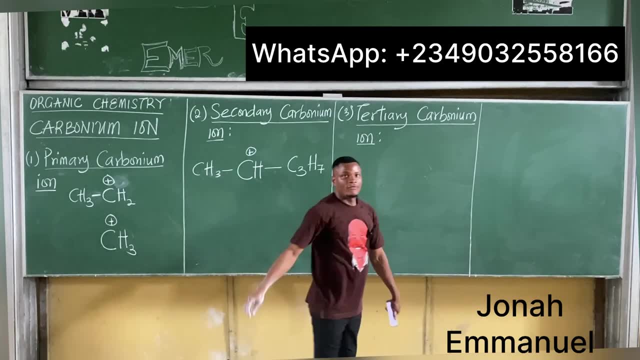 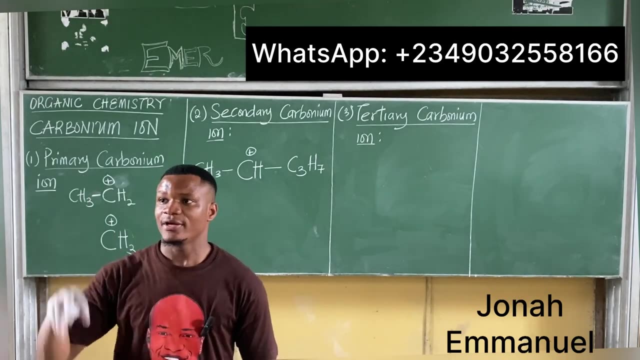 tertiary carbonium: carbonium ion. for a tertiary carbonium ion: the carbon for a tertiary carbonium ion: the carbon for a tertiary carbonium ion: the carbon bearing water. the plus sign is attached bearing water. the plus sign is attached bearing water. the plus sign is attached to water. three archive group. so it's as: 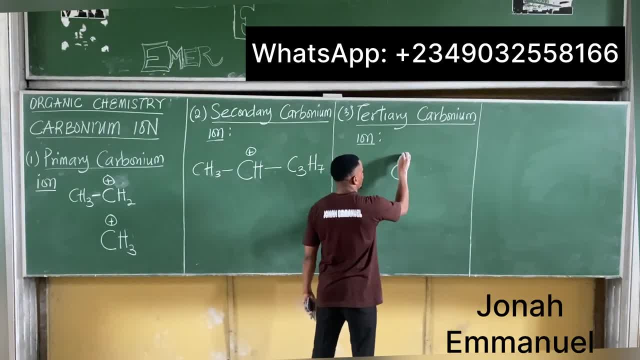 to water three archive group. so it's as to water three archive group. so it's as simple as this, simple as this. simple as this: becomes c there, having the plus sign becomes c there, having the plus sign becomes c there, having the plus sign, please the plus. i can still be here. 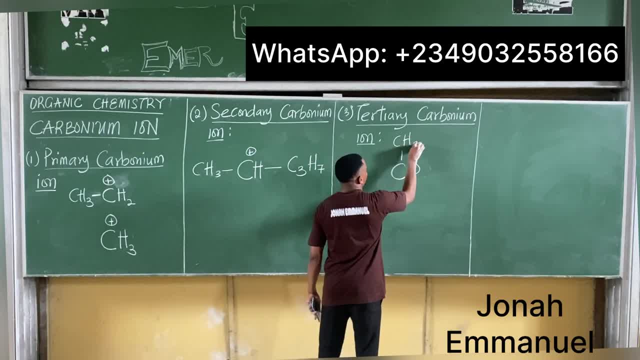 please, the plus i can still be here. please, the plus i can still be here. still okay, i now have my first archive. still okay, i now have my first archive. still okay, i now have my first archive. ch3, ch3, ch3- my second archive, group c2: 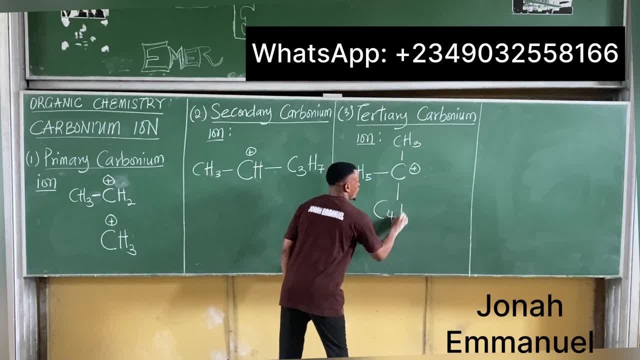 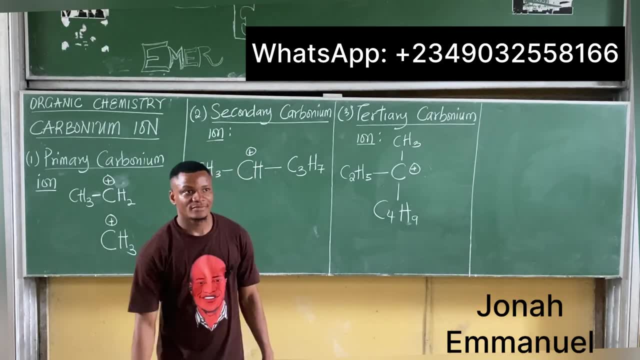 my second archive group, c2. my second archive group, c2- h5. my third archive is c4 h5. my third archive is c4- h5. my third archive is c4- h9- h9- h9 becomes a tertiary, becomes a tertiary, becomes a tertiary. carbonium ion. 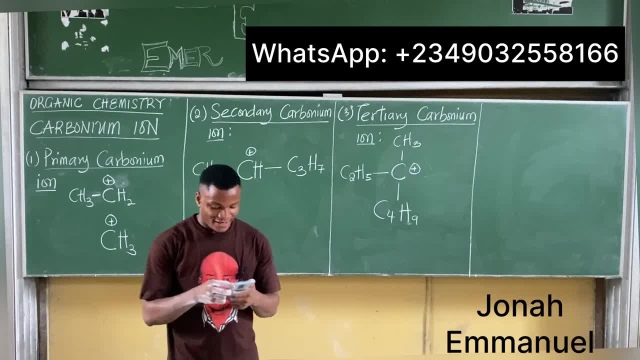 carbonium ion. carbonium ion becomes a tertiary, becomes a tertiary, becomes a tertiary- carbonium ion. carbonium ion. carbonium ion. let's see why we need this example. let's see why we need this example. let's see why we need this example. let's use this to do a fast question. let's use this to do a fast question. let's use this to do a fast question. so this is what should be happening. so this is what should be happening. so this is what should be happening. something like this, or even if you even something like this, or even if you even. 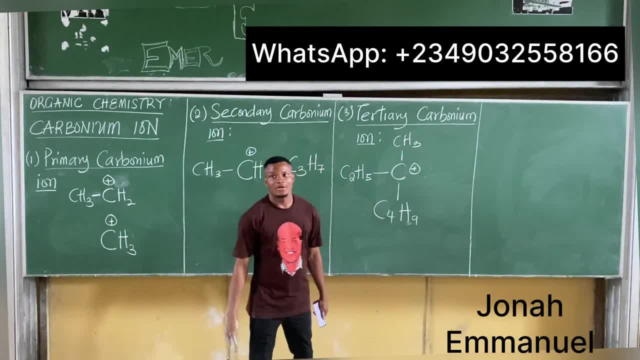 something like this: or even if you- even if you brought this one up here and this, if you brought this one up here and this, if you brought this one up here and this man here see, okay, man here see, okay, man here see okay- even if you use metal, metal material, 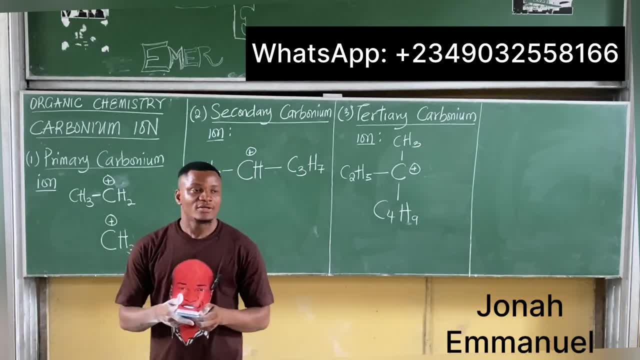 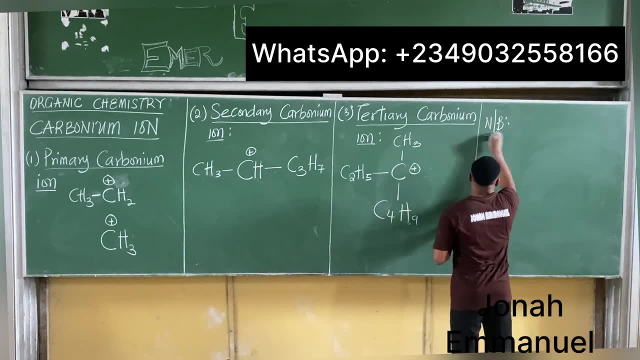 even if you use metal metal material. even if you use metal metal material, it's still okay, it's still okay. it's still okay. okay, all right, let's note something. okay, all right, let's note something. okay, all right, let's note something notes. let's note something, notes. 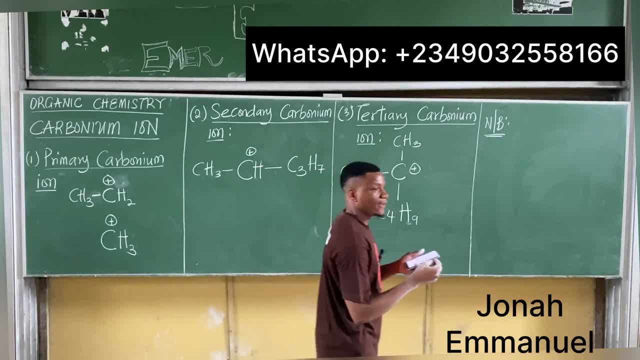 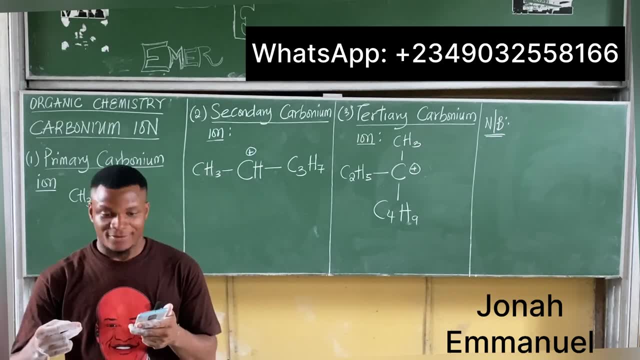 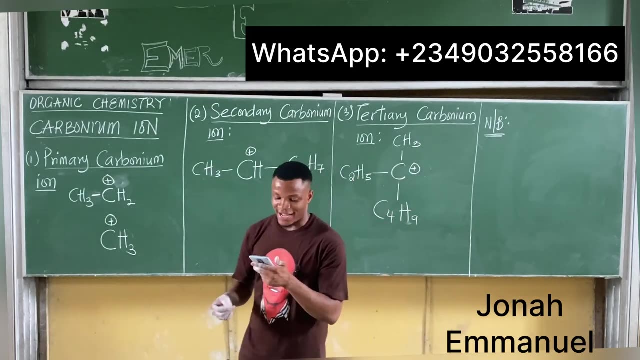 the hydrogen of the. the hydrogen of the. the hydrogen of the notes notes. notes, notes. is it break time? the hydrogen of the primary comma. the hydrogen of the primary comma. the hydrogen of the primary comma. secondary and tertiary carbonium ion. secondary and tertiary carbonium ion. secondary and tertiary carbonium ion. the hydrogens. 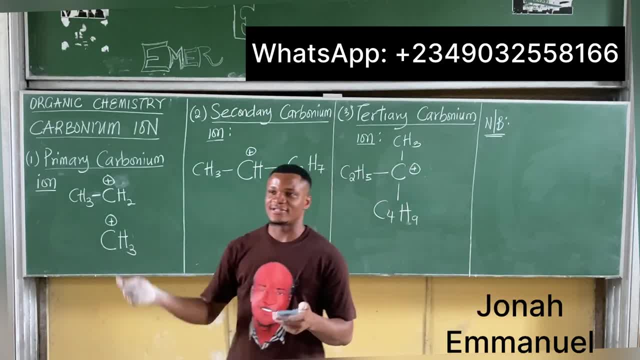 the hydrogens, the hydrogens. hydrogens or hydrogen. so use hydrogen or hydrogens or hydrogen. so use hydrogen or hydrogens or hydrogen. so use hydrogen or hydrogens. hydrogens- that's hydrogen in bracket s. that's hydrogen in bracket s. that's hydrogen in bracket s the hydrogen or hydrogens of the primary. 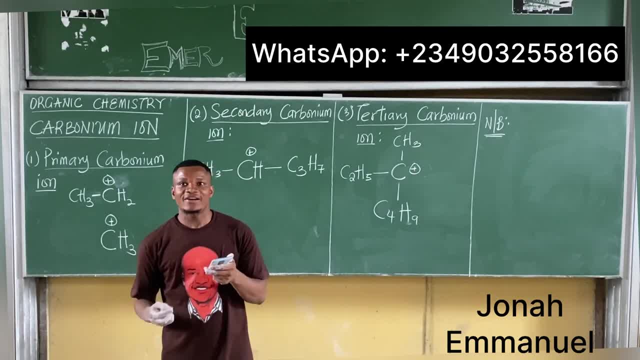 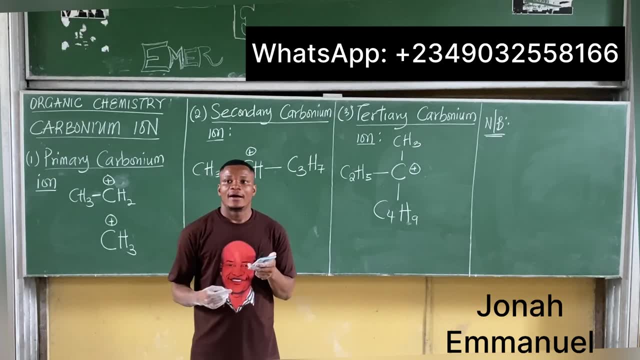 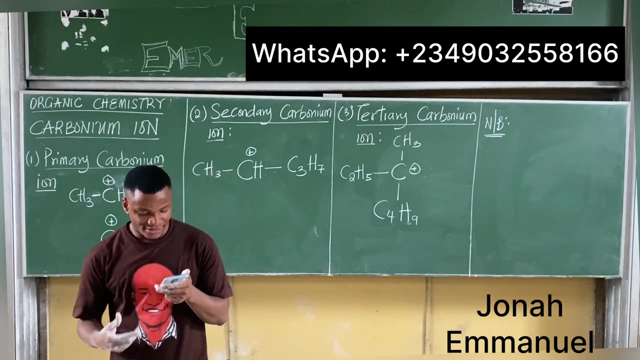 the hydrogen or hydrogens of the primary, the hydrogen or hydrogens of the primary comma, comma comma, secondary and secondary and secondary and tertiary carbonium ion. i refer to us. i refer to us primary comma, secondary and primary comma, secondary and primary comma, secondary and tertiary hydrogens respectively. 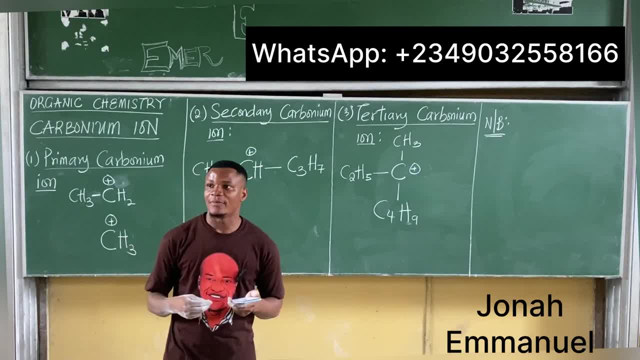 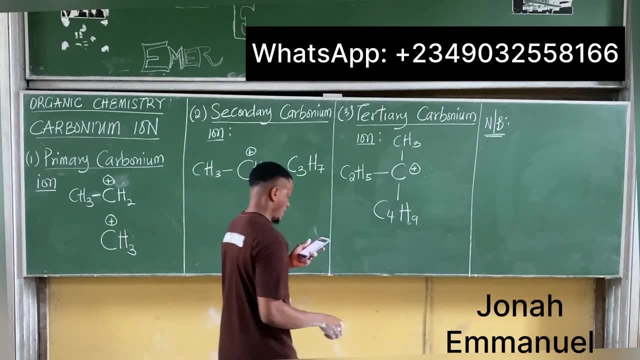 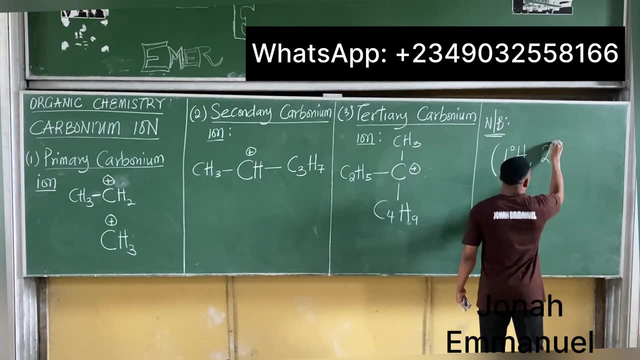 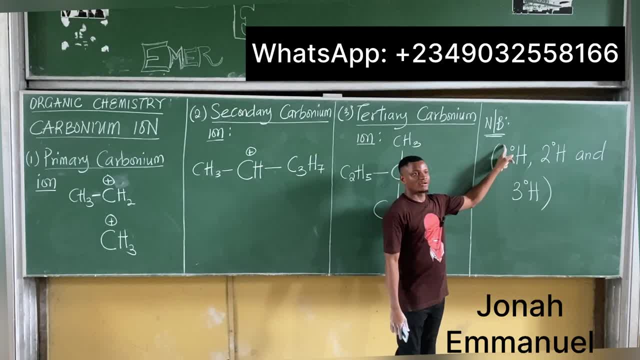 written. as written as so please. if you see this what you see, so please. if you see this what you see, so please. if you see this what you see. one, not one. not one not or one to preserve- this means primary, or one to preserve: this means primary. 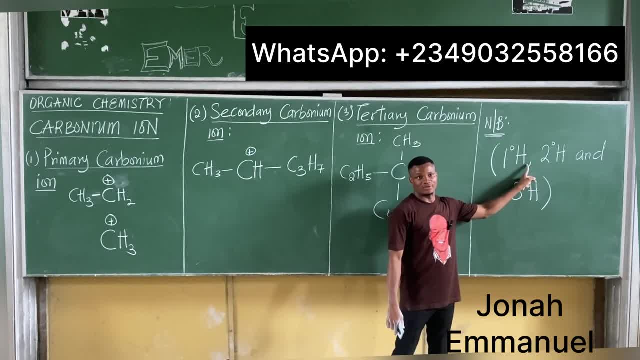 or one to preserve. this means primary. if you see this with a c, it means what? if you see this with a c, it means what? if you see this with a c, it means what? they're primary carbon. they're primary carbon, they're primary carbon. so what this means is primary, so not like. 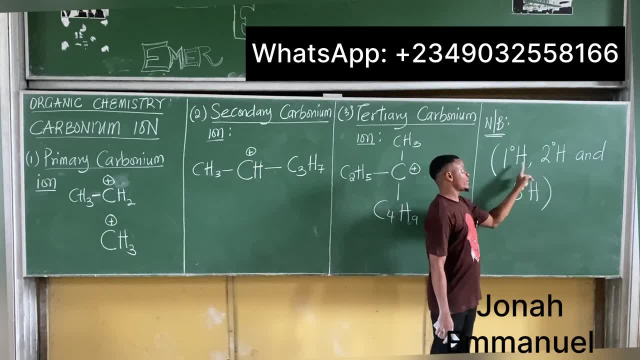 so what this means is primary, so not like. so what this means is primary, so not like. that means secondary. so that is hydrogen. that means secondary. so that is hydrogen. that means secondary. so that is hydrogen. or c. this means primary hydrogen, or c, this means primary hydrogen. 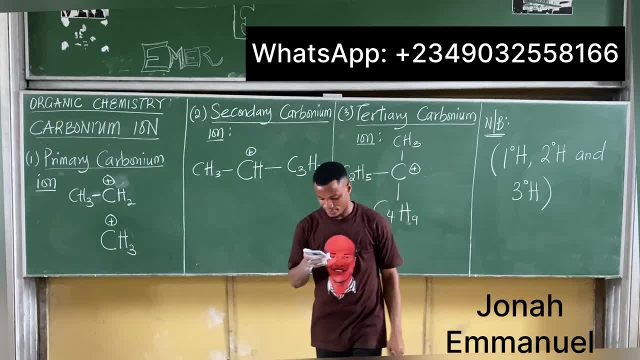 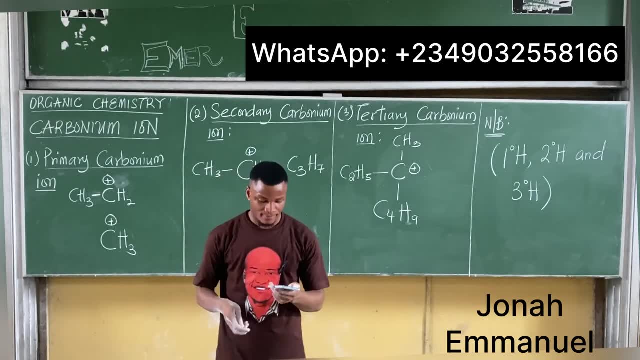 or c. this means primary hydrogen, secondary hydrogen, secondary hydrogen, secondary hydrogen, tertiary hydrogen, tertiary hydrogen, tertiary hydrogen. does this? who stop? let's take an example, please. who stop? let's take an example, please. who stop? let's take an example, please. all right, sample problem, please. all right, sample problem, please. 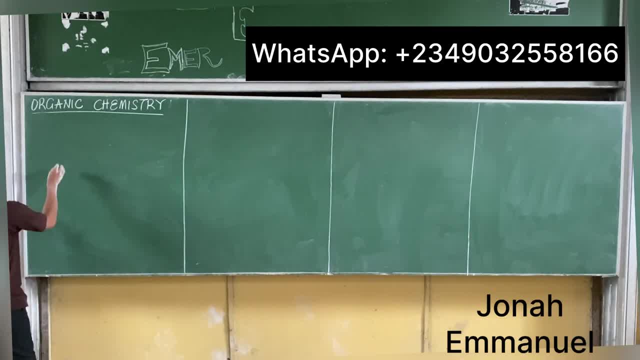 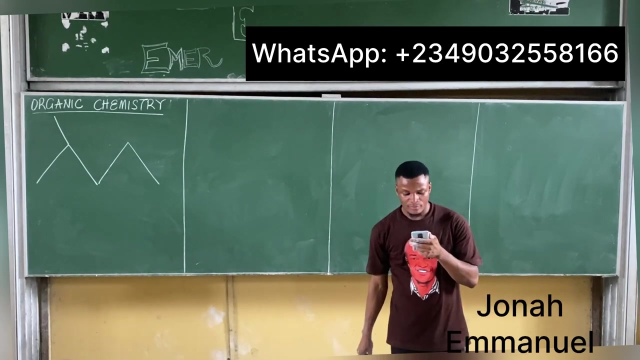 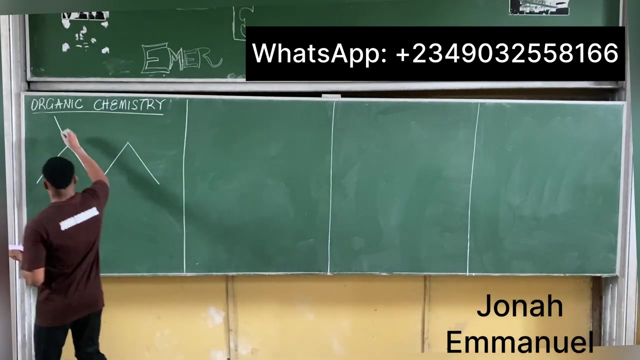 all right, sample problem, please. given the molecule below. given the molecule below. given the molecule below: all right, all right, all right. given the molecule below this. given the molecule below, you have this. so, given the molecule below, you have this. so, given the molecule below, you have this. so this molecule here. 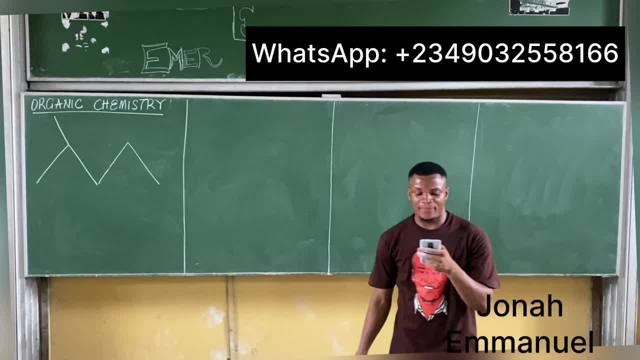 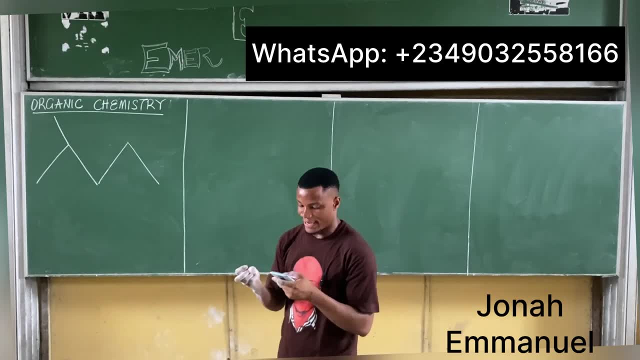 this molecule here? this molecule here: how many primary, secondary and tertiary? how many primary, secondary and tertiary? how many primary, secondary and tertiary carbon atoms, carbon atoms, carbon atoms: how many primary, secondary and tertiary? how many primary, secondary and tertiary? how many primary, secondary and tertiary carbon atoms are present? 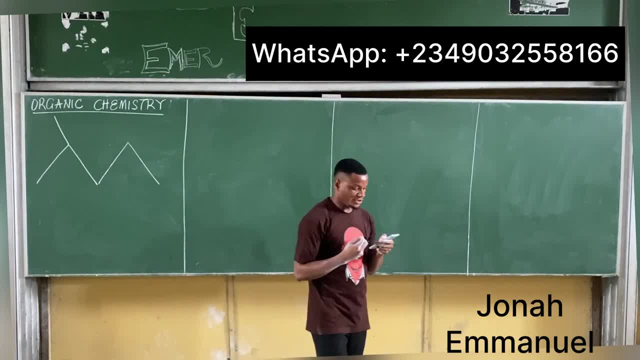 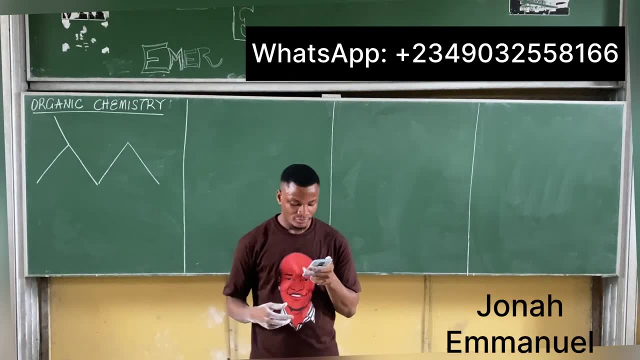 carbon atoms are present. carbon atoms are present in the molecule. how many primary in the molecule? how many primary in the molecule? how many primary, secondary and tertiary, secondary and tertiary, secondary and tertiary carbon atoms are present? carbon atoms are present. carbon atoms are present in the molecule, in the molecule? 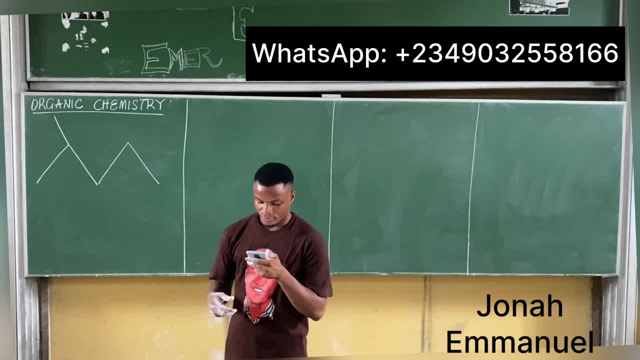 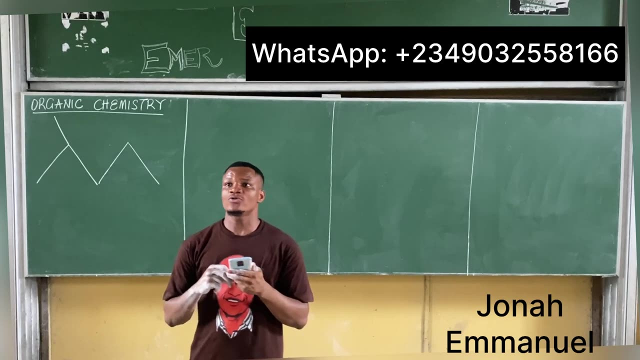 in the molecule. also find out the number of primary. also find out the number of primary. also find out the number of primary, secondary and tertiary hydrogen present. secondary and tertiary hydrogen present. secondary and tertiary hydrogen present. also find out the number of primary. also find out the number of primary. 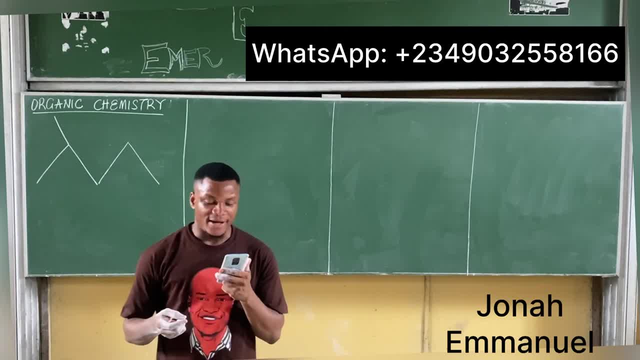 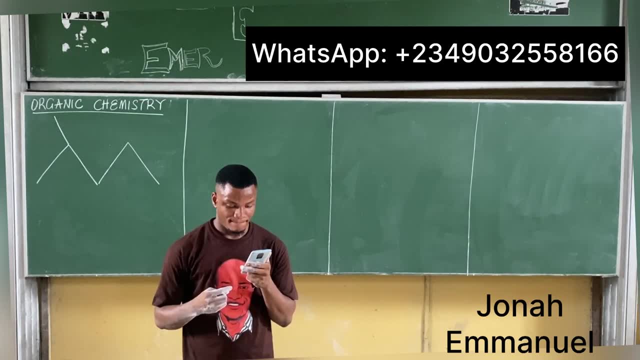 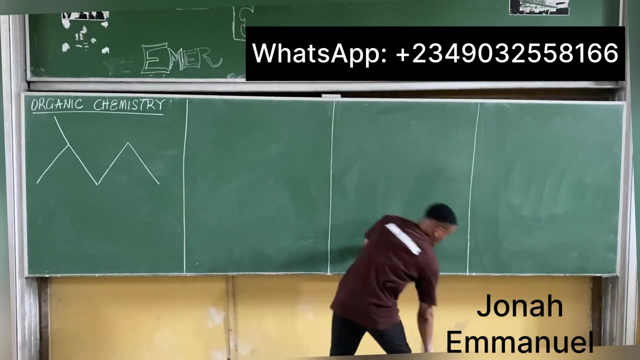 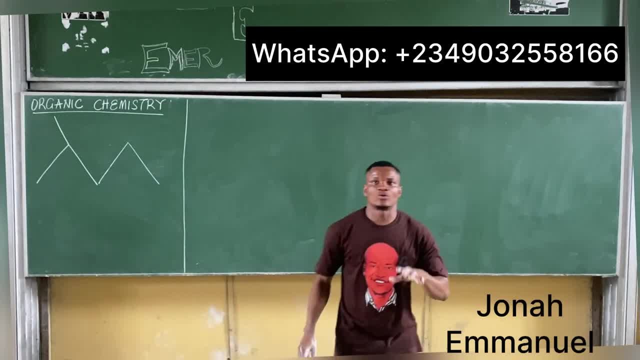 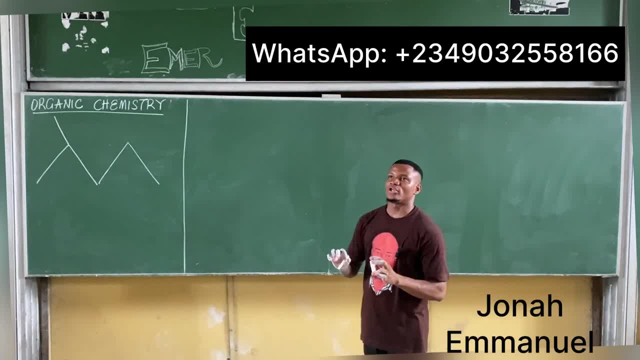 when it comes to doing this, um, when it comes to doing this, when it comes to doing this, um, when it comes to doing this, your best bet comes to doing this. your best bet comes to doing this. your best bet, your best bet would be, your best bet would be: 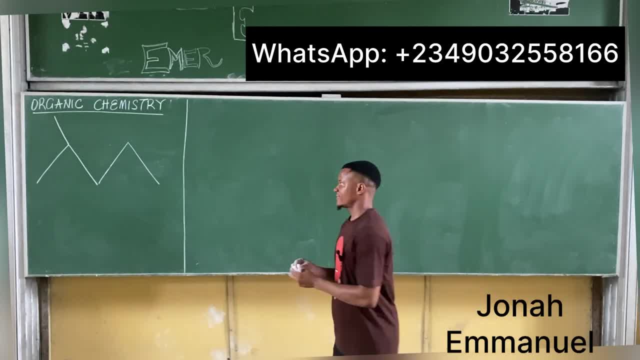 your best bet would be: try to draw out the complete structure. try to draw out the complete structure. try to draw out the complete structure. so, first things first. i'm having so, first things first. i'm having so first things first. i'm having one, two, three, four, five. so 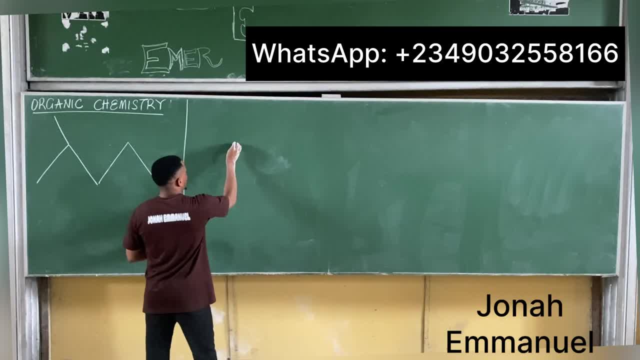 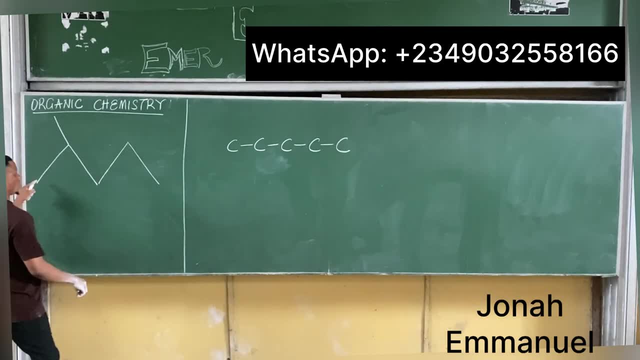 one, two, three, four, five. so one, two, three, four, five. so one, uh, excuse me, one, two, one, two, one, two, three, four, three, four, three, four, five. observe that this is carbon one, five. observe that this is carbon one, five. observe that this is carbon one, two, carbon two. i have this one here. what's? 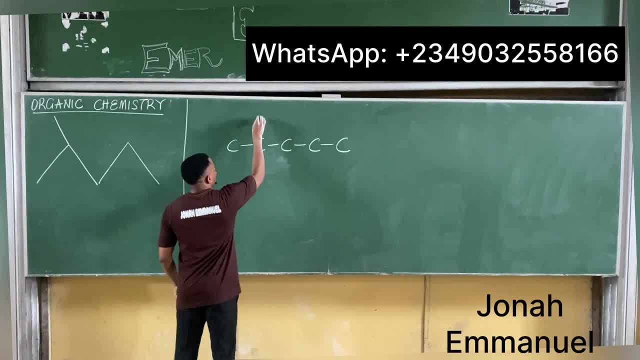 two, carbon two. i have this one here. what's two? carbon two. i have this one here. what's this? this, this, so carbon two. i'm adding, so carbon two. i'm adding, so carbon two. i'm adding ch3, ch3- ch3 as a material, as a material. 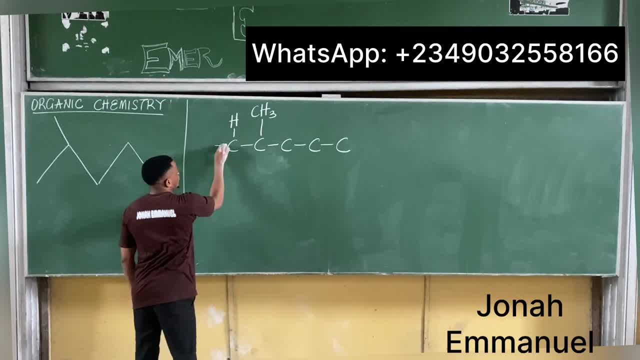 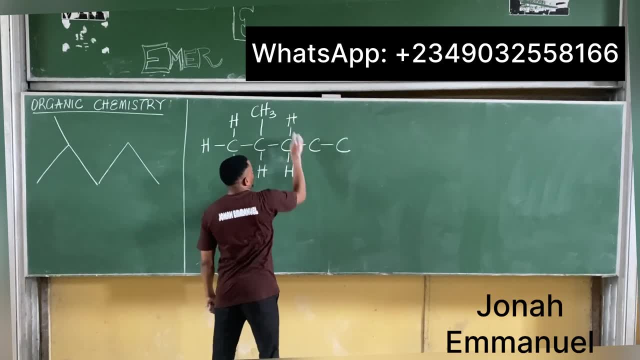 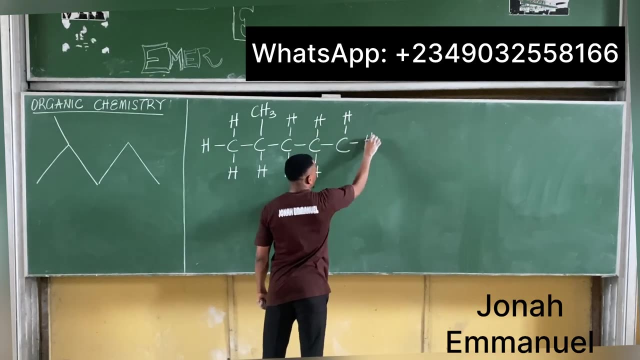 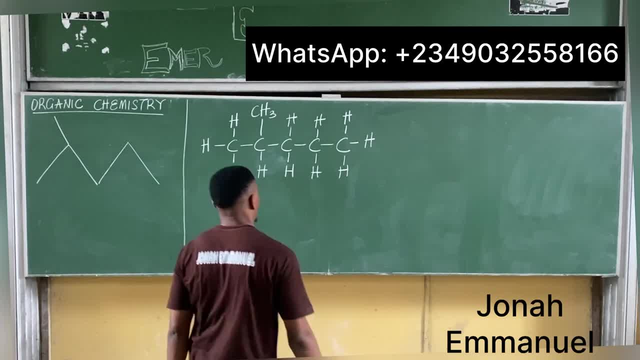 four. all right, so i have four. all right, so i have a complete structure here, a complete structure here, a complete structure here. okay, so i have this now. okay, so, i have this now. okay, so i have this now. we are, we are, we are actually identifying for each of them. 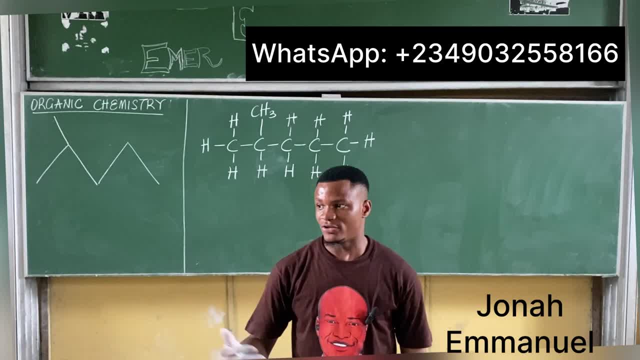 actually identifying for each of them, actually identifying for each of them. identify each of the carbon here as a identify each of the carbon here as a. identify each of the carbon here as a primary, primary, primary, a secondary and a tertiary- my first, a secondary and a tertiary: my first. 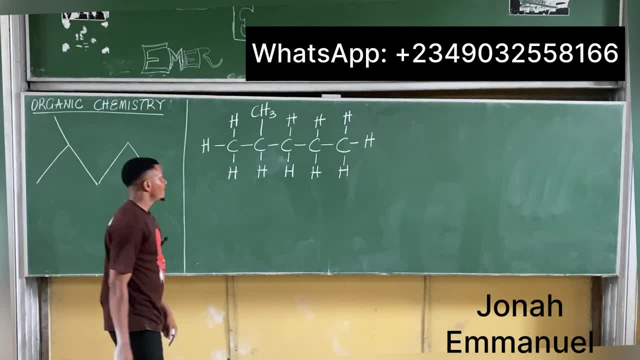 a secondary and a tertiary. my first step should now be step, should now be step, should now be: label each of them, label each of them, label each of them. uh, so let me call here, uh, so, let me call here, uh, so let me call here: a b. 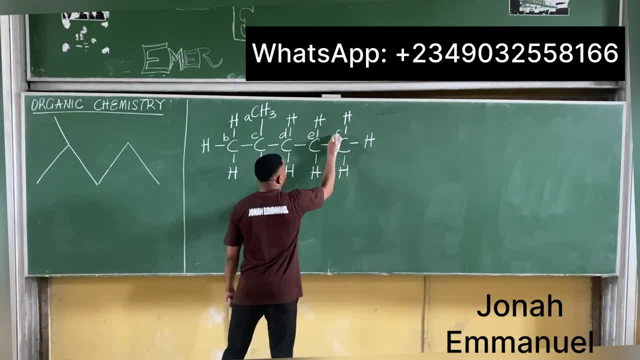 a, b, a, b, c, d, e, c, d e, c, d e and f. so i'm labeling this, i'm labeling and f. so i'm labeling this, i'm labeling and f. so i'm labeling this. i'm labeling this: a, b, c, d, e and f. 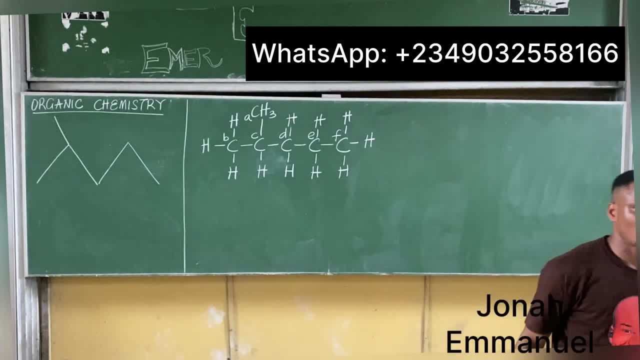 a, b, c, d, e and f. so i'm labeling this. i'm labeling this: a, b, c, d, e and f. so carbon: a primary or carbon, a primary or carbon, a primary or secondary, b primary secondary, c primary secondary b primary secondary, c. primary secondary b. primary secondary, c primary secondary, d e f. 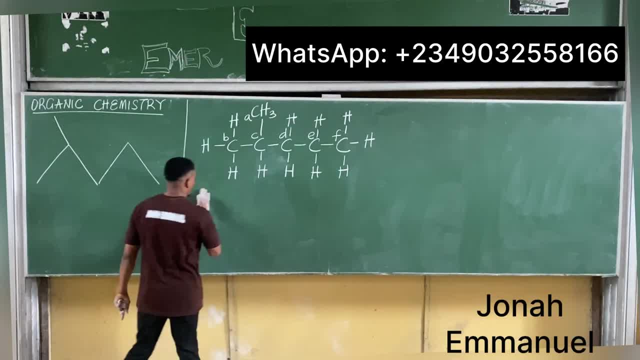 secondary d e f. secondary d e f. what do we have? so it's simple, um. what do we have? so it's simple, um. what do we have? so it's simple, um. first things first, first things first, first things first. let's get which of them are. 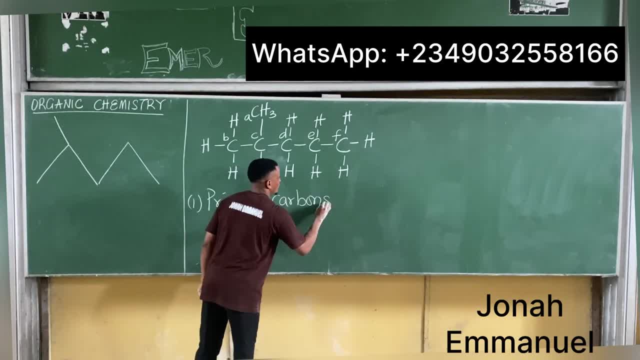 let's get which of them are. let's get which of them are: primary, primary, primary carbons, carbons, carbons. what's the idea of primary carbons? what's the idea of primary carbons? what's the idea of primary carbons? primary carbons are simply carbons that. 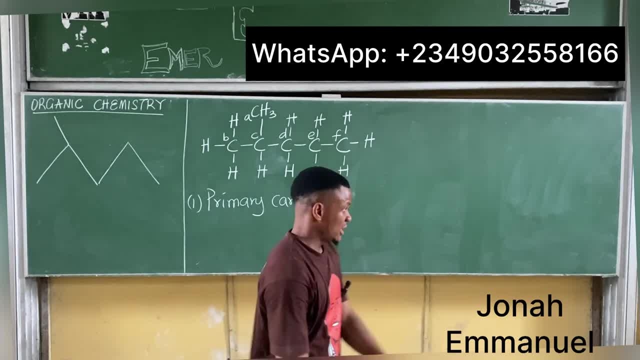 primary carbons are simply carbons. that primary carbons are simply carbons that have one there, one archive group attached. have one there, one archive group attached. have one there, one archive group attached to them. if i look at this to them, if i look at this: 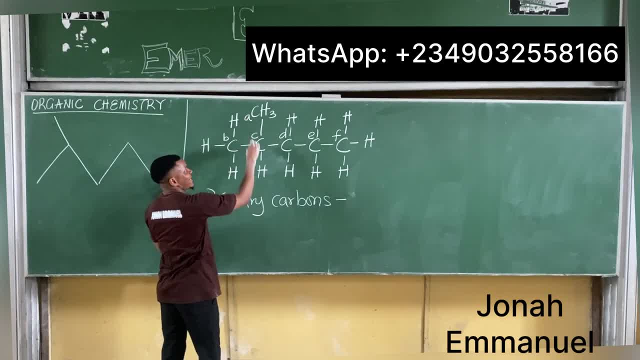 to them. if i look at this, look at carbon a. look at carbon a. look at carbon a. carbon a is attached to just this one here. carbon a is attached to just this one here. carbon a is attached to just this one here. this archive group, please observe. 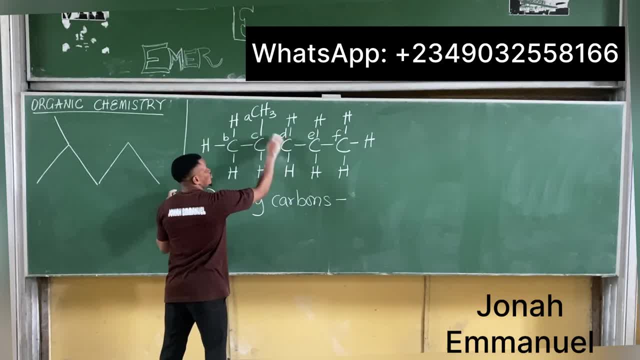 this archive group. please observe this archive group. please observe carbon a. here is attached to just this carbon a. here is attached to just this carbon a. here is attached to just this archive group. so carbon a becomes archive group. so carbon a becomes archive group. so carbon a becomes a primary carbon. 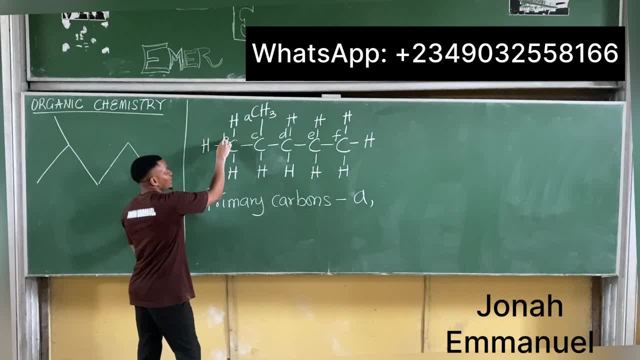 a primary carbon, a primary carbon. hold on, hold on, hold on also. observe carbon b. also observe carbon b. also observe carbon b. carbon b have one, two, three, three. carbon b have one, two, three, three. carbon b have one, two, three, three. attachments please, attachments, please, attachments, please. look at carbon b. this carbon here has 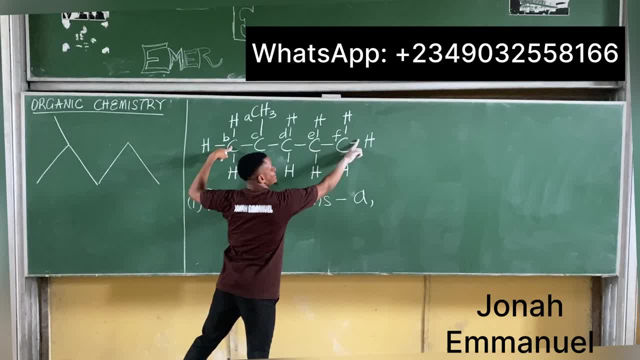 look at carbon b, this carbon here has. look at carbon b: this carbon here has just one, two, three hydrogen, and then all just one, two, three hydrogen, and then all just one, two, three hydrogen, and then all of this, of this, of this, so carbon b, so carbon b. 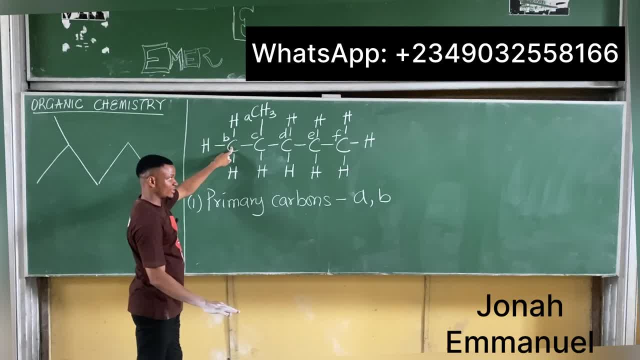 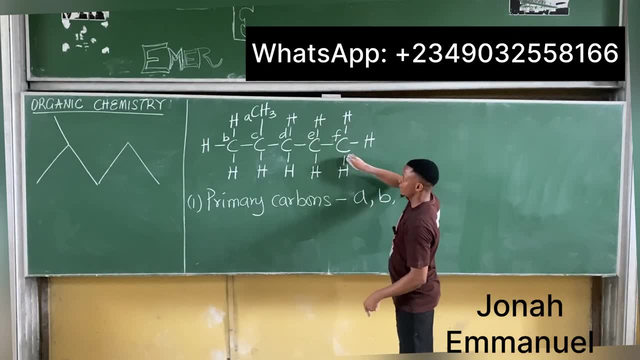 so carbon b is a primary, is a primary, is a primary carbon. carbon carbon. hold on, still, hold on, still, hold on, still. what about carbon c or carbon f? what about carbon c or carbon f? what about carbon c or carbon f? observe that carbon f is just one, two, three. 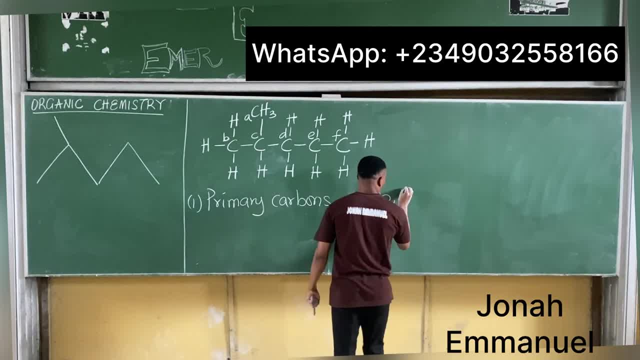 observe that carbon f is just one, two, three. observe that carbon f is just one, two, three, and then all of this attached to this, and then all of this attached to this, and then all of this attached to this carbon. here, f is also a primary carbon in. 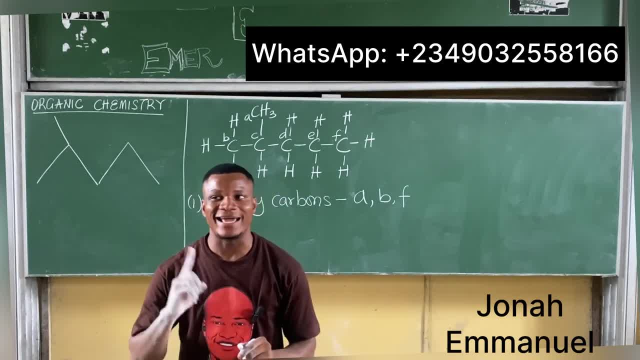 carbon. here f is also a primary carbon in carbon. here f is also a primary carbon in quotes: primary carbons are always carbons. quotes: primary carbons are always carbons. quotes: primary carbons are always carbons. at the extreme, don't forget that. at the extreme, don't forget that. 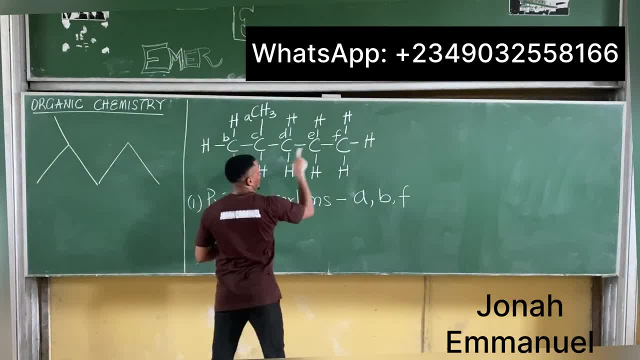 at the extreme. don't forget that primary carbons are always carbons at the primary carbons are always carbons at the primary carbons are always carbons at the extreme. at the extreme will always be extreme at the extreme will always be extreme at the extreme will always be a primary. 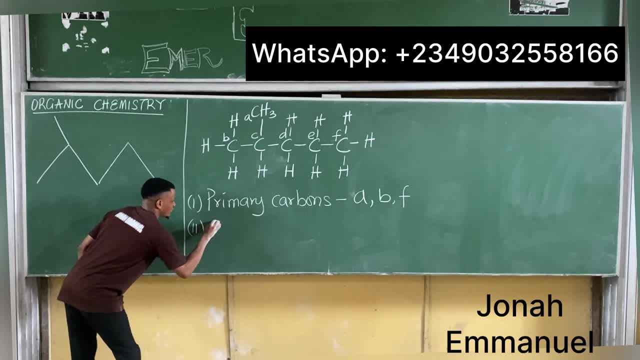 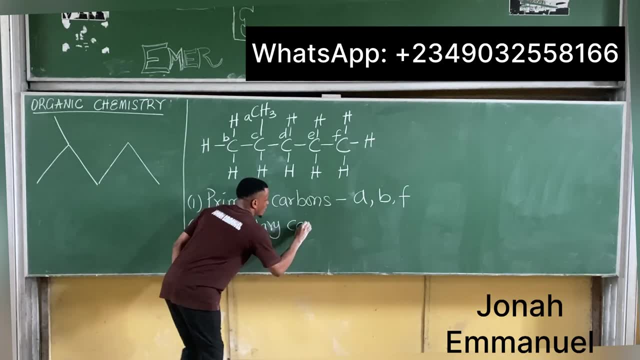 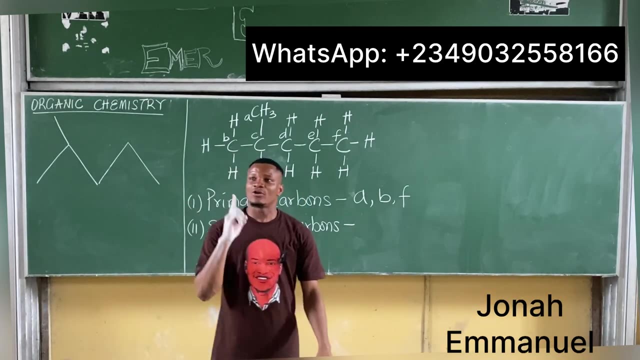 a primary, a primary carbon, carbon carbon. all right, let's try secondary, secondary carbons, carbons, carbons, carbons for secondary carbons. which do we look for? secondary carbons, which do we look for? secondary carbons, which do we look at? now listen, the idea about secondary is: 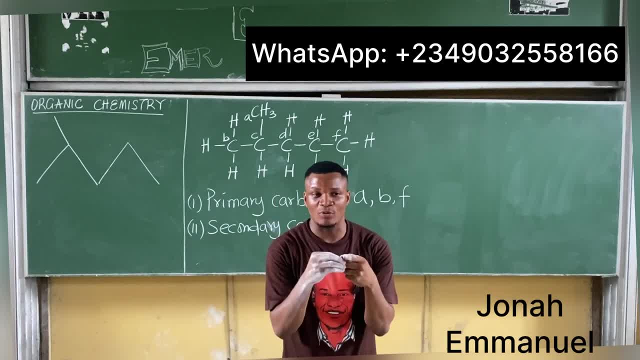 at now listen. the idea about secondary is at now listen. the idea about secondary is that what happens there now two, that what happens there now two, that what happens there now two. archive group would rather attach to it. archive group would rather attach to it. archive group would rather attach to it. which of them here has two archives? 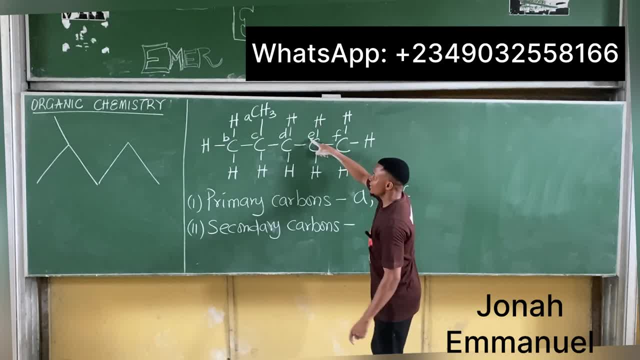 which of them here has two archives? which of them here has two archives attached to it? attached to it. attached to it. look at e. e has this one as an attachment. look at e. e has this one as an attachment. look at e. e has this one as an attachment and also this one as an attachment, so e. 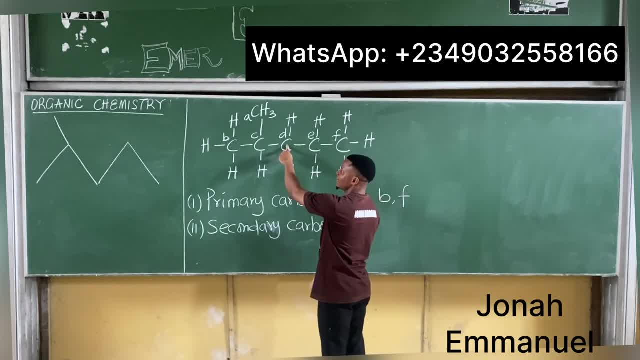 and also this one as an attachment. so e and also this one as an attachment. so e is what the secondary is, what the secondary is, what the secondary look at d d has all of this as an look at. d d has all of this as an look at d d has all of this as an attachment on one side. 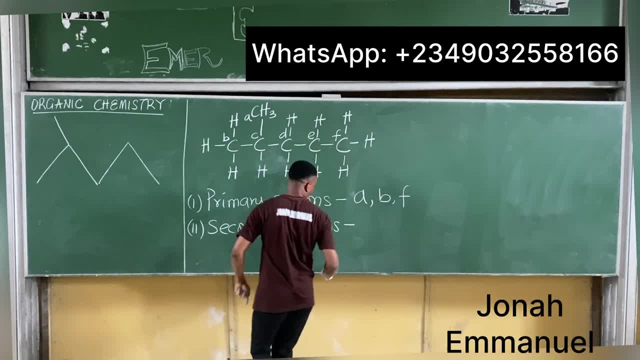 attachment on one side. attachment on one side. d also has all of this as an attachment. d also has all of this as an attachment. d also has all of this as an attachment. so therefore, carbon d and e are both. so therefore, carbon d and e are both. 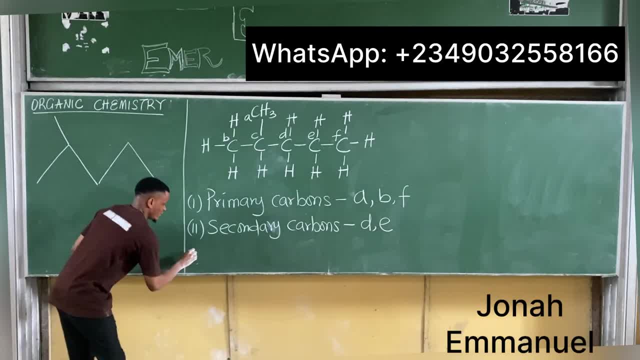 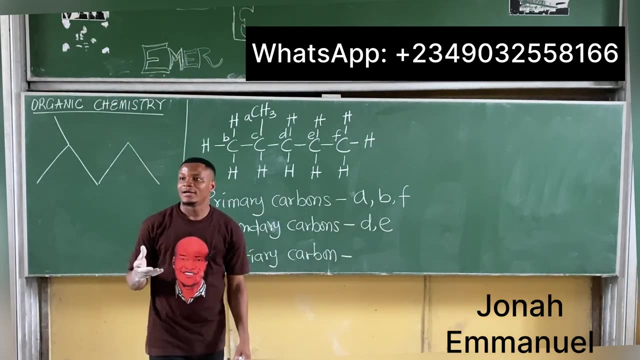 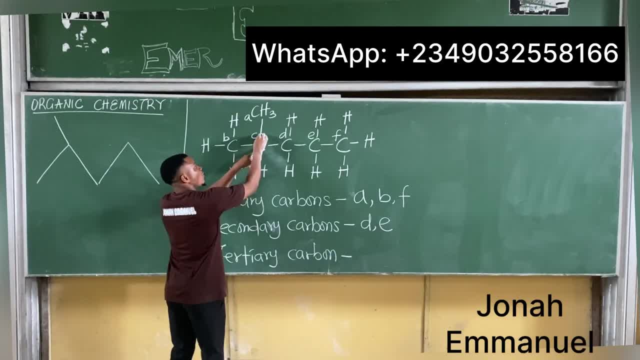 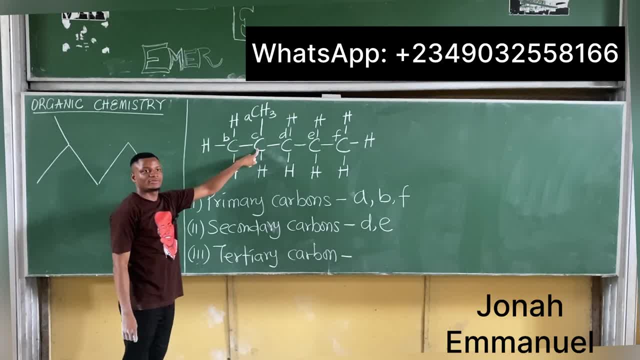 attachments. see how to get there three attachments. see how to get there three attachments, because we're there, attachments, because we're there, attachments, because we're there. it's tertiary carbon, that's it. it's tertiary carbon, that's it. it's tertiary carbon, that's it. so carbon c: 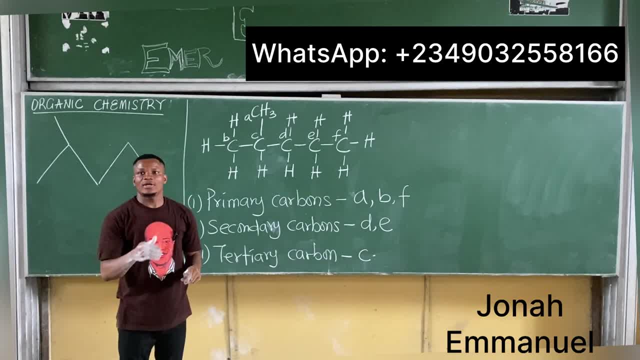 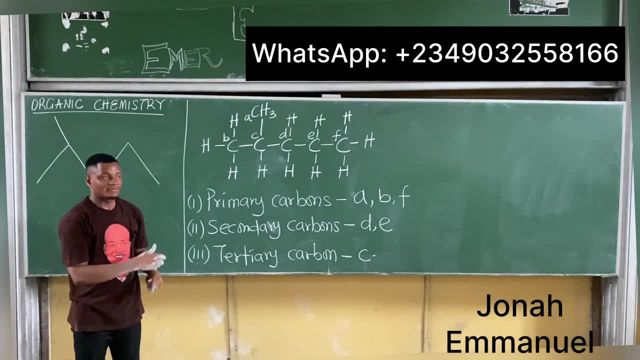 so carbon c. so carbon c is tertiary. do we get this? or should i give you a? do we get this? or should i give you a? do we get this? or should i give you a note, note, note, let me know, let me know, let me know, do you get this? 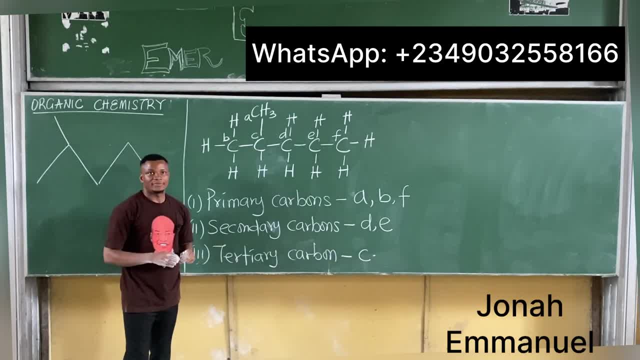 do you get this? do you get this? so it's simple, look up, so it's simple, look up, so it's simple. look up by one again. look up by one again. look up by one again. look up. let's say don't buy if you look up. 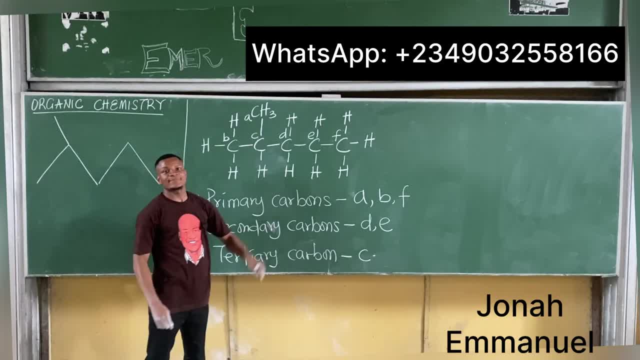 let's say: don't buy if you look up. let's say: don't buy if you look up. let's say: look up one by one, so classify. let's say: look up one by one, so classify. let's say: look up one by one, so classify the following as primary, secondary or. 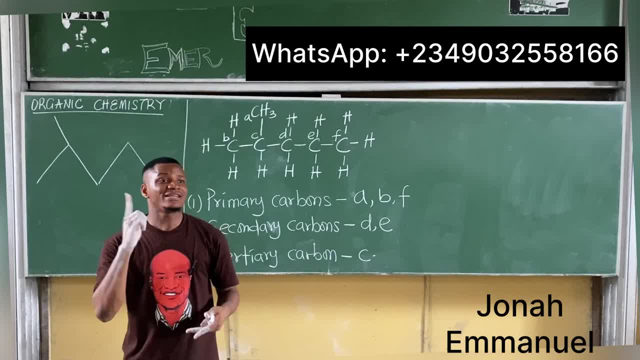 the following as primary, secondary or the following as primary, secondary or tertiary is simple. look at how many tertiary is simple. look at how many tertiary is simple. look at how many archive in the attachment is archive. archive in the attachment is archive. archive in the attachment is archive attachment, not hydrogen. 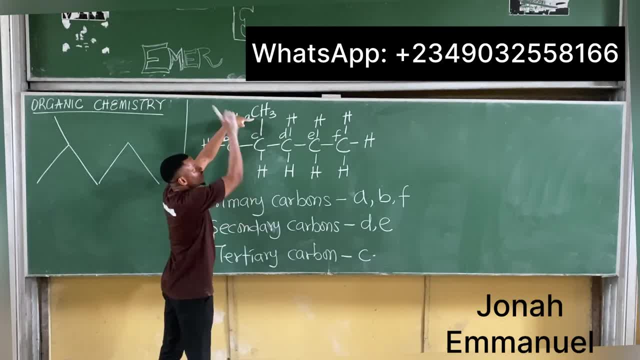 attachment, not hydrogen. attachment, not hydrogen. start with a here's carbon a here. this start with a here's carbon a here. this start with a here's carbon a here. this man here has only one attachment. this man here has only one attachment. this man here has only one attachment, this one coming down. 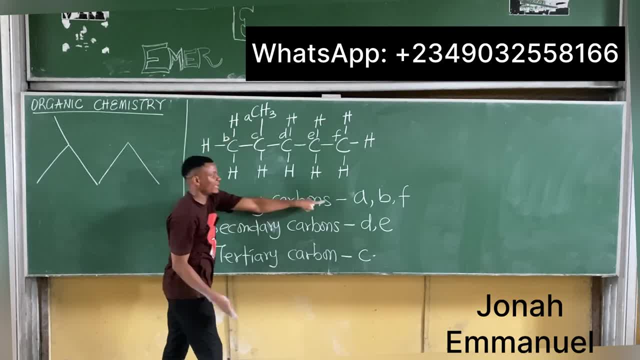 one coming down, one coming down, this one's about hydrogen. so because of this one's about hydrogen, so because of this one's about hydrogen, so because of their primary a, that's all their primary a, that's all their primary a, that's all come to. b. b has just one attachment. these 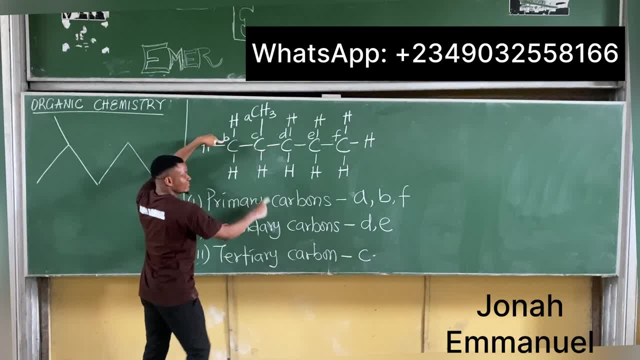 come to b. b has just one attachment. these come to b. b has just one attachment. these ones are hydrogen, they don't count. ones are hydrogen, they don't count. ones are hydrogen, they don't count. so it's just one attachment b. so it's just one attachment b. 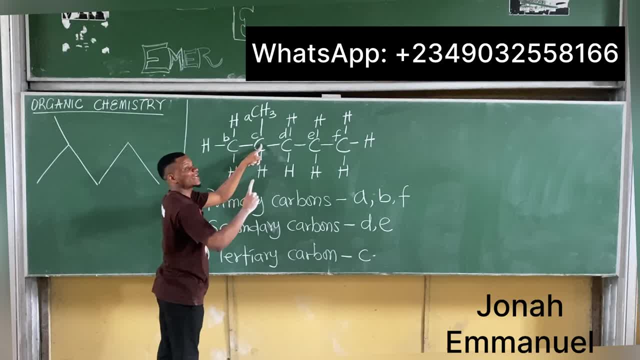 so it's just one. attachment b is primary, come to c. c has three is primary. come to c. c has three is primary, come to c. c has three attachments, attachments. attachments: aside the hydrogen, so i said hydrogen, aside the hydrogen, so i said hydrogen aside the hydrogen, so i said hydrogen here. c has one, two and three, so it. 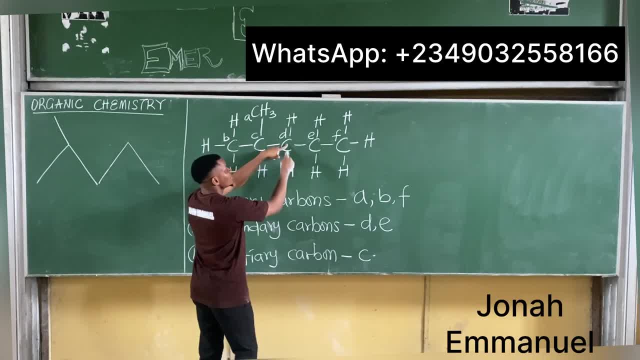 here c has one, two and three. so it here c has one, two and three. so it becomes a tertiary carbon. that's simple, becomes a tertiary carbon. that's simple, becomes a tertiary carbon. that's simple. come to d? d aside. the hydrogen has only. come to d? d aside: the hydrogen has only. 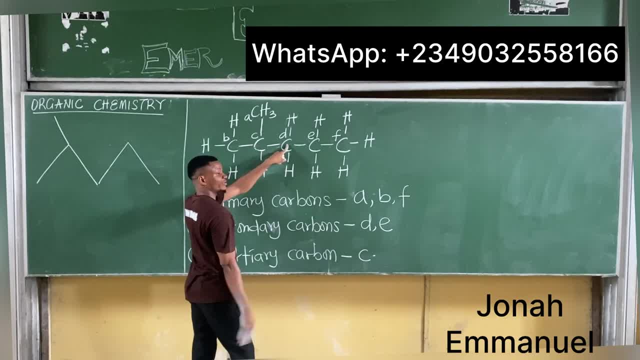 come to d? d aside. the hydrogen has only two attachments: this one and this one. two attachments, this one and this one. two attachments, this one and this one. that's secondary, that's secondary, that's secondary. come to e aside. the hydrogen e has just come to e aside. the hydrogen e has just. 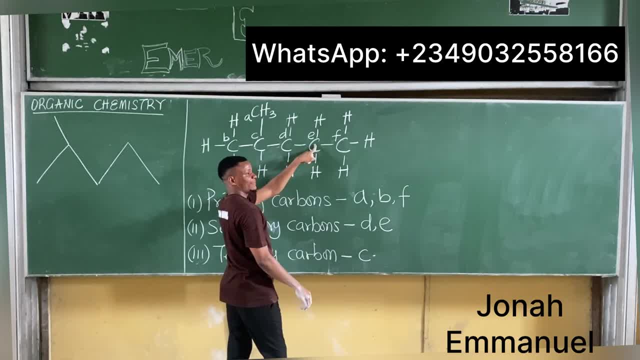 come to e? aside the hydrogen, e has just one and two attachments. is one and two attachments is one and two attachments. is um secondary. come to f? f. aside the um secondary, come to f? f aside the um secondary, come to f? f. aside the hydrogen, it has just one attachment. 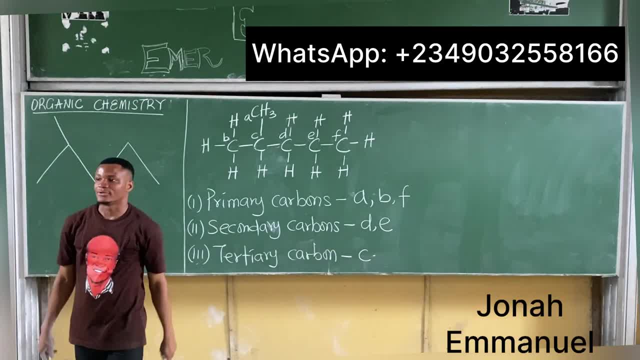 hydrogen. it has just one attachment. hydrogen, it has just one attachment. that's primary. it's as simple as that. that's primary. it's as simple as that. that's primary. it's as simple as that. no big deal. no big deal, no big deal, all right, all right. 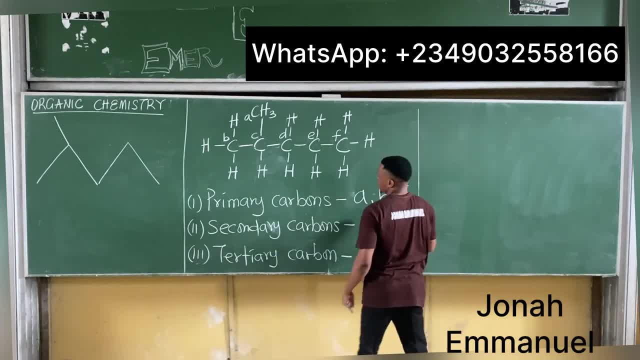 all right, our next task. they said we should find our next task. they said we should find our next task. they said we should find. so let's, let's call this the a part. so let's, let's call this the a part. so let's, let's call this the a part. the big part said we should find. 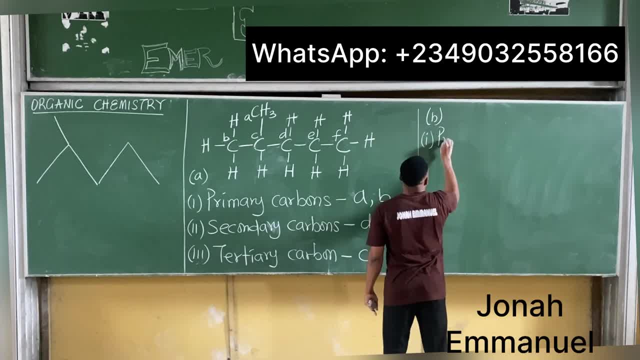 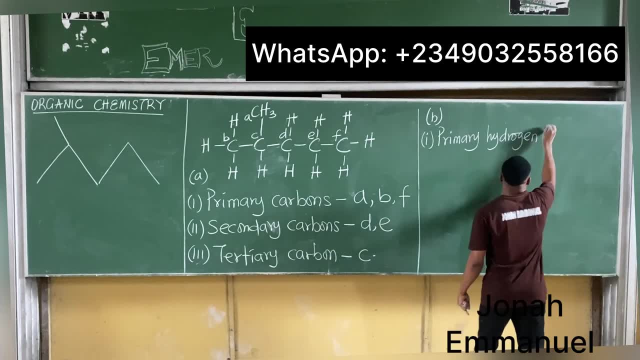 the big part said we should find. the big part said we should find the number of primary hydrogen, the number of primary hydrogen, the number of primary hydrogen, primary primary primary hydrogen, hydrogen hydrogen. we said the symbol is what there. we said the symbol is what there. we said the symbol is what there one not. 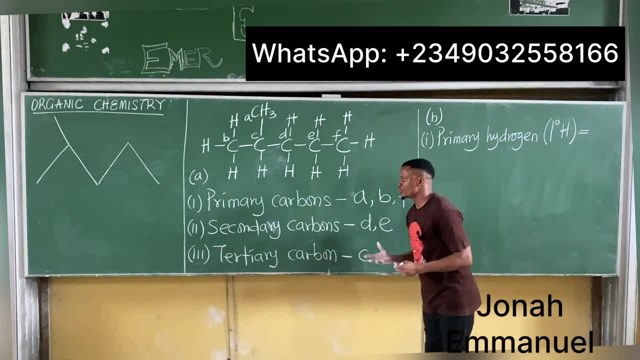 one, not one, not h. how many the primary hydrogen are h? how many the primary hydrogen are h? how many the primary hydrogen are? simply the hydrogens of the primary, simply the hydrogens of the primary, simply the hydrogens of the primary carbons. my primary carbons include one. 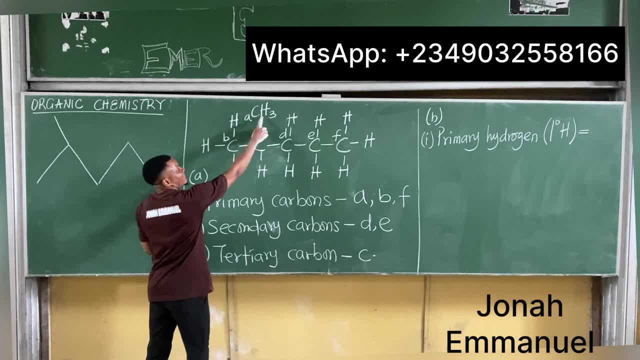 carbons. my primary carbons include one carbons. my primary carbons include one, two, two, two, three. so if i count, this one has how many three. so if i count, this one has how many three. so if i count, this one has how many there, there. 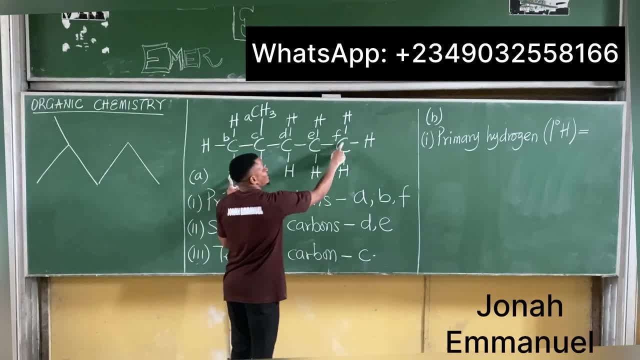 there three. this one has how many there three, three. this one has how many there three, three. this one has how many there three. this one hasn't been there. this one hasn't been there. this one hasn't been there to combine all of them, because i'm in there. 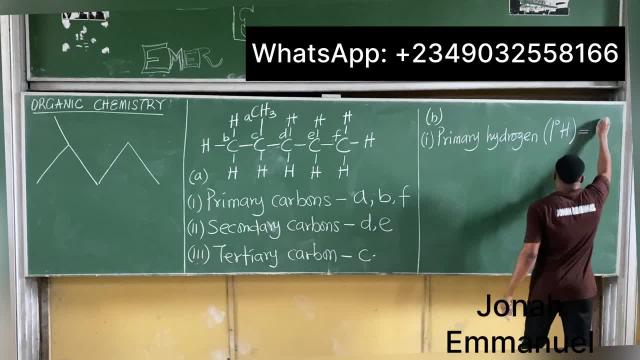 to combine all of them because i'm in there, to combine all of them because i'm in there. nine: i'm having nine um primary. nine i'm having nine um primary. nine i'm having nine um primary. yes, so one, two, three for f. yes, so one, two, three for f. 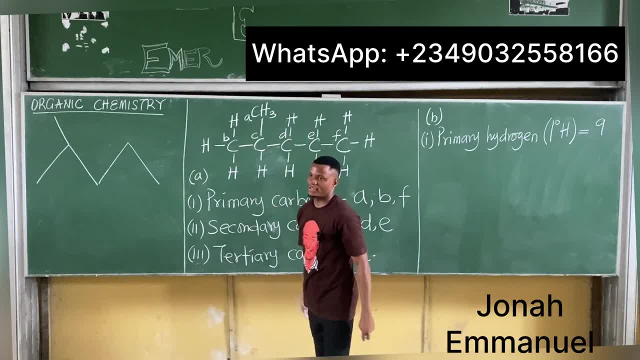 yes, so one, two, three for f, three for eight. that's six. one, two, three, three for eight. that's six. one, two, three, three for eight. that's six. one, two, three, nine, nine, nine, that's it. that's it. that's it, number two. let's look at. 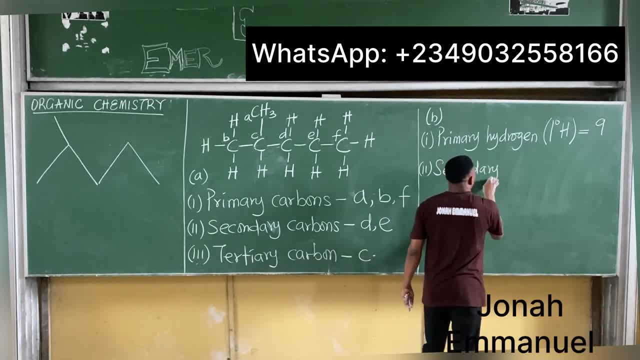 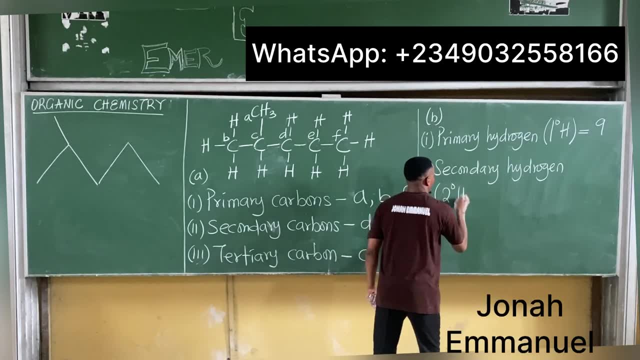 number two. let's look at number two. let's look at secondary carbon: secondary hydrogen, please. secondary hydrogen, please. secondary hydrogen, please. secondary hydrogen, that's secondary hydrogen, that's secondary hydrogen. that's this h, this h, this h. please check how many please. please check how many please. 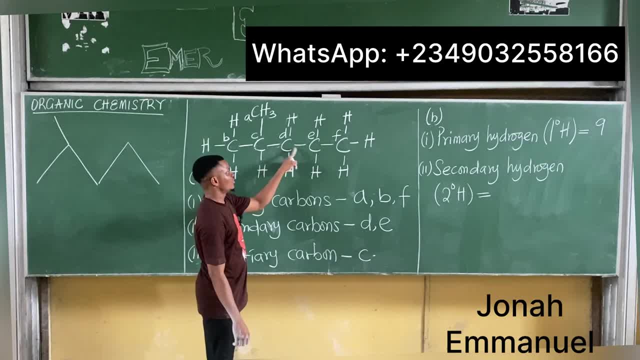 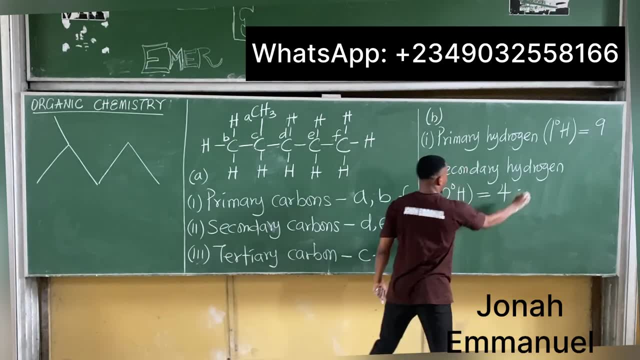 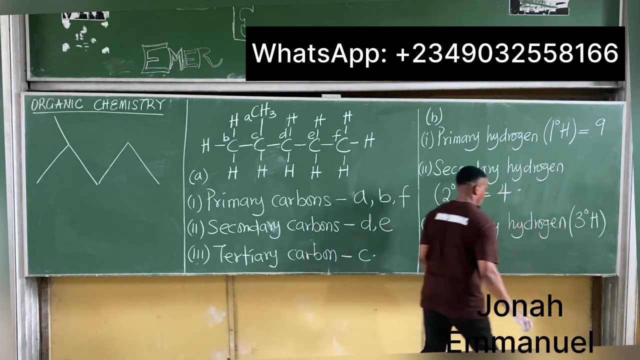 My secondary will adjust this: 2.. It becomes the hydrogen of this 2 and then 3,, 4.. So I have 4, secondary hydrogen Number 3.. Tertiary hydrogen: That becomes 3, naught H: Please check. 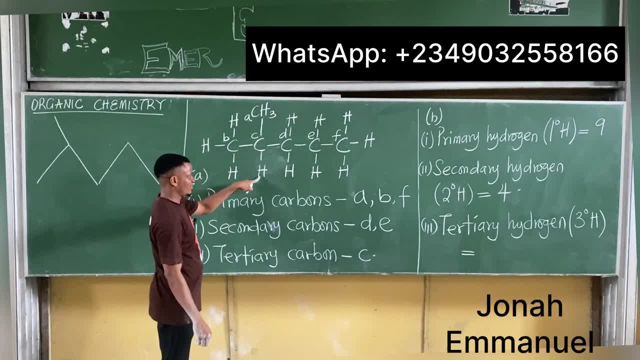 How many tertiary do we have? So this carbon has what there Here? just 1 hydrogen. This one here has just 1 hydrogen. That's how it's done In a short cut, in a short format. from here I can tell you how many they have. 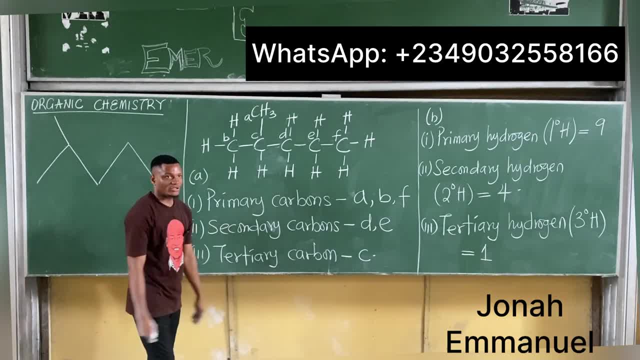 Your primary carbon will always have 3 hydrogen. In total it will be 3 times the number of primary carbon. So 3 times. how many do I have here? 1,, 2,, 3. That gives you 9.. So primary will always have 3 carbon, Note it. Secondary will always have 2 carbon. So it becomes 2 times the number of secondary atoms, or secondary carbon, 2 times 2, that's 4.. Tertiary will always have 1 hydrogen. So it becomes 1 times the number of what Tertiary carbon. 1 times 1, that's 1.. That's it. So it's always number of primary carbons times 3.. Number of secondary carbons times 2,. number of tertiary carbons times 3, times 1, please. Number of tertiary carbons times 1,. please Let's take one more example on this and then we'll proceed For this same example. for this example, let's have to get number of primary, secondary, tertiary and their hydrogen. 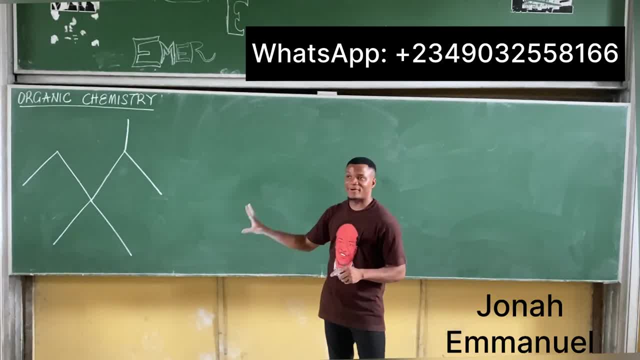 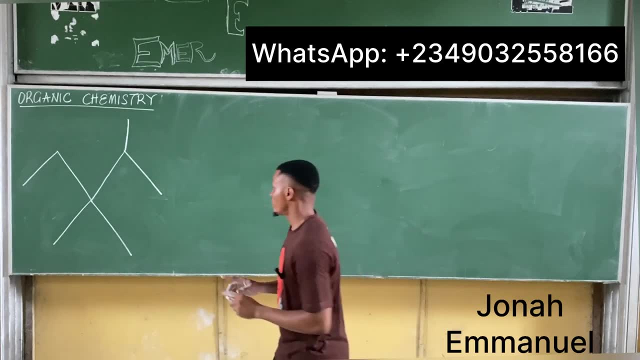 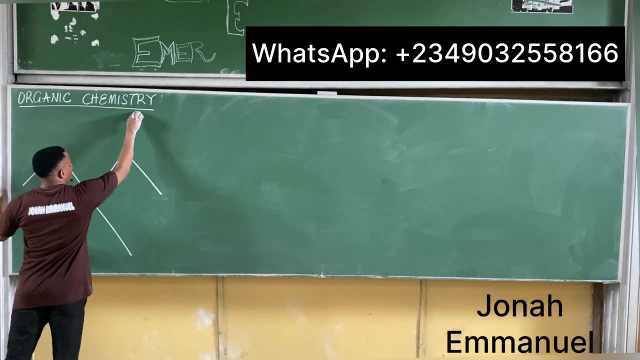 Now listen. Try to draw a structure, for A complex structure like this would be time-wasting. What do I do? Figure it out. Number 1. Primary are always at the extreme. What does it mean? This one here is a primary carbon. 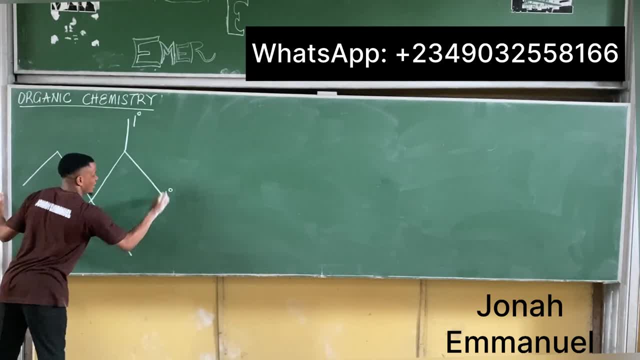 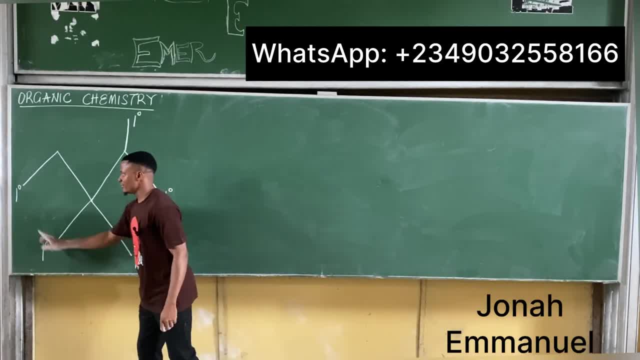 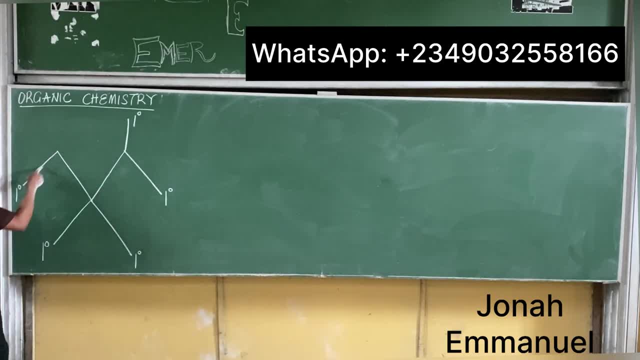 Next up this one here. Please check How many attachments does it have here To the console over there. Secondary carbon, That's all. Don't forget at each junction. So this junction, this junction, this junction, please. 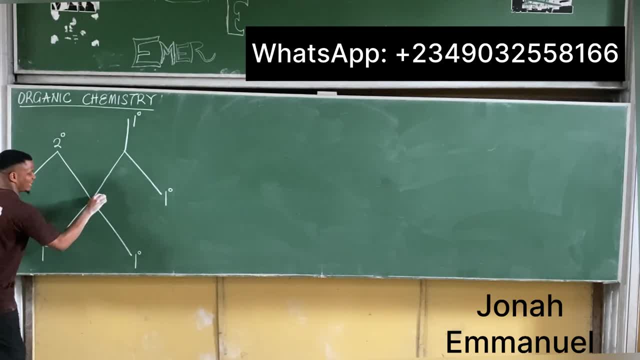 This one has how many attachments to the console over there. It's called a quaternary carbon. This one has how many attachments there To the console over there, Because what's there? Tertiary carbon. That's all. So I have five, primary one. 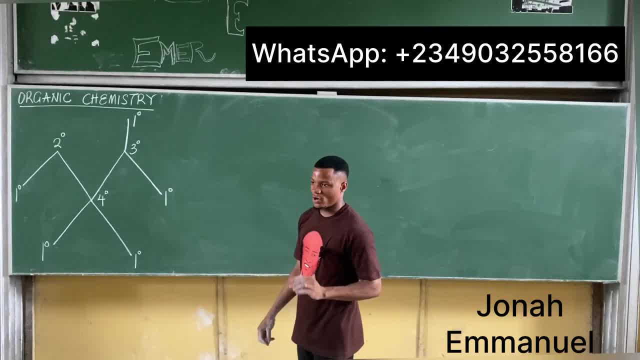 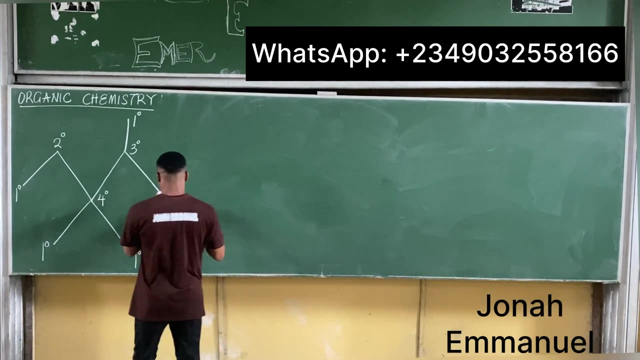 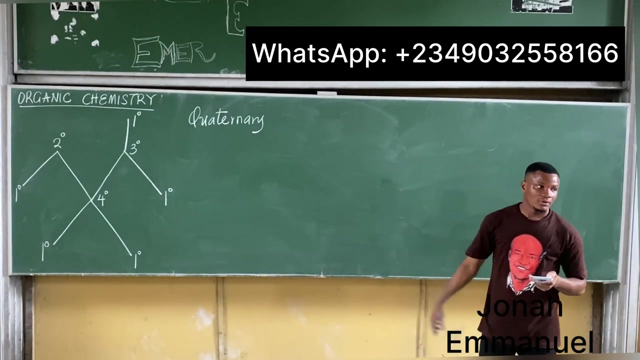 secondary one, tertiary one, quaternary carbon. Quaternary is spelled quaternary, Quaternary, Quaternary carbon. No, I'm not drawing the place. Thank you, If you have something to draw, I said you don't have to draw. 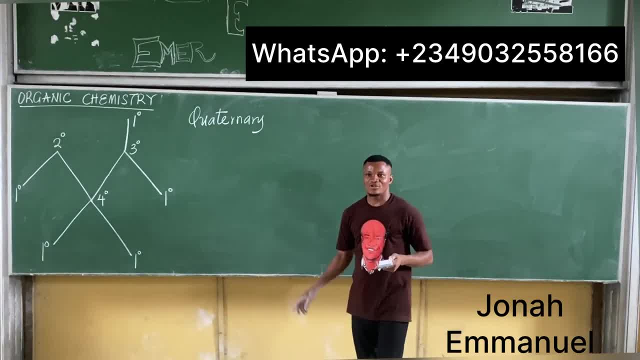 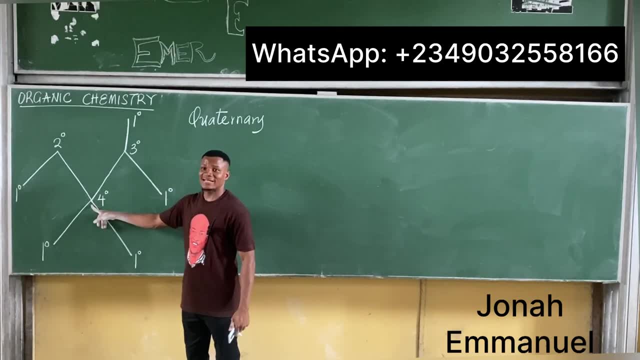 Drawing this stuff is complex. Try to draw it out. It's so much of a headache. Just know. yes, chief, How is this one here? How is it It has four tertiary. Now one. Listen, listen, At each junction is a carbon. So there's a carbon. 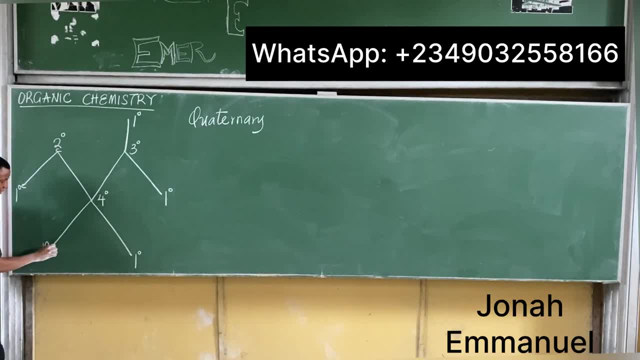 here, here, here, here, here, here, here and here. This one has one, two, three tertiary. Extremes are always primary, Don't stress. This one has one, two secondary. This one has one, two. 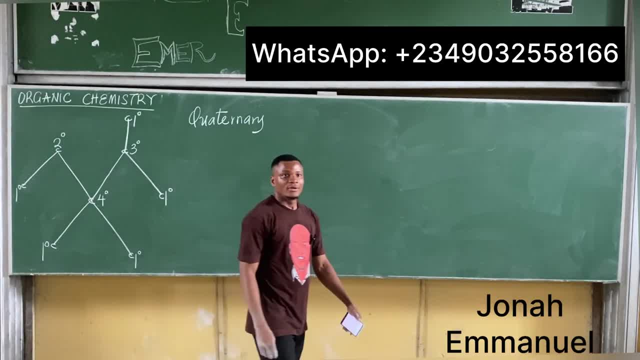 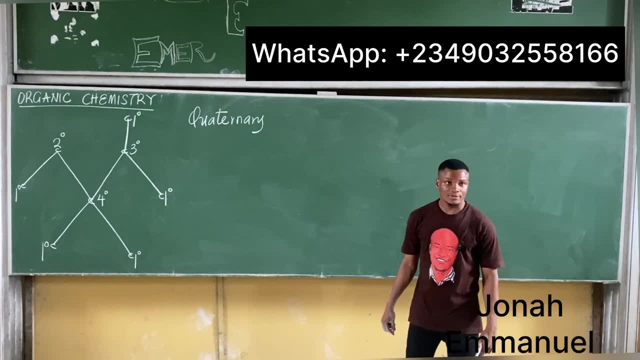 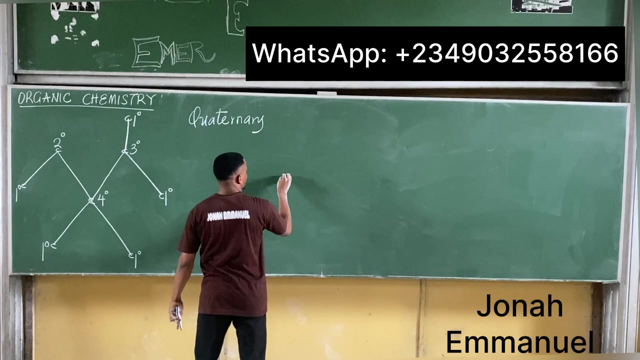 three, four, quaternary. Is that simple? Yes, Yes, Yes, Yes, Yes, Yes. Okay, let's draw this. Let's draw this. This becomes CH3.. This one becomes CH3.. One, I'm having CH3 here compared to this. 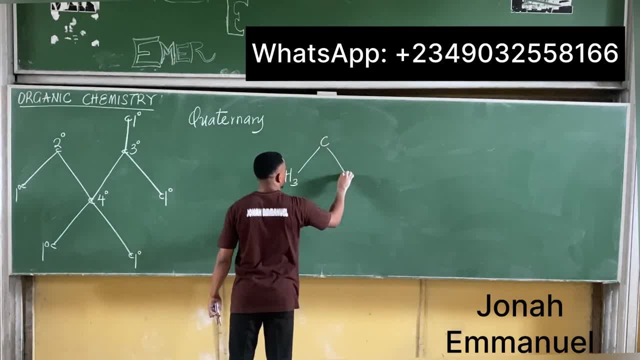 That becomes what? there? This? Okay, All right at this place. That's up. and this 1, 2.. How many left there? 2.. Abhi, come here. I have a carbon here, This one, This one has coming down. I have this one here, This carbon here. This is 1, 3, 4.. 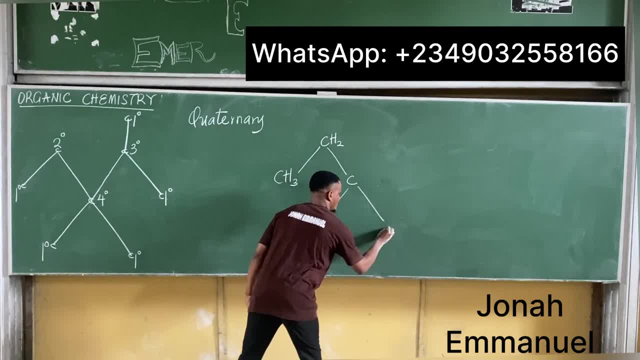 From this center. one like this, This center, one like this: C 1 plus 3, 4.. This one is now going up like this. This one is now going up like this: The carbon. somewhere here, This carbon has another. 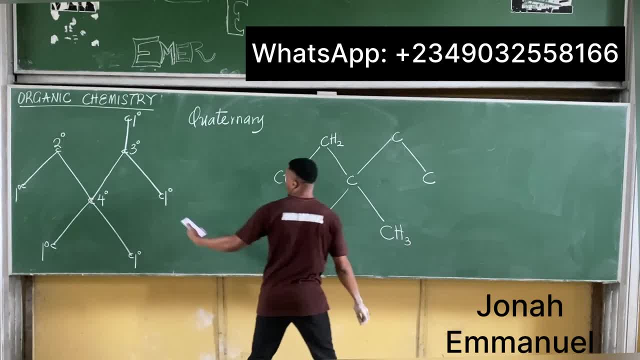 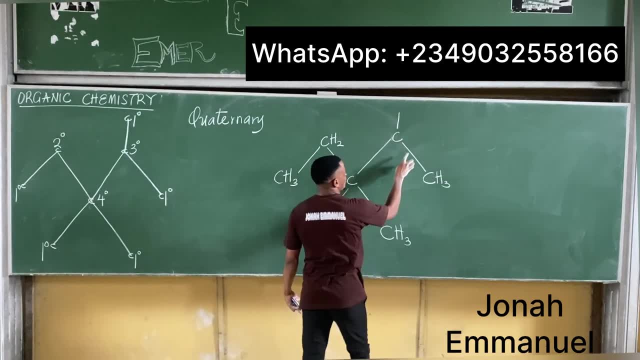 attachment down. So it's coming down this way. This one is left alone. So 1 plus 3, 4.. This one is going up, So I'm going up here. This is 1, 2, 3 plus 1, 4.. Here has to be one there. Let's see. 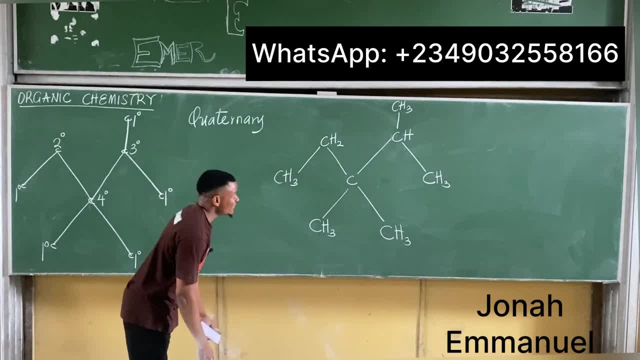 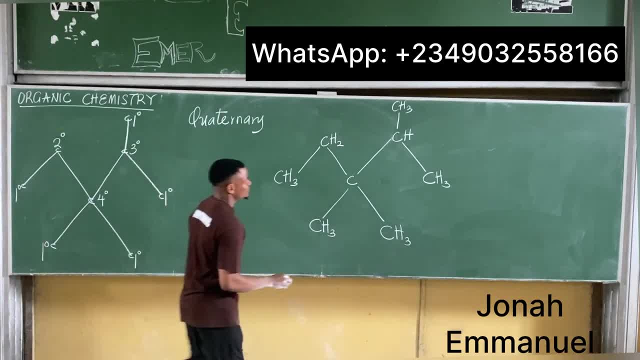 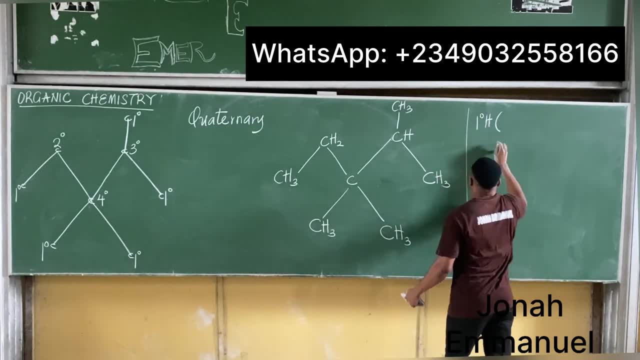 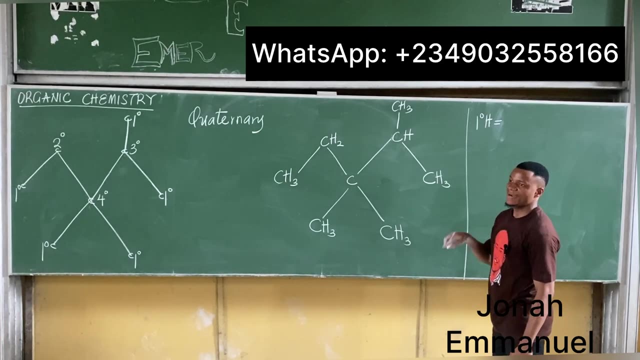 For primary. Look up here For primary, For primary, Primary hydrogen H, Please. We said it's equal to what there. Number of what Number of primary carbon Abhi, How many there? 5. Times, what number there? 3. That should be equal to what there? 15 primary hydrogen. Now check it out. 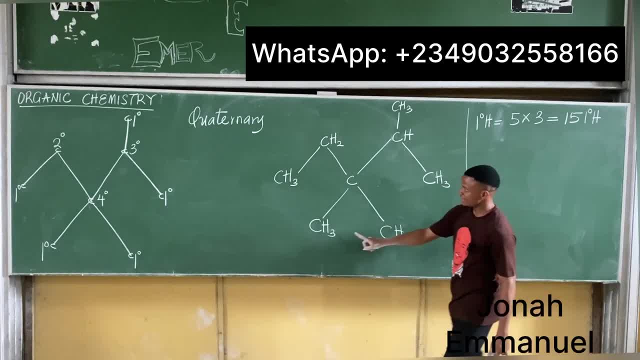 This is a primary: 3,, 6,, 9,, 12, 15.. It's correct. Let's look at secondary hydrogen. We said it's equal to number of secondary carbon. Please, how many secondary carbon do you have here? Just 1.. 1 times For this. 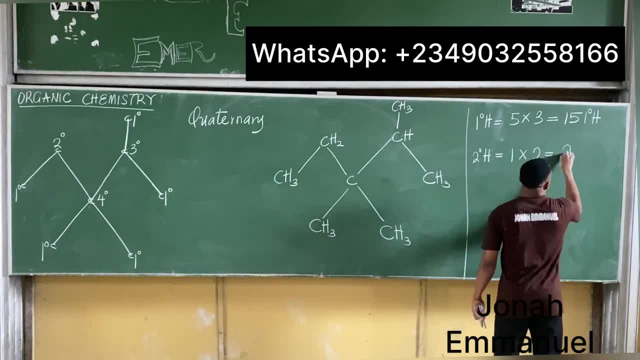 one's number there: 2.. 1 times To give you what there: 2.. Okay, 2.. Let's do it this way. Secondary hydrogen, And that's correct. This is my only secondary, This one here, That's this one. 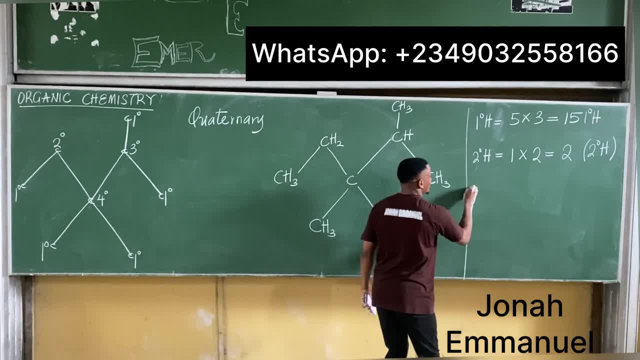 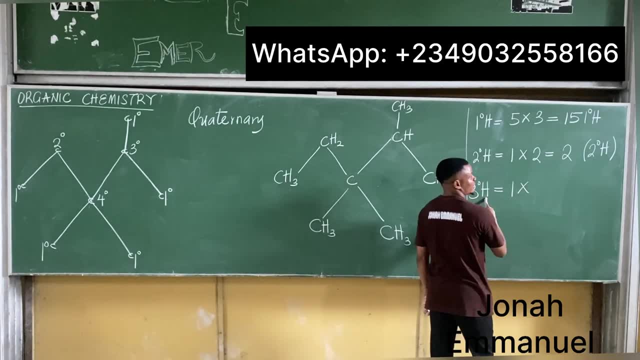 How many there? 2. It's correct, Let's do tertiary hydrogen, Please. how many tertiary hydrogen do you have there? 1. You're multiplying this one by how many? By 1. 1 times To give you what there? 1 tertiary hydrogen. Where's the tertiary man? See him here, Abhi. How many? 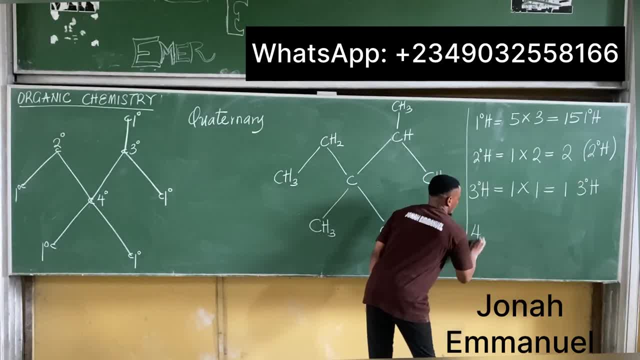 hydrogen here, 1.. For quaternary, That's equal to how many quaternary carbon do you have there, 1. 1 times Multiply this by what there 0.. Now give me what there 0 quaternary hydrogen. So check out the. 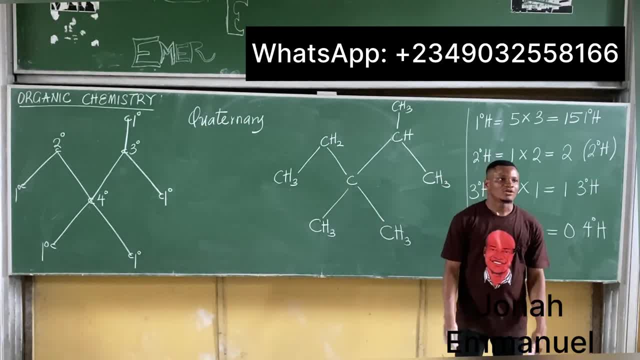 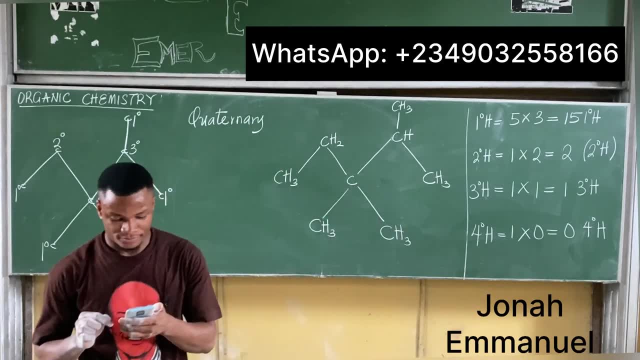 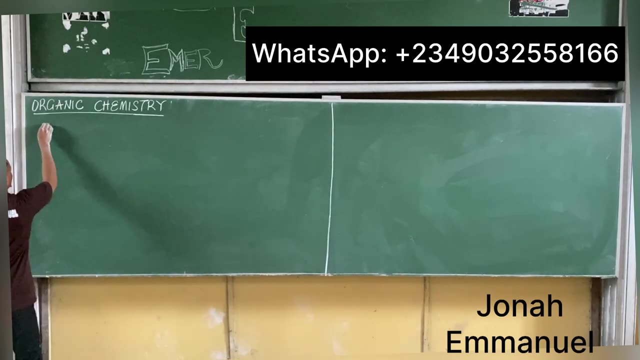 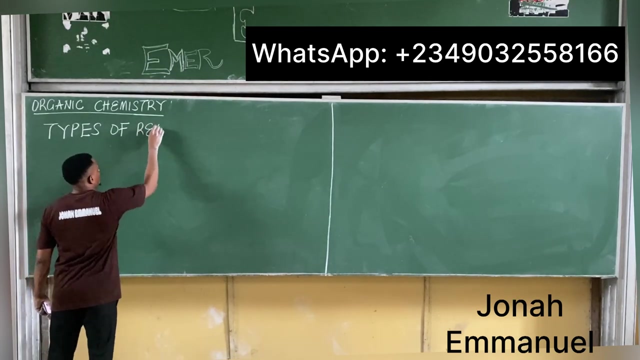 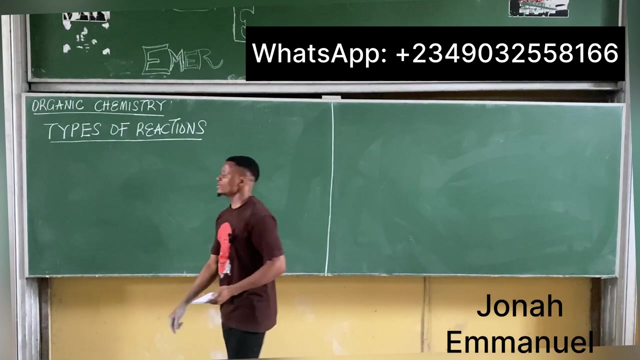 quaternary carbon. There's no hydrogen on it, So that's it. Number of carbon times: 3, 2, 1, 0.. It's not that deep, All right. All right, Let's look at types of reaction. I'll keep this within the scope of your text. 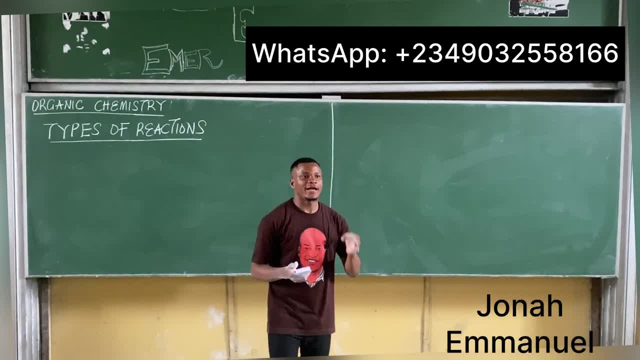 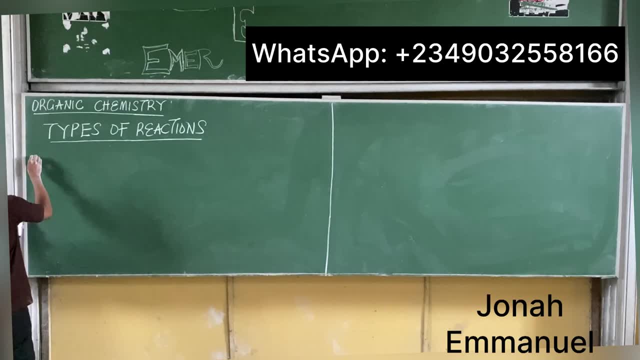 There are three types of reactions. Number one: addition reaction. That's number one. Number two: substitution reaction. Number three: elimination reaction. Number three: elimination reaction. There are three types of reactions. Number one: elimination reaction. Number two: elimination reaction. 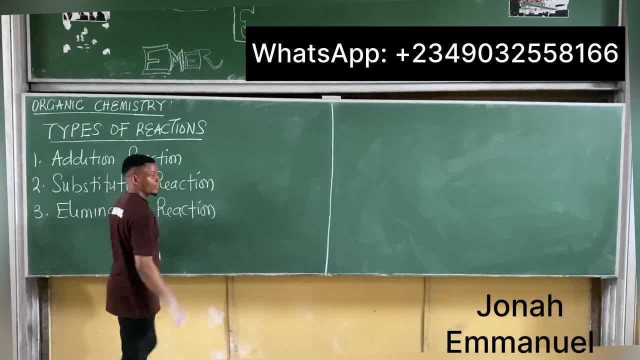 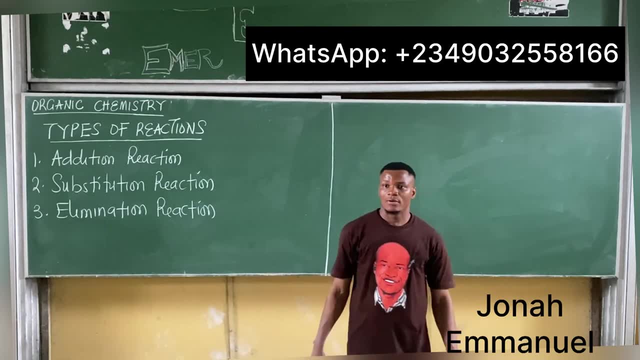 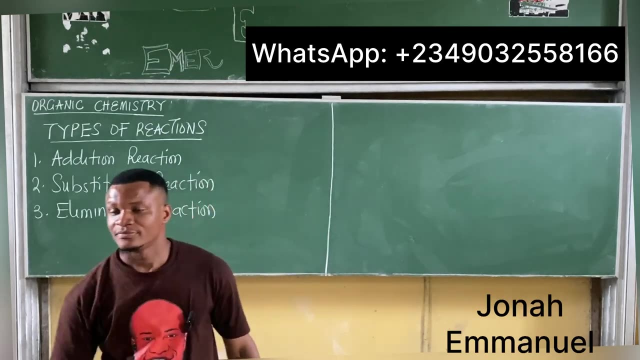 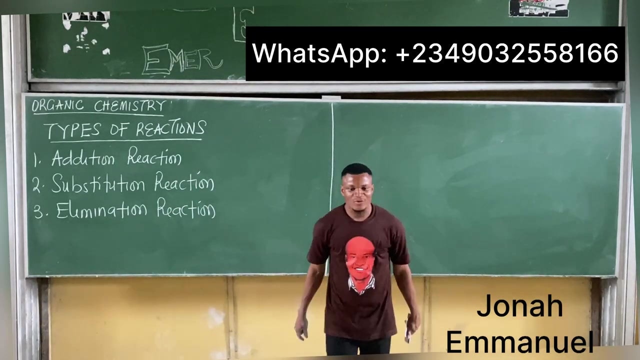 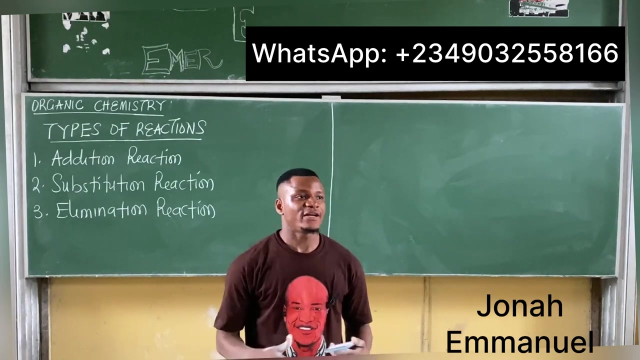 Number three: elimination reaction. Number four: elimination reaction. What's the first one, Elimination reaction. So if they call it rearrangement too, no problems. So one of the questions you would see most likely is: classify the following reactions as addition, substitution and what there, elimination. 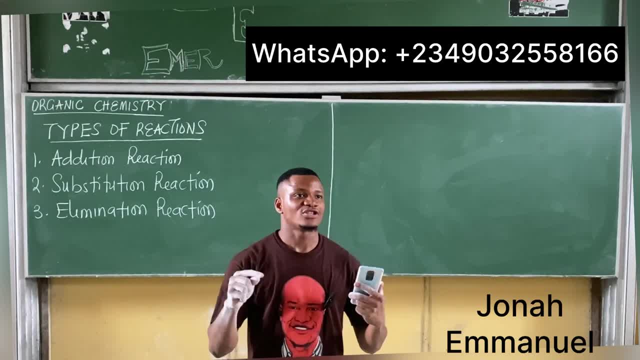 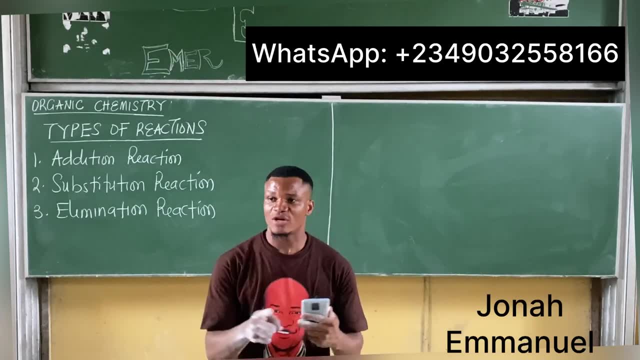 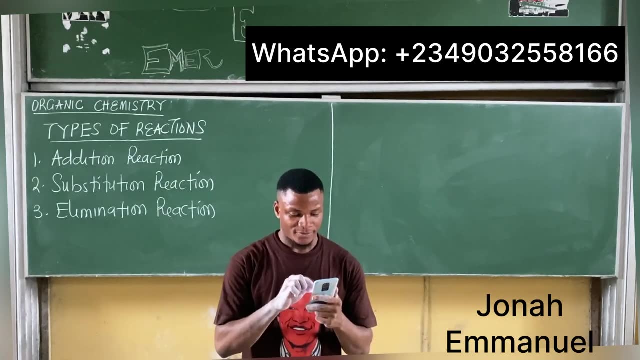 So how do you easily know which is addition, which is substitution, which is elimination After addition? I said substitution, not subtraction. Somebody go and write subtraction in the exam And it's not a joke. If you've ever mapped student scripts before, student script is one of the funniest thing. 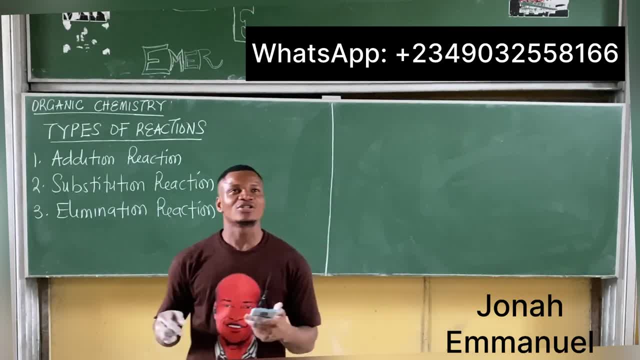 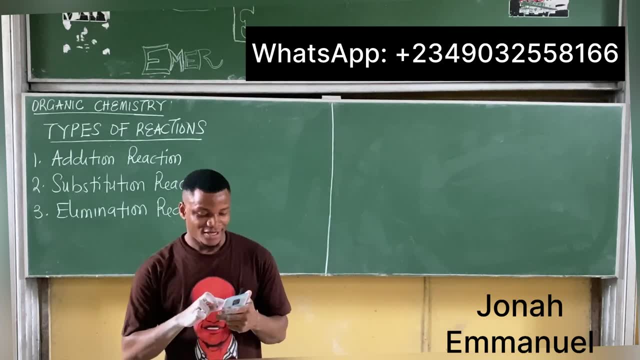 you can map. I tell you Like you see things and you ask yourself this one: are you using your brain to write, or what? No, I'm serious: Student scripts. That's why I'm not moved with this. what do you call it? 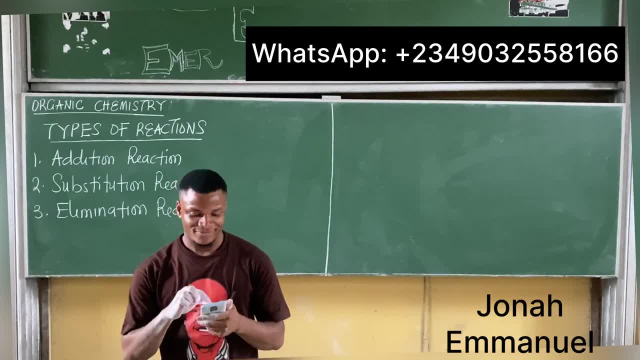 I burn the paper. It doesn't move me, But I've seen things, though. Somebody I taught somebody. I taught types of rock, types of rocks. I taught them types of rocks. I had the person repeat it over and over and over again. 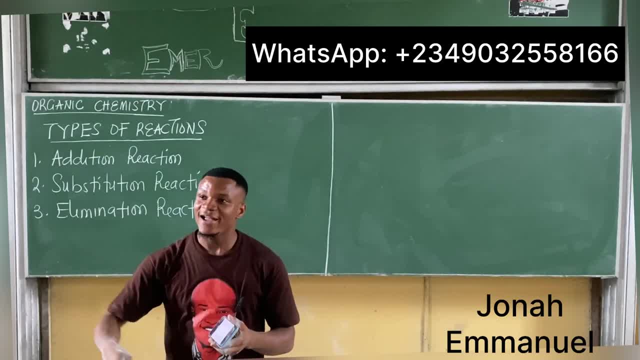 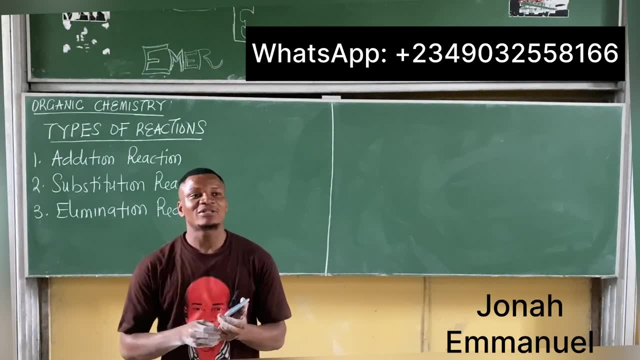 The day before exam. The person repeated it over and, over and over again. So I was happy that they would get types of rock. I gave them tests, Types of rock. So one time they write for me: number one, Zuma rock. 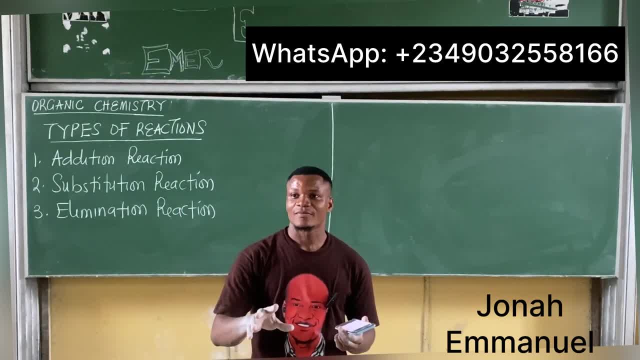 I'm not kidding, right, I'm not kidding Now. types of rock ignores sedimentary metamorphic. This guy repeated it, like he repeated it in front of me. how many times Then in exam? he now wrote for me: Zuma rock. 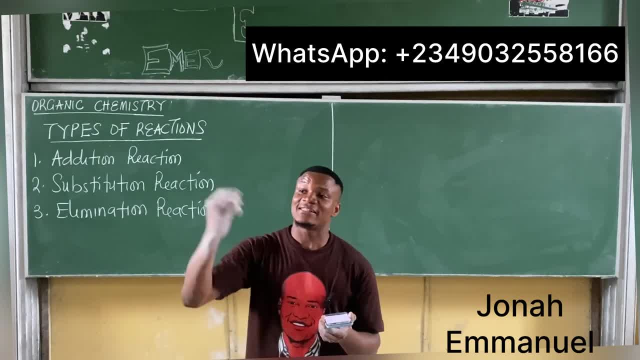 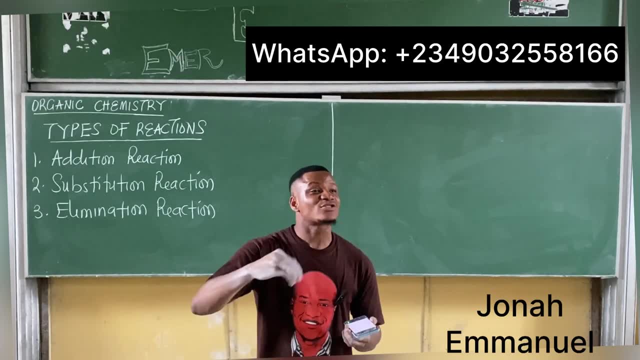 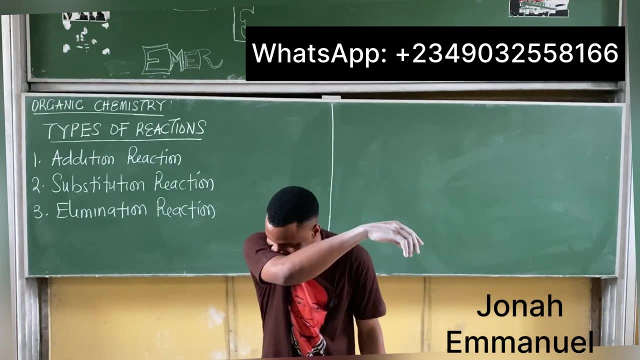 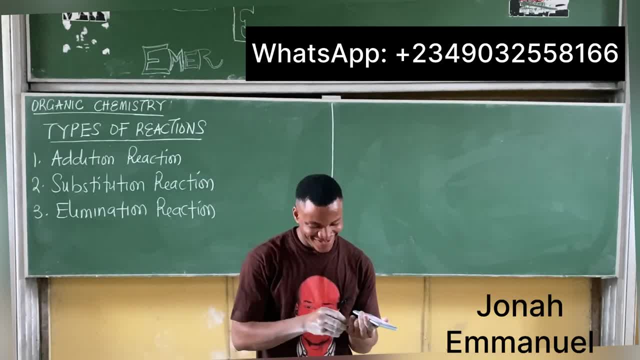 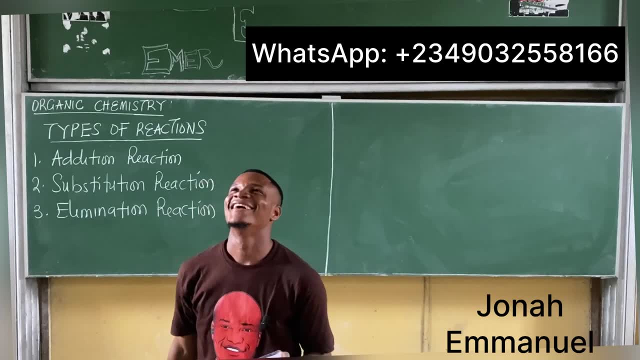 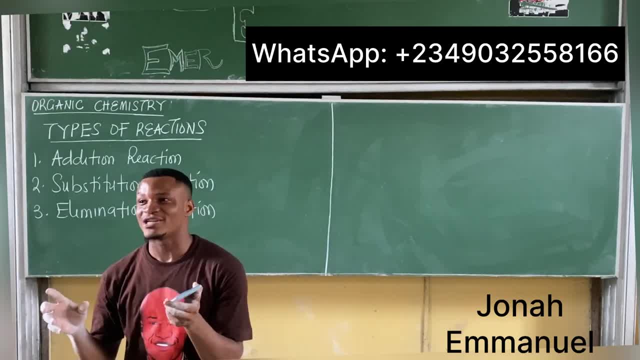 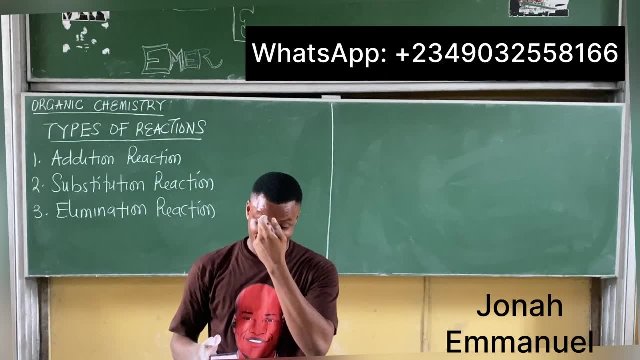 Like you forgot that Aso rock is not actually a rock, It's actually a piece Aso rock. Can someone for me write something that I can still remember? Okay, Okay, substitution reaction. trust me, and this same person will tell you: i, i. 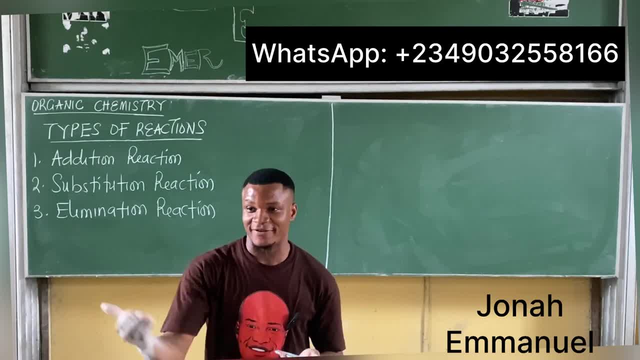 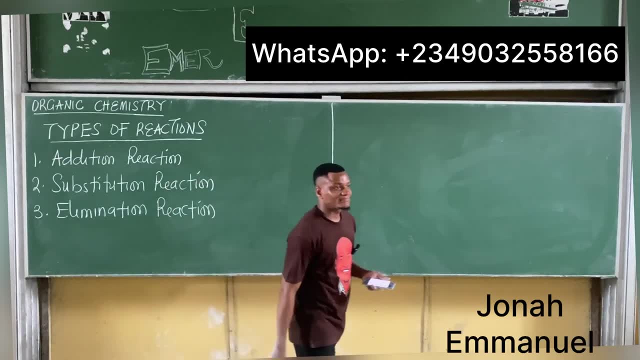 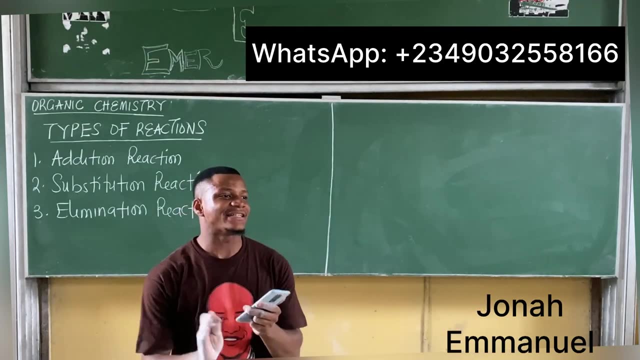 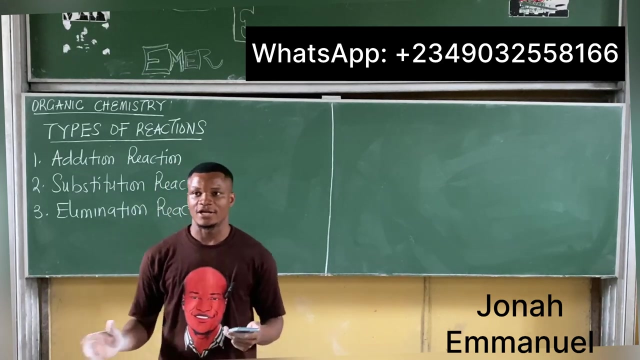 bought the thing. i finished everything. 15 minutes still left. i submitted on time. all right, so if i have addition, substitution, elimination, how can i easily identify take down leads? how to easily identify any? how to easily identify anything? please help me watch if this i i'm feeling that this space will. 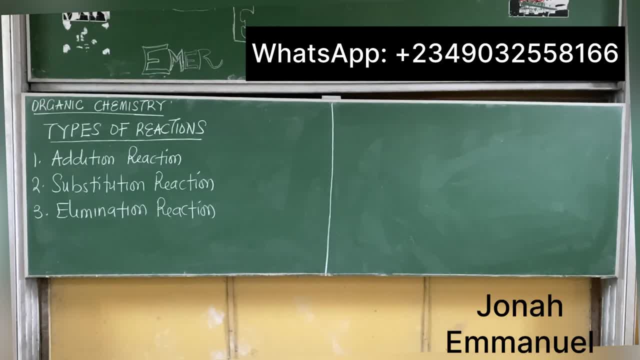 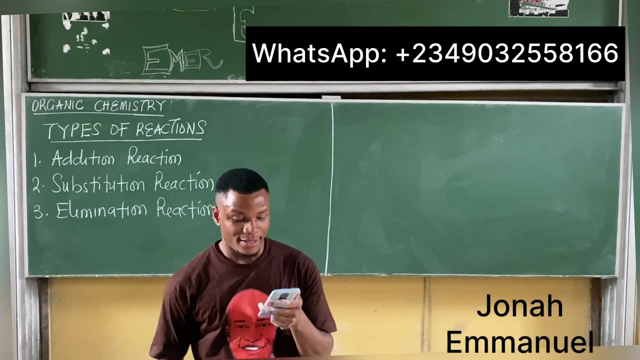 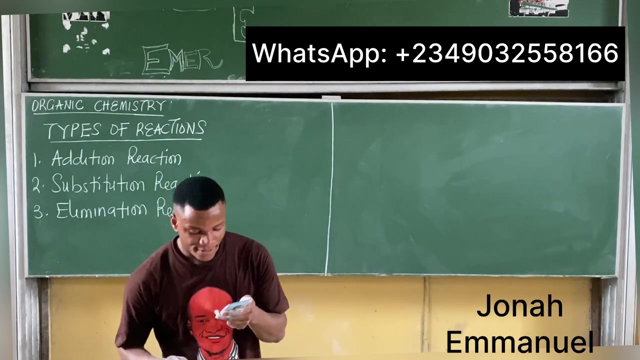 simply escape. they've just used space and this error, whatever. just let me know, all right, how to easily identify any number one, how to easily identify any number one: for addition reaction comma: the complex hydrogen structure. for addition reaction comma: the complex hydrocarbon, please. the complex hydrocarbon. 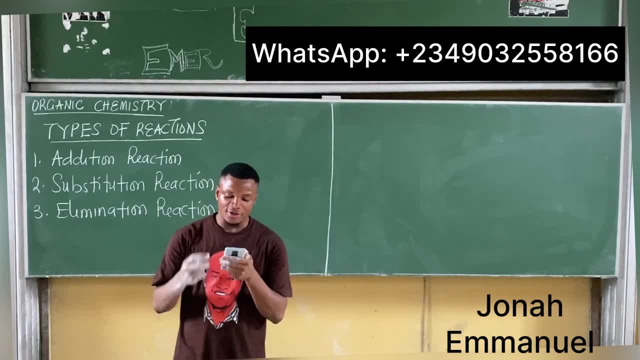 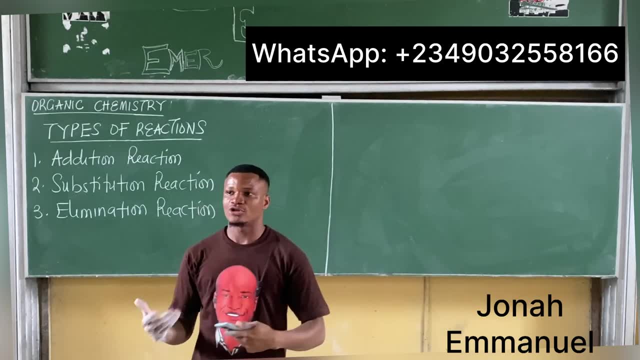 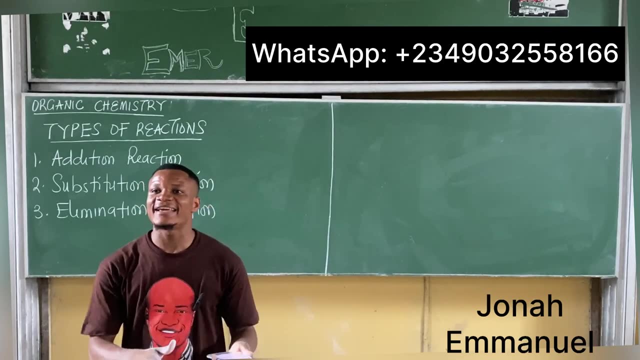 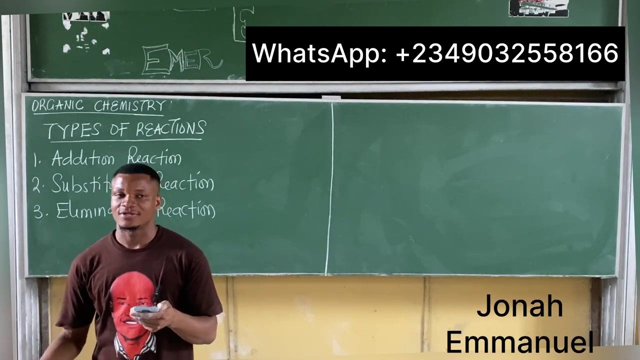 for additional reaction. the complex hydrocarbon structure is broken down to a simpler hydrocarbon structure. so the complex hydrocarbon structure is broken down to a simpler hydrocarbon structure. example: alkyne to alkene, alkyne to alkane, of course. example al kind, that's y e to al king. so triple bond has broken down toward their 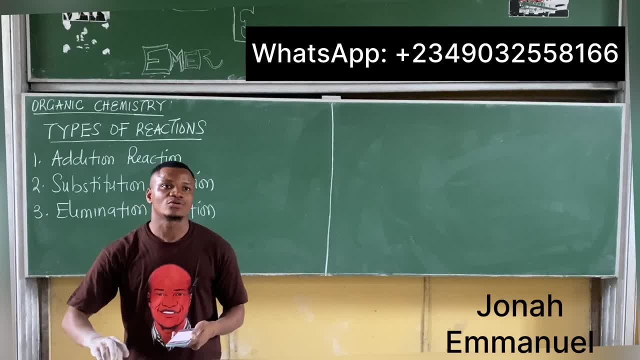 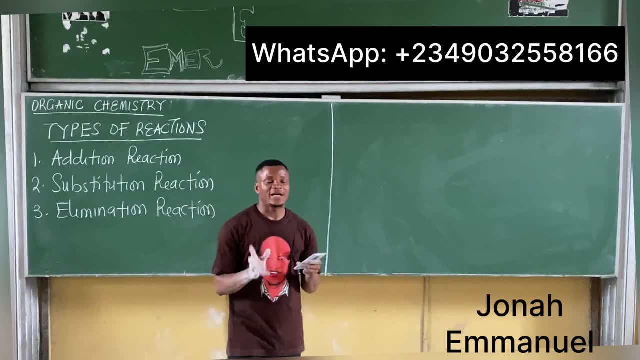 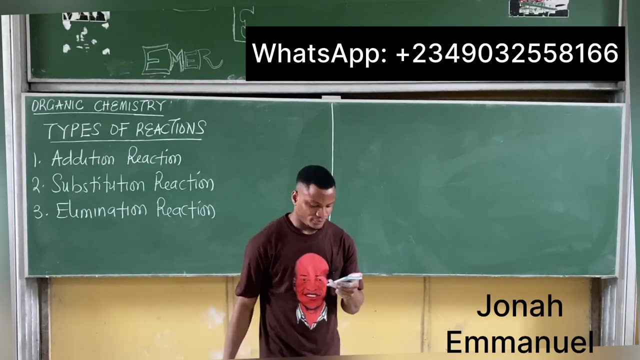 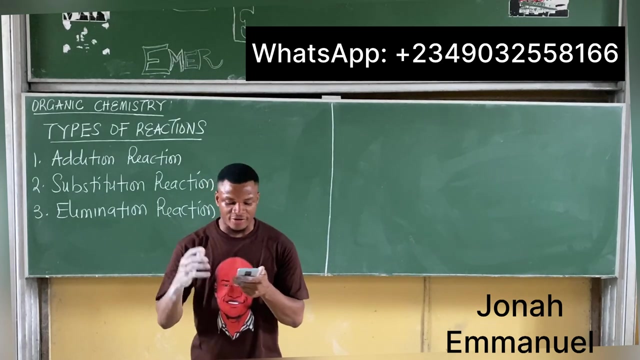 double bond, or from al king to al king, that's from double bond to single board. so that's it. so that's that's how you identify addition. there will be um a breakdown of complex hydrocarbon to simpler one. number two: number two: substitution reaction for substitution reaction: number two: 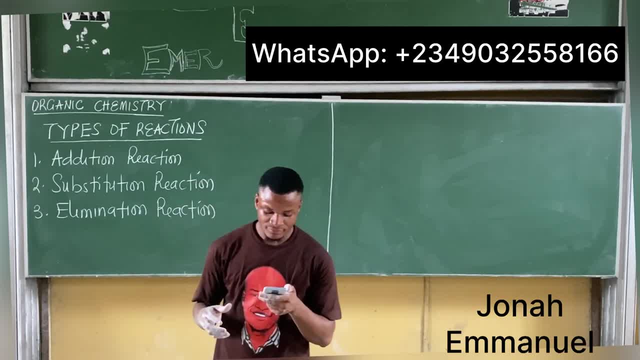 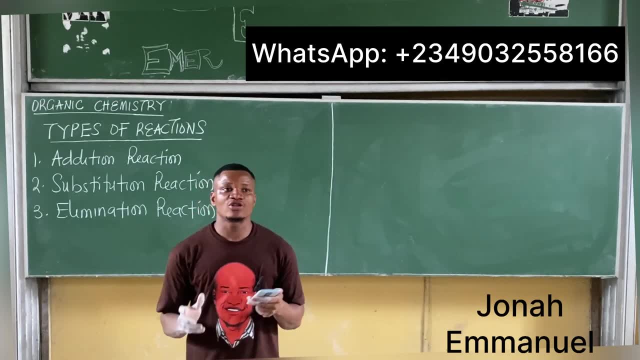 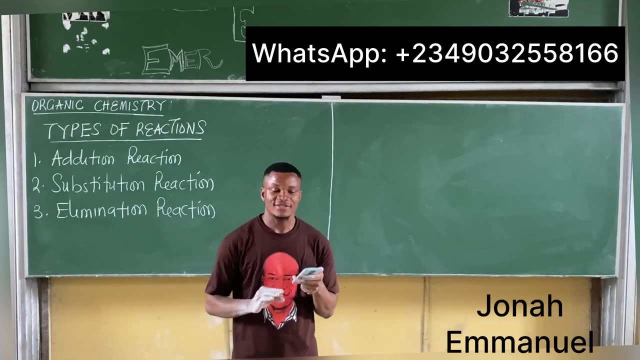 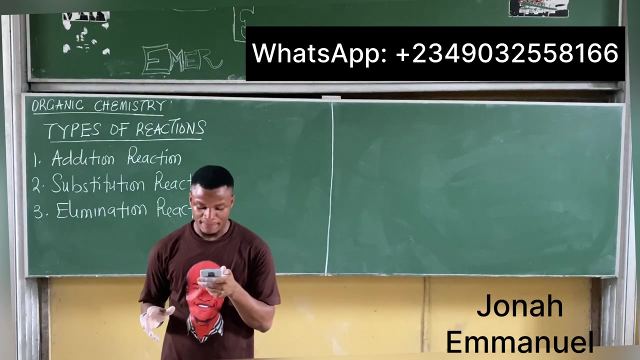 for substitution reaction. the hydrocarbon structure for substitution reaction: comma. the hydrocarbon structure in bracket, sometimes complex, remains the same, please. for substitution, it remains the same with some of the substituents, with some of the substituents in bracket for substitution reaction: comma. the hydrocarbon structure in bracket, sometimes complex. 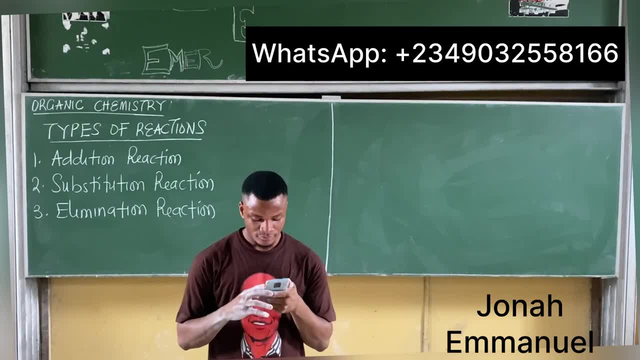 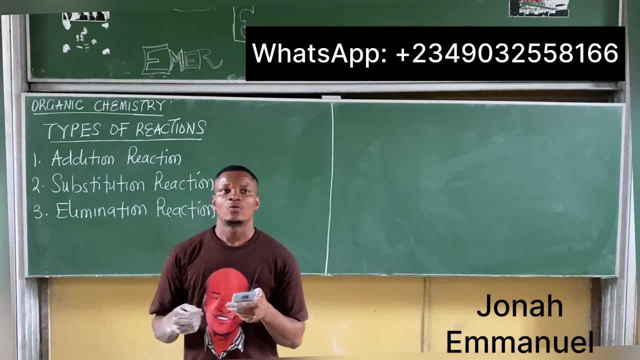 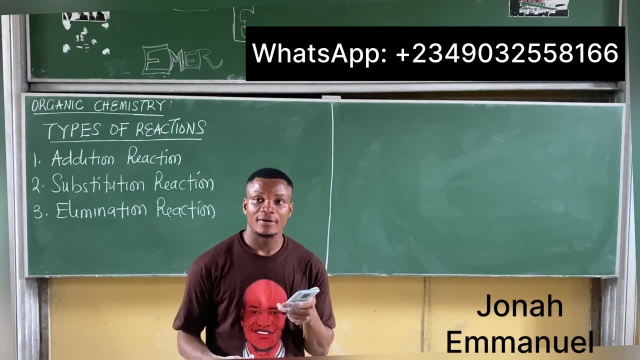 remains the same in bracket, sometimes complex, with some of the substituents in bracket a of the substituents in bracket lacrima with some of the substituents in bracket with some of the substituents in bracket: hydrogen, coma, alkyl group, etc. 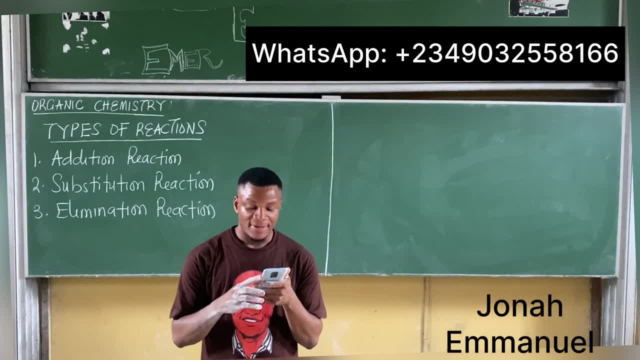 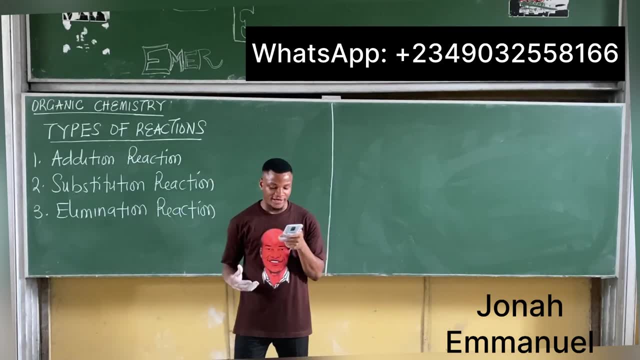 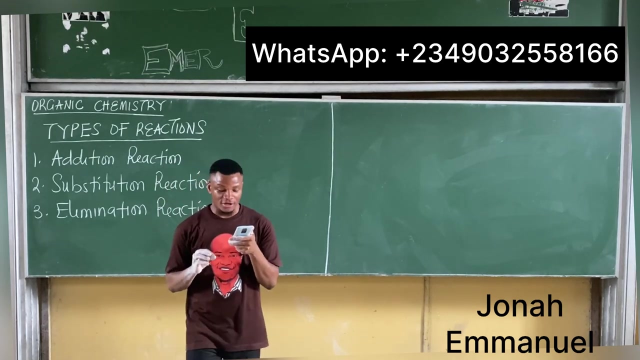 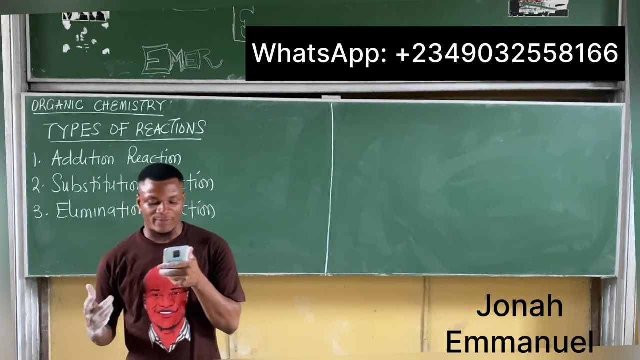 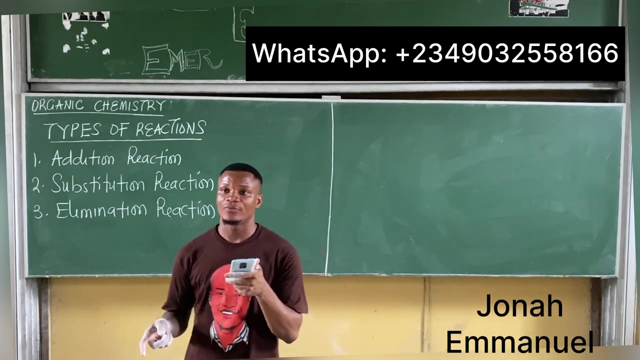 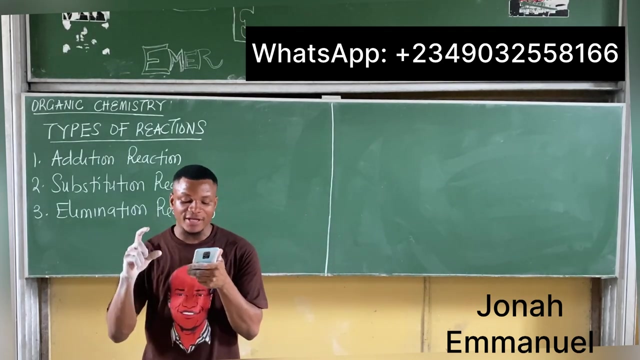 being replaced by another substituent. being replaced by another substituent: full stop. majorly for substitution reaction. majorly for substitution reaction comma. majorly for substitution reaction comma. majorly for substitution reaction comma. the hydrogen structure retains its structure without being broken down. majorly for substitution reaction comma. the hydrogen structure retains its. 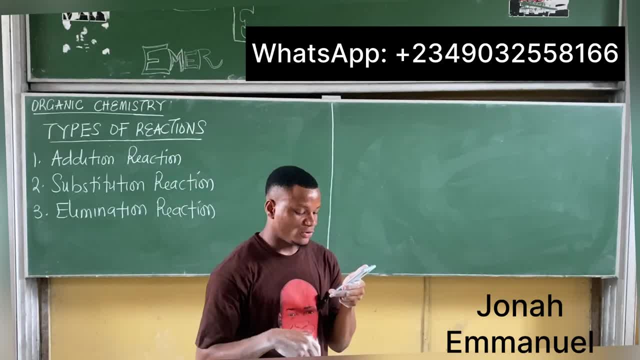 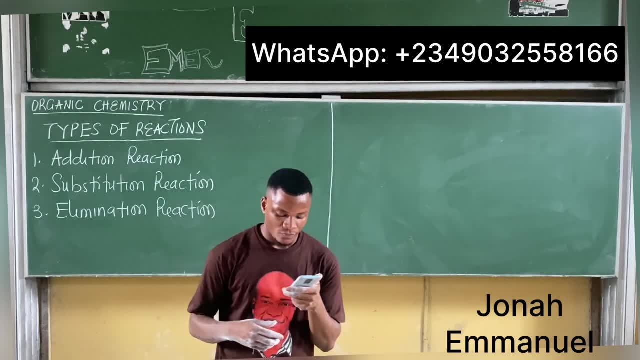 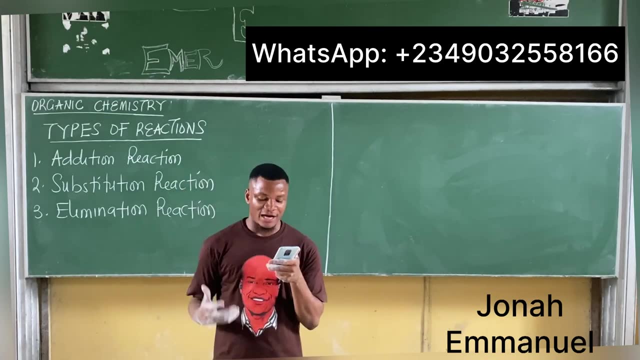 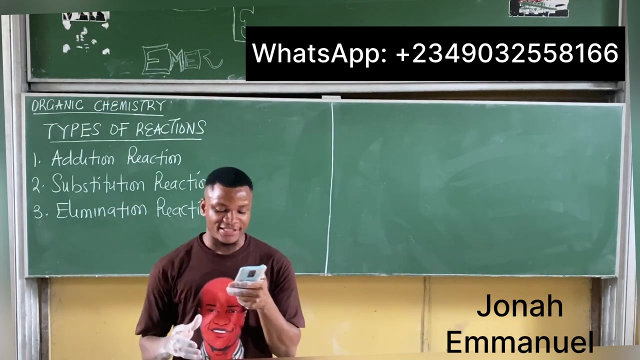 structure without being broken down or without being broken to a simpler hydrogen structure. BETudos- BETudos retains its structure without being broken. retains its structure without being broken down or broken to a simpler hydrocarbon, although some substitutes may be added, or although some substituents may be added. 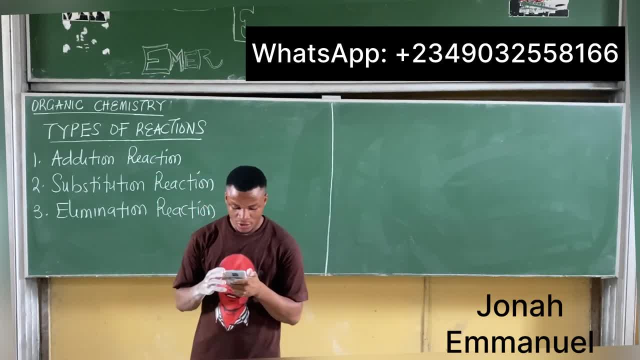 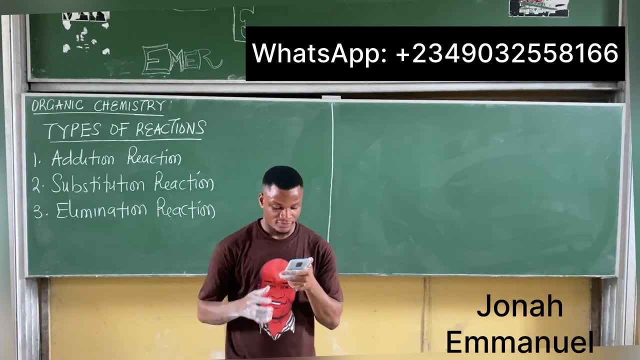 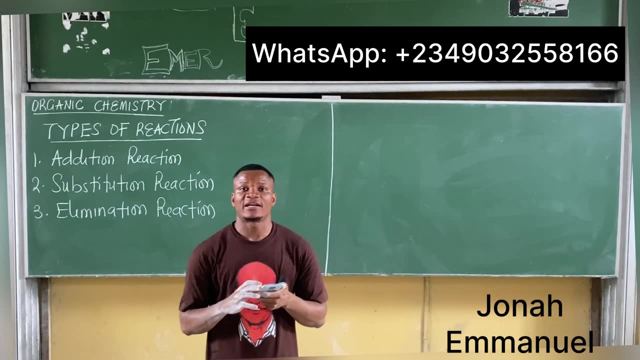 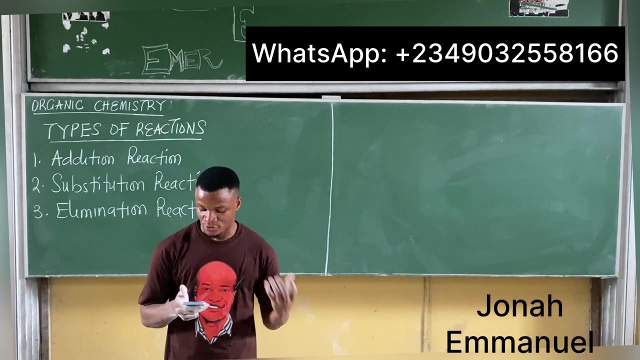 or removed, although some substituents may be added or removed. Finally, number three. finally, number three, for elimination reaction. for elimination reaction, one or more substituents are totally removed. for elimination reaction, one or more substituents are totally removed. 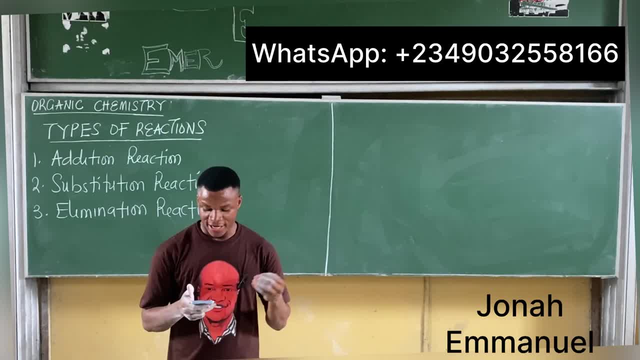 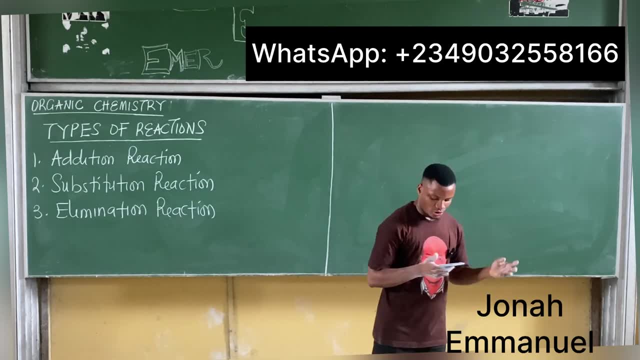 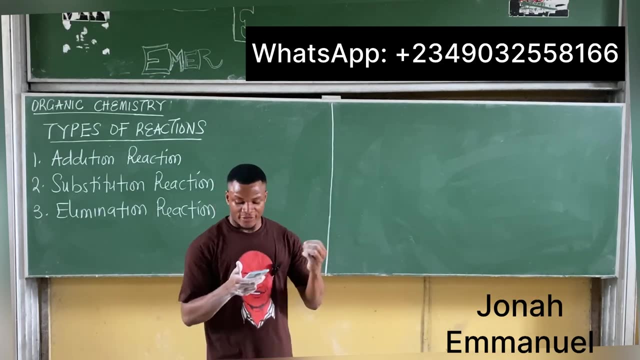 from a hydrocarbon totally removed from a hydrocarbon without replacement for elimination reaction: one or more substituents are totally removed from a hydrocarbon without replacement. without replacement, Full stop. This can cause the hydrocarbon to form another homologous series. 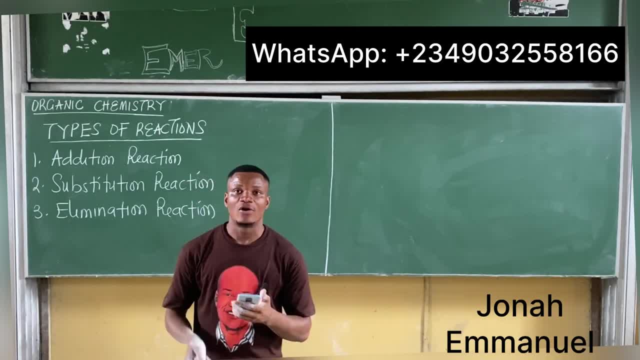 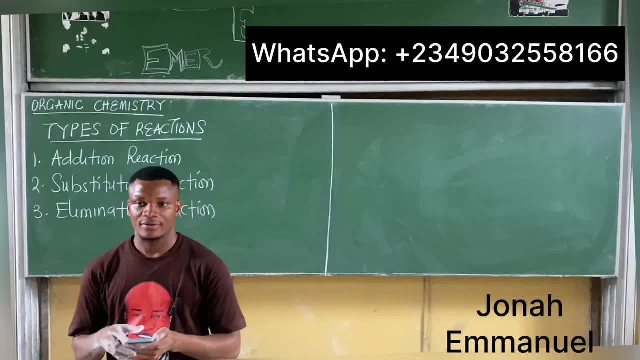 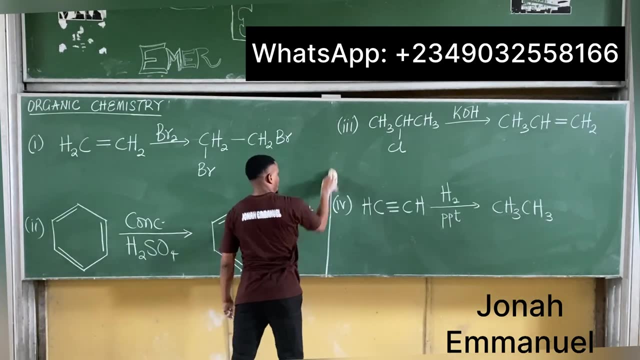 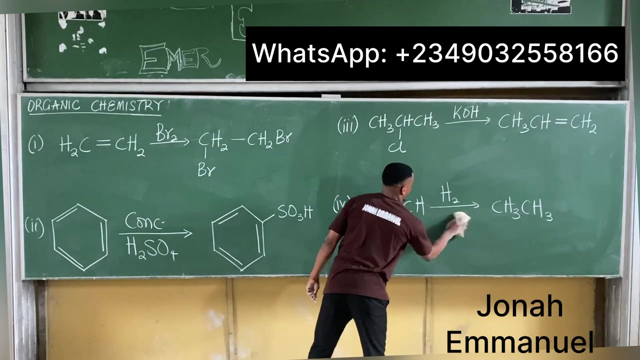 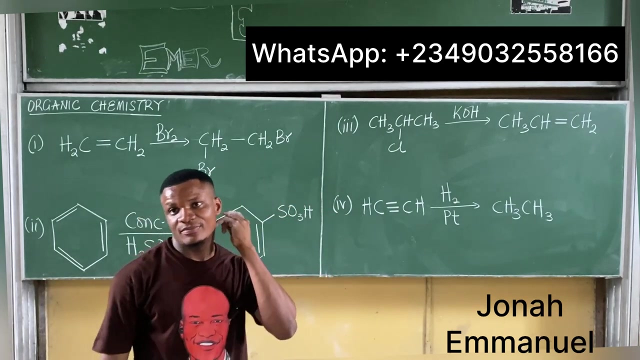 This can cause the hydrocarbon to form another homologous series. All right, let's take some examples and then we'll go and break. Yes, Yes, P-P-T, P-T-B-P-D-N-I, Platinum- I saw P-P-T there. 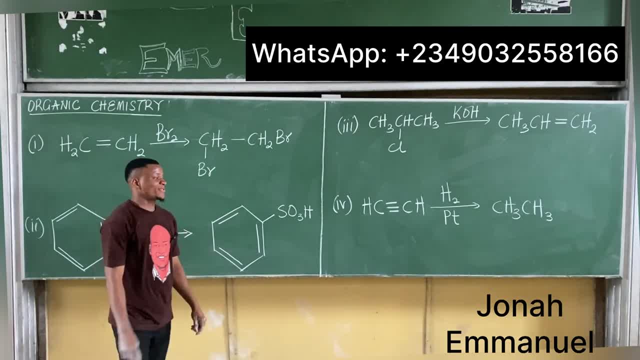 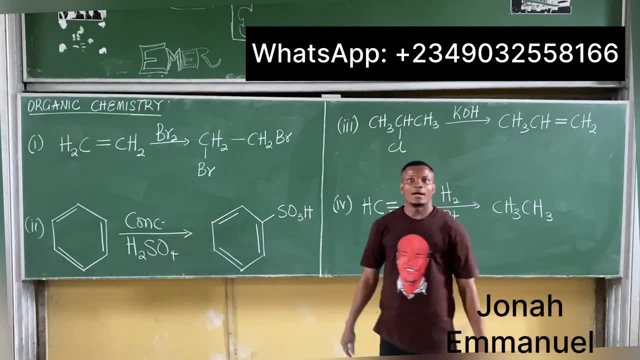 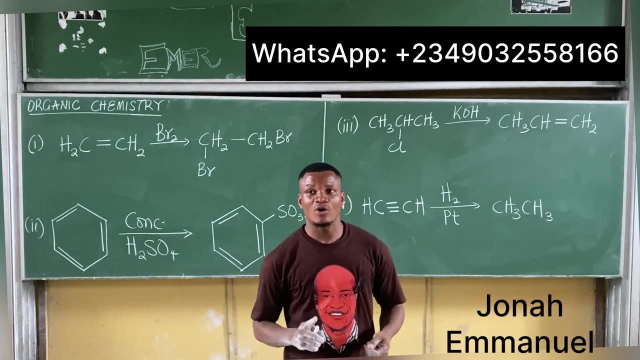 I saw P-P-T there. I saw P-P-T there. I was like, well, we'll throw it away. So look up. please Expect these kind of stuff. if not in tests in the exam, I would say for your test, focus more on how to name compounds. 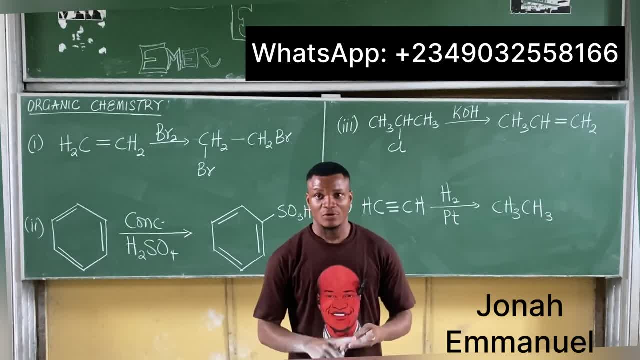 in how to draw the structure if you're given the name. We've done that before now, But let's get this man up, please. So classify the following here as either addition, substitution or multiplication. So classify the following here as either addition, substitution or multiplication. 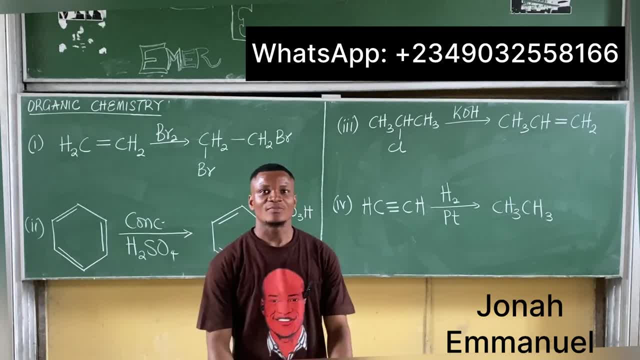 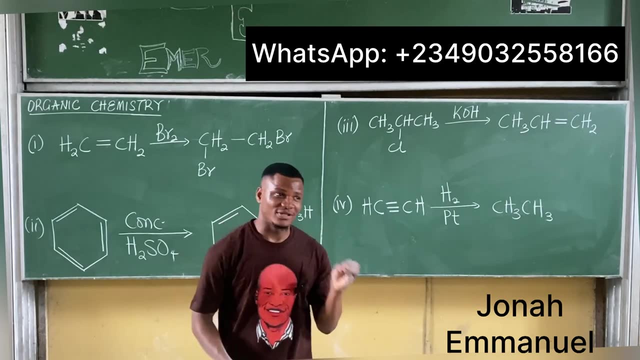 So classify the following here as either addition, substitution or multiplication or elimination, or, as we call it, rearrangement. look up, please. how is it done? listen, it's simple. for addition, the easiest way to spot an additional reaction is that a complex structure is broken. 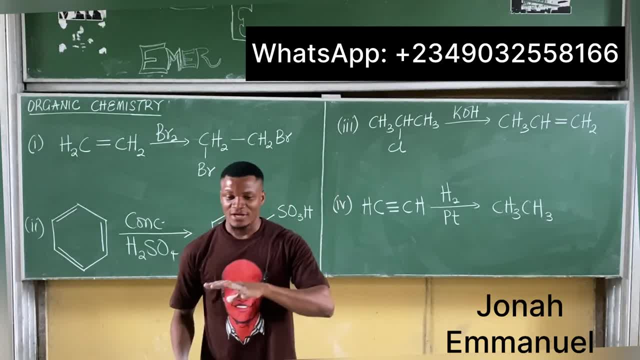 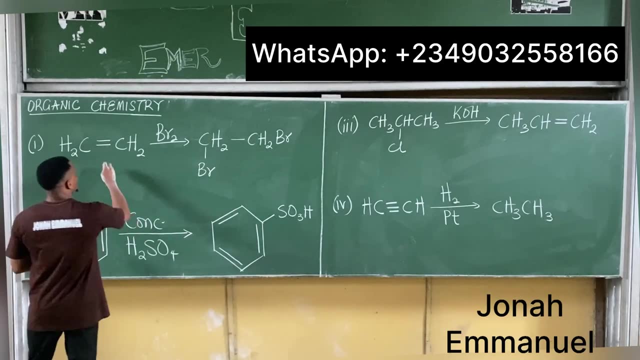 down to a simpler one example. is there any one that involves our kin or our kind breaking down to alkin or alkin breaking down to our king? anyone there, which of them, there number one, al king, is breaking at the water? al king, this one number one. here is an additional reaction. 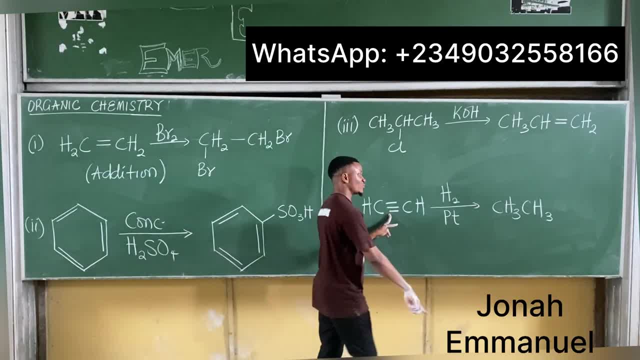 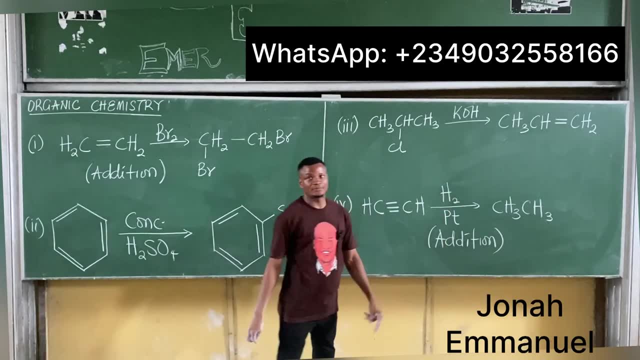 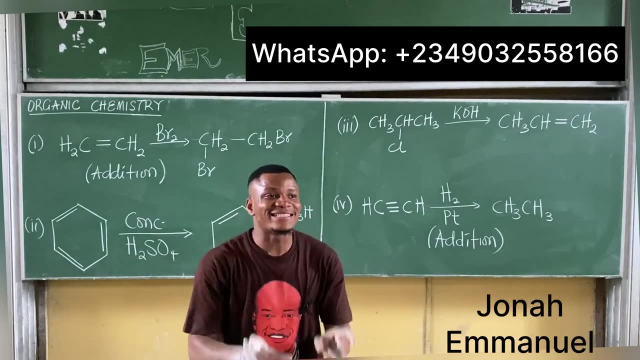 number four: al kind is breaking down toward there. okay, it's an additional reaction. that's number one. number two for substitution: check. very well, for the two sides i will have exactly the same structure, just a change in perhaps an attachment. please check, is anyone that has the same structure on? 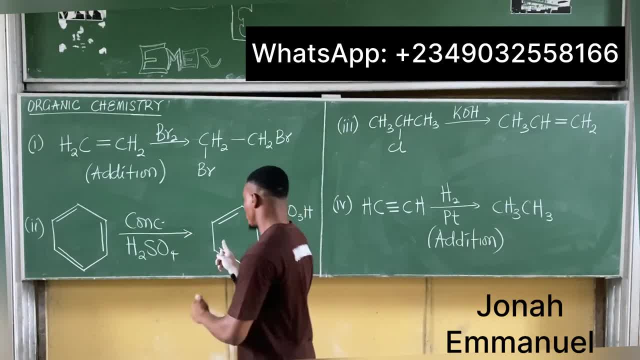 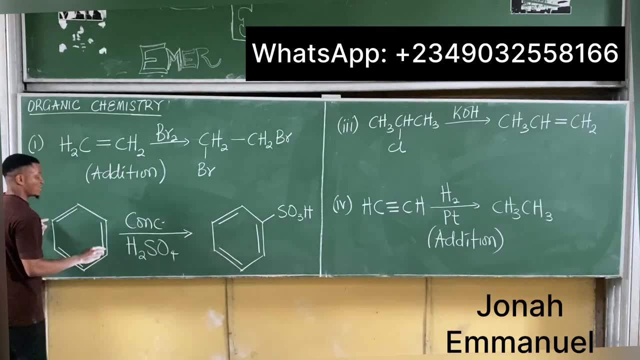 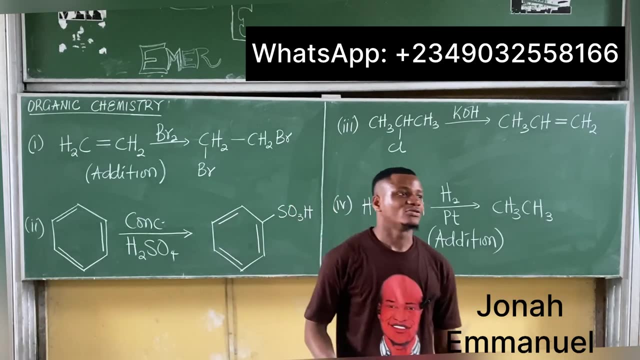 both sides. which of them is that? number two, please observe: this is a benzene ring. this is a benzene ring. the only difference is that this is called. what about this structure? no, the man's name. now, we did this in a previous class. this is called kekulé structure, we said. we said benzene was. 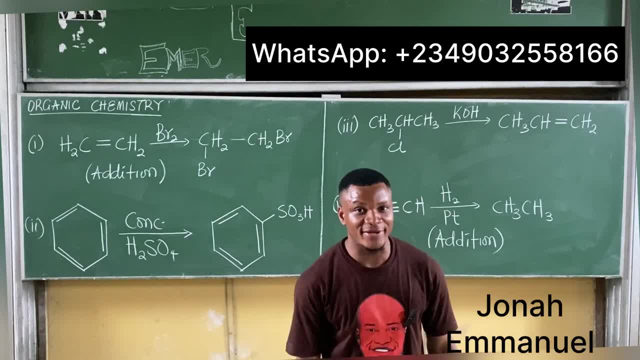 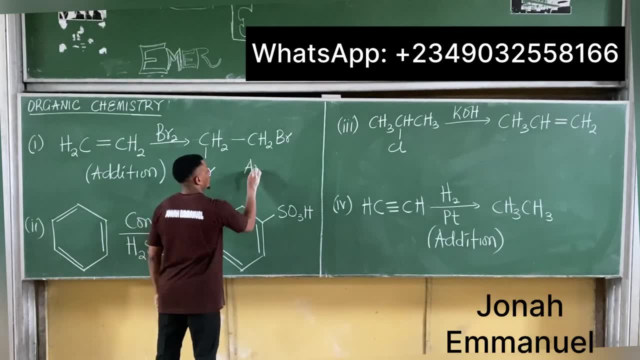 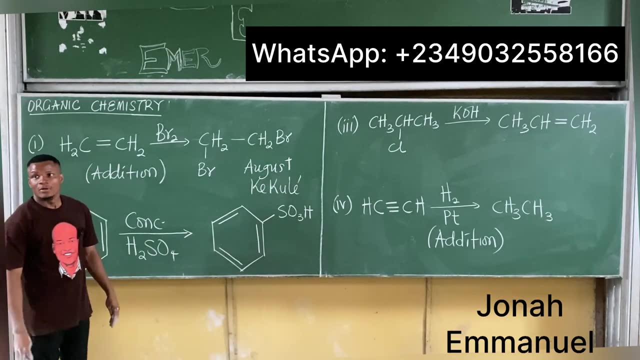 discovered by a man called what there? august kekulé. abhi, that's, that's another exam question. august, that's the name. all right now, listen, listen, observe that this and this are the same thing. the only difference is that for kekulé structure here is supposed to be a hydrogen. 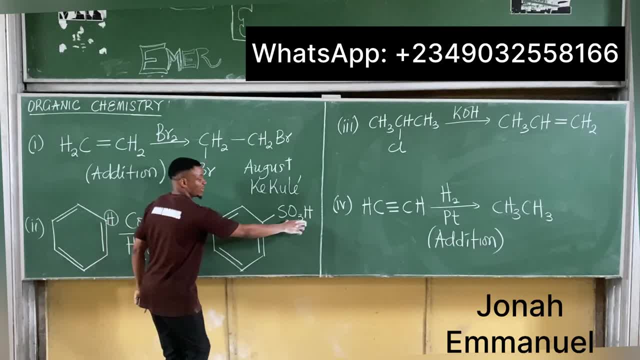 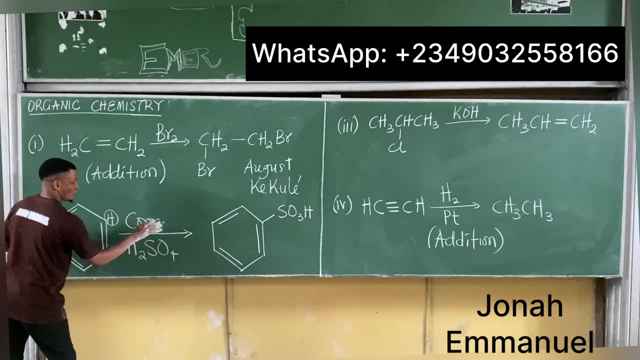 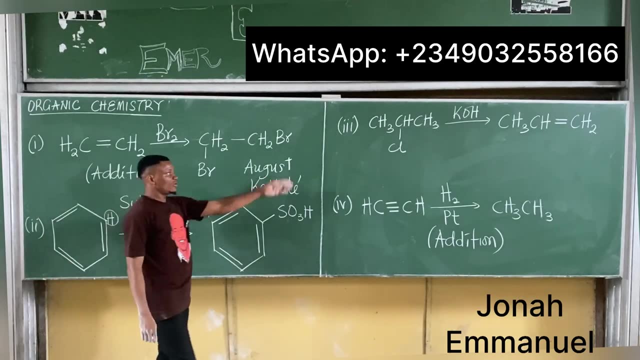 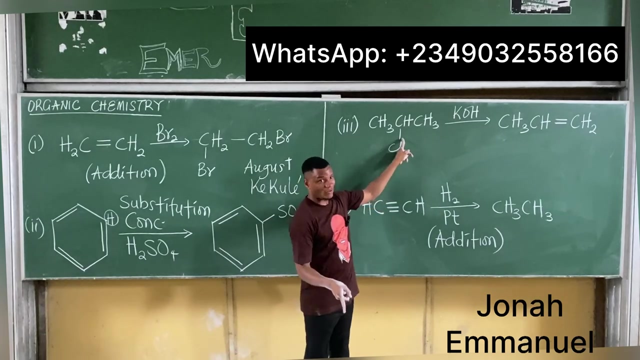 the hydrogen here has been replaced by this one here. so this is because what there? substitution reaction? uh, where do i write that one? yeah, uh, let me write it here. so what you have? number two is substitution. look at three critical. number three: observe that the reactant is not breaking down. it's from alkane to alkene. 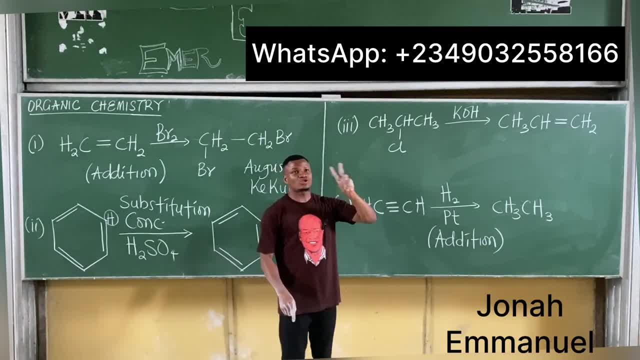 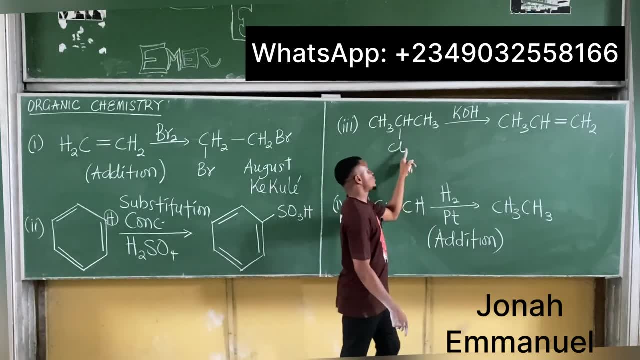 it's not breaking down number one, so it's no addition. number two is not the same thing on both sides. azimuth was just alkyne, alkene, and maybe this one was changed. that said, it's what substitution, but then object became what there? an alkene? it's not like saying for um an elimination. 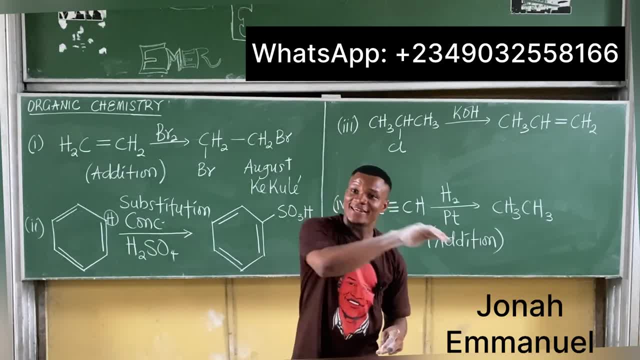 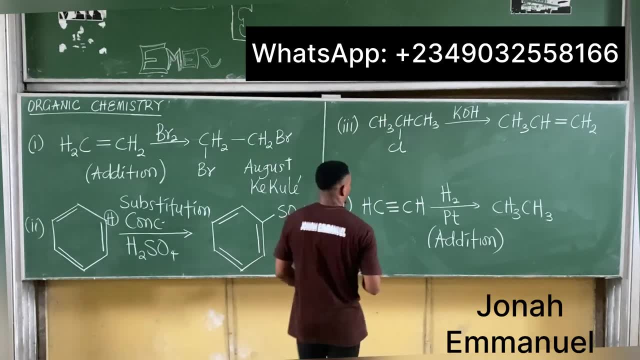 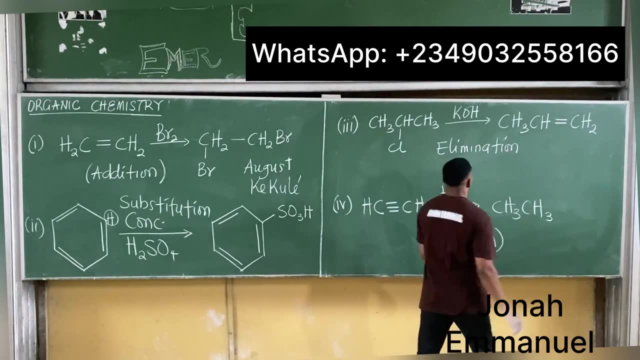 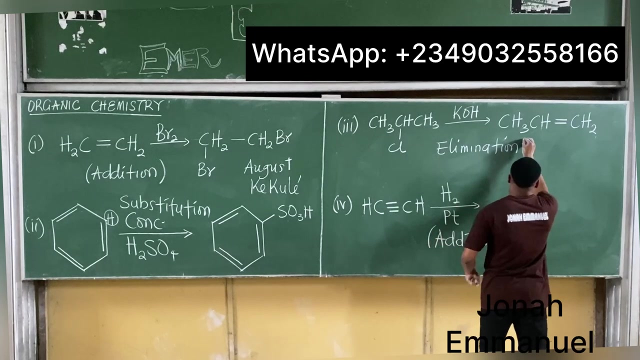 it's more like a build up process. so if it is breaking down, it's most likely addition, if it is building up, it's what there most likely. what there becomes. uh, this one's actually dehydration reaction. dehydro halogenation, please sorry, uh, halogen, Dehydrohalogenation. 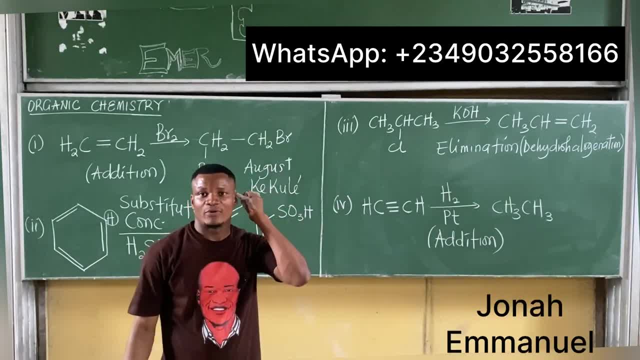 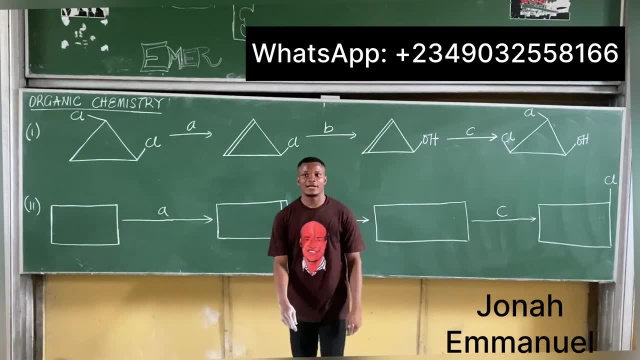 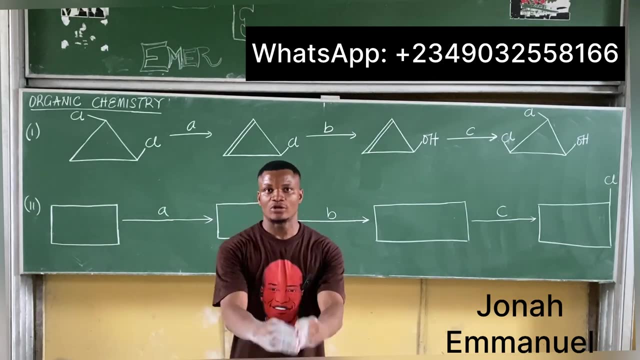 all right, so that's how this is done. let's look at the cons. one�ive podría. so alas, tax, please. before. that's a last action before a break, allow stats please. so alastax, please before uh break. it was good. identify each of these as either addition, substitution or elimination for. 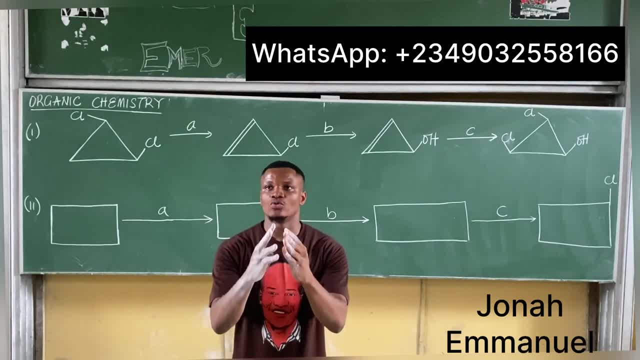 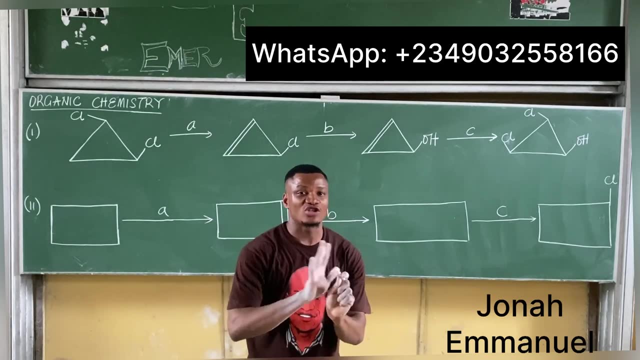 both cases, that's one and two. your easiest one to do is always substitution, always your easiest. so if I were you, I won't stress much, I'll get substitution for each of them. for substitution we say, the compound itself does not change. come to the first one here. which one do I have? a structure where it didn't really. 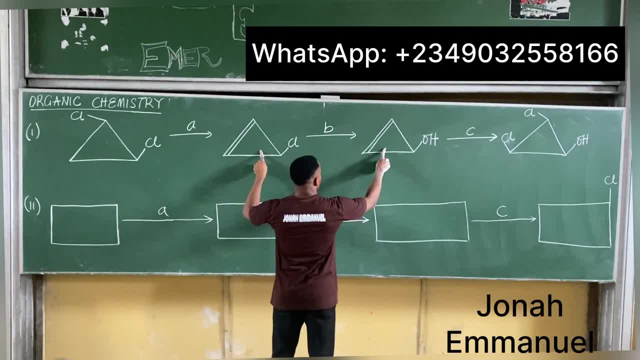 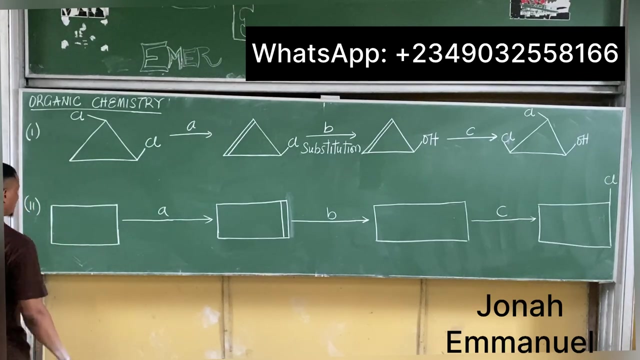 change. that's this one here. observe, so observe that this two are same thing there. the only that happened was that here was what substituted with this, so B becomes what there substitution. the substitution is that simple. that's for the first one, for the second one, which of them will go substitution? this was our king to our king. 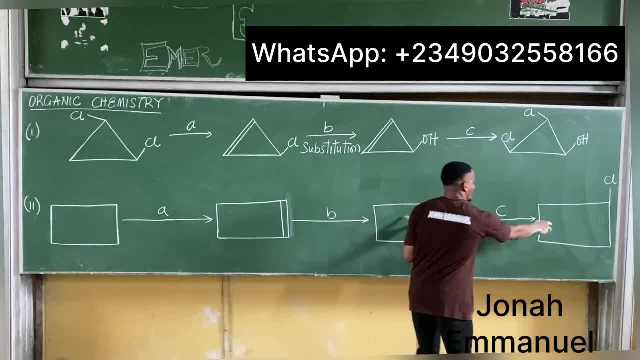 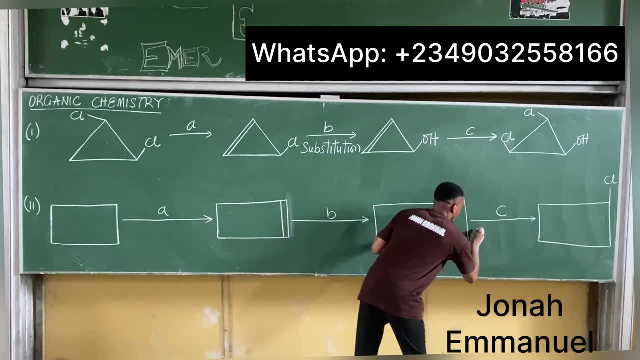 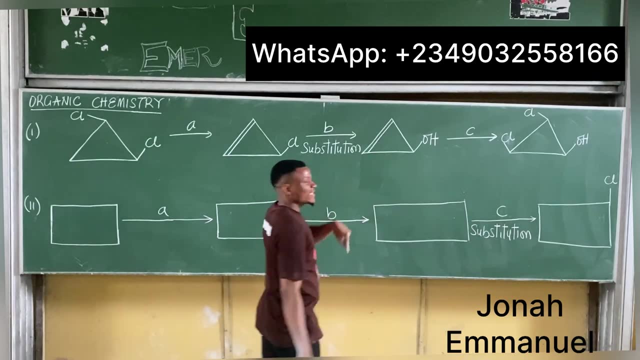 our king to our king. observe here: C is alkane, and alkane, Just like hydrogen, here was replaced by what there? Chlorine. So this one becomes what That's always like, the easiest one to get. The next one to get is addition. I think addition is easier, For addition, the complex one breaks down. So 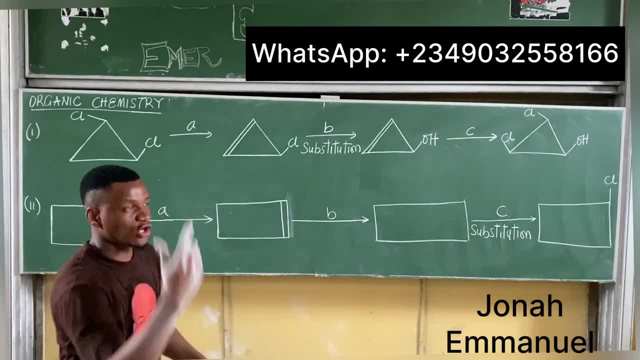 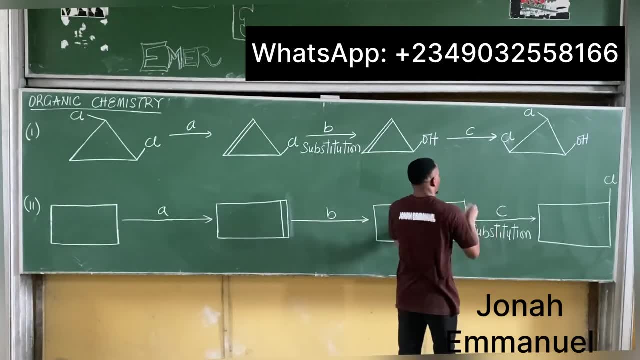 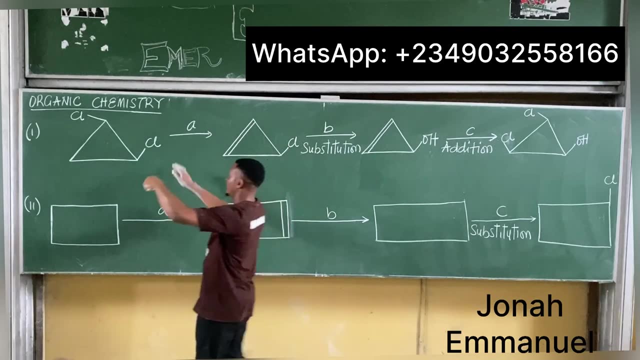 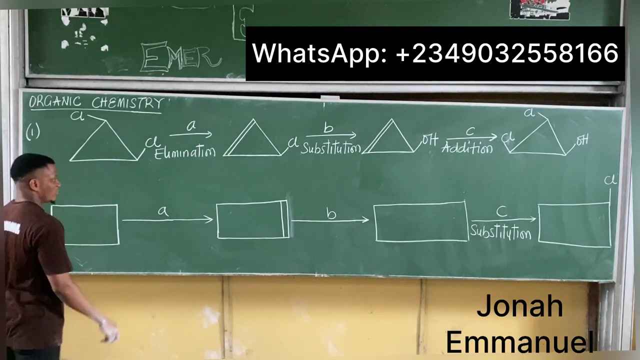 what do I have? Double bond to single or triple bond to double? What do I have there? Observe C: from double bond to single. It has broken down. That becomes what there, What we say for building up. It becomes what there. All right, Coming to these two, which of them? 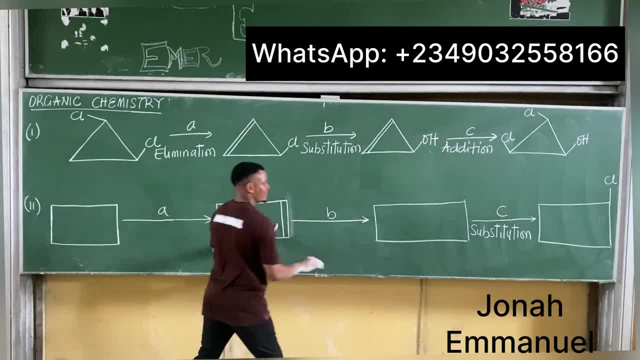 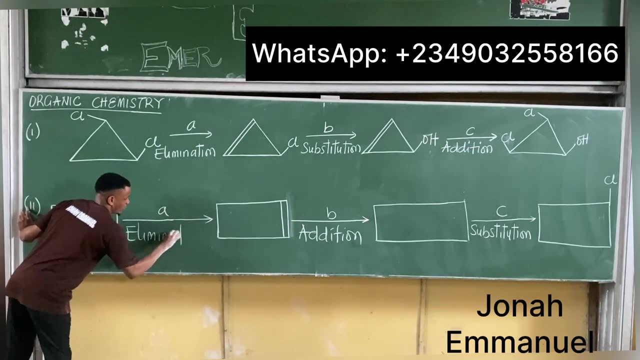 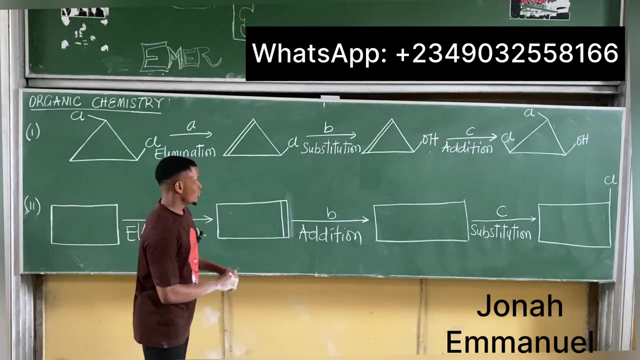 there. From here to here it has been broken down from an alkane to what there, An alkane. So it becomes what there. Addition: That becomes what there. All right, Most likely in your test or exam you will see this way. Listen, You will see. 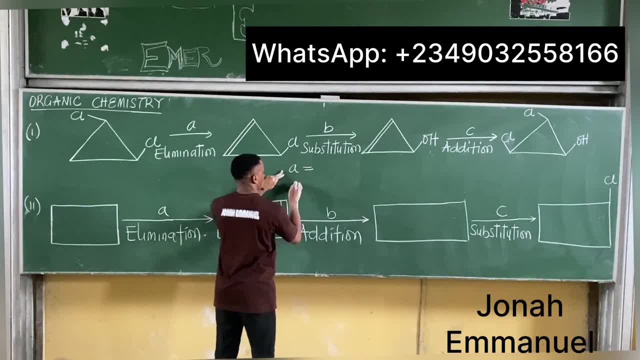 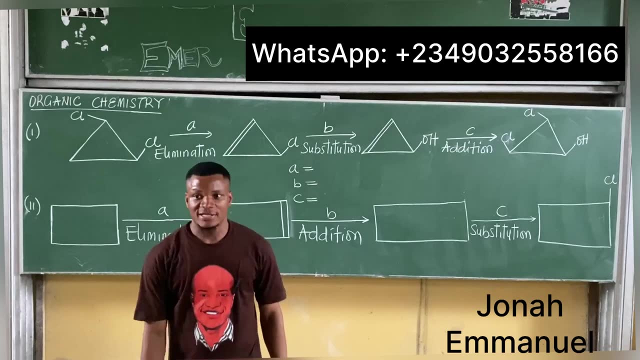 this stuff here. It will now tell you: A is equal to, B is equal to, C is equal to. For this one here, A is equal to elimination, B is equal to substitution, C is equal to what there Addition Any questions? All right, Let's take a break, please. Let's take a break. 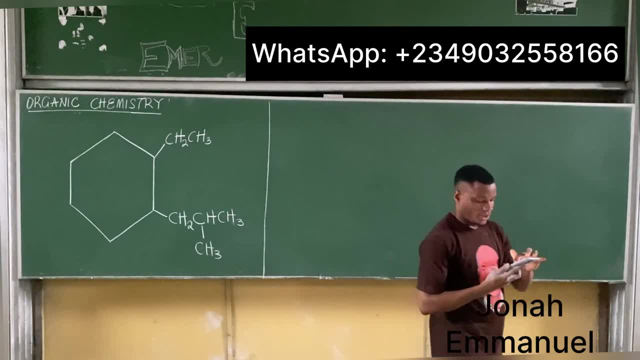 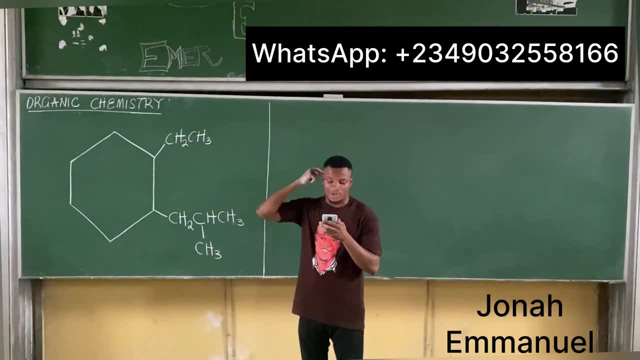 All right, Let's take some past questions please. So this is from 2021.. The question says how many? That's this question 2 from 2021.. 2A says how many primary carbon does this stuff have, How many primary here? 2B says how many secondary. 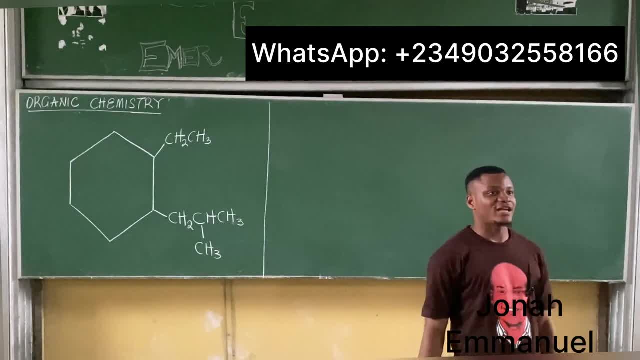 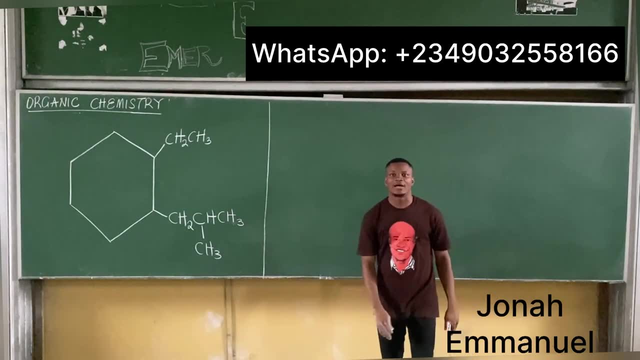 Does it contain? 2C says: how many tertiary carbon does it contain? So please, on your own, please, very fast, please, Write out how many primary carbon you see here, how many secondary carbon you see here and how many tertiary carbon you see here. please. 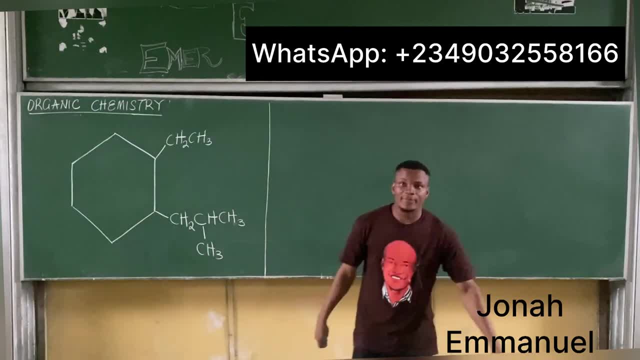 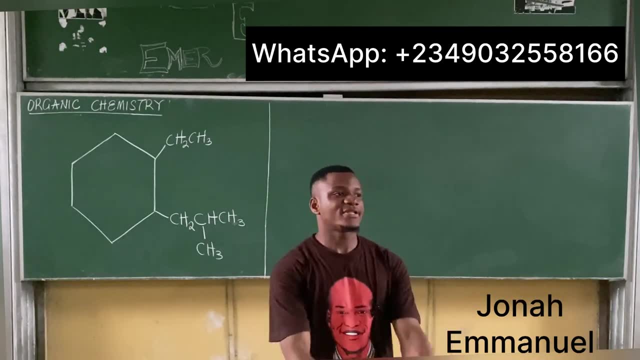 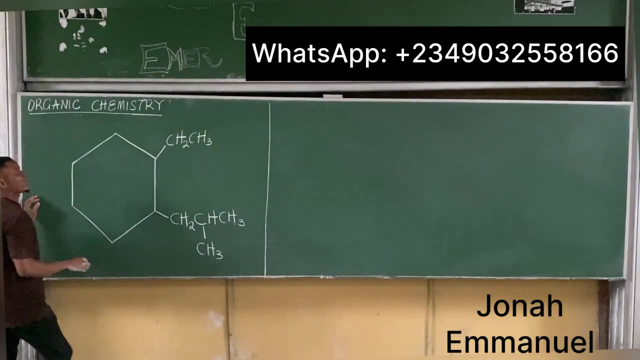 Very fast, please. All right To look up, discover the number of primary, secondary and tertiary carbons here. It all boils down to how well you know structures. First, it's very easy to get. I think these ones are easy to get. Let's try to see if we can get carbon. 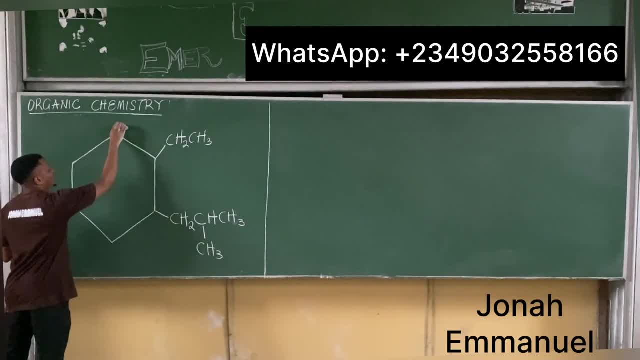 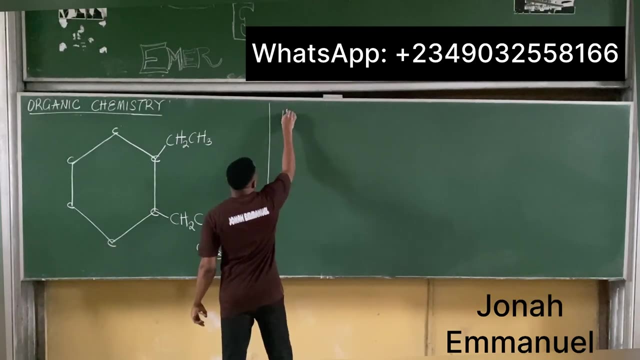 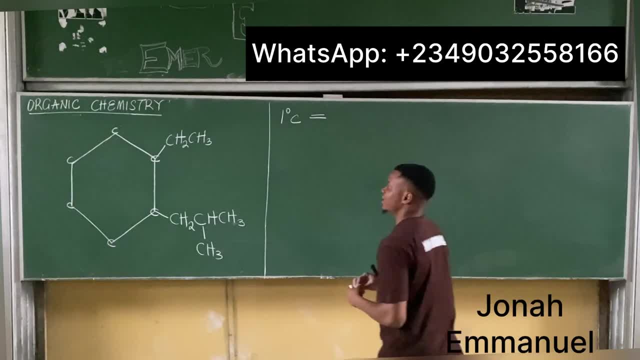 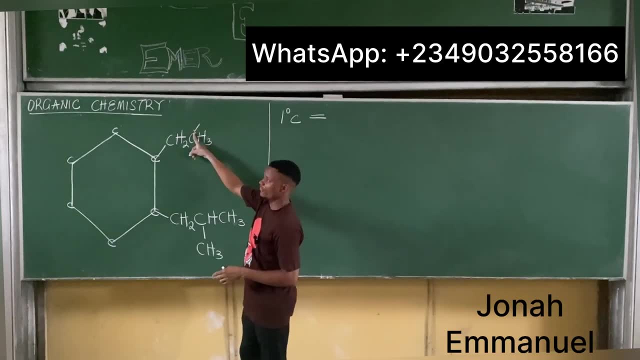 Almost always attached to 3-hydrogen. If I look at this very well, I said it's at the extreme. My primary carbon here will be this one here, this one here. of course, at the extreme, This one has just one attachment, which is all of this. So that's the first primary. 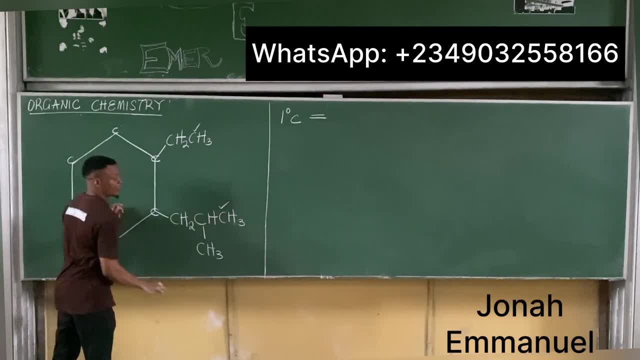 The second primary will be this one here. This is a primary because this one is attached to all of this. More like I can detach this from here and I'll still have this one here. The third primary I have is this one here. Of course, this one has just one attachment. 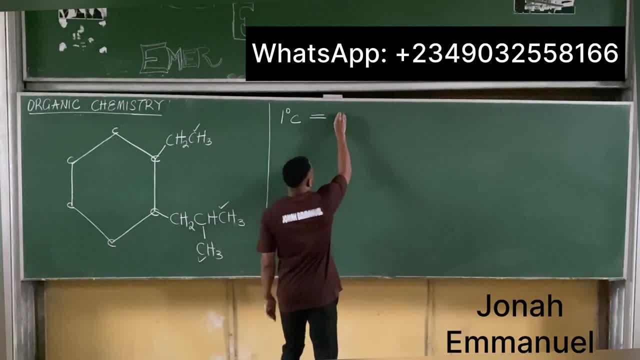 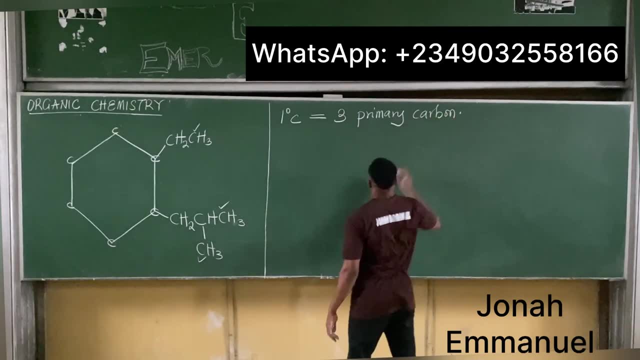 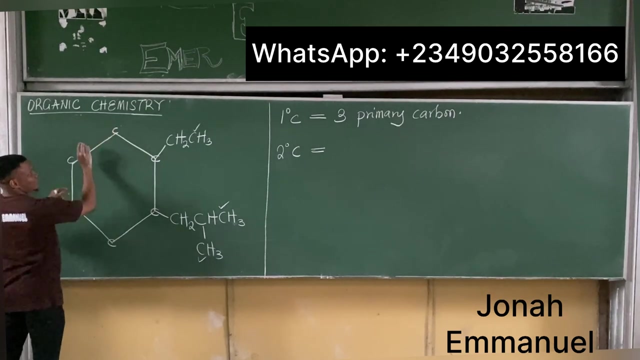 to all of this. So I have three, Three primary carbons. Let's get secondary carbon. For secondary carbon, look at those carbons that have two attachments. One of them will be this one here. This one has two attachments. This is okay. let me call this hold on. let me call this primary, Let me. 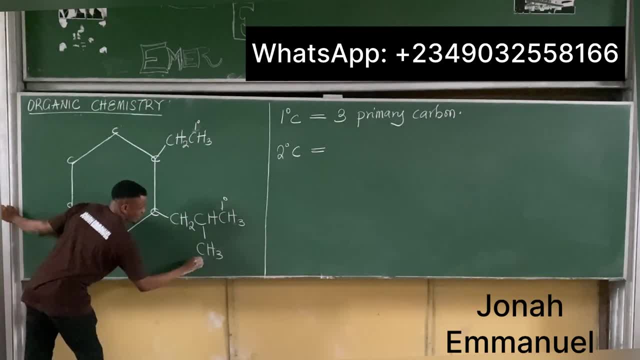 call this one here primary. Let me call this one here primary. This one has two attachments: This is secondary. This one has two attachments: This is secondary carbon. This one has two attachments: this and this. This is secondary carbon. This one has two attachments: this and this. This one. 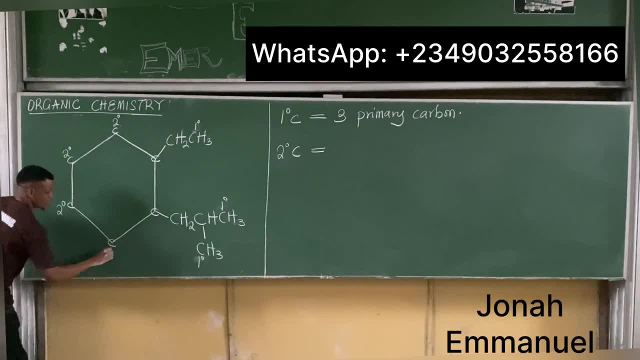 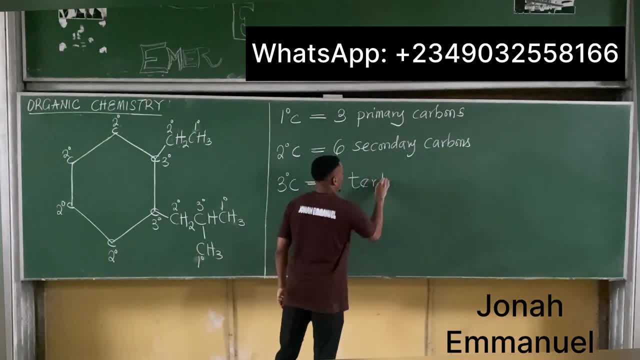 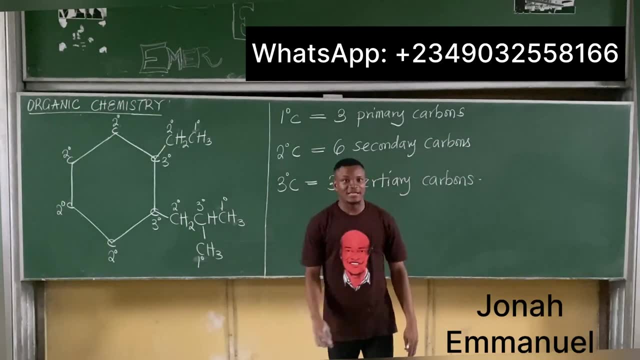 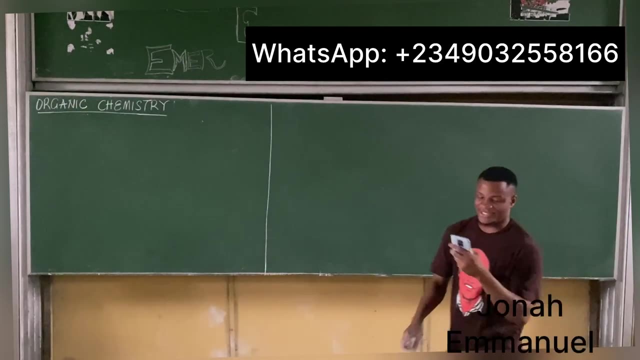 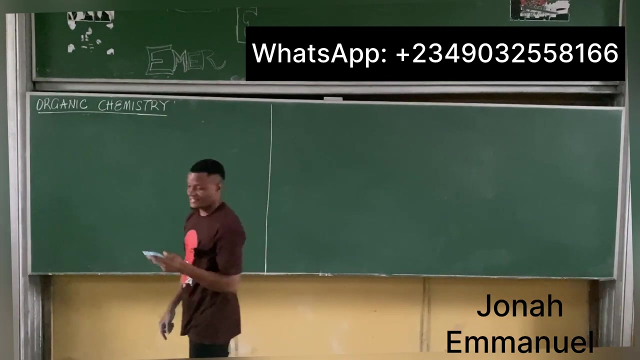 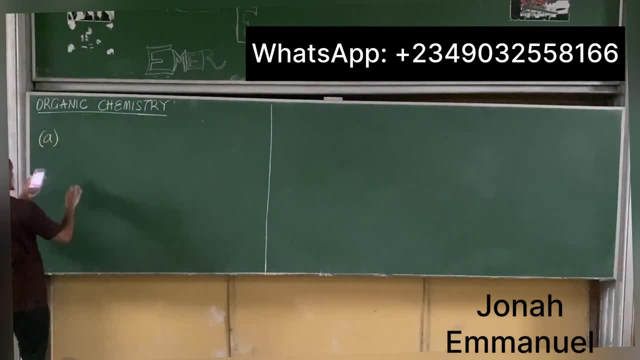 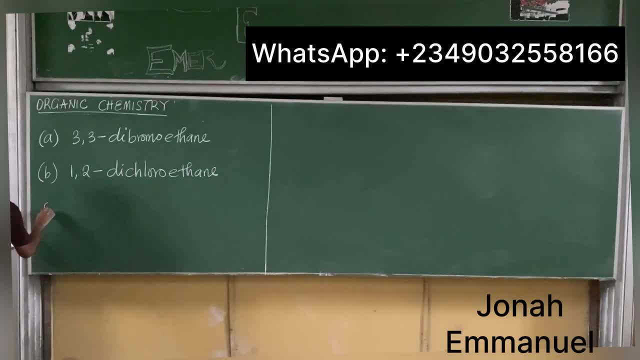 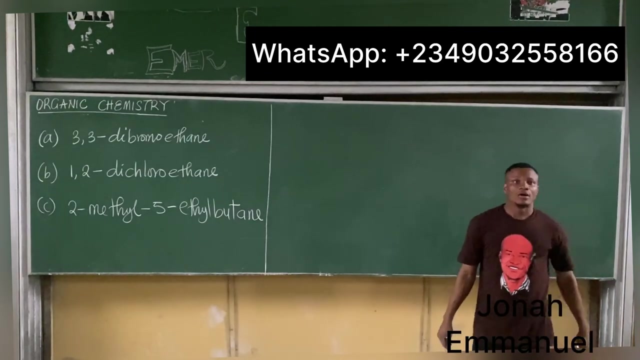 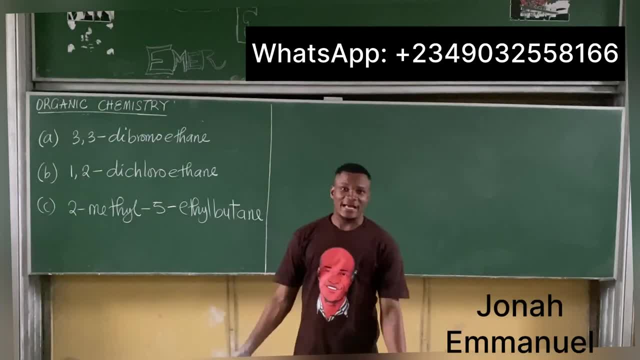 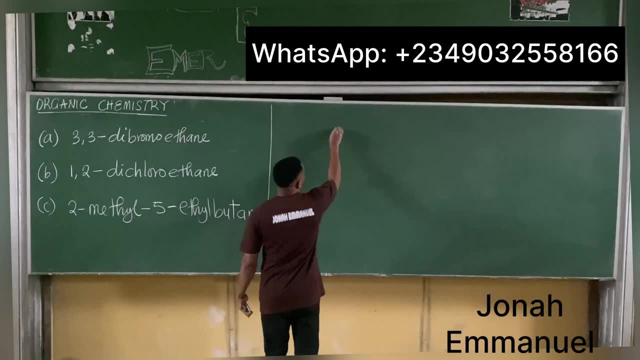 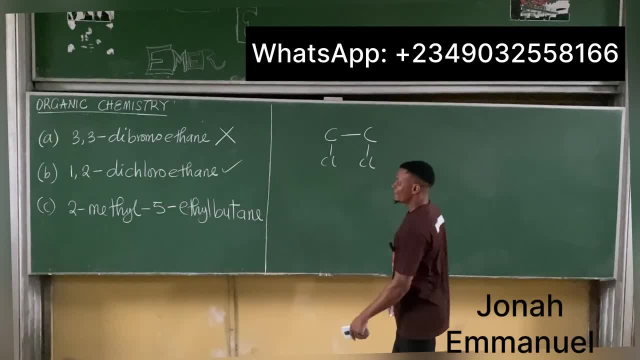 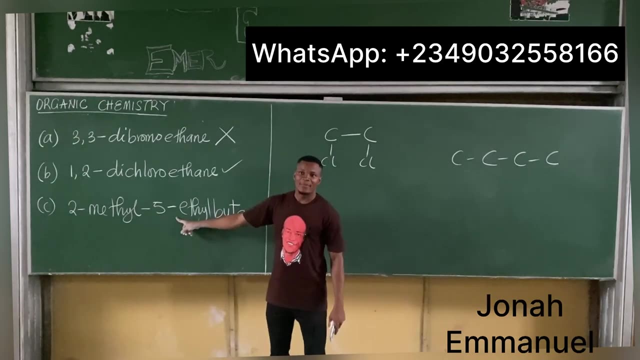 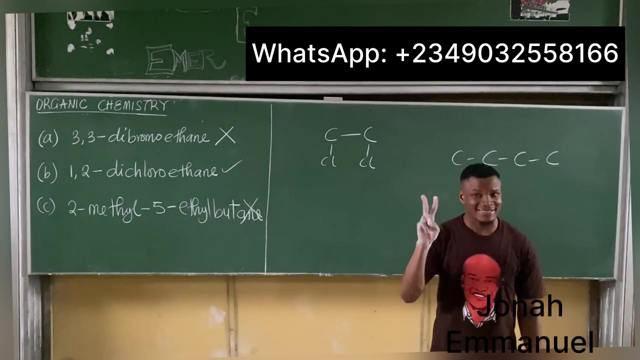 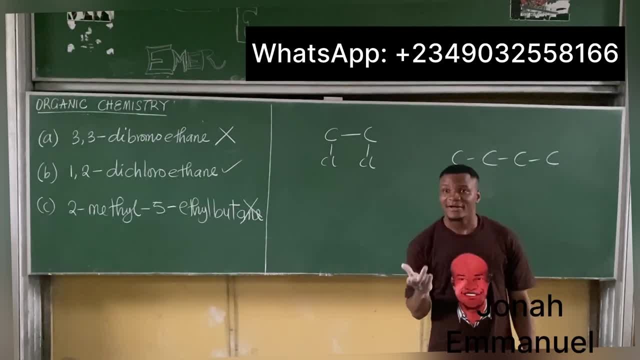 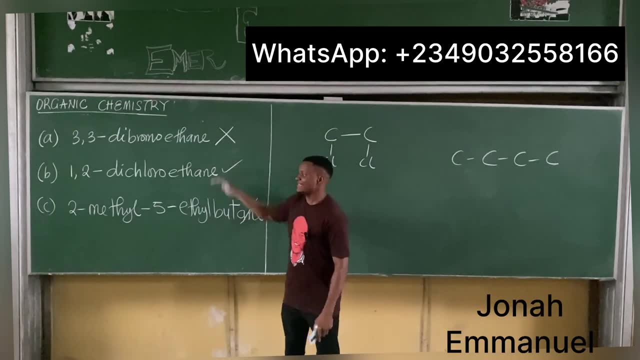 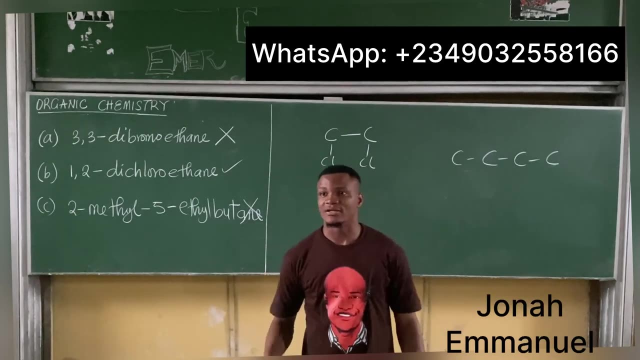 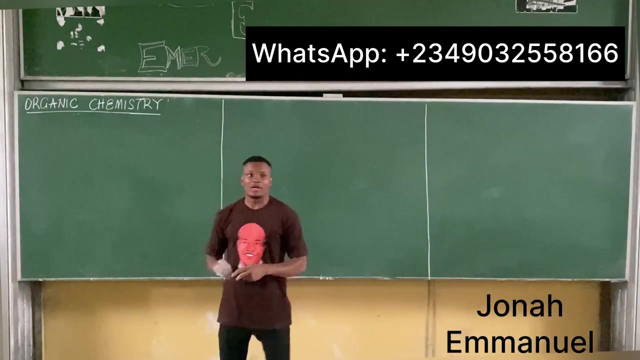 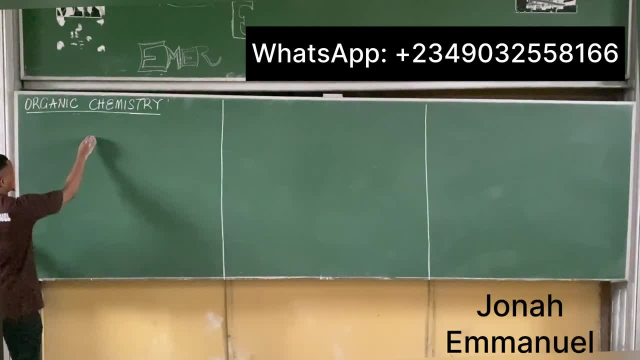 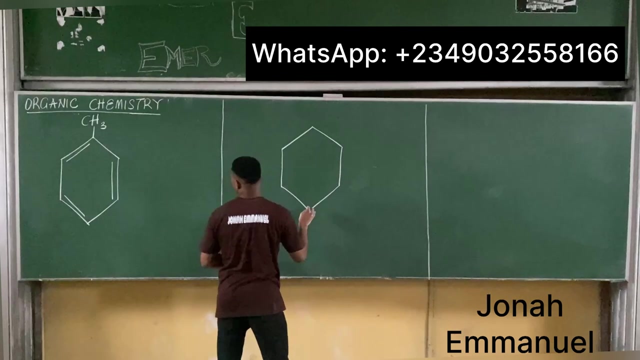 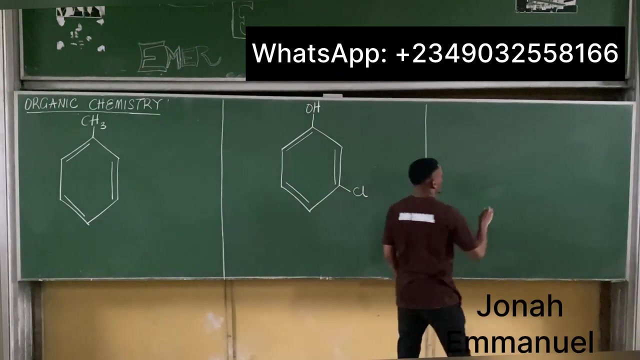 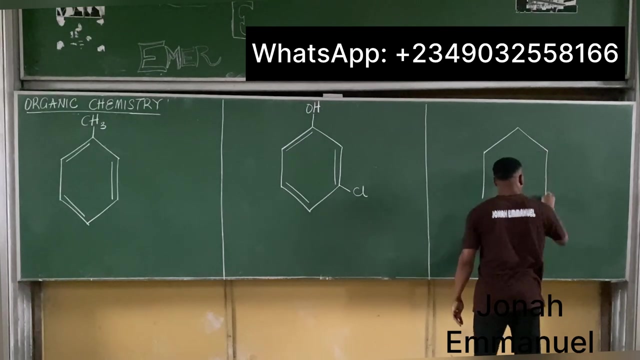 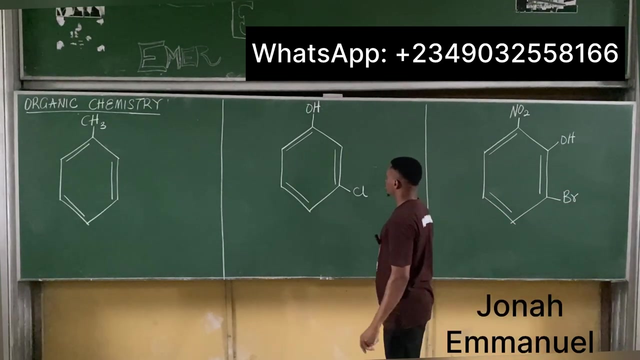 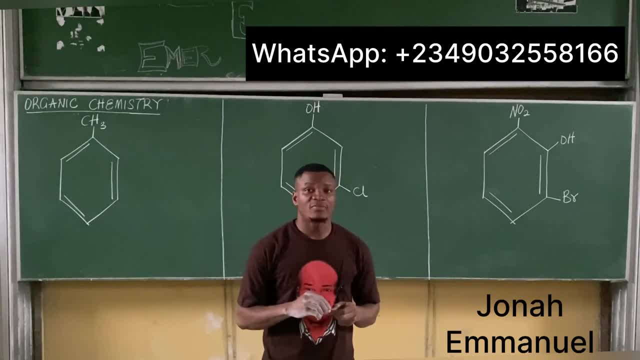 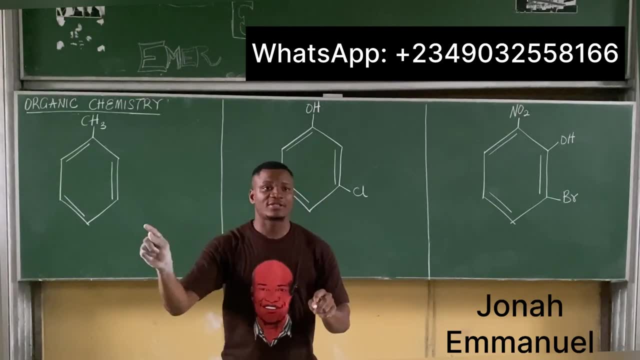 Look up, please, very fast. please Listen, please, before you go, look for where to get our notes, My notes. I've gone through the past: patients, the so-called reactions, as some example in my notes. All right, 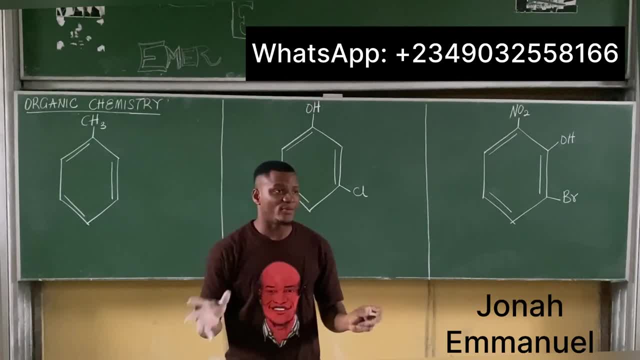 All right, I can't start going through all of them again. I'll just pick a handful of them that I think are important. Please go check them. Get notes from whoever has a note. Let's see how we can name these please. 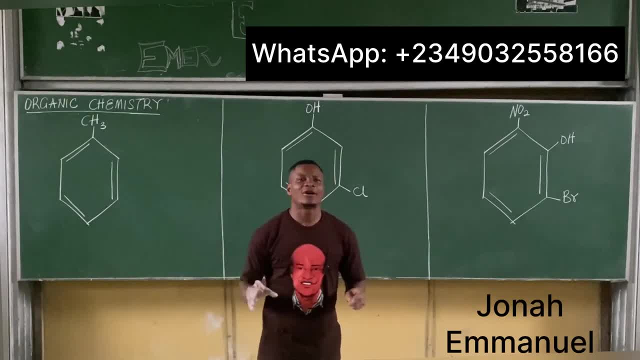 I have to bring this one back, so I'll show you something. There's something peculiar about naming of the benzene and benzene derivative. We talk about benzene. When we did in the last class was it last class Two, two class ago. 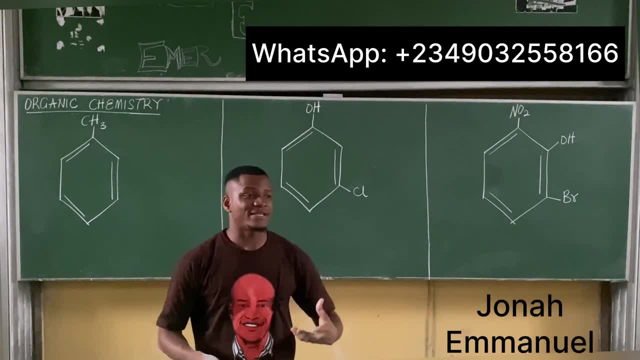 So we did benzene and, okay, we did the aromatics, And we said benzene and toluene Are the proper aromatics. And we said there's something called benzene derivatives. We talked about something called toluene. 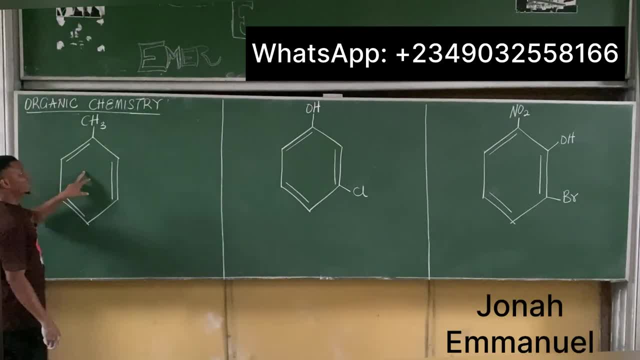 Toluene is simply what there, Benzene is what there, A material, What you have here is called a toluene And in this class, I gave you toluene, I gave you styrene, I gave it again there, naphthalene. 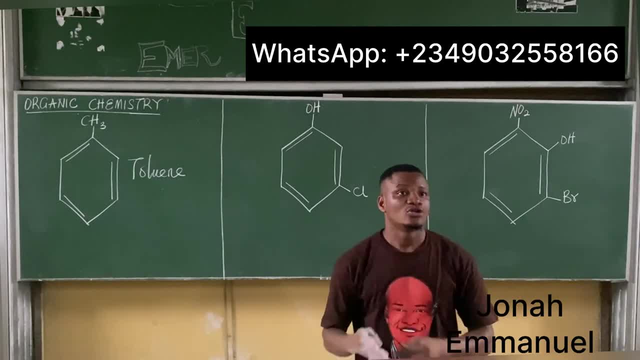 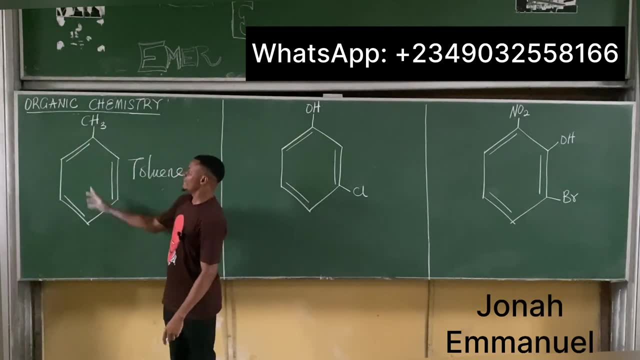 Are they? Yes, Yeah, So I gave you different structure. Please go check it out. So this one is called a toluene. When you have benzene with CH3, it's called toluene. When you have benzene with OH, it's called what there? 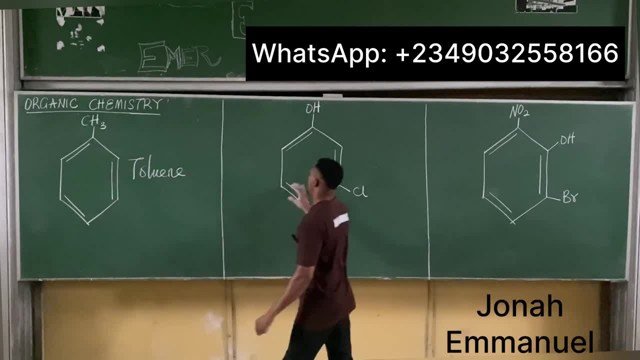 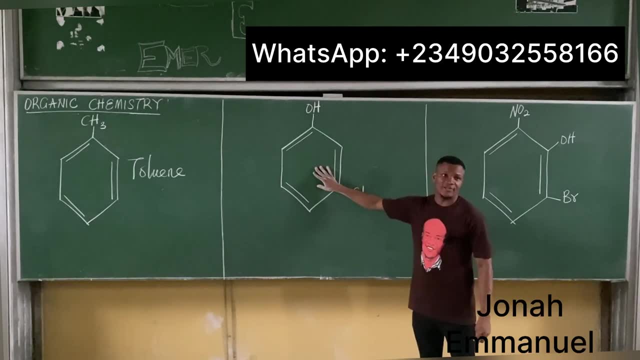 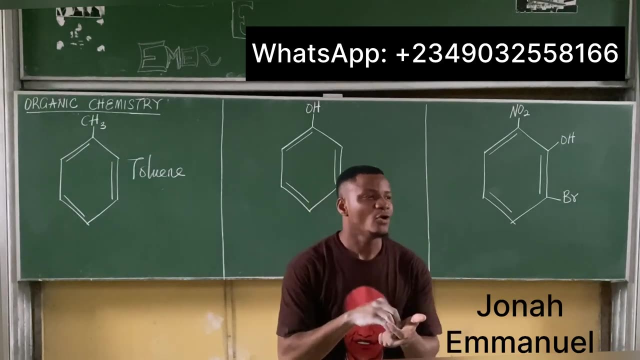 Phenol, Phenol. It's called a phenol, By the way. come back to this, please Come back to this, please. Now, something peculiar about benzene that we mentioned was this: Always note the structure For a benzene structure that has two substitutes. 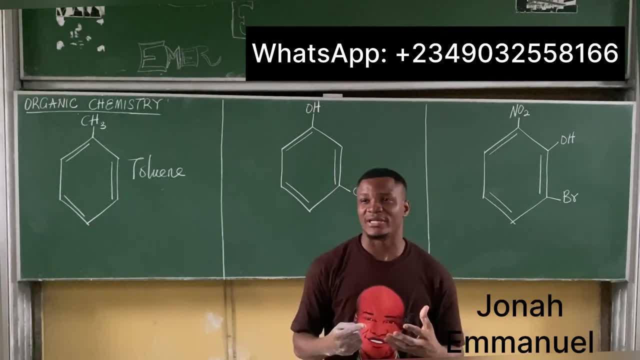 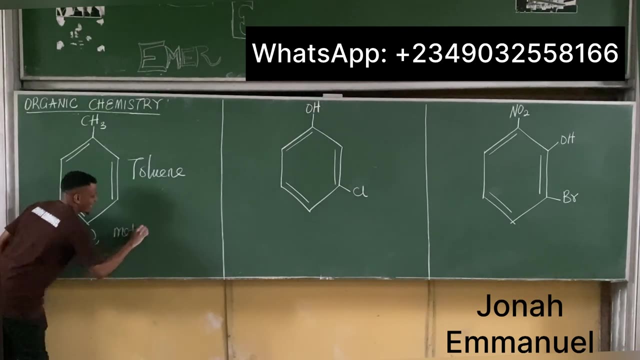 It has two substitutes. It has two substitutes, It has two substitutes And it becomes what? there? An OMP concept. We talk about OMP concepts. OMP is called the auto-meta-octo-o, meta-m and then para-b. 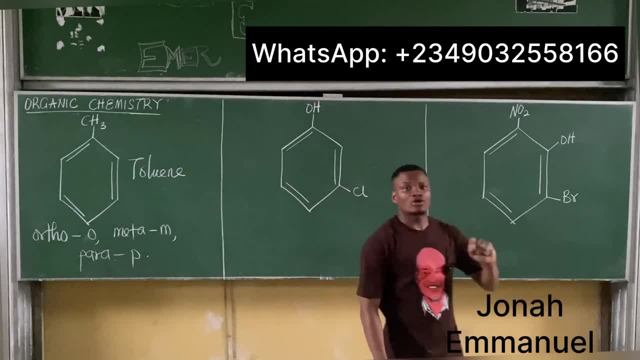 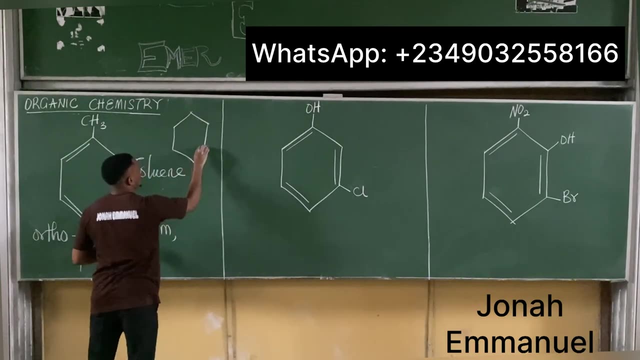 Listen and listen carefully. Auto meta and para is only used when I have two substituents, substituents on your benzene ring. there are, here's your, here are your positions, please. so here's my benzene. look up, here's my benzene, please. here is where your major substance attached, your auto has. 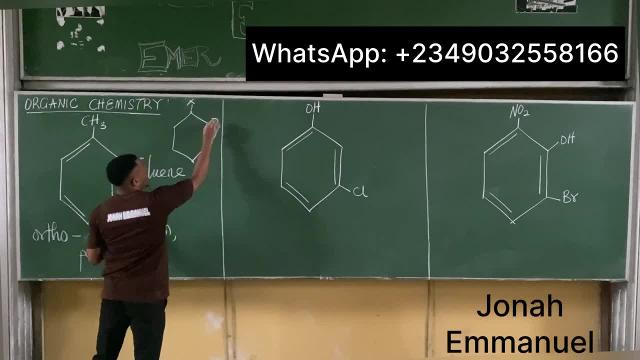 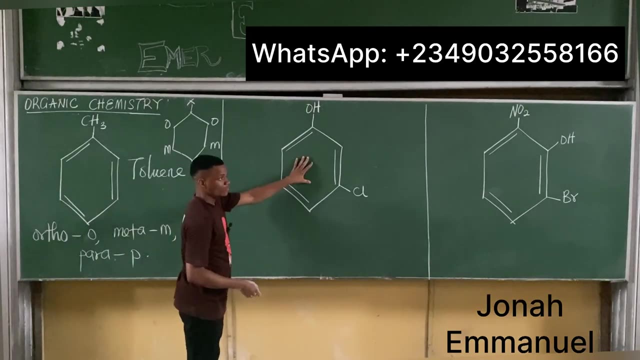 two positions. the auto positions are here and here, that's auto. meta has two positions. the meta positions are here and here. para has just one position and that's here. so if i have a benzene structure such as this, where i have two- again i'm repeating- it only works for two substituents. 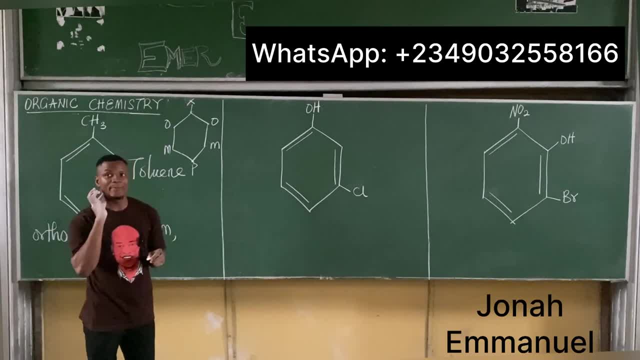 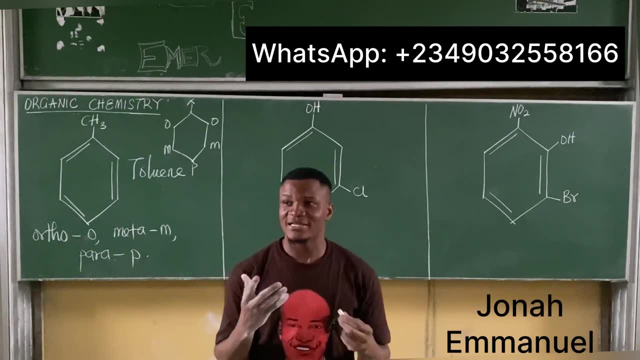 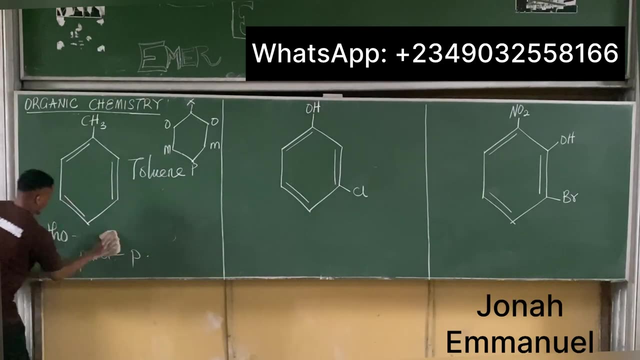 like this one. here i can now bring in the omp concept. how does it work? usually, benzene usually have what's called two different names. basically, i have two different names. the first name- the first name is when you consider the structure as a benzene. the second name is when you consider 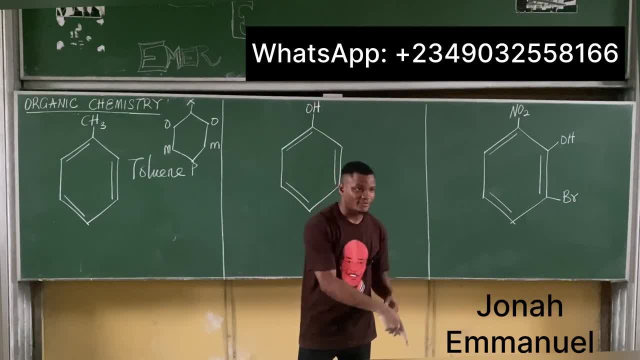 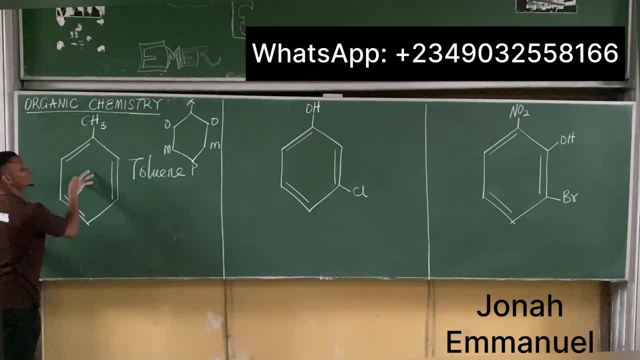 the structure as a benzene derivative. i'm calling this man a toluene because he's a benzene derivative. if i'm to consider the structure as a benzene, it means this one becomes the benzene and hence everything attached to this becomes automatically a substituent. if i want to look at the structure, 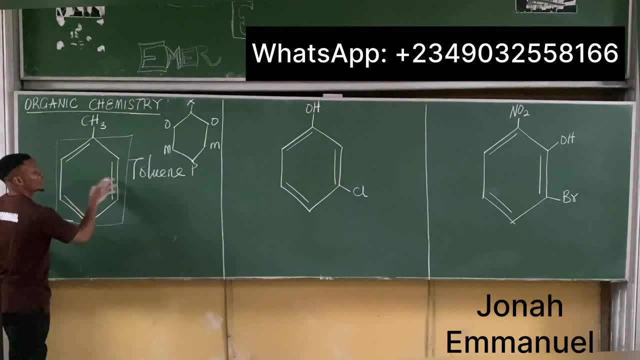 of this structure. So as a benzene derivative, this is called a toluene. But as a benzene, this one becomes a substituent. I will do my positioning. It becomes one. So it becomes what there One: methyl. 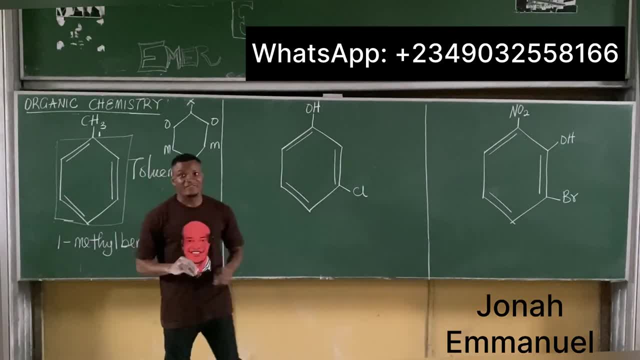 In case you are asked to provide two names, the first name will be calling this as a benzene derivative, toluene. or consider this man as benzene and call it a substituent One, methylbenzene. Same thing here. 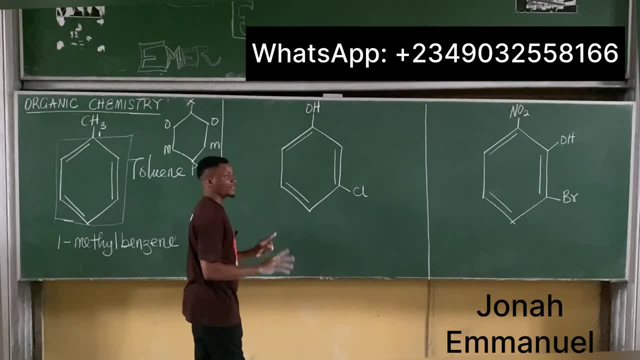 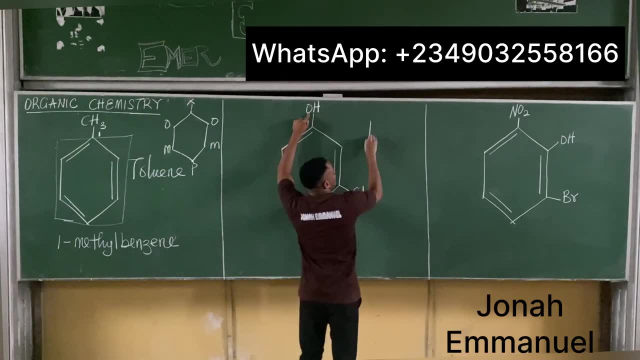 First things first. consider this structure as a benzene derivative. By benzene derivative I mean benzene with this one here. One benzene has an OH. It's called what there, A phenol. So as a benzene derivative this one becomes a phenol. 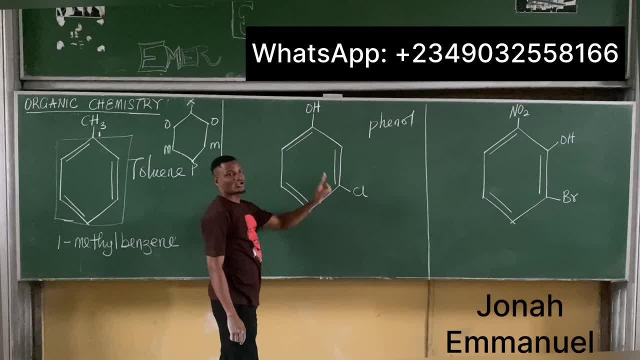 That's concept one. Concept two: Looking at this structure, I have just two substituents And we said: if you have two substituents, call it what there. OMP, Bring in. OMP. Observe that chlorine is at this position here. 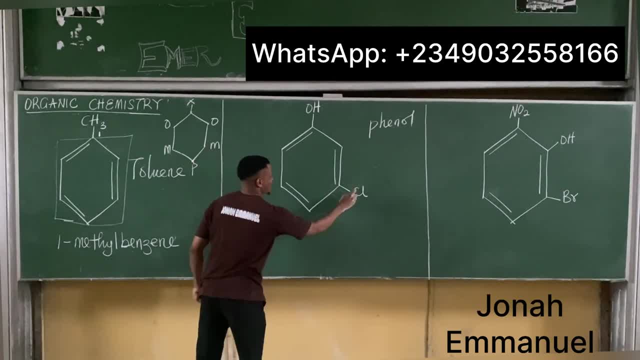 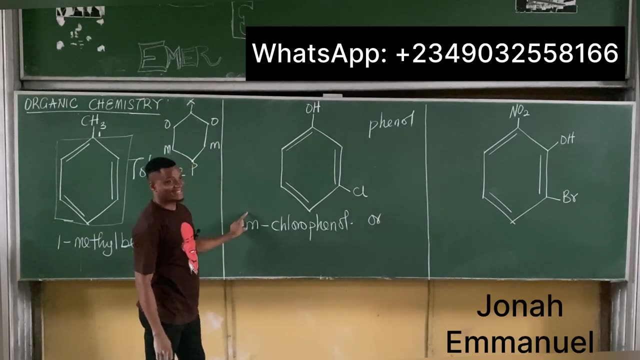 That's what there, The M position. So hence this becomes what there M: Chloro Enol, That's O. Or this is the best, Here's your best shot, Or you can choose to use numbering. 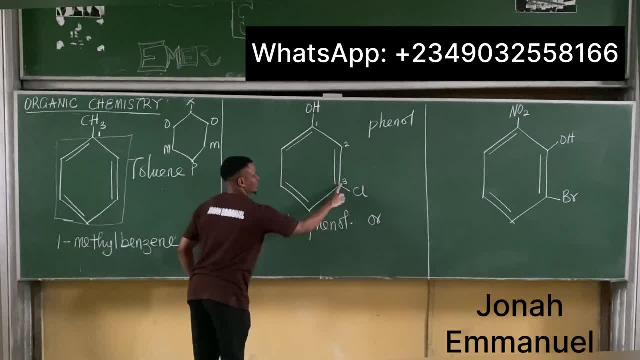 One, two, three. So it becomes what there? Chlorine, Three Chloro, Or Hold on. Hold on One, two, three. Stick considered as a benzene derivative, Phenol, Please. What is most proper is the M-OMP concept. 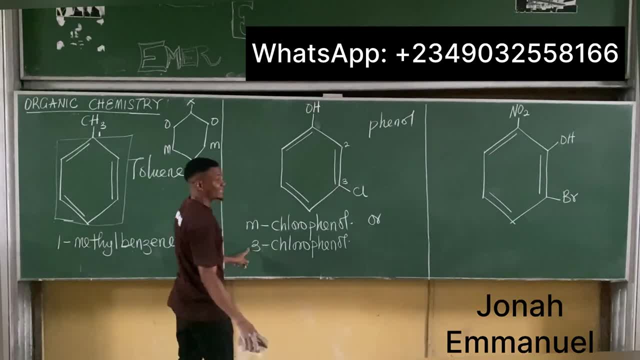 In fact, don't worry, Let me take off the numbering. But I'm saying this can still exist, But it's not the proper IUPAC name. But don't worry, Let's use OMP. So I don't get you off track. 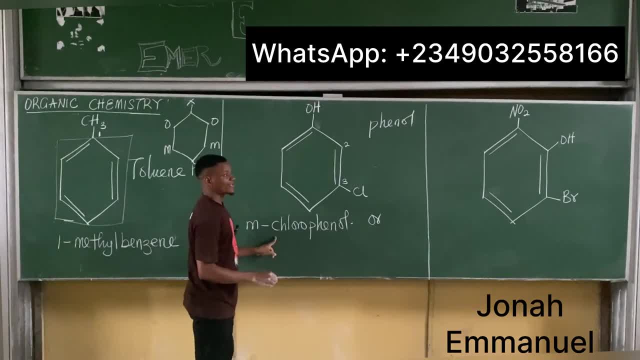 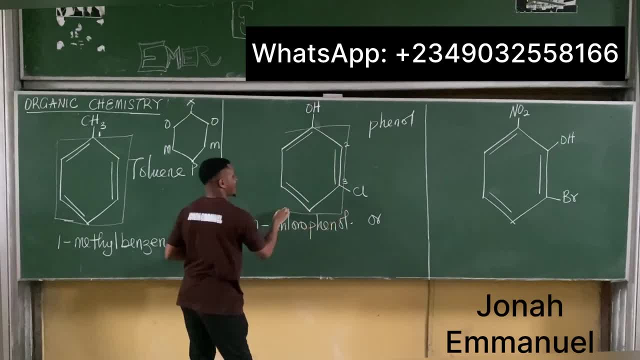 If I consider this as a benzene, it means that everything attached to it becomes a sub-subtract. So these two are now sub-subtract, No longer phenol, but now hydroxy. So I'm having one, two, three. 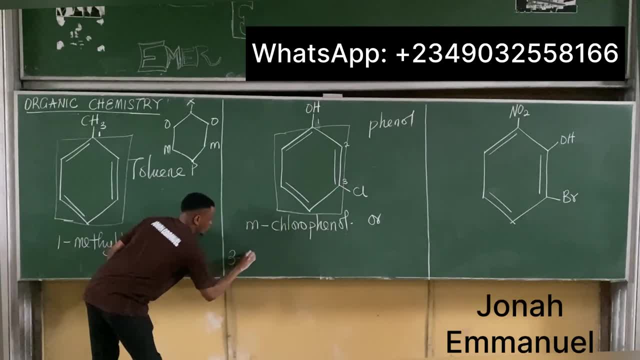 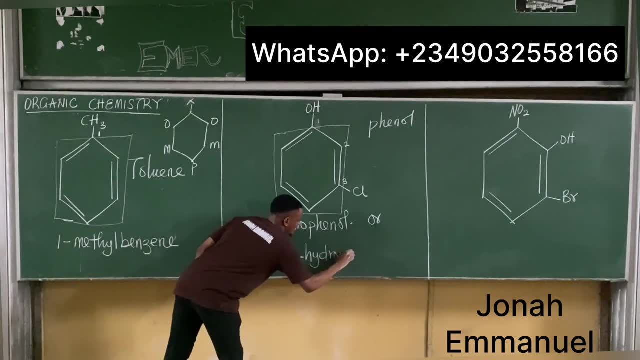 So because what there Becomes three Chloro One, Hydroxy, Hydroxy, Hydroxy, Hydroxy, Please. in the hydroxy, the L is not attached Hydroxy Benzene, So please observe. 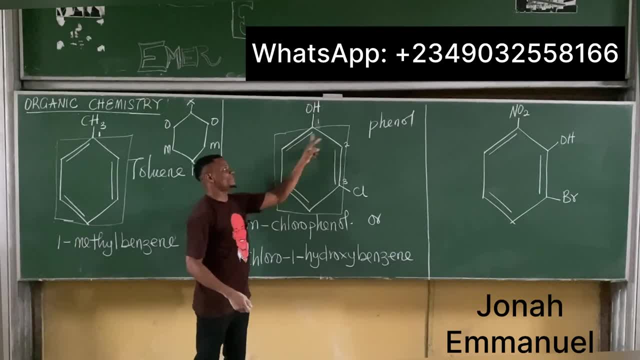 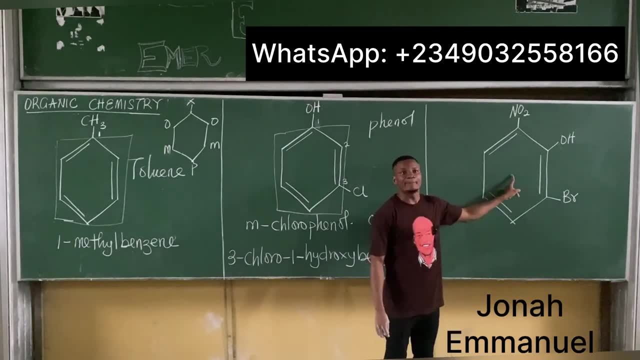 As a benzene derivative is phenol. as a benzene structure is OH, and this All right. Get this one done, please. In this case, OMP concept will not apply. Again, I am stressing: OMP only apply for what there. 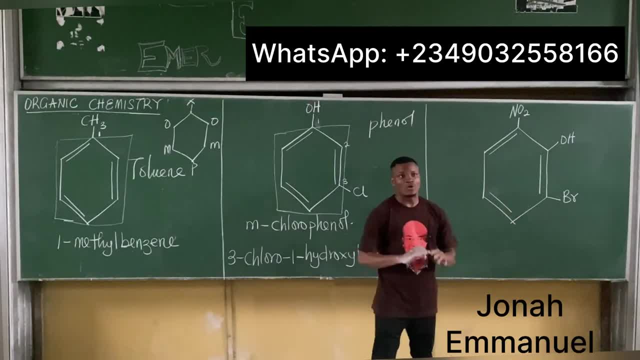 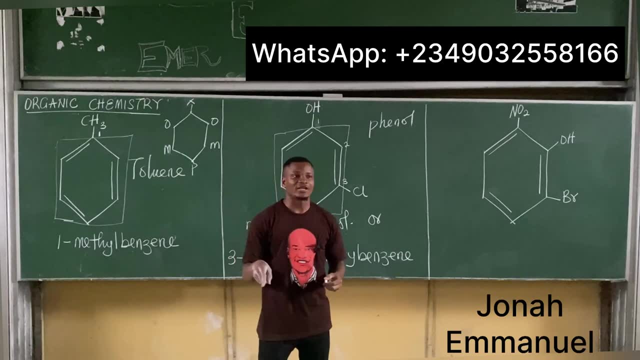 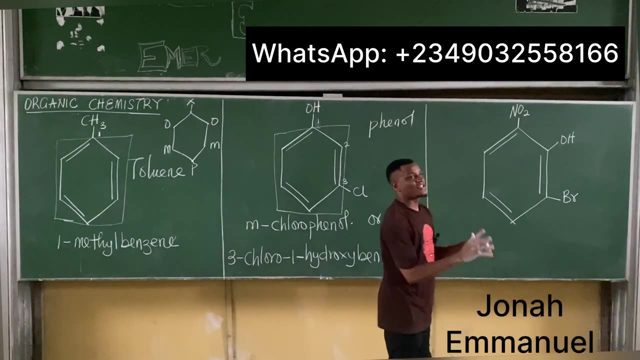 Two substituents, Two substituents, It's three substituents. OMP will not apply, So let's get this first as a benzene derivative and then as what? again there As a benzene. As a benzene derivative, it means I'm calling both the benzene and whatever is attached. 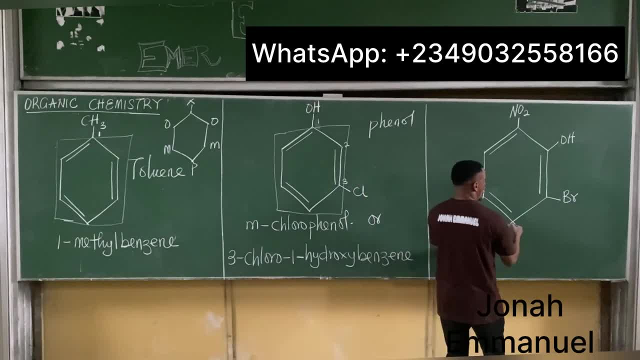 to the top as one. What will be there? Call all of this. What will be? If it's CH3, it's toluene. If it's OH, it's phenol. If it's NO2, this is what we call there- nitrobenzene. 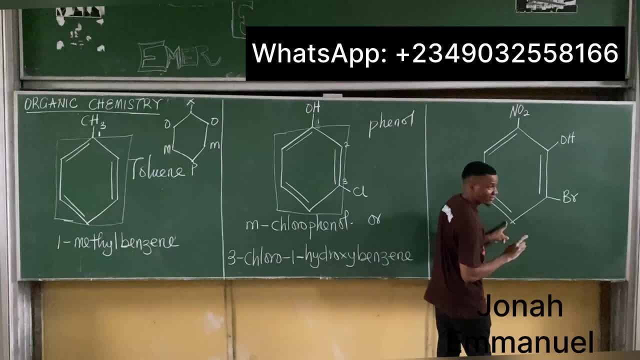 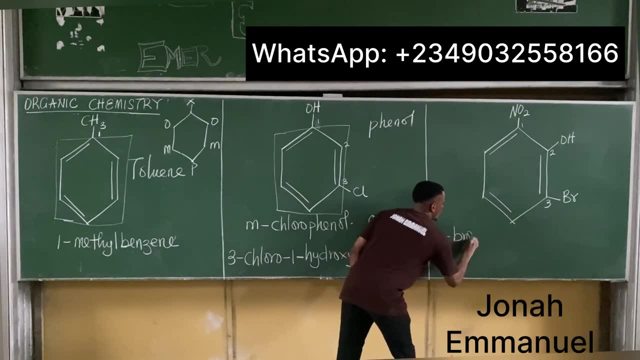 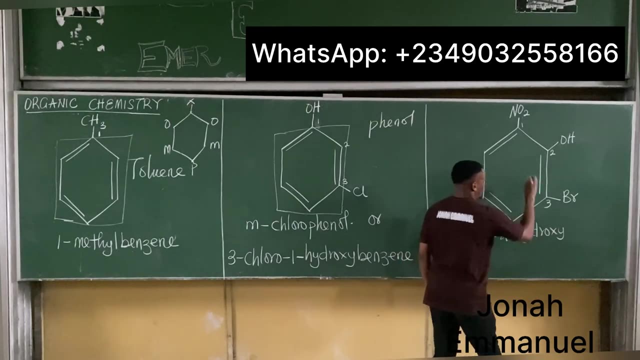 Since I can't use OMP here, what do I use there Numbering? I'm having one, two, three, So it becomes three-gromo-2-hydroxynitrobenzene. Okay, Or Now call this as a benzene structure. 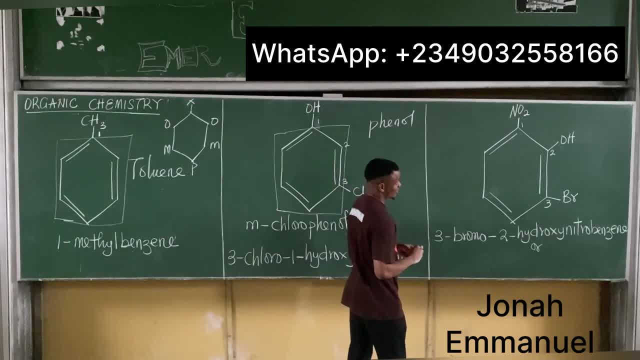 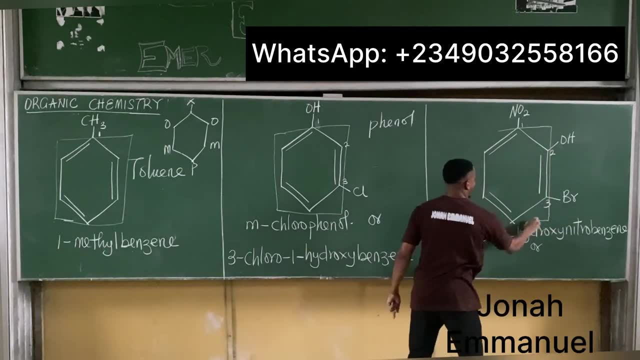 Well, this is not a proper benzene substituent. whatever, All right, Call this as a benzene. As a benzene- I'm taking this one here- It means that every attachment is now considered a substituent. So because what there? 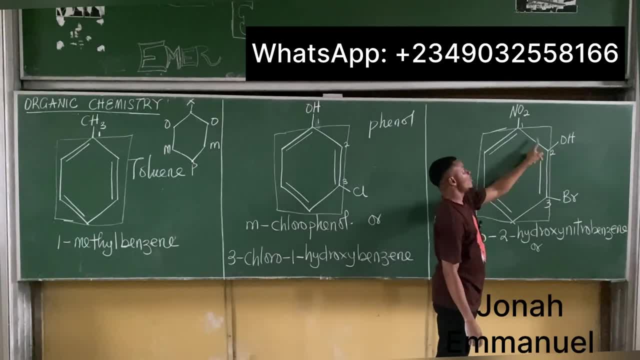 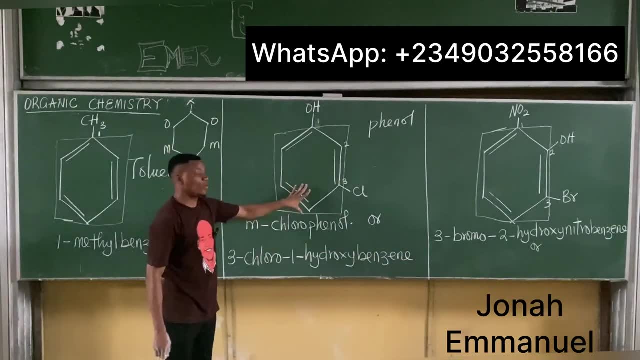 Three-gromo-2-hydroxynitrobenzene, So that's like. So the idea is this: Know when to use OMP and when not to. That's the idea: Know when to use OMP and when not to. 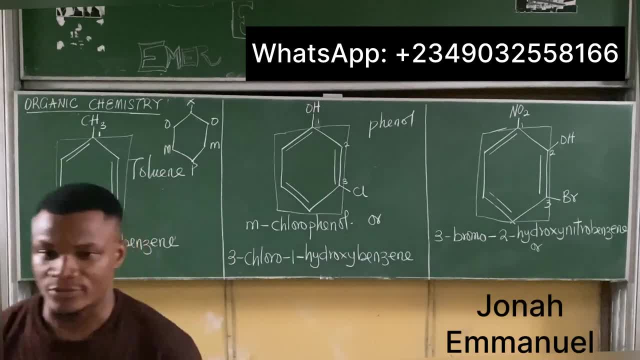 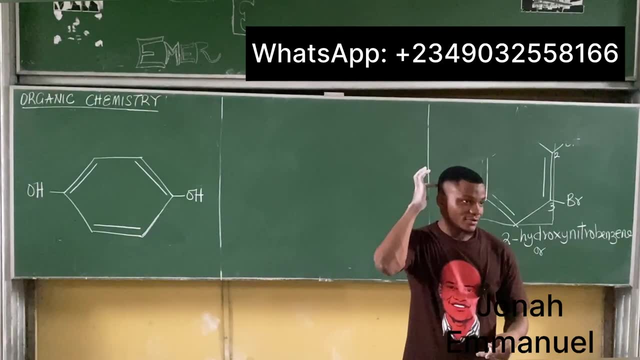 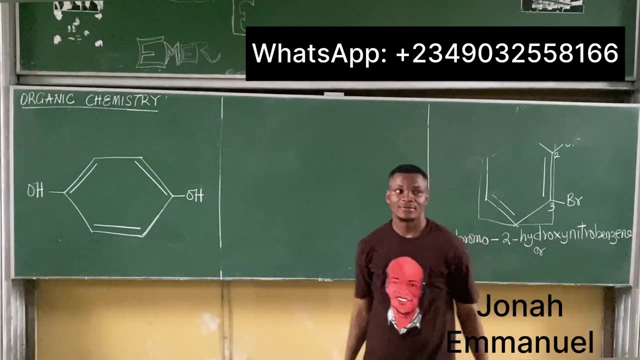 That's the idea. Let me give you other examples. What do you have here? Huh, Pdihydroxy, Am I having Pdihydroxy? So here they're just testing your mind by turning it off, just flipping it. 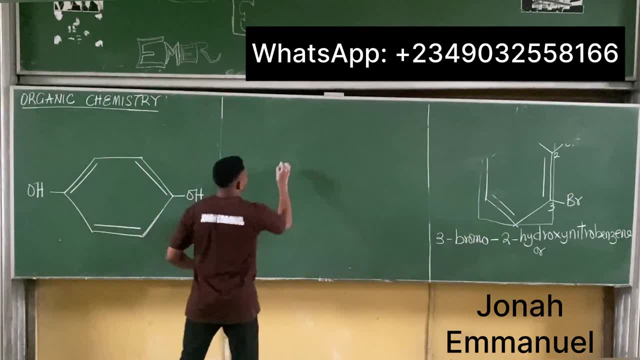 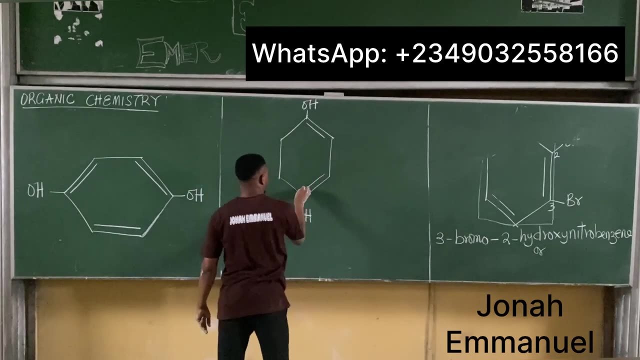 The same thing. Okay. So that means if I flip this man properly, I should be having something of this nature: perhaps Here is OH, Here is OH, Okay, This, this, this. So I have this. So if I flip, they'll have the same thing. 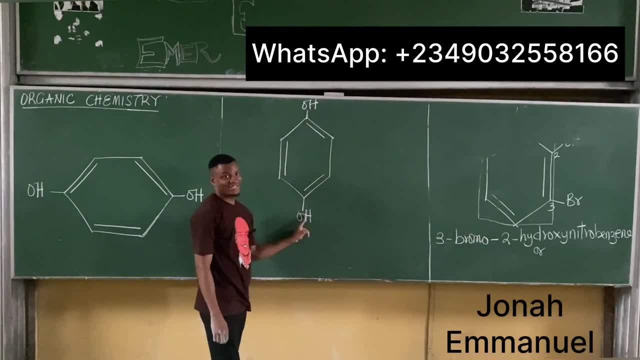 So how do you call this? Again, I have two substituents. OMP concept comes in OMP, P-hydroxy Phenol Becomes P-hydroxy Phenol. Consider this now as a benzene. 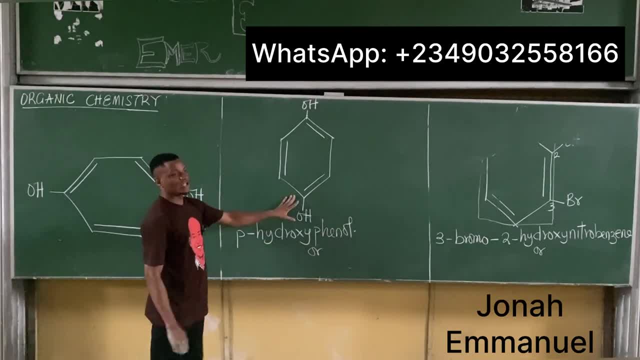 They can actually provide two names. Consider this as a benzene. What will it be there? One, two, three, four. So because one, there One, four. Di-hydroxy, P-hydroxy, P-hydroxy. 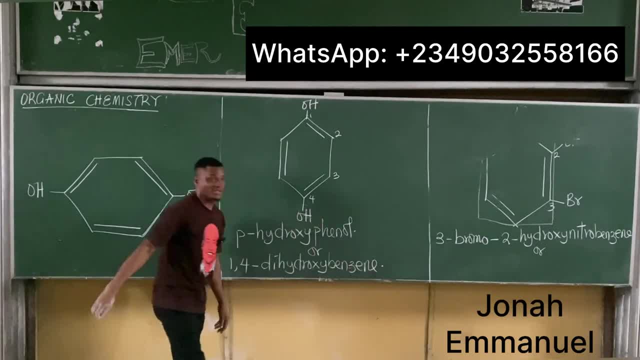 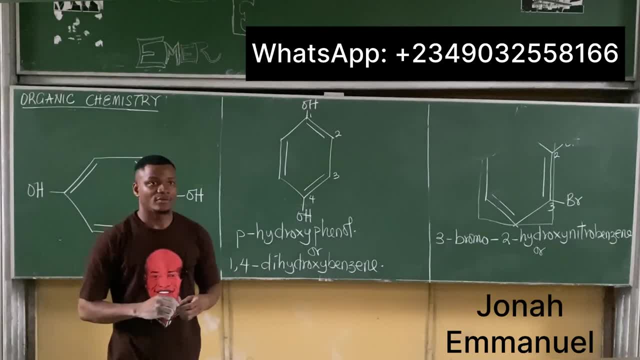